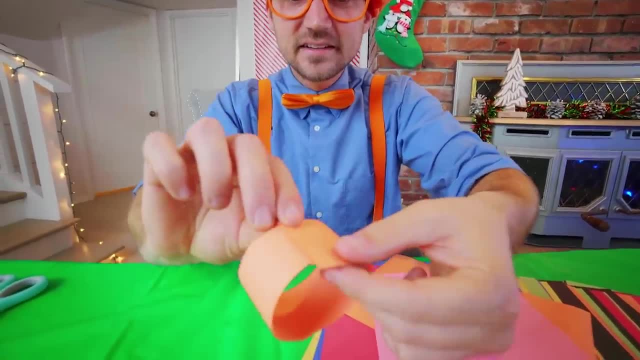 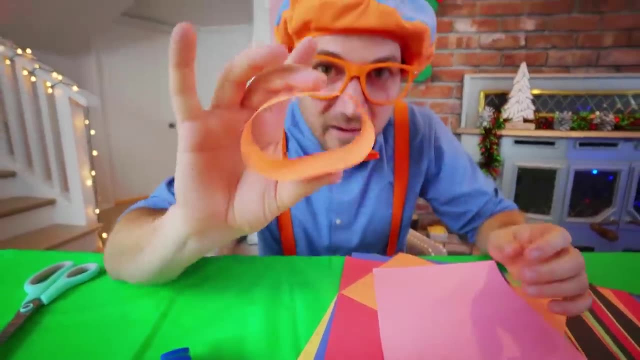 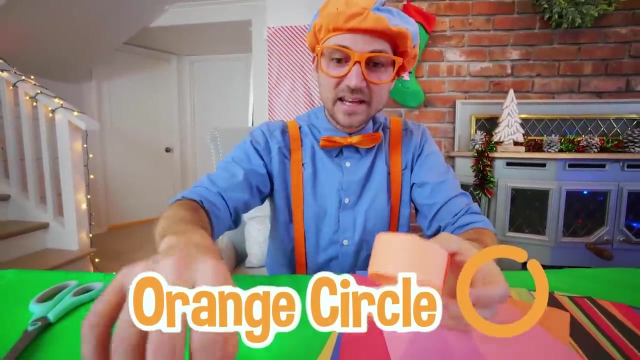 to wrap this around from end to end. Yeah, just like that. Then take your stapler and staple it down. Oh hello, Wow, it's an orange circle. All right, now what we're gonna do is take a pink stripe. 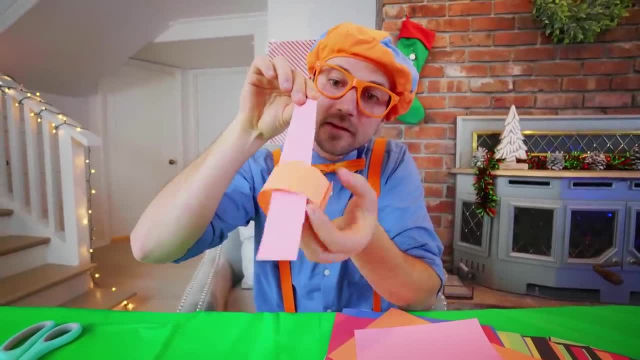 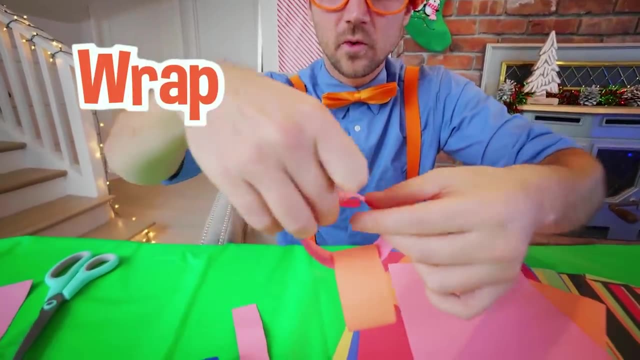 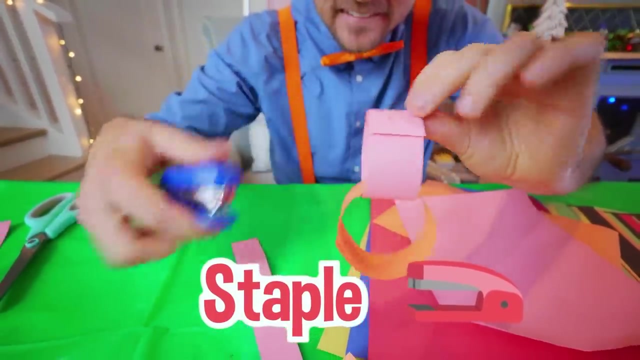 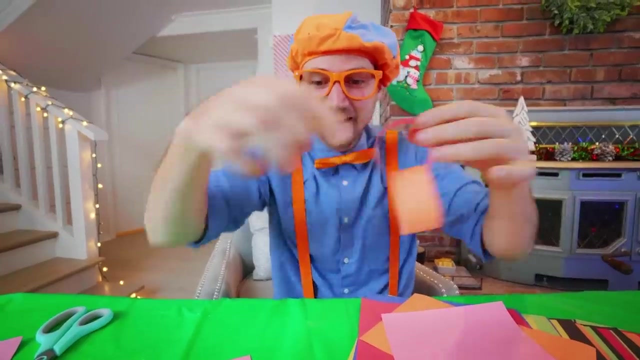 Put it through the orange stripe. There we go. Yeah, perfect, We did it. Look at that, Yeah, Okay, now we're gonna wrap that around the orange stripe, Okay, and then we're going to staple that one together. Whoa, do you see what we're doing? Yeah, now they don't even come apart. Okay, let's put. 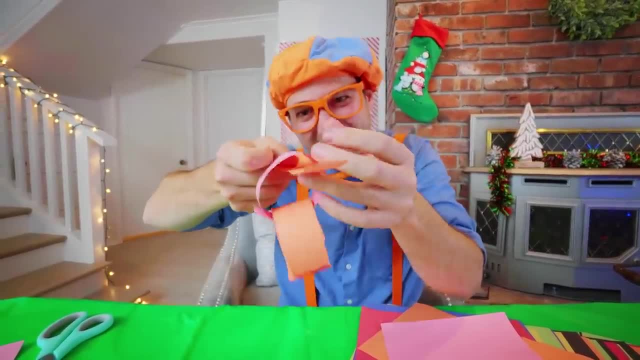 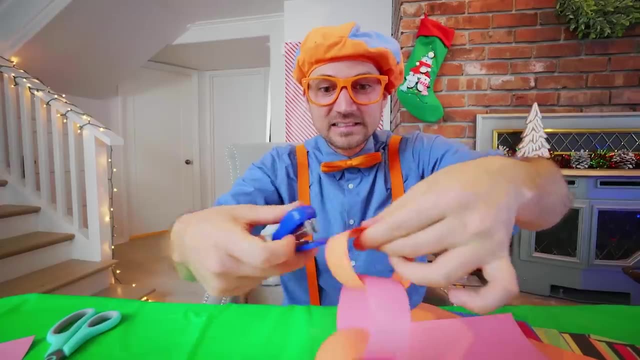 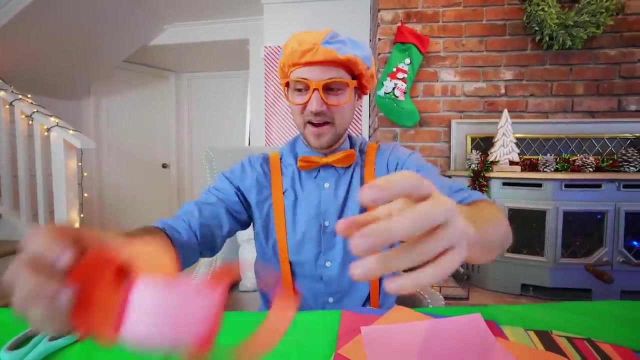 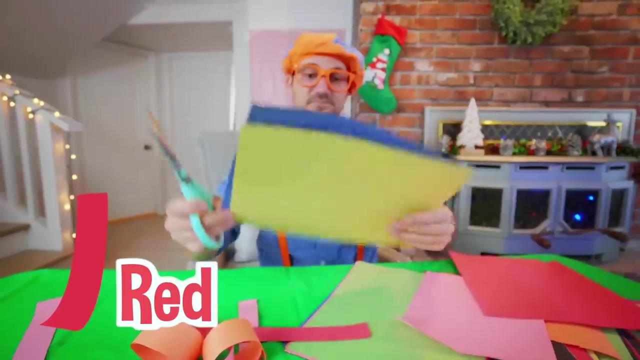 the orange one through, Yeah, see, And then loop it around And then staple it. Whoa, Whoa, So cool. All right, I think we're ready for some more colors. Okay, let's take some red. How about blue and yellow? 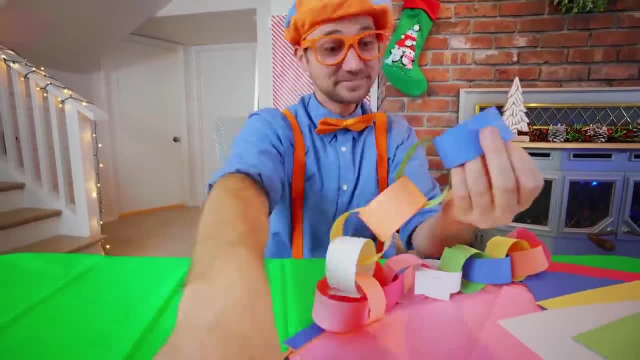 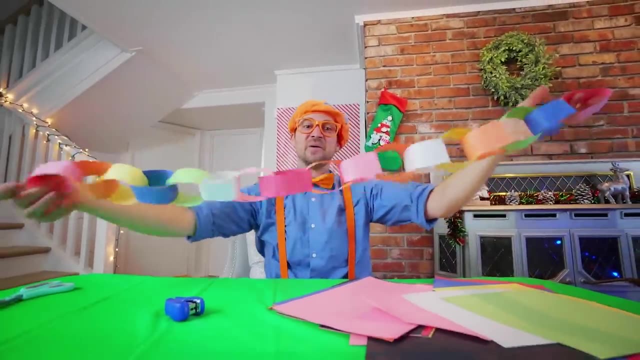 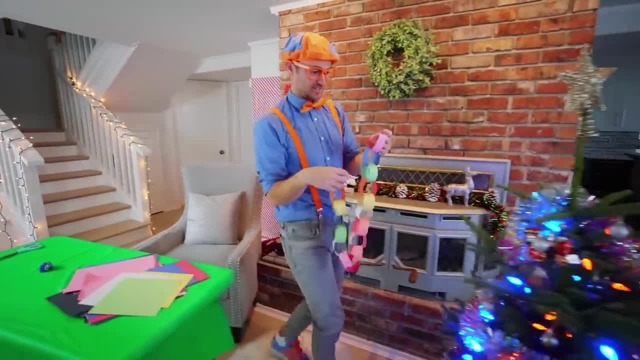 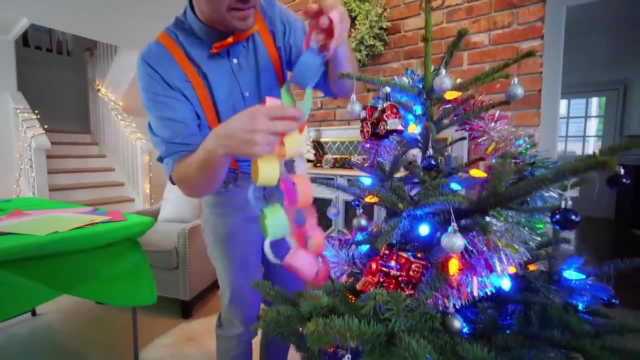 So now what you want to do with your chain is go to your Christmas tree, Yeah, And then you wrap it around the tree. How about, right, Let's start right here. There we go. That looks like a great place to start. 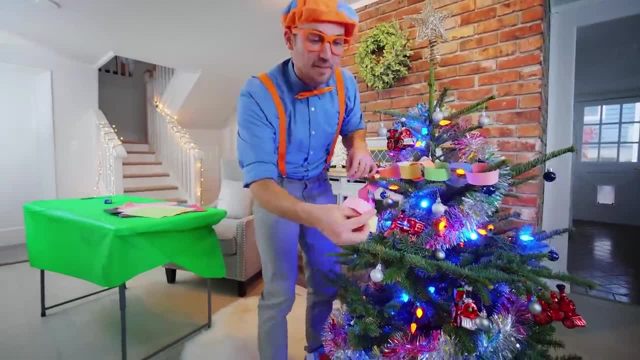 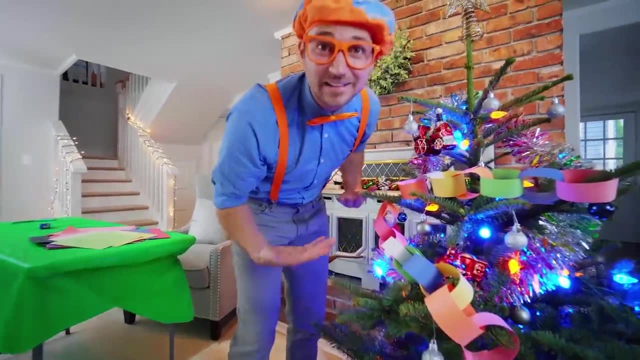 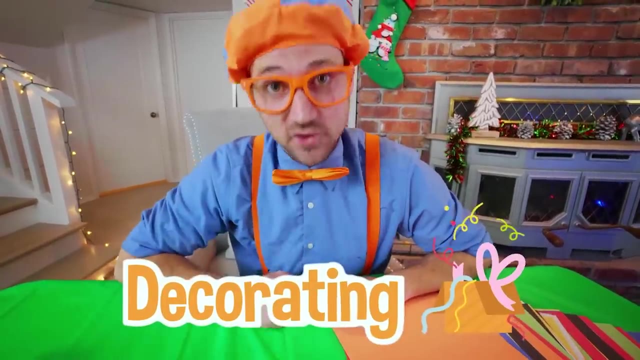 And then I'm going to wrap it back this way. I'm not even going to go around the whole tree. Okay, How about like that? How does that look? Yeah, that is awesome. We have done such a great job decorating this Christmas tree together. 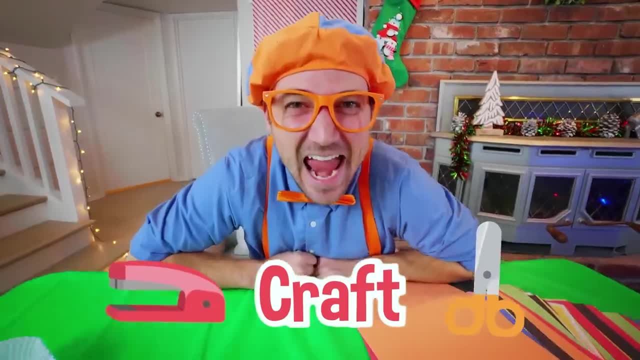 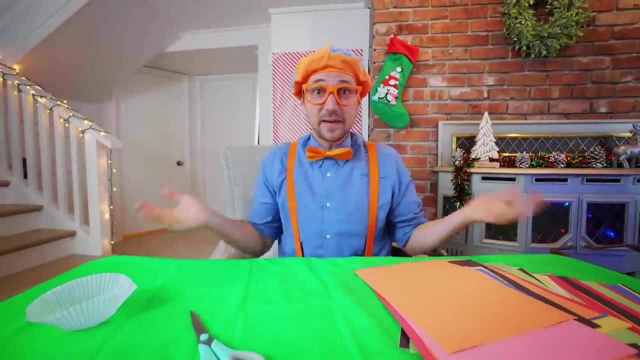 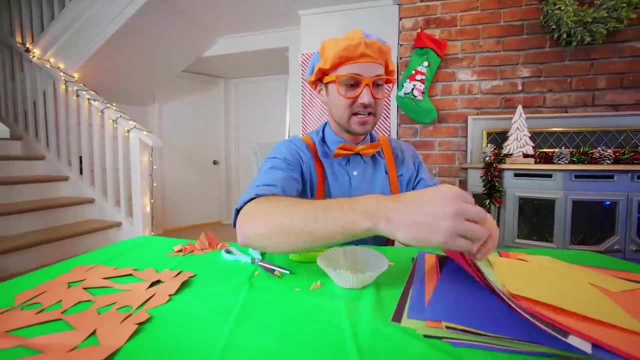 But we have another craft to make. Yeah, And this craft is a snowflake ornament. Yeah, Have you ever seen a snowflake before? Yeah, It's basically just frozen rain falling down from the sky. Wow, How about Just a plain white one? 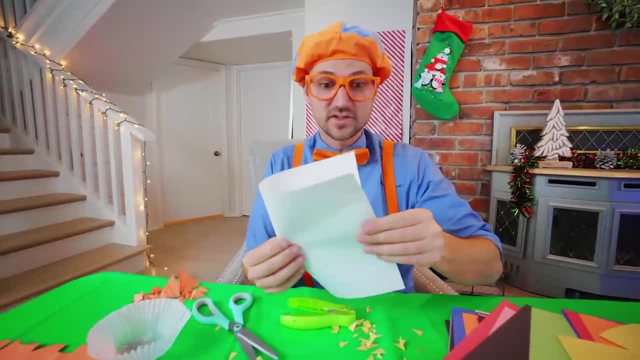 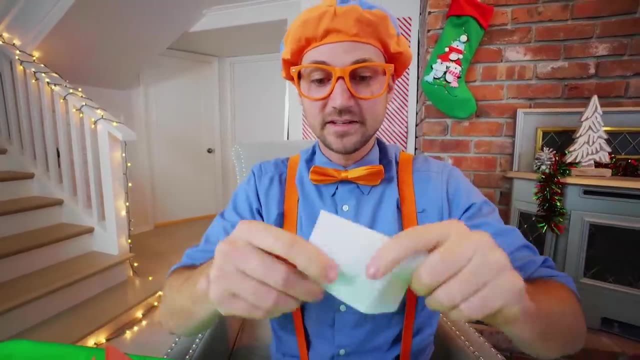 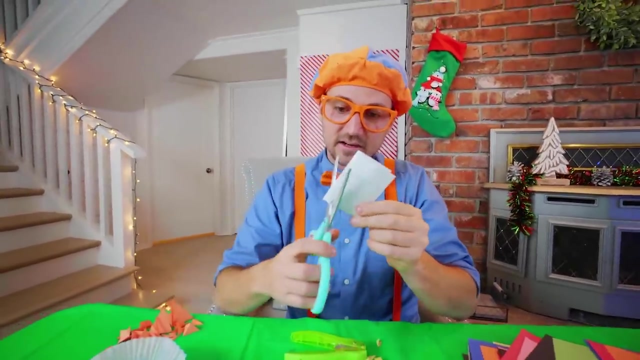 Yeah, That's like the color of real snowflakes. And this one, let's make another big one. There we go, Let's fold it, fold it and fold it. There we go. Okay, Now let's do a little bunch of cuts. 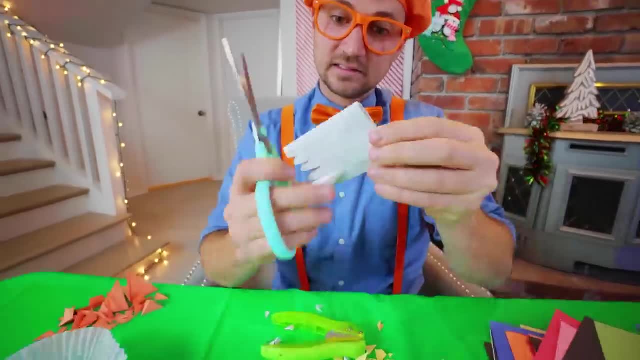 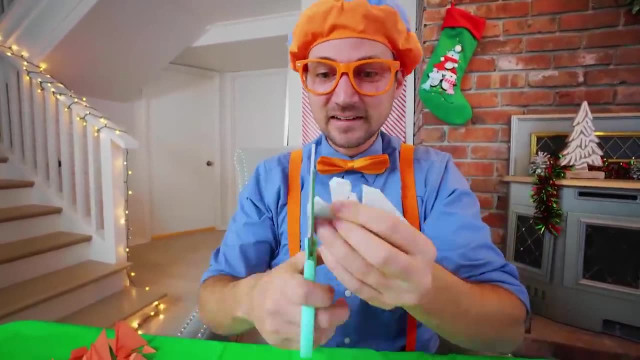 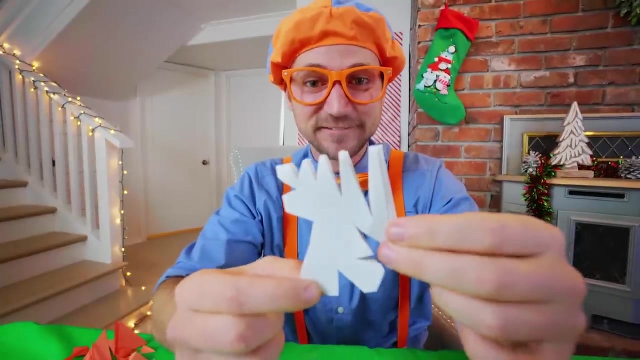 Let's do a bunch of cuts. Let's do a bunch of cuts. Let's do a bunch of cuts. Wow, All right, How does this look? Do you think this is going to turn out really cool? Yeah, Hey, I have an idea. 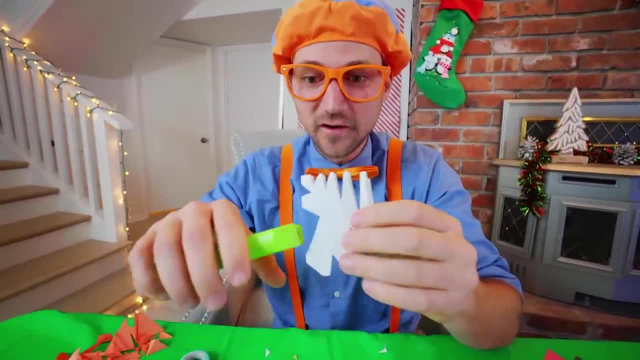 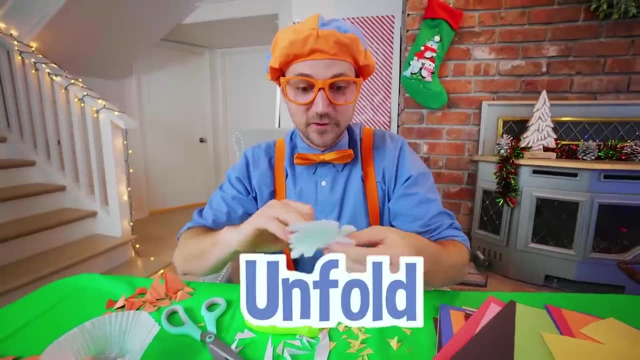 Why don't we take a hole puncher and punch in a hole at this stage? That's cool, Okay, Oh, it's a little tough. Oh, actually we might need to unfold it one time. Whoa, Speaking of unfolding it, it looks so cool. 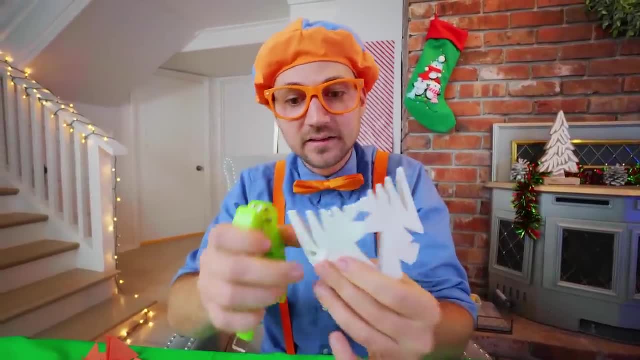 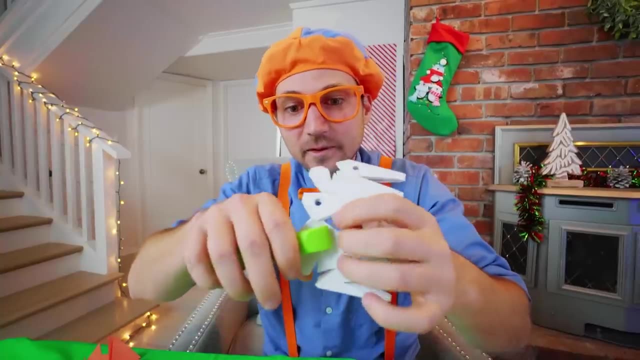 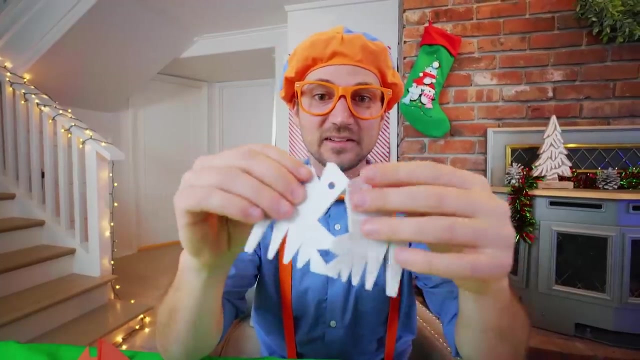 I can't wait to see it. All right, how about let's make a hole punch right there? Whoa, let's make a hole punch right here. Yeah, another one right here, And another one right here. Okay, now let's unfold it. 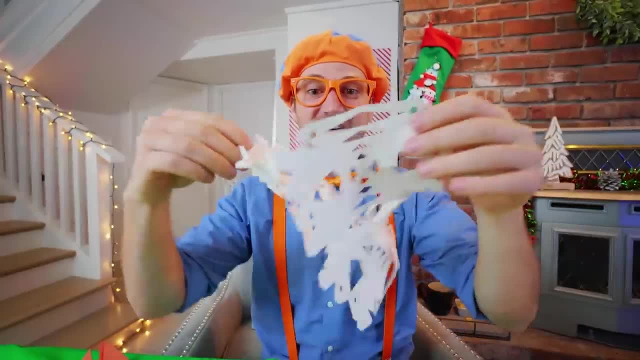 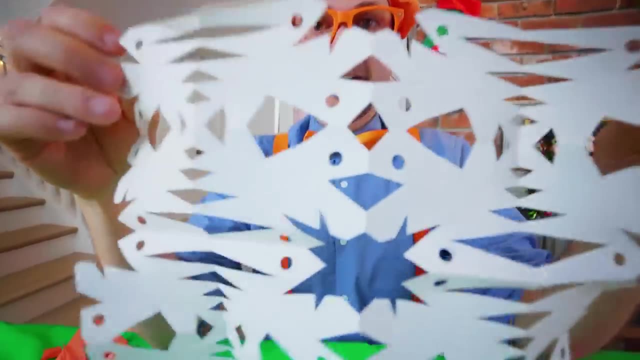 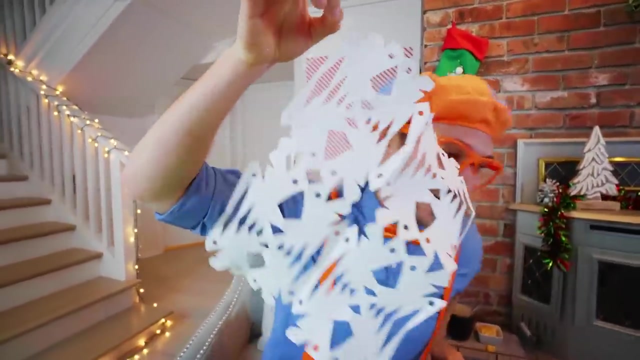 Whoa, whoa, whoa. This one is awesome. Whoa, All right, we definitely have a lot of holes already punched in it, So I think we should just hang it up and put it on the tree. Whoa. 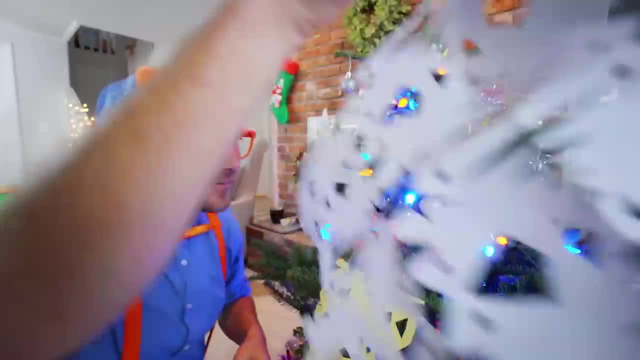 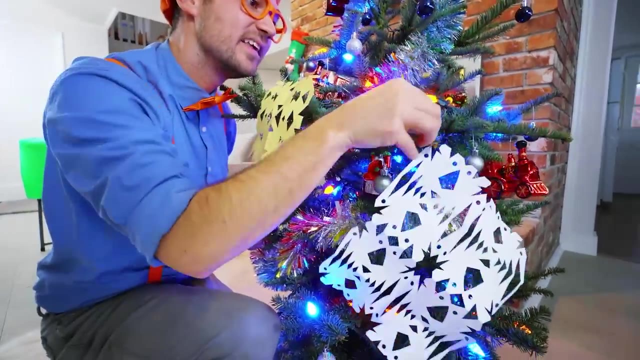 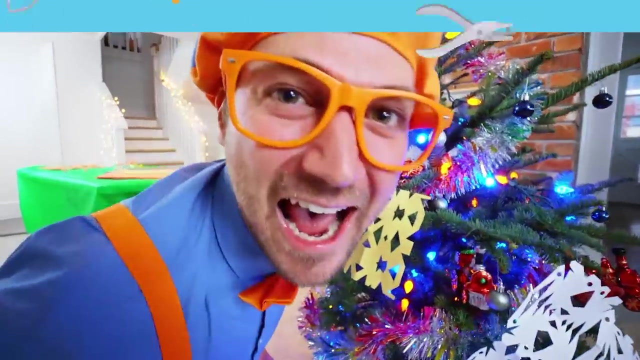 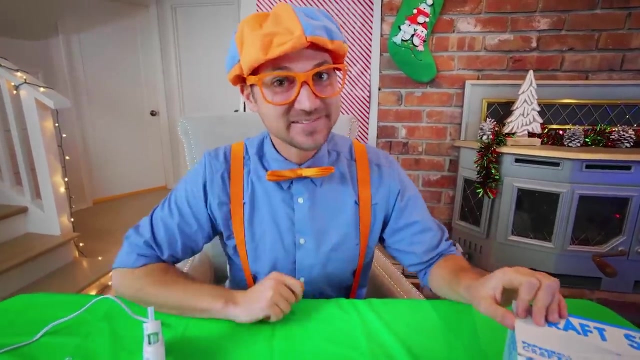 Okay, here we go. How about right over here, Right there? Yeah, that looks great. How does that snowflake look? Yeah, good job. Wow, we have done such a great job decorating this tree, But we're not done yet. 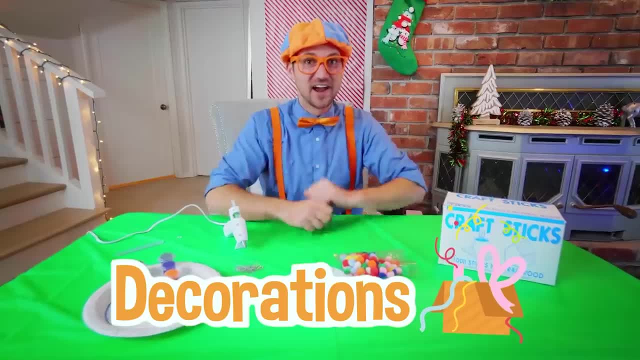 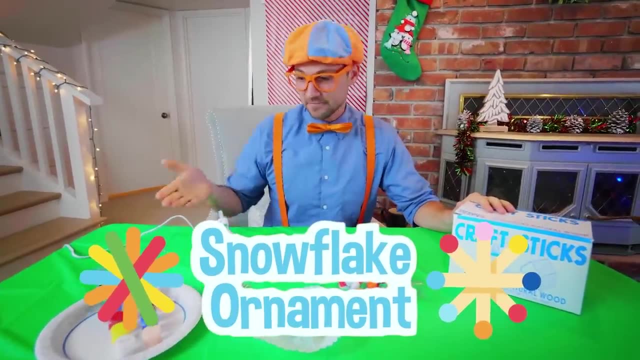 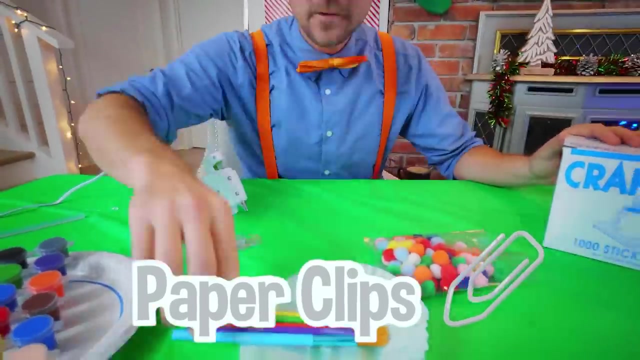 Yeah, we need to continue the decorations with another at-home ornament, And this is a snowflake ornament. So what we have here, as you know, we have some colorful paint, a hot glue gun, some paper clips, some paint brushes for the paint. 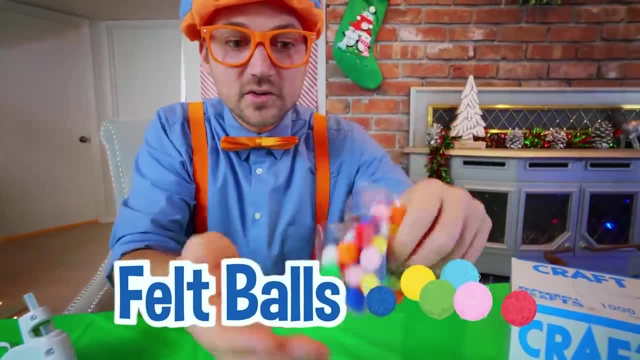 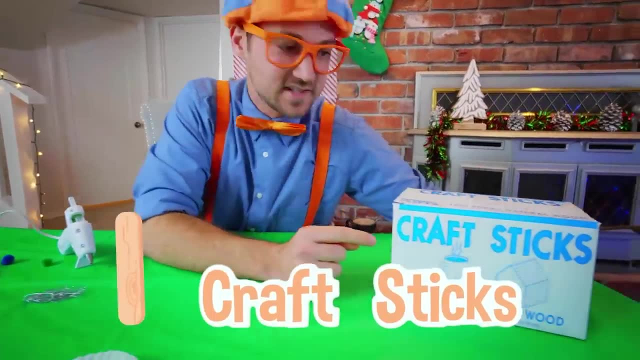 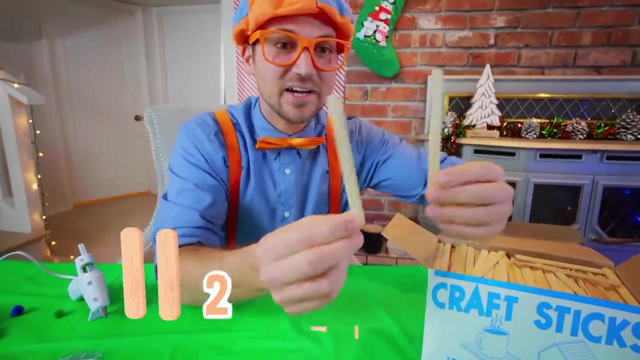 some felt balls- Wow, they're so colorful, Look at them. And we have some craft sticks. Yeah, you've probably seen these before, haven't you? Yeah, they're like popsicle sticks. Yeah, two popsicle sticks. 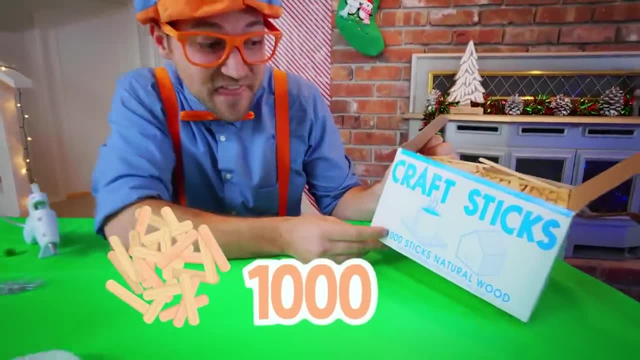 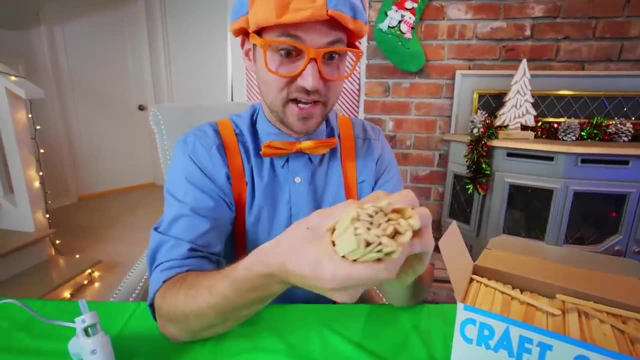 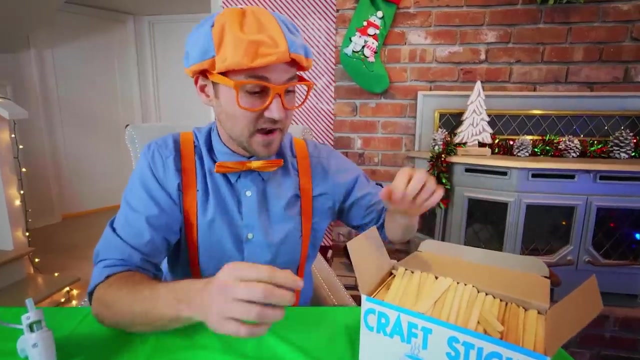 Whoa. and it actually says there's a thousand sticks Whoa, that is a lot of popsicle sticks. Okay, well, I think we should probably count them, so then we can make sure that we got all a thousand of them. 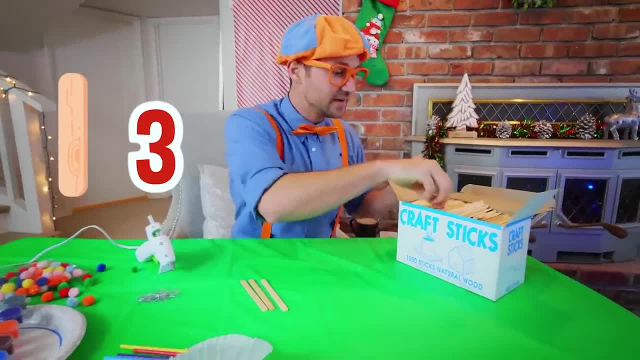 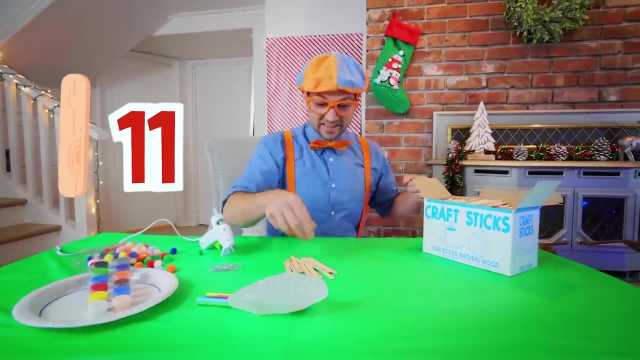 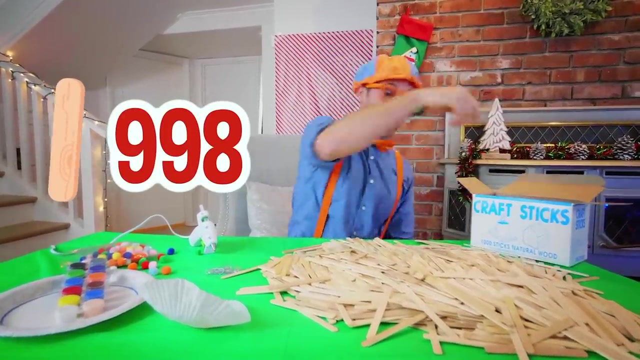 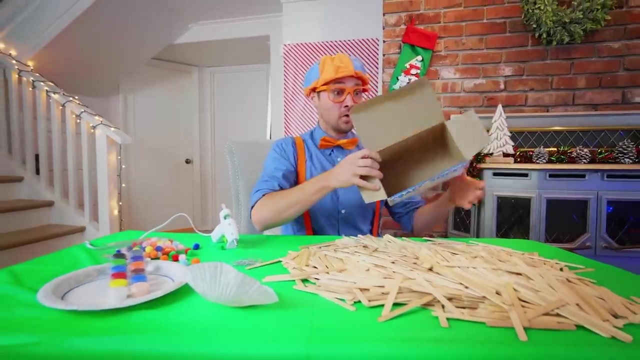 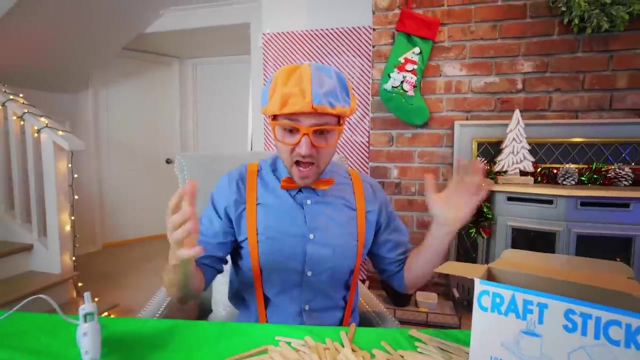 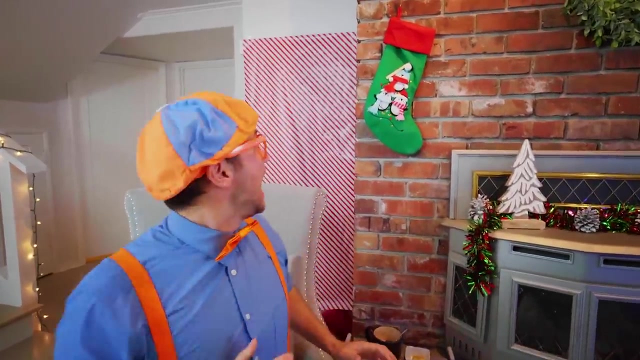 Ready. One, two, three, four, five, six, seven, eight, nine, ten, eleven, 997, 998, 999.. Oh no, 999.. Where's the thousandth? Oh no, Hey, yeah, you're right. 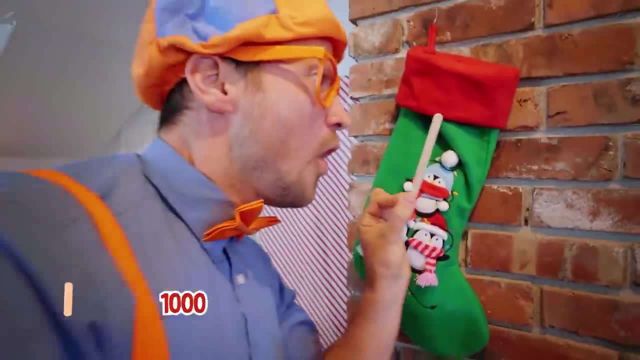 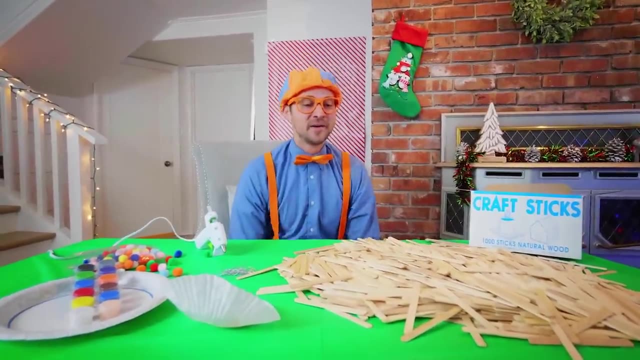 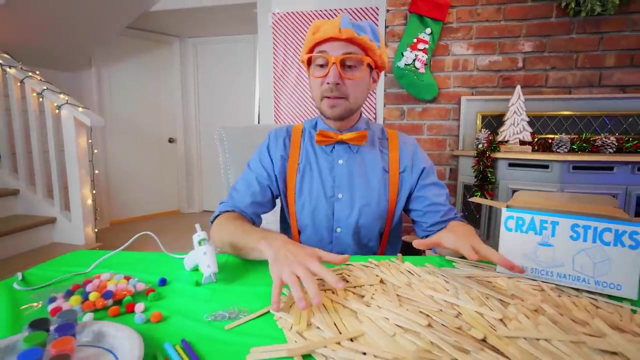 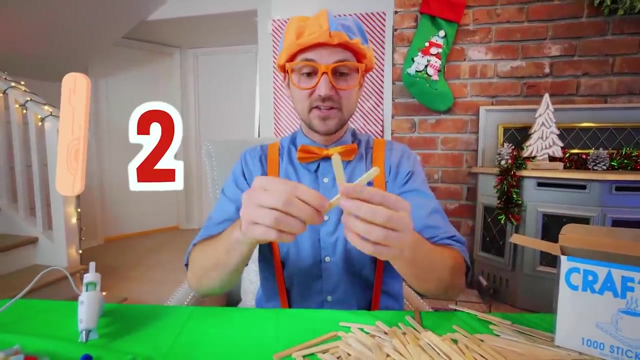 Right up here You got it: 1,000 popsicle sticks, Yes, Okay. well, we should probably get going on our craft now. huh, Now that we have all these popsicle sticks in all of our crafts, Okay. so first let's take one, two, three and four popsicle sticks. 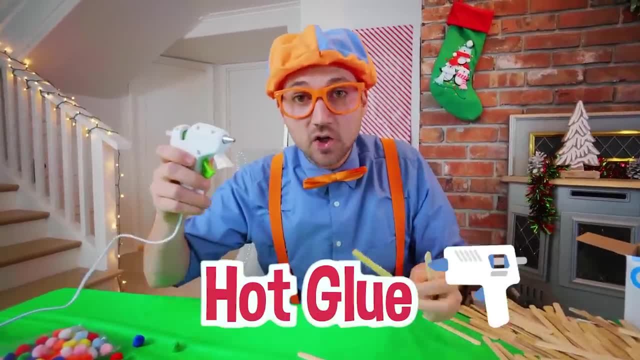 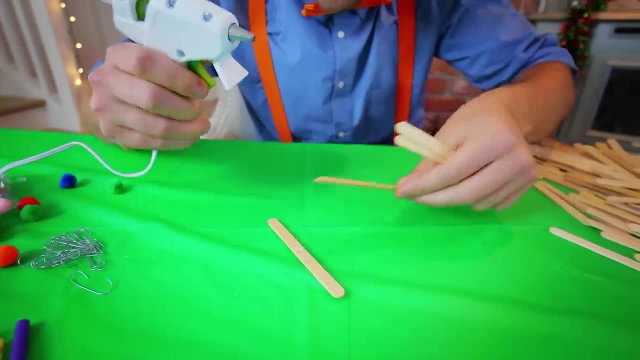 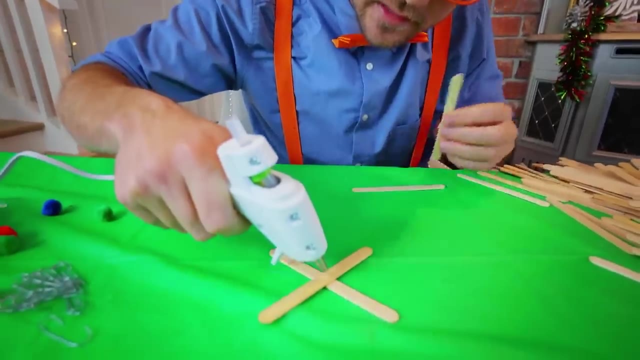 And let's super glue- actually hot glue- them together. So let's put just a little bit right in the center And this is very hot, so I would assume a grown-up will help you with this. okay, I'm going to put another one right there and then put it just like that, okay. 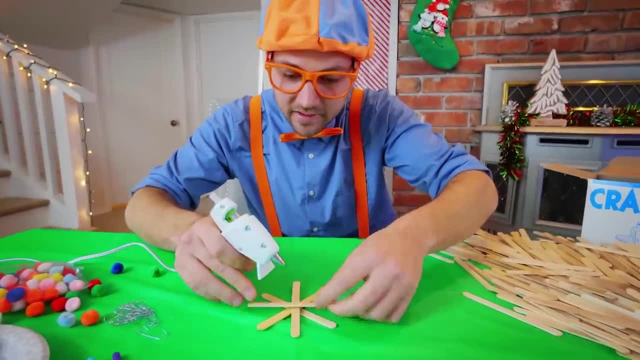 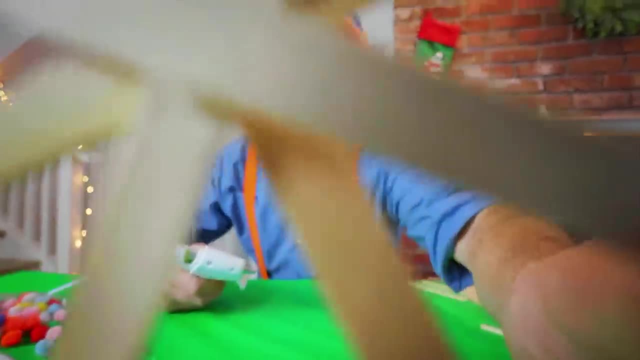 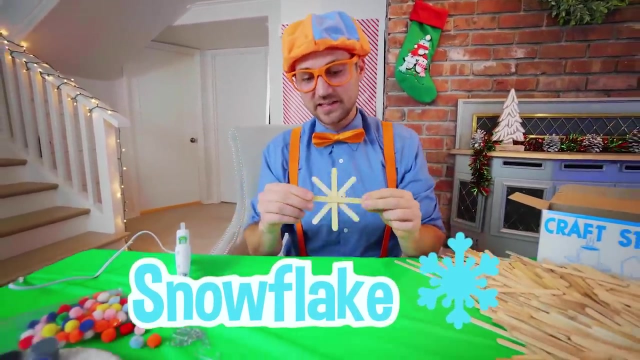 Another one right there and we're going to go just like that. Yeah, how does that look? Whoa, whoa looks really good. huh? Yeah, looks like it Looks like a snowflake. Okay, we're not done yet. 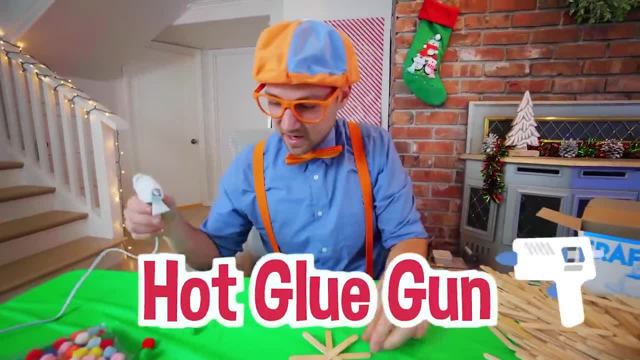 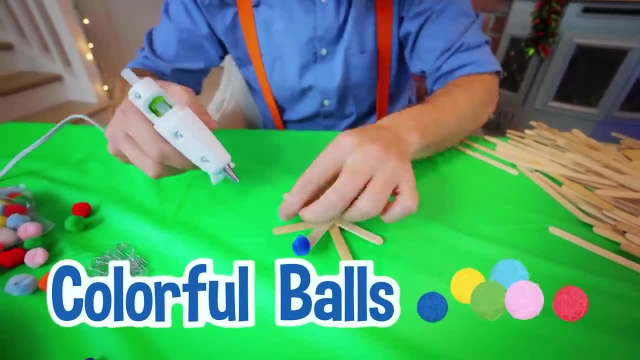 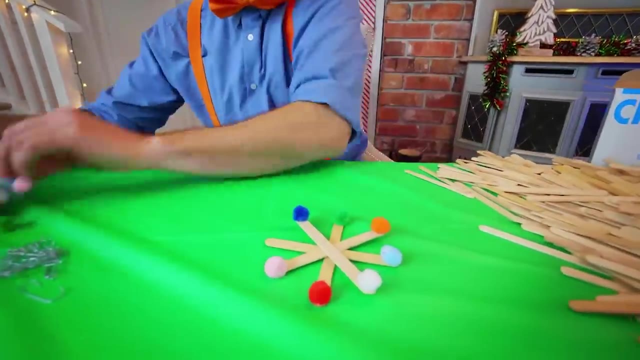 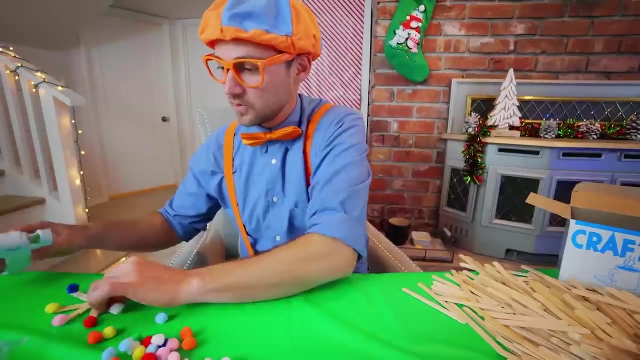 We need to decorate the snowflake, So I'm going to take the hot glue gun and put some right on the edges and put some of these colorful balls. Wow, How does this look? Yeah, Yeah, Okay, we'll let that sit right over there. 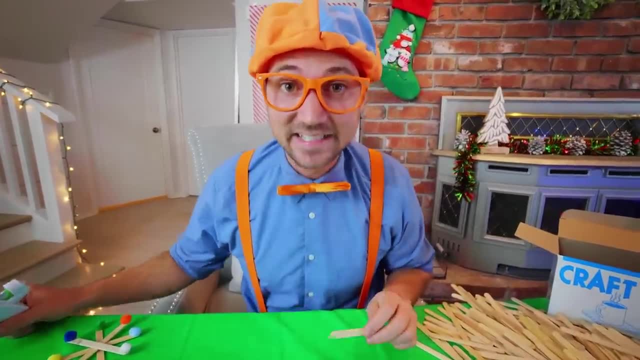 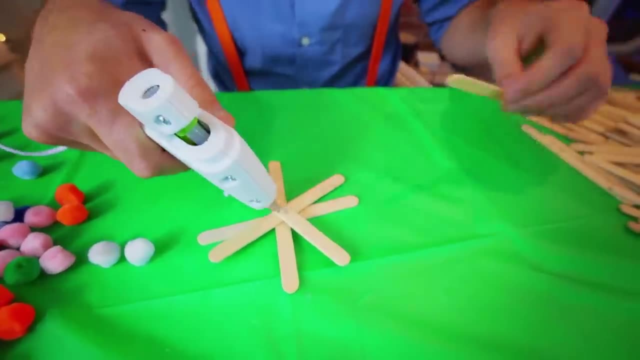 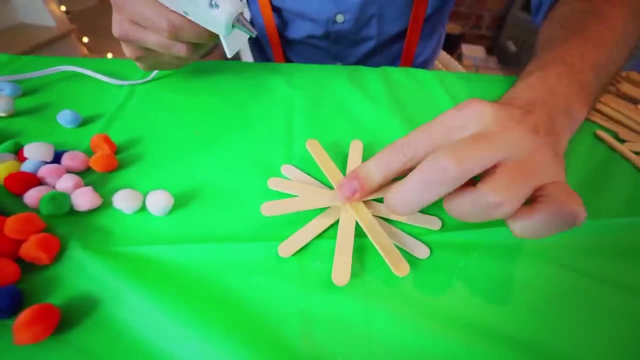 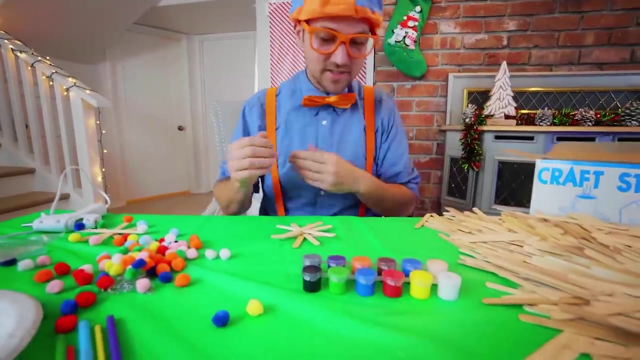 Now we make another one, and this one we'll use paint. Look at that, Hey, I think we have room for one more Now. that looks like a great snowflake, Haha. Okay, Now this one. let's use some paint. 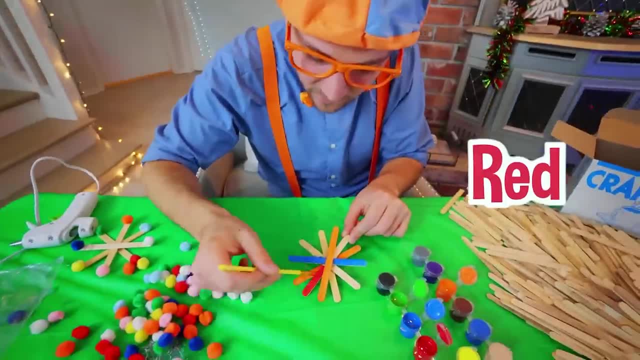 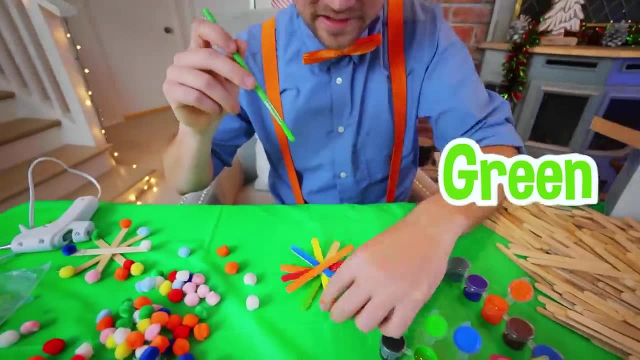 Orange, Blue, Blue, Red, Yellow, Green. Wow, Looks really good. Do you like it? Yeah, I like it too. Wow, Turned out really good. Let's look at all the colors We have: green, Yellow. 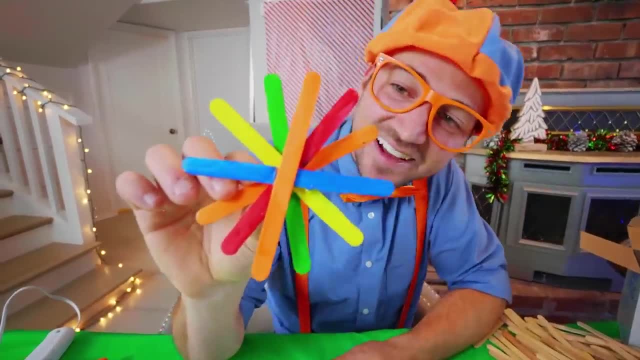 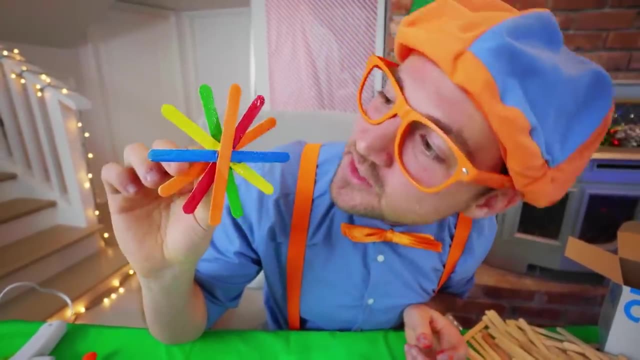 Blue, Orange, Blue, Red, Yellow, Blue, Red, Yellow, Green. Wow, Looks really good. Do you like it? Yeah, I like it too. Wow, Turned out really good. Let's look at all the colors. 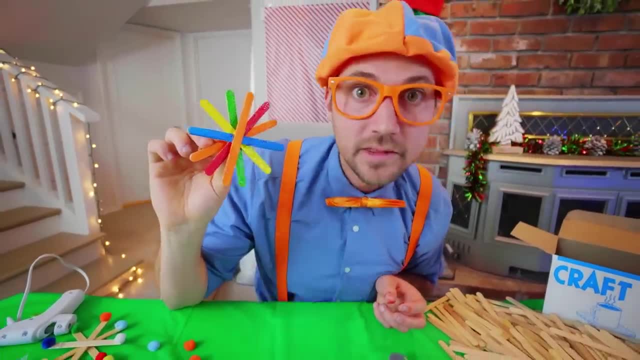 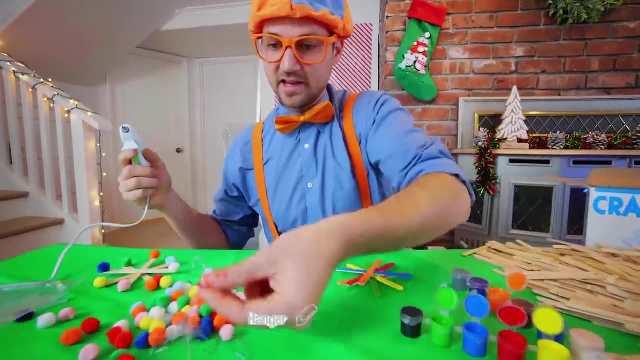 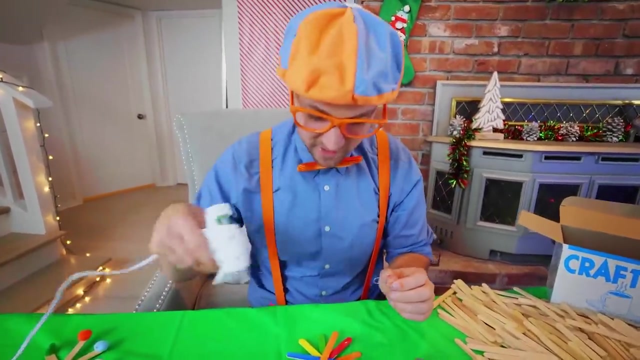 Orange, Red And that's all. Haha, Okay, Well, last step, We need to hot glue another hanger on the top. Yeah, there we go, And you could actually hot glue some of these soft balls on it too, but we're not gonna. 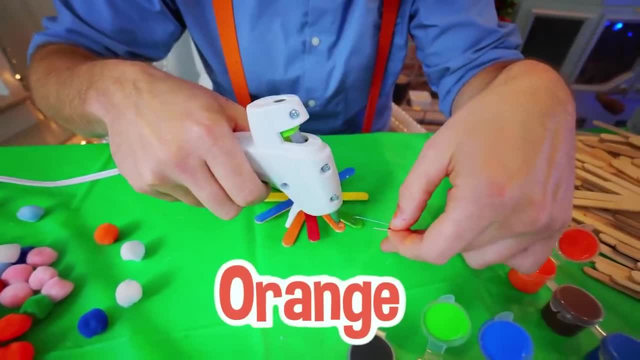 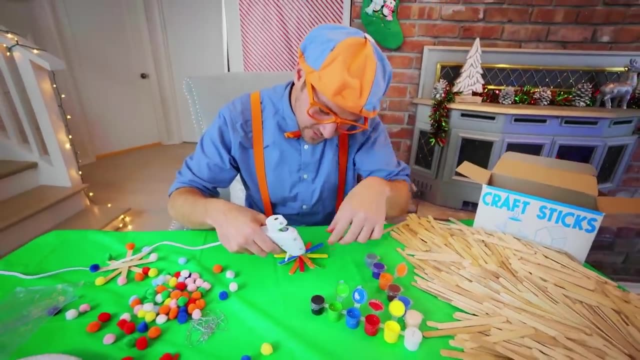 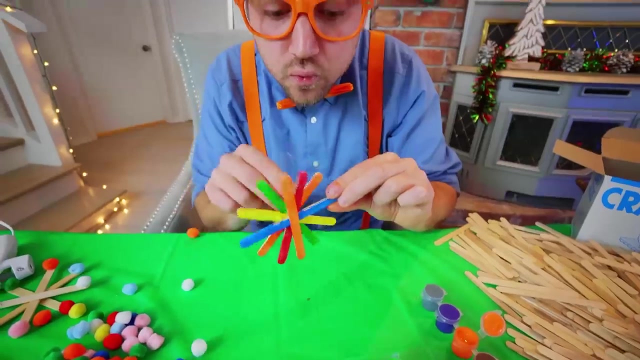 We're just going to hot glue right on the orange, because that was the first color we did, So it's actually nice and dry. There we go, Perfect, Awesome. That looks really really good. Okay, We'll let this one dry, but I think in the meantime we should take this one, the one. 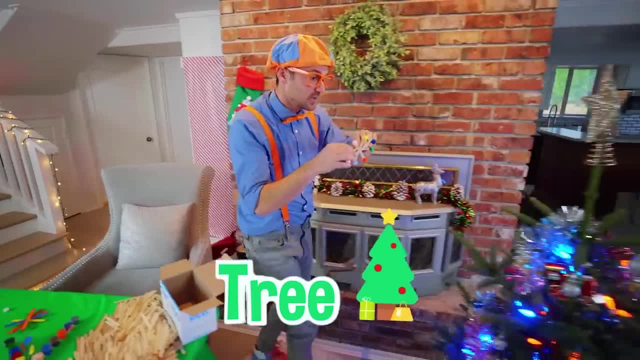 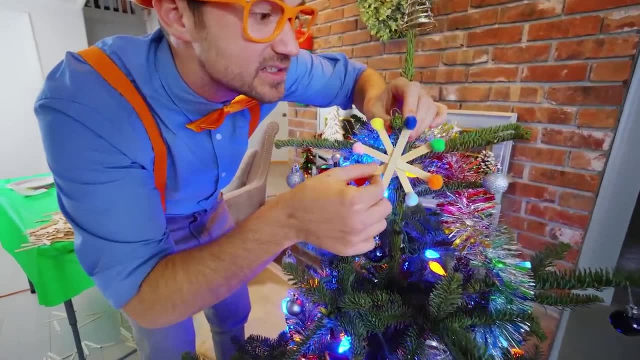 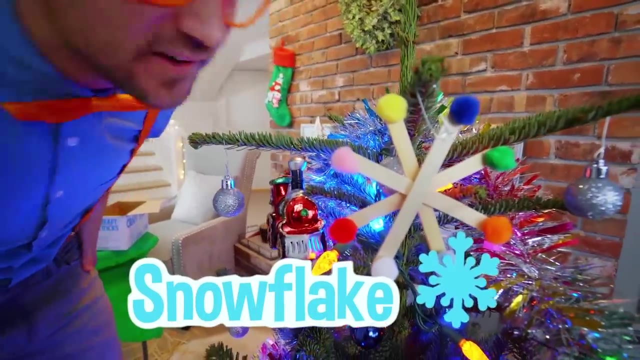 we did earlier- and put it on the tree- Wow, Okay, How about right near the top? huh, Yeah, Let's take the hook, Hook it right there. Wow, How does that snowflake look? Wow, I love it. 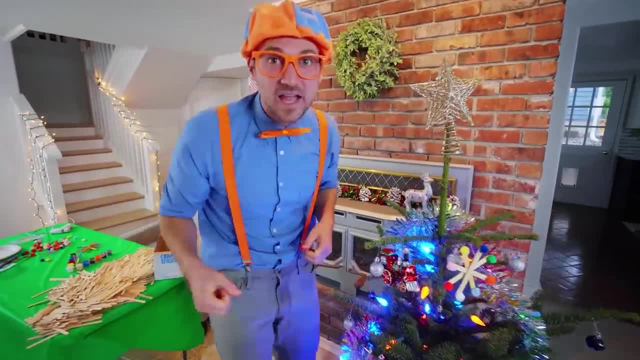 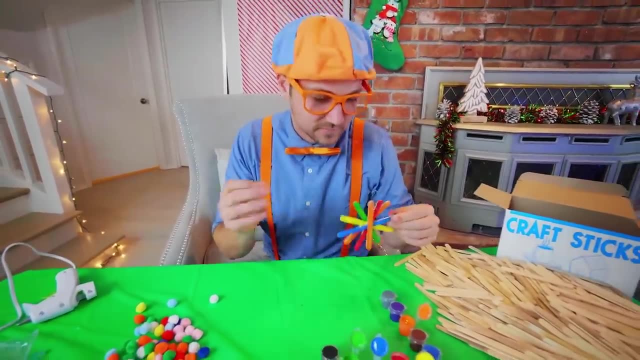 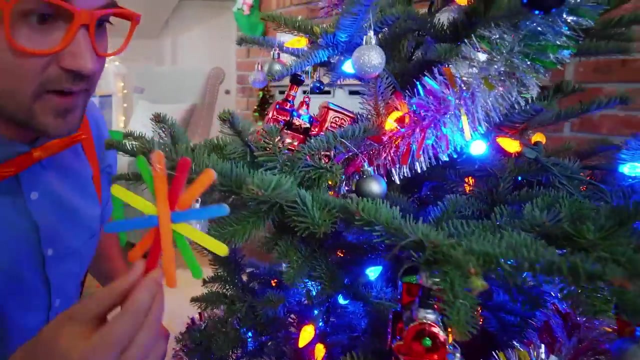 Good job, Haha, Okay, I think we should go get the other one. Ooh, Haha, Okay, Yep, I think it's dry. Okay, Perfect, All right, How about right down here? Yeah, Wow. 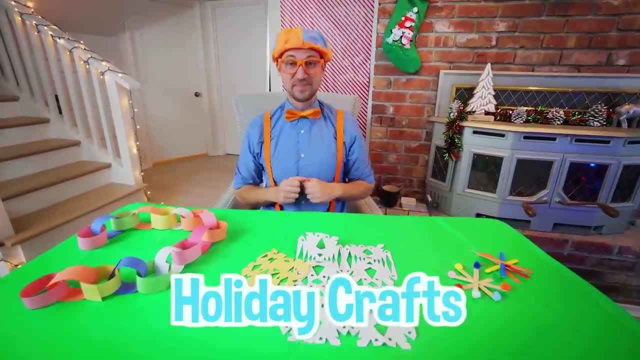 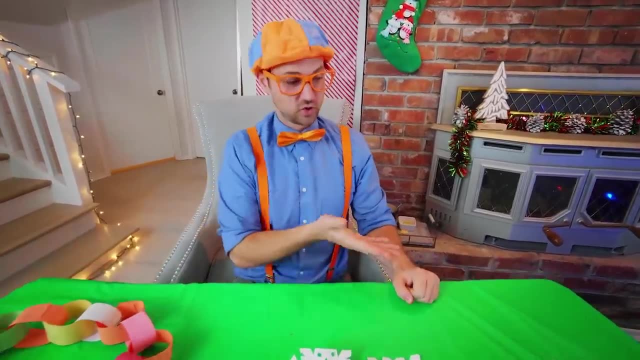 Look at all of these holiday crafts we made together. Whoa, Did you have fun? Yeah, I sure did too. I really enjoyed making all of these with you. Well, I'm excited to see what ones you make this year. Yeah, 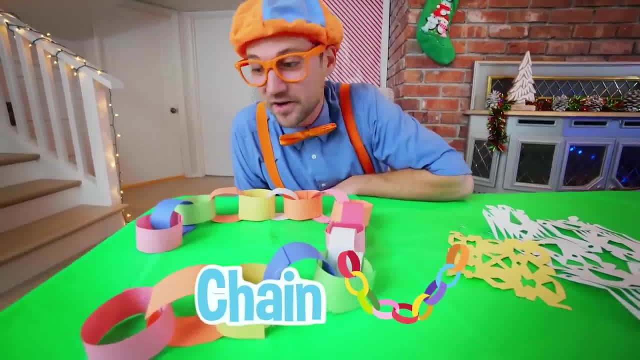 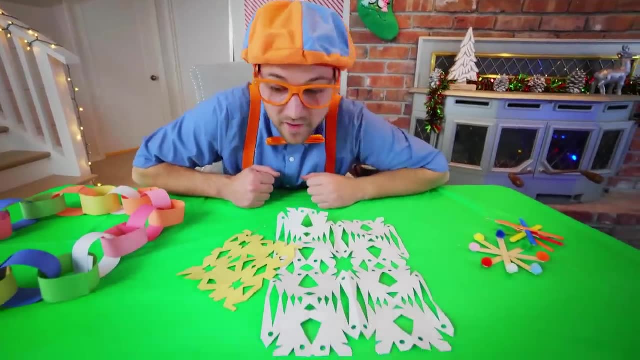 Are you going to make the chafe? Yeah, What a great tree decoration that is. You could also probably hang it from a wall, Haha, Whoa. What about the construction paper snowflakes? Wow, They look so cool, huh. 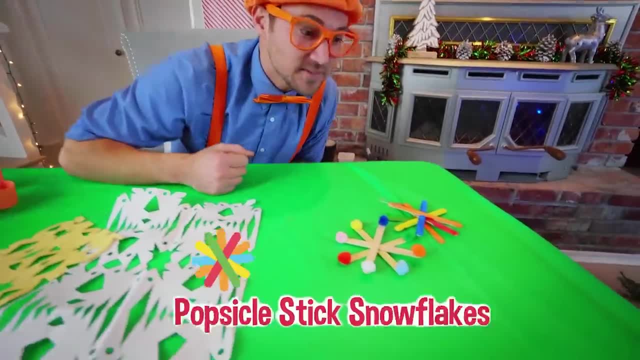 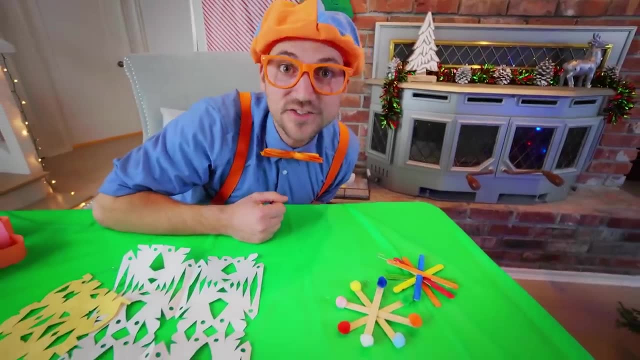 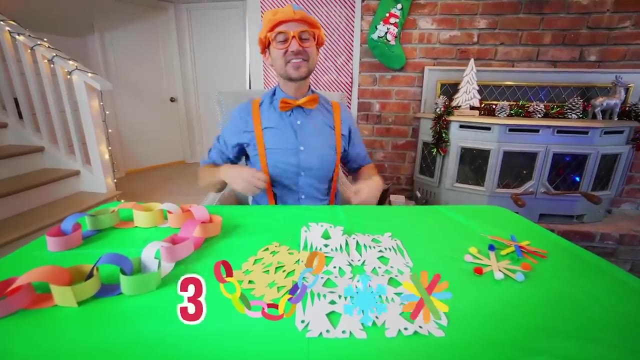 Yeah, Haha, Ooh, The popsicle sticks. Yeah, The snowflakes made from popsicle sticks. Wow, Those are also so cool and colorful. Maybe you'll make just one, Maybe you'll make all three, Yeah. 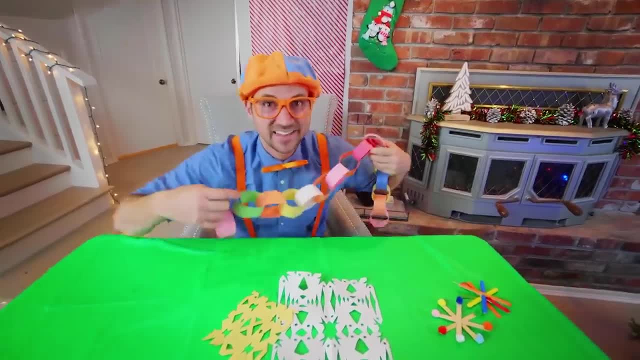 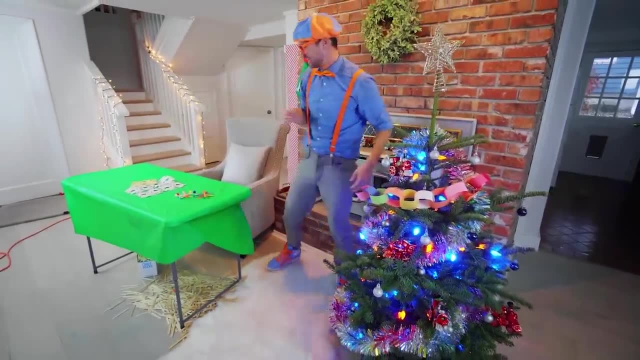 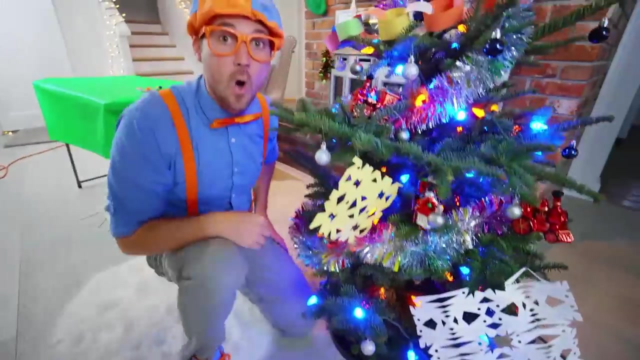 Well, I can't leave before decorating the tree one more time. Okay, How does that look? Haha, Real good, That looks really good. huh, Whoa, So cool, Whoa, These are so colorful. That looks perfect, huh. 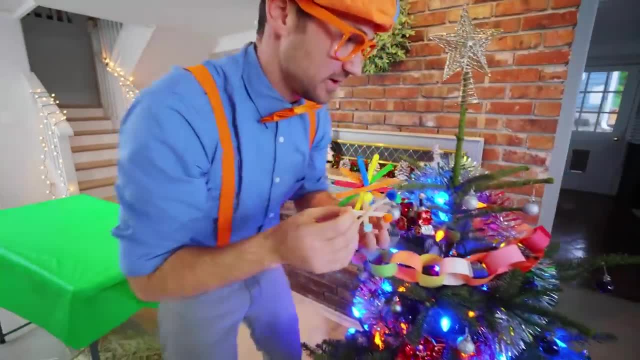 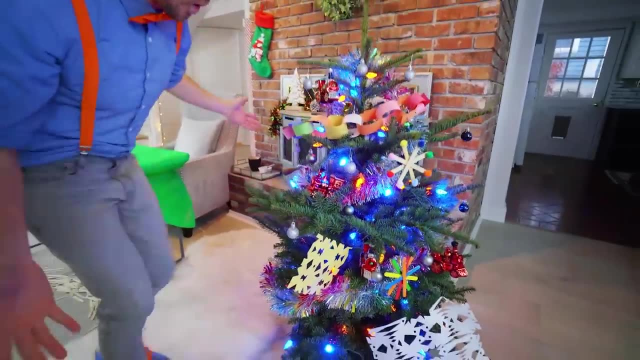 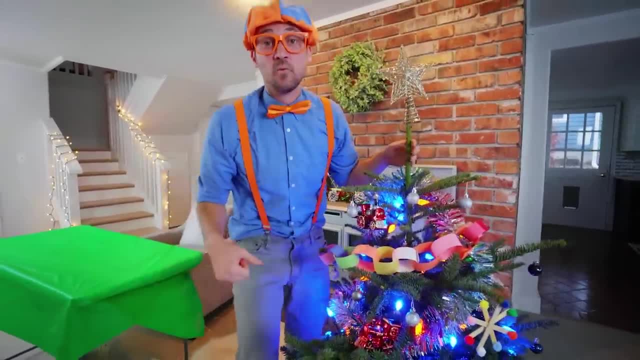 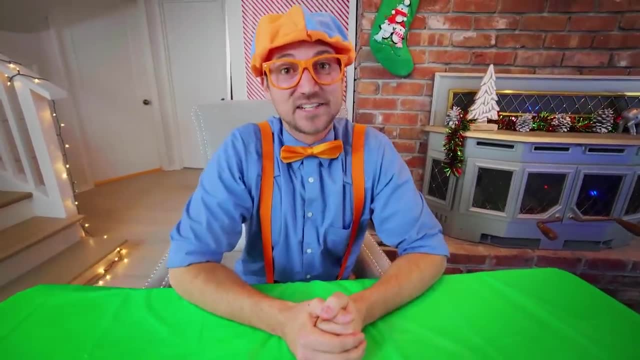 I love it. Yeah, Haha, That was awesome. Well, you did such a great job with all these crafts and decorations that we've done. I just want to wish you happy holidays, merry Christmas and thank you so much for being. 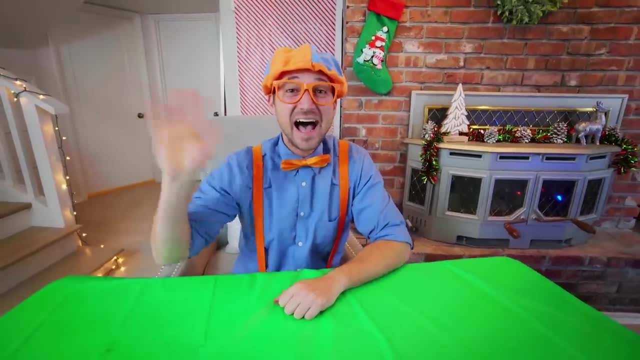 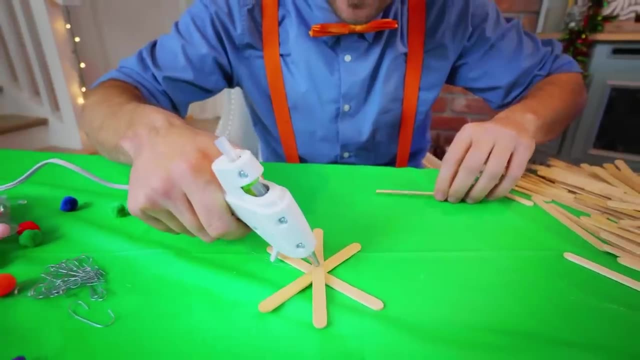 my friend. See you again, Bye-bye. Haha. Well, I had a lot of fun with you, but this is the end of this video. but if you want to watch more of my videos, all you have to do is subscribe. 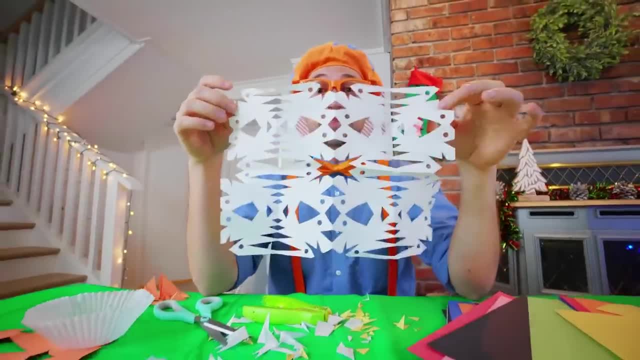 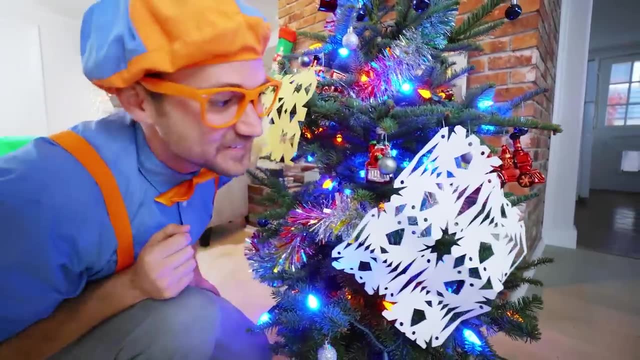 All you have to do is search for my name. Will you spell my name with me? B-L-I-P-P-I, Blippi, Good job, Bye-bye, Haha, Haha, Hello, Hey, It's me Blippi. 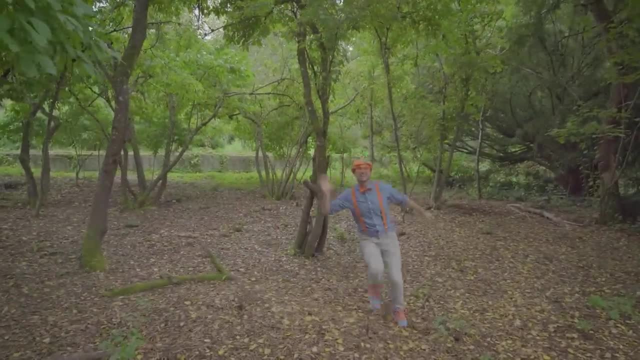 Wow, Look at this place. It's so beautiful. There's so many leaves on the ground And these trees are so big. Hey, Did you see that leaf just fall from the tree? Yeah, It's so beautiful, I love it. 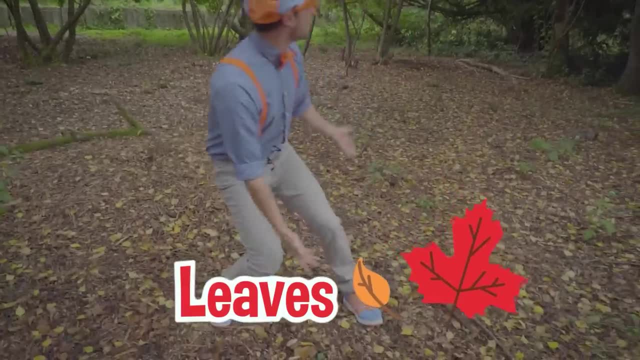 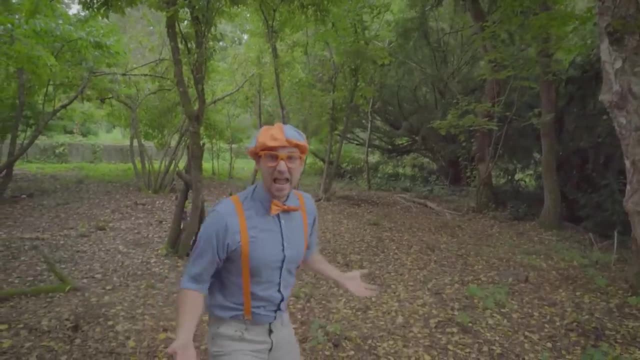 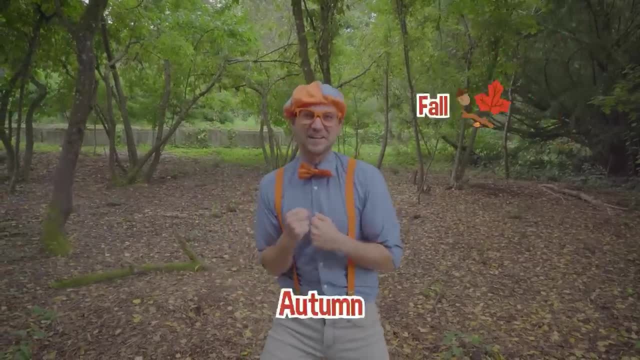 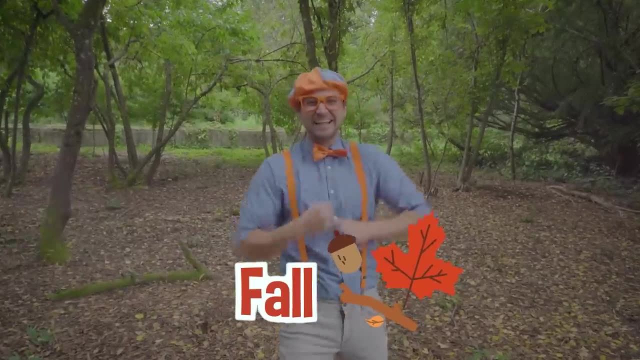 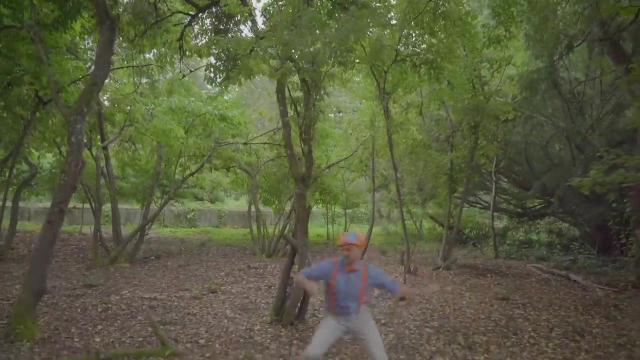 Haha, Also known as autumn, And in this video, you and I are going to learn about the season of fall. Haha, Alright, This is going to be so much fun, Let's go. Hahaha, Whoa, Haha. 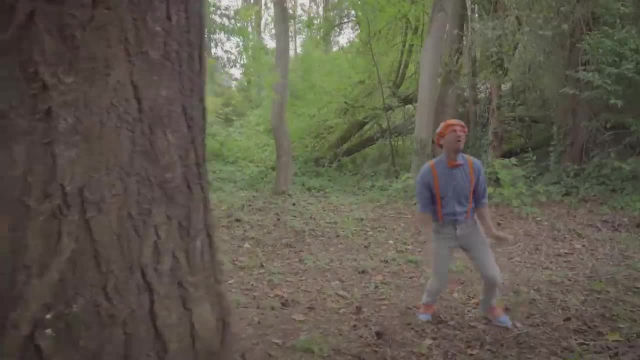 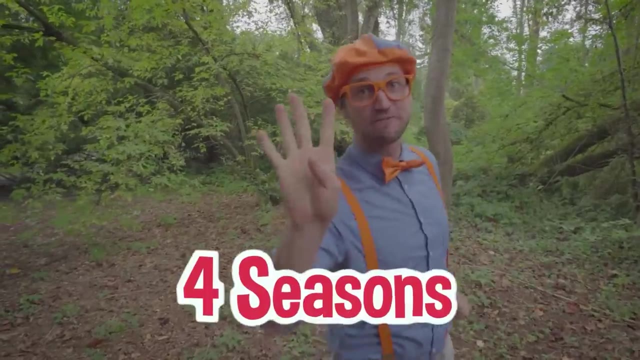 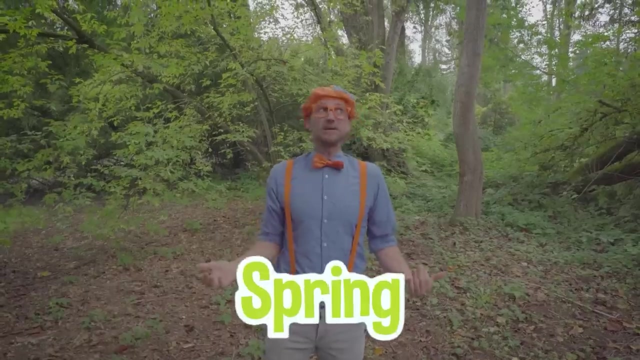 Wow, It's so beautiful I can't hear anything. Oh, Haha, Wow, I sure do love the outdoors. Hey, did you know there's four seasons throughout the year? Let's list them All, right. the first one is spring. 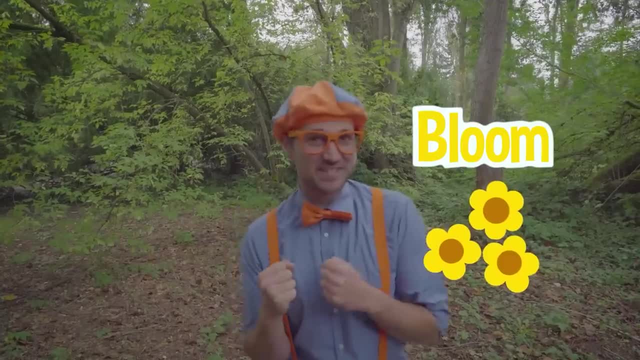 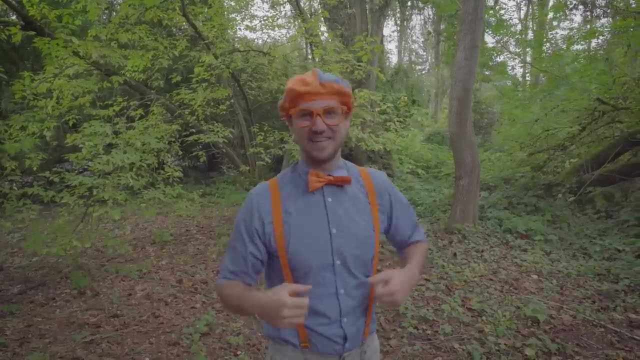 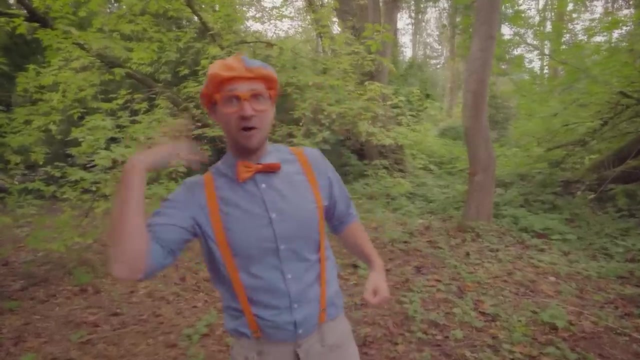 That's when the flowers start to bloom. It starts to warm up a little bit. Sometimes it rains a lot during spring. Yeah, wow, everything's just growing So nice, Sheesh, so hot right now. Yeah, this is summer. 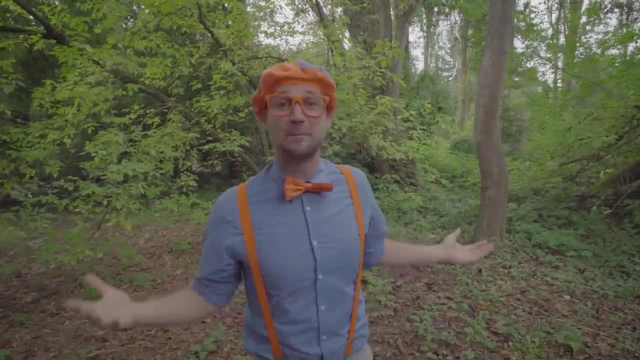 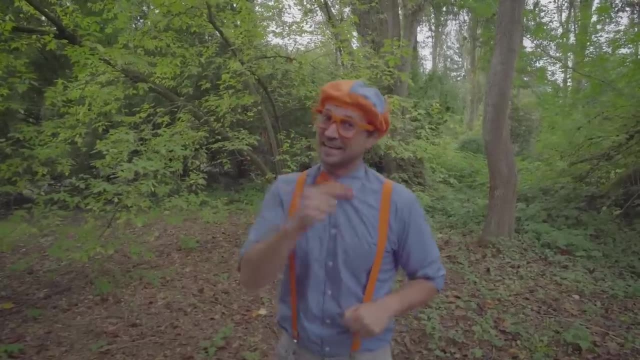 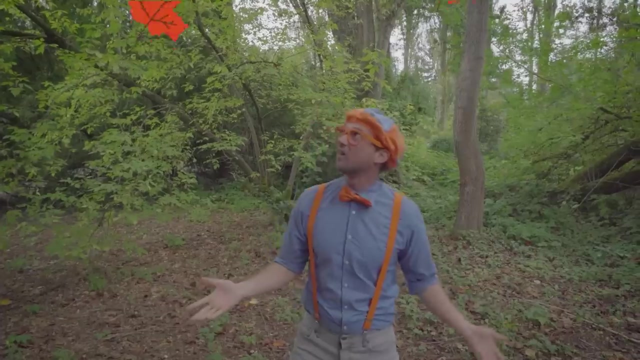 Whoa, I love summer, I love going to the beach, I love laying down on a towel and I love soaking up the rays. Can't forget about drinking lemonade during summer. And then comes fall. Yeah, see all the leaves falling down. 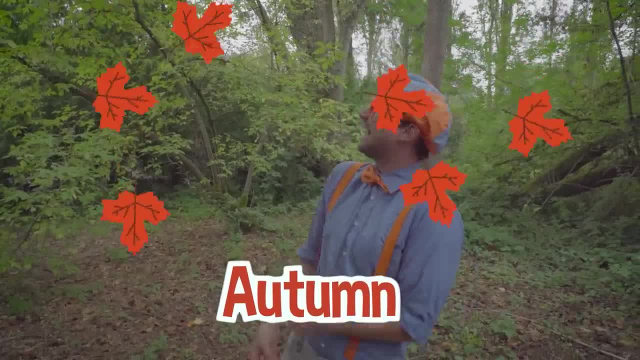 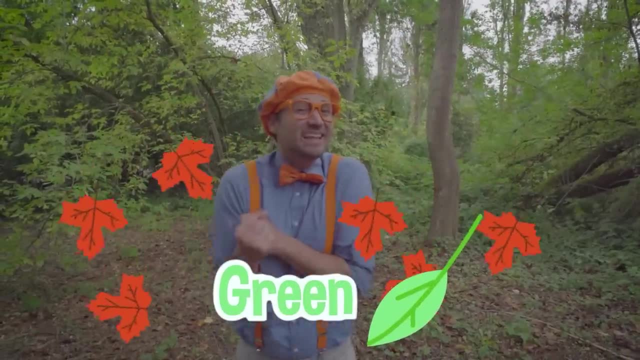 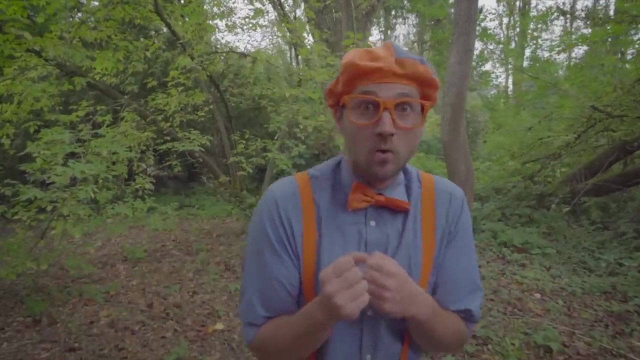 Yeah, another word for fall is autumn. wow, The trees and the leaves. the leaves start to change colors. They might have been green, but then they change into orange and red and yellow. and such beautiful colors, Ooh, brr, oh. what season is this? 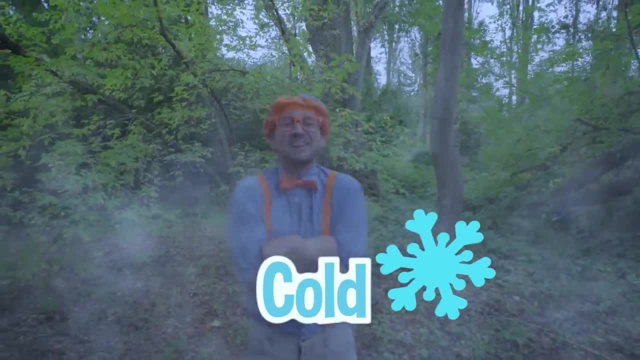 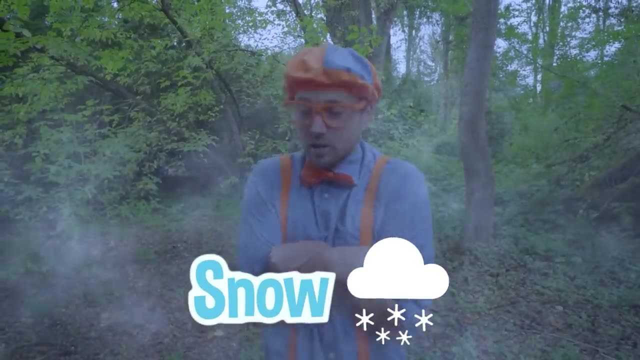 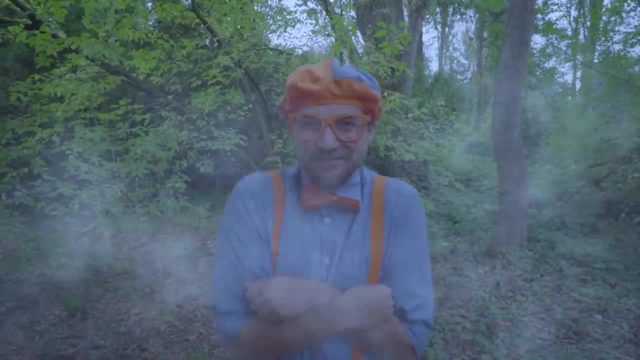 It's so cold. Oh yeah, this is winter. Ooh, This is when it starts to snow in some places around the world. It definitely becomes a lot colder, Brr, and this is when you can do some fun winter sports. 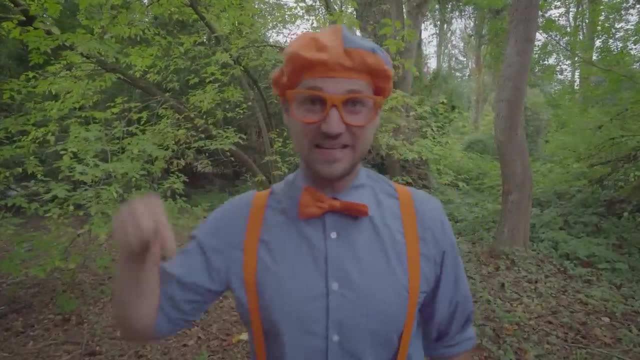 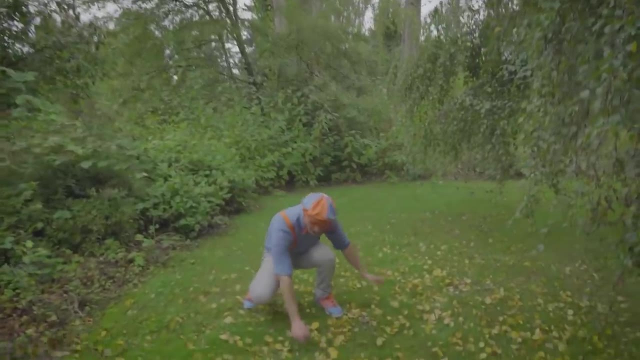 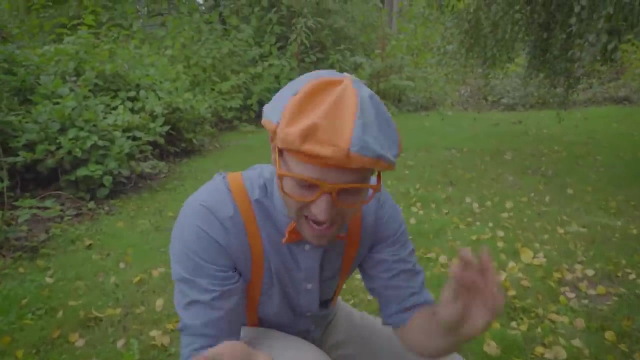 But okay, those were the four seasons, but this season right now is fall, So let's learn about fall. Yeah, Whoa, look at all these leaves on the ground. Do you see them? Whoa, I love fall time. 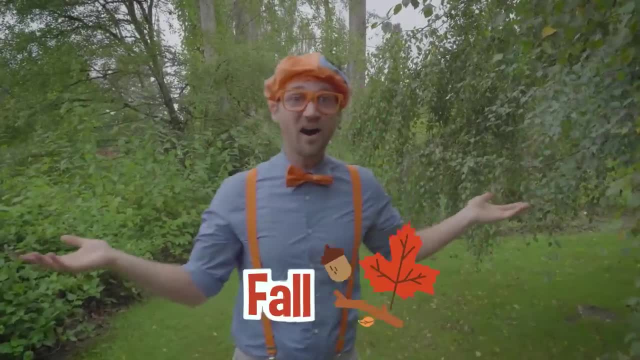 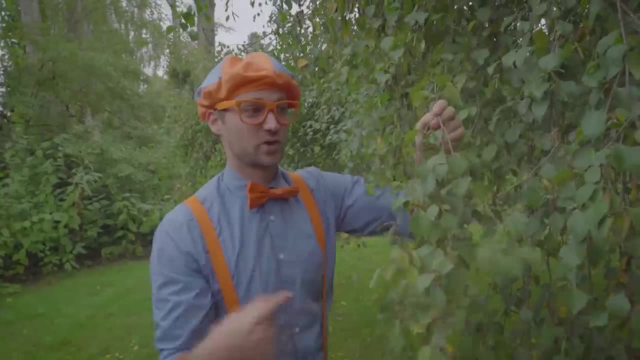 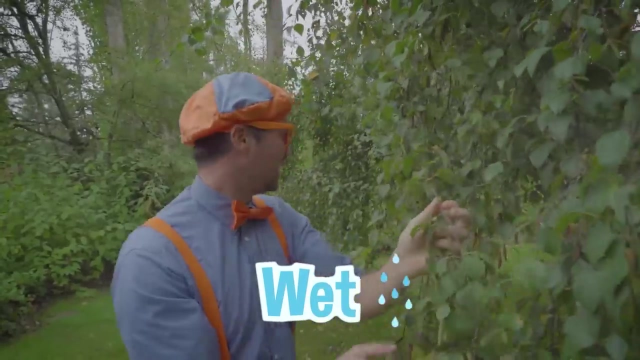 Yeah, these leaves are falling on the ground because it's fall. Hey, check it out. See these leaves. They're the color green. Whoa, they're so nice And nice and wet. yeah, Hey, and then during fall time, whoa. 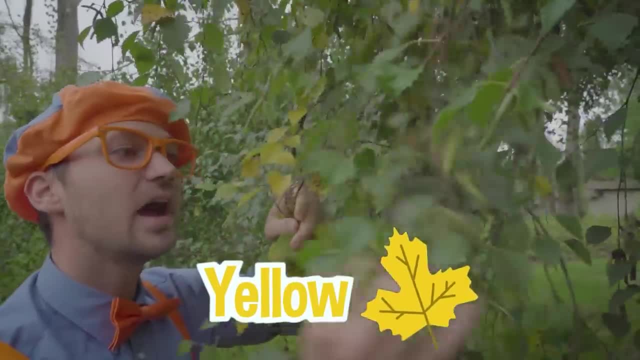 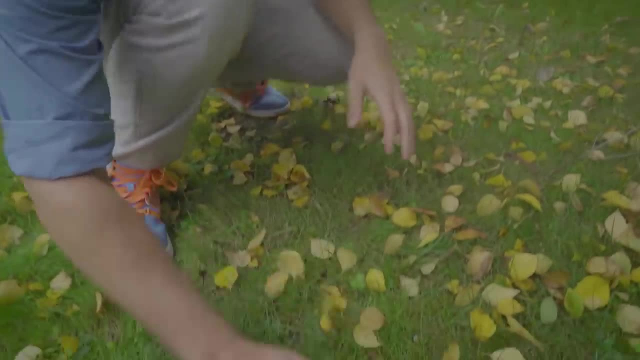 Do you see how these same leaves are turning yellow? Yeah, and they're actually kind of dry, Kind of dry. They're drying up and then they fall down to the ground. Whoa, Look at all these leaves. Oh, I'm gonna collect some. 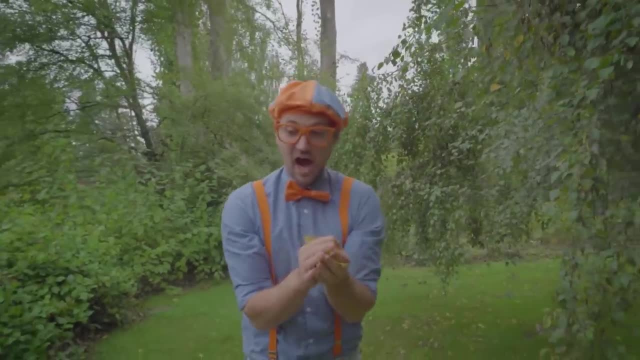 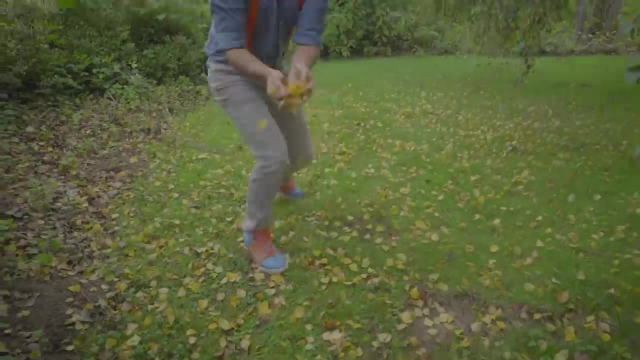 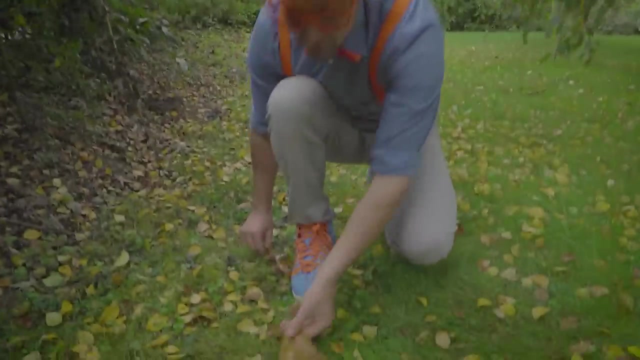 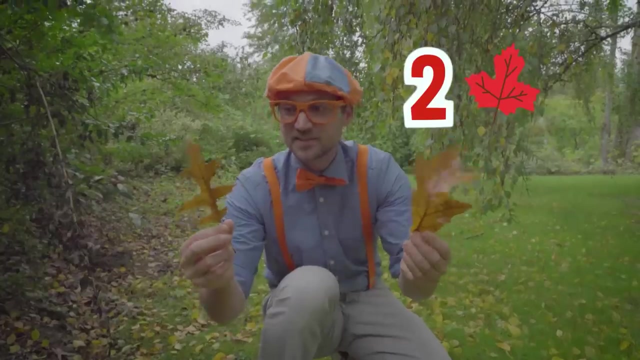 And I'm gonna use them for an art project. later I'll show you the art project. It's gonna be so cool. Whoa, there's so many Whoa. Look at these two leaves. Wow, one, two, Two leaves. Hey, what color are these leaves? 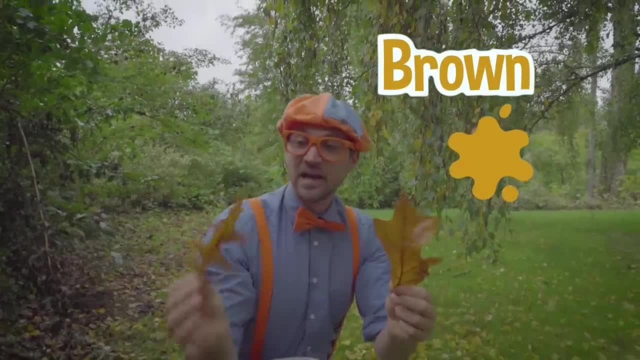 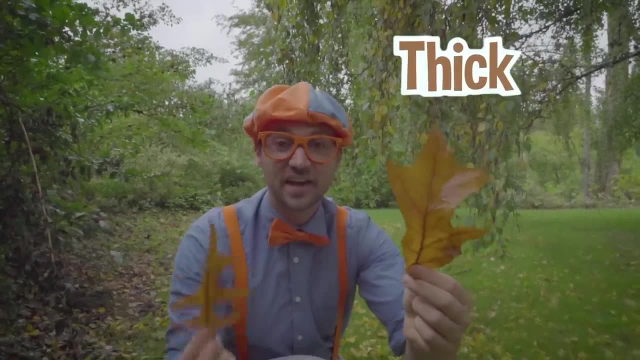 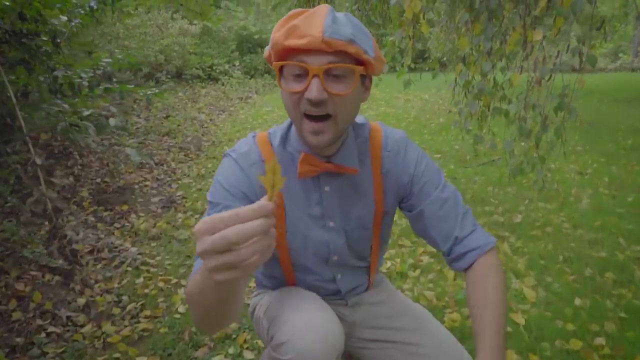 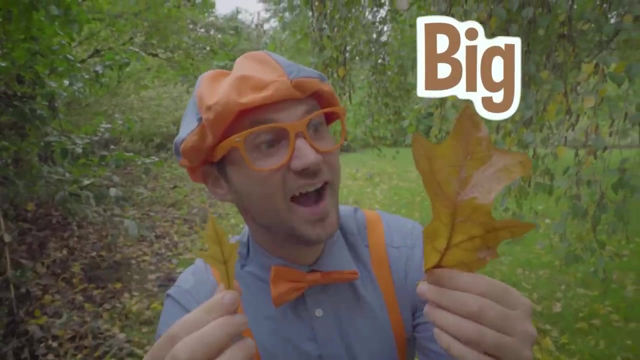 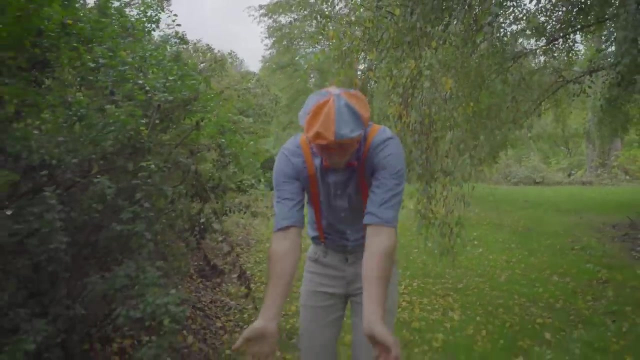 Yeah, they're both the color brown and this leaf is really thin. This leaf is really thick. Wow, This leaf is really small and This leaf is really big. Okay, I'll collect these leaves and use them for our art project later. Wait a second, Here's some more leaves. Whoa. 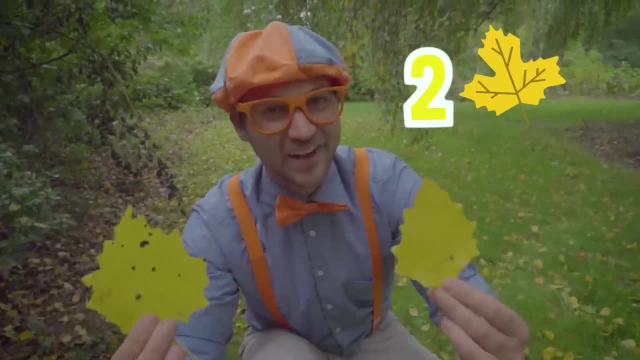 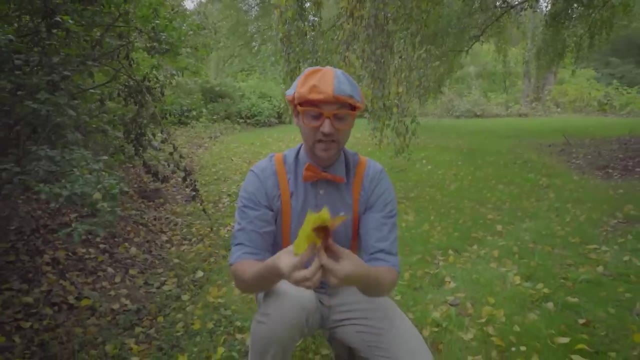 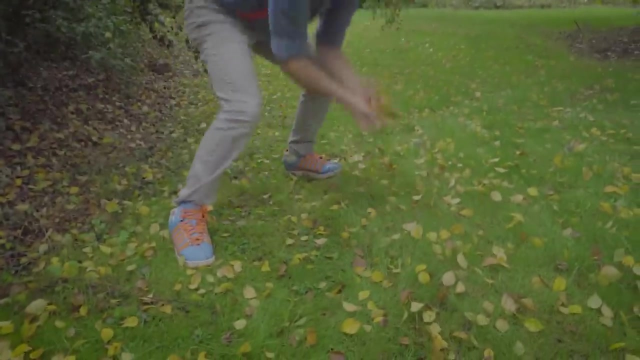 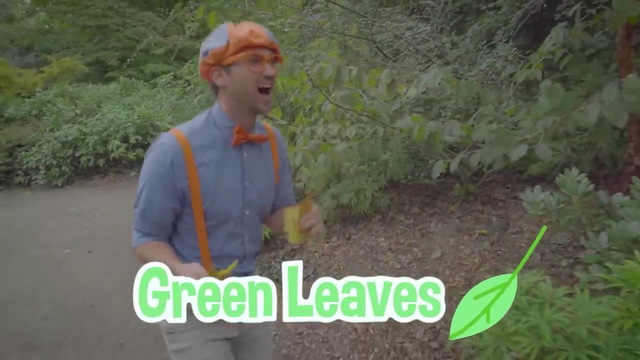 Two more leaves, one two. and what color are they? Yeah, the color yellow. Oh, We have so many great leaves for our art project. Okay, let's continue to collect these leaves. Wow, look at all of these green leaves. green is such a cool color. 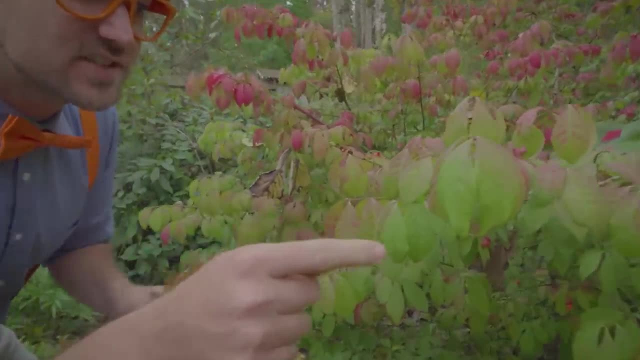 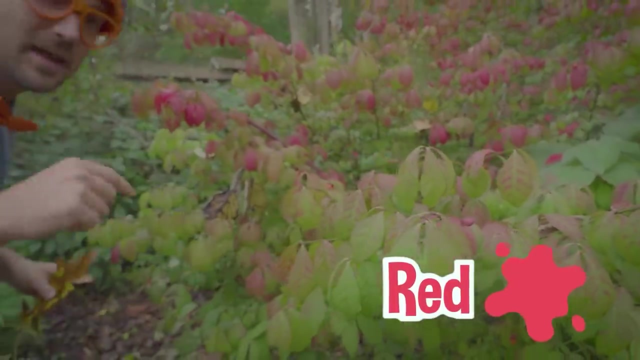 This is so cool. Check it out. Do you see these leaves? They're the color green and then they're slowly Changing to the color red. Hey, maybe we can look on the ground and see if we can find some red leaves That fell off. 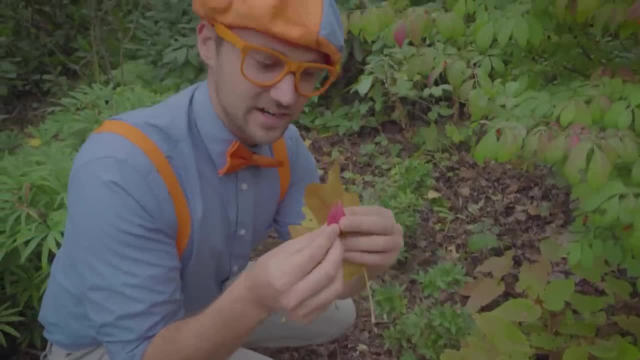 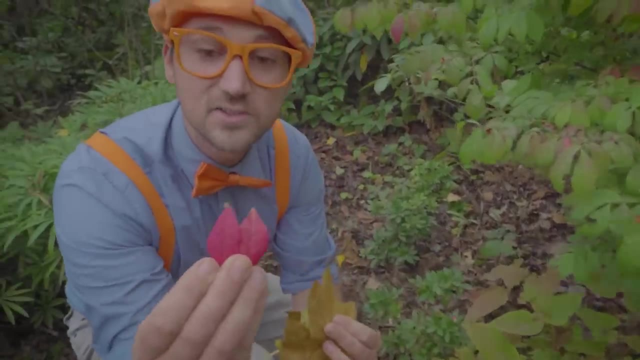 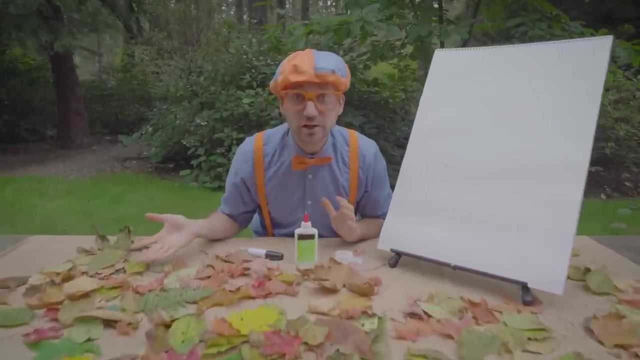 Hey, Here's two right here. Here's one. Where'd the other one go Here? it is All right. Here's two red leaves. Good job, Look at all these leaves. Yeah, you and I did a really good job collecting all of these leaves. 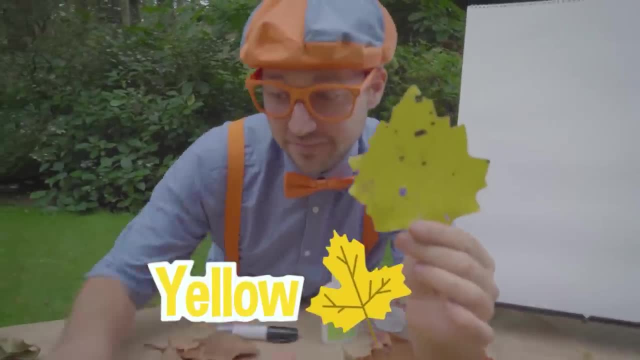 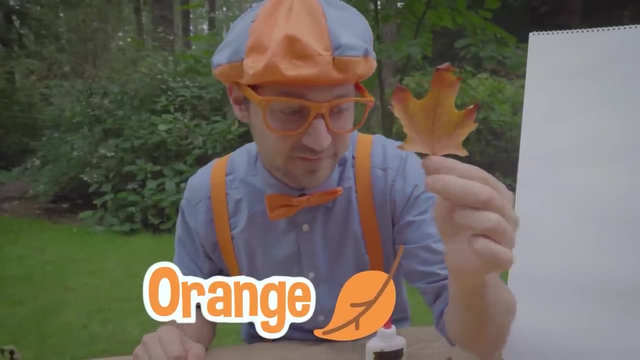 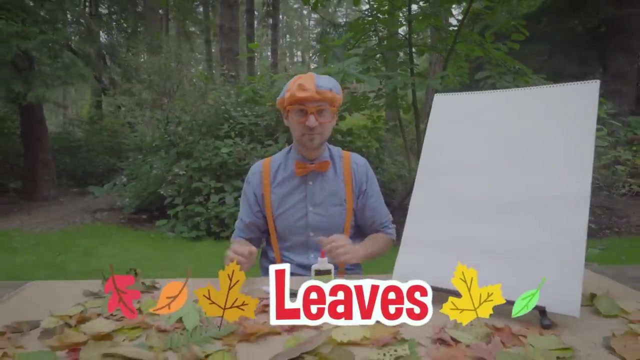 Hey, check it out. We have a yellow leaf, we have A green leaf, we have an orange leaf and We have a brown leaf. There's so many leaves to use. Yeah, Remember what I said earlier: We were collecting the leaves for an art project and here we are. 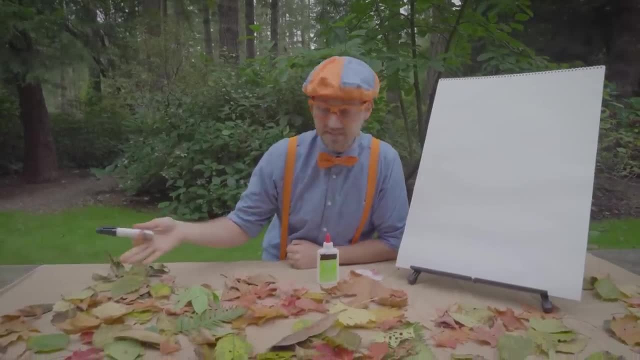 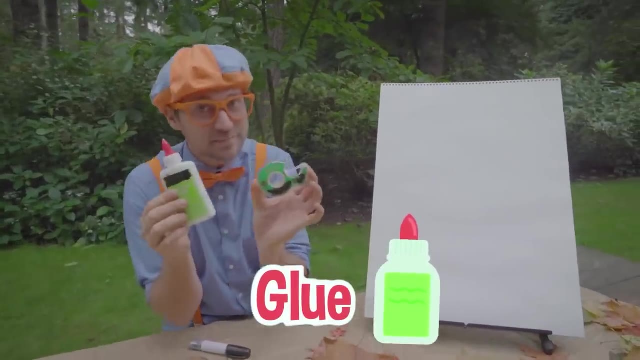 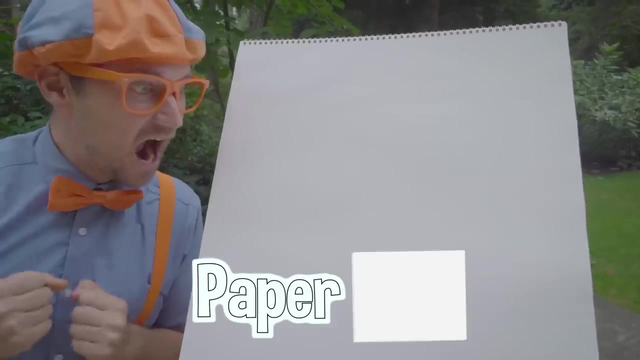 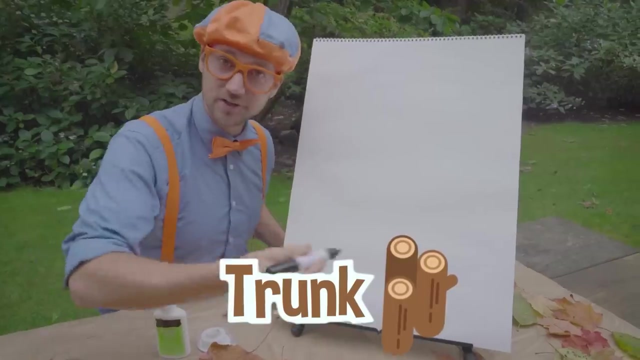 so the art project consists of the leaves, a black marker, Some glue and Oh or some tape and a big white piece of paper. Whoa, Okay, first thing we have to do is take our black marker and draw the trunk of the tree. 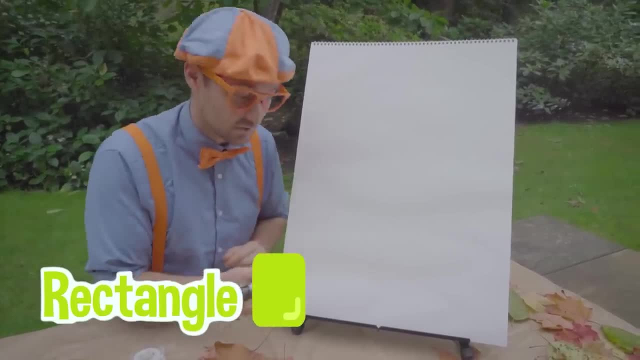 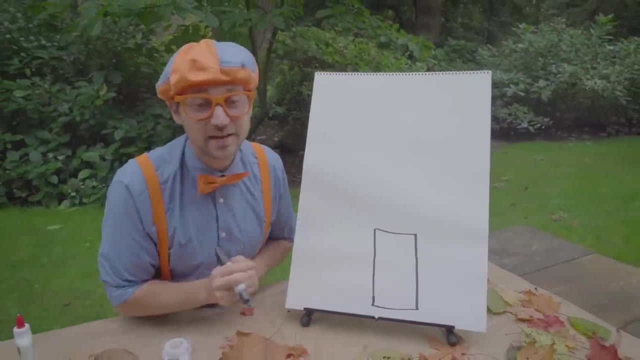 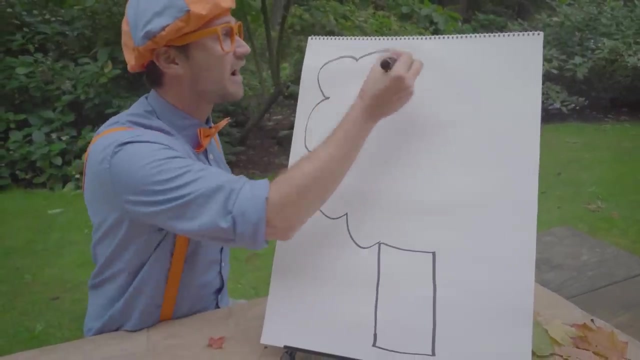 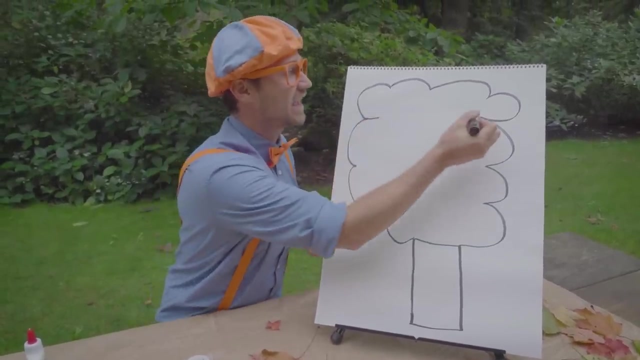 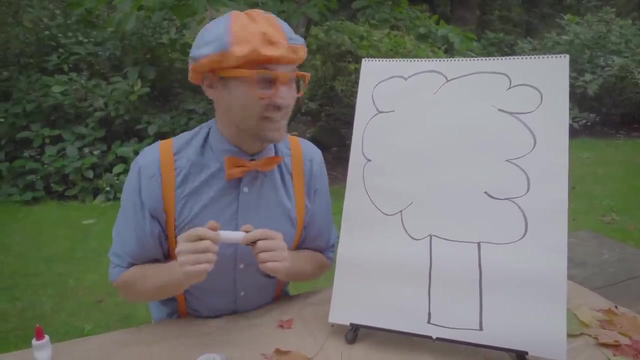 which is gonna be a tall rectangle. Ready- Perfect, that shape is a rectangle. Now we need to make all the leaves. Here we go. Yeah, that looks like a great tree. Yeah, there we go. Perfect, That's a nice fluffy tree. 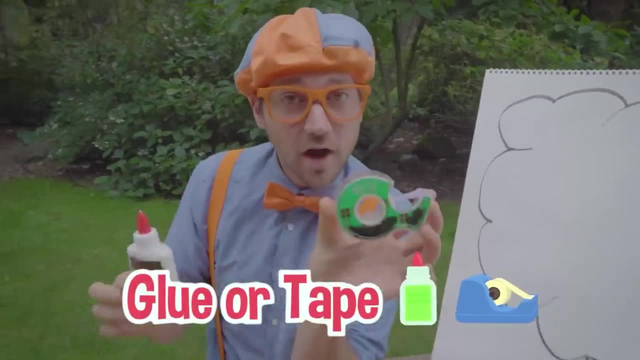 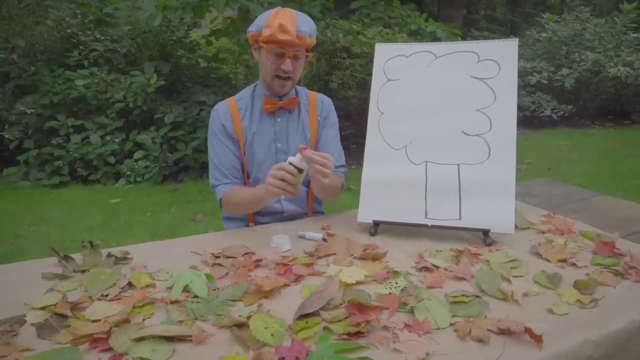 Okay, now the next thing: we're gonna take either our glue or our tape and then put it on the tree with, obviously, the leaves. All right, I'm gonna try the glue first. Let's see. Ooh, this leaf looks great. 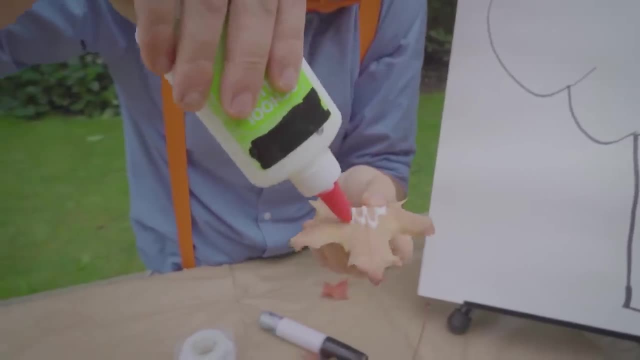 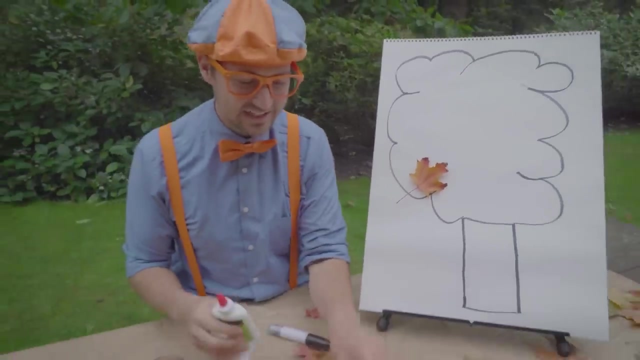 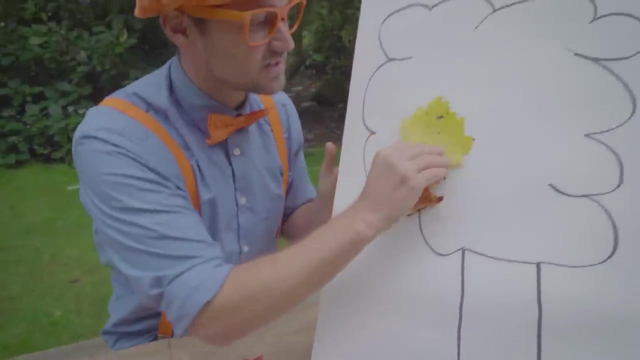 Yeah, all right. Nice amount of glue on the back. Stick it right there. That looks amazing. How about a yellow leaf? Put some more glue. Wow, this is gonna look so great. Whoa, Look at this green leaf. 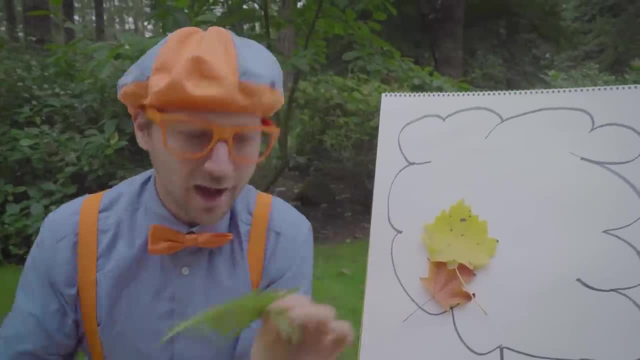 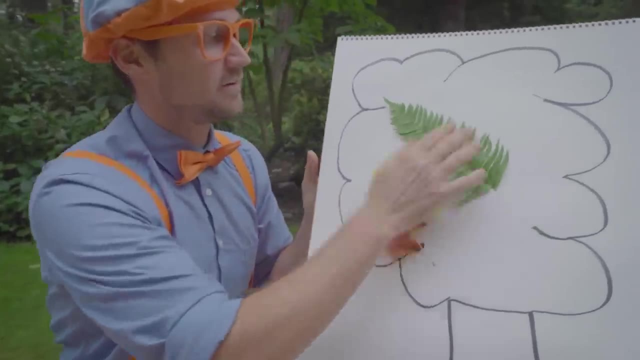 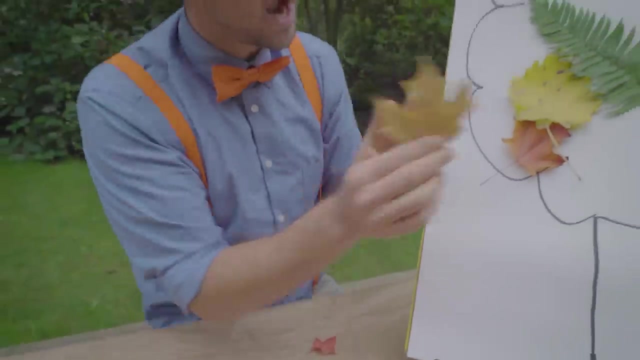 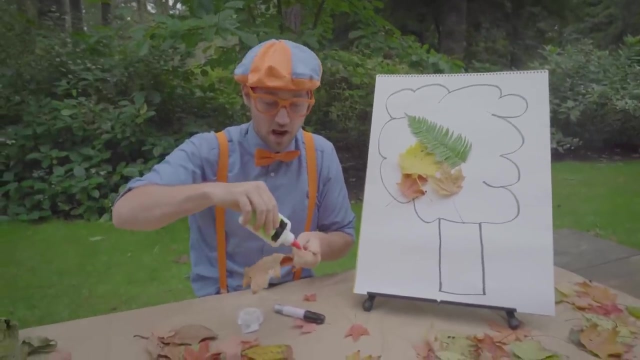 Wow, It's like a miniature tree. All right, Nice long bead of glue right there, Perfect, Ooh, This is so much fun. I wonder how many leaves we're gonna glue on this piece of paper in all. I don't even know. 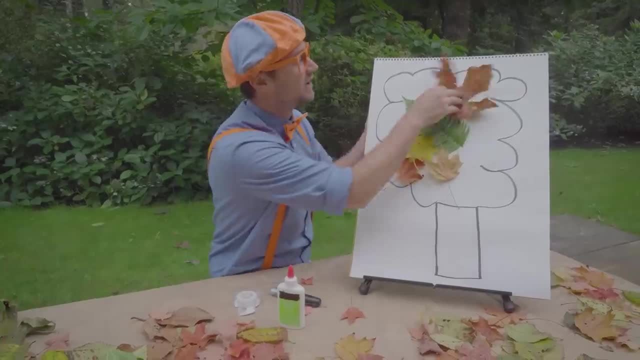 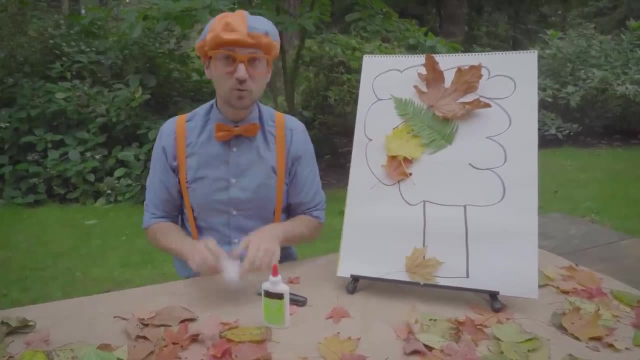 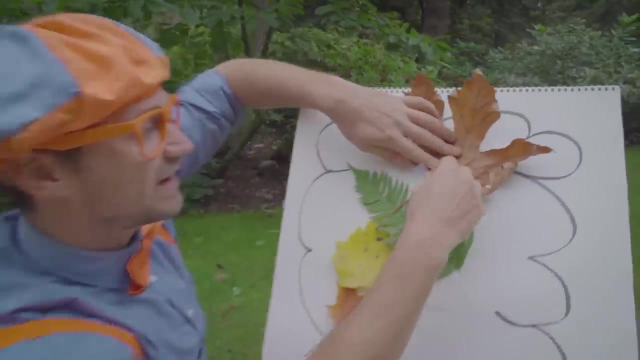 I'm just gonna keep gluing these leaves, One after the other. Whoa, Whoa. I don't know if that leaf is sticking up there. Hey, why don't we try the tape? Maybe the tape will work better. All right. 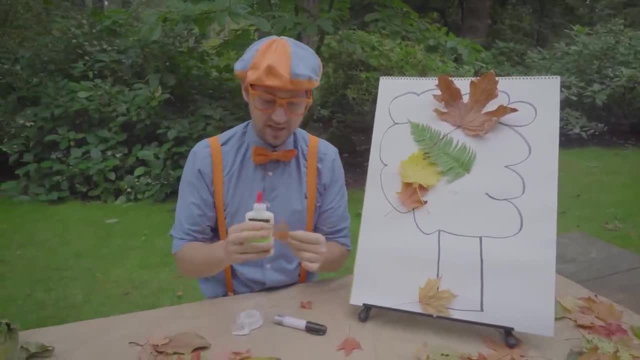 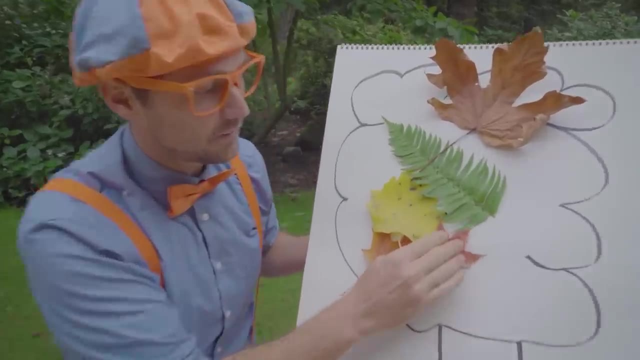 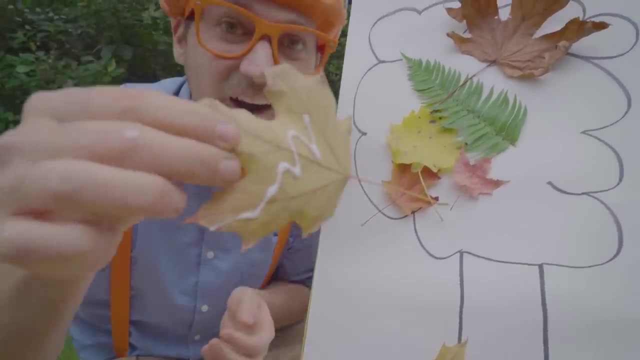 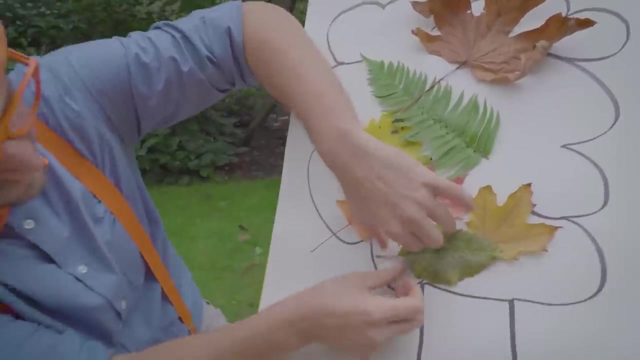 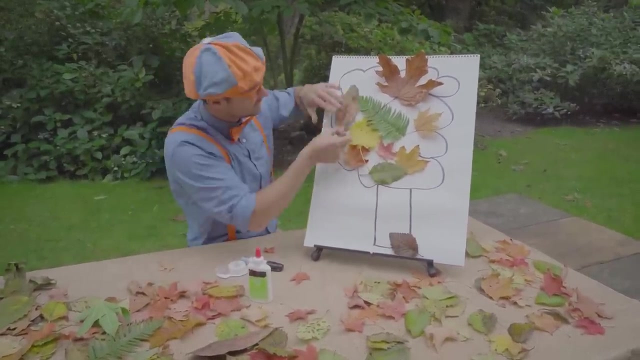 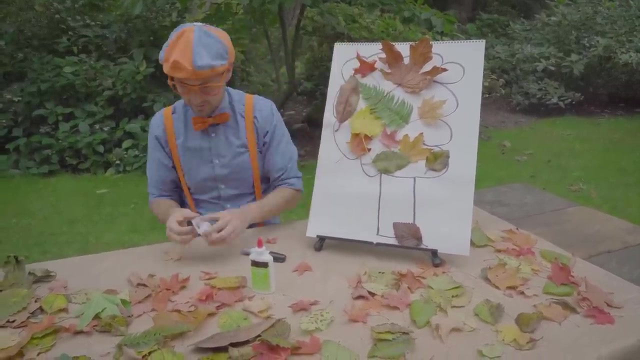 Yeah, that worked great. All right, sometimes in life, if something doesn't work, you can try something else and maybe the next thing will work. Wow, perfect, This is looking so good. Another one: Whoa, Let's go guys. 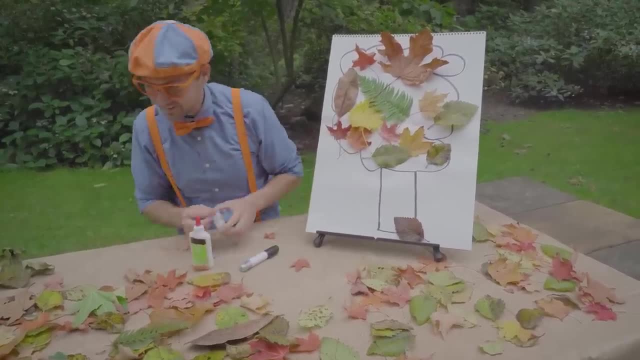 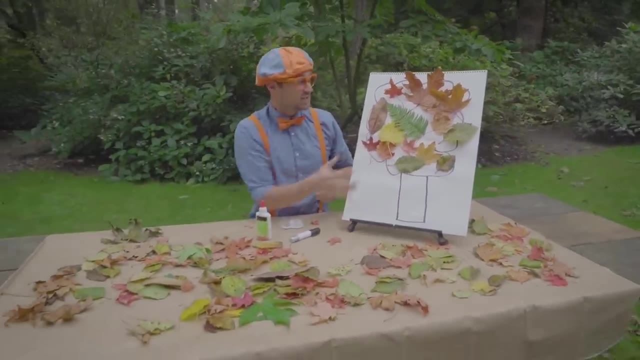 Ooh, One, two, three, four, five. Let's go. One, two, three, four five. One two, three, four, five. Whoa Good job. You and I just made a tree on paper. 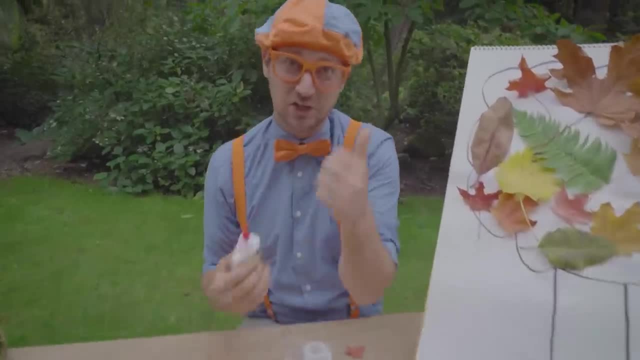 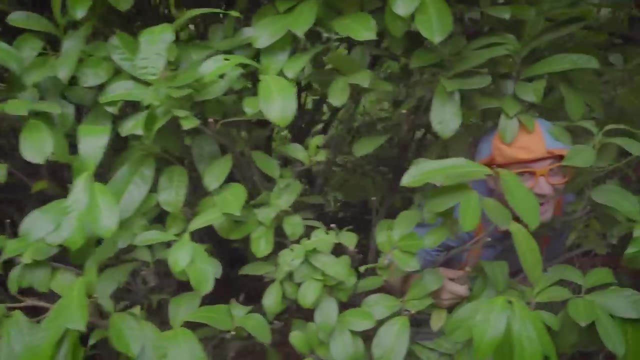 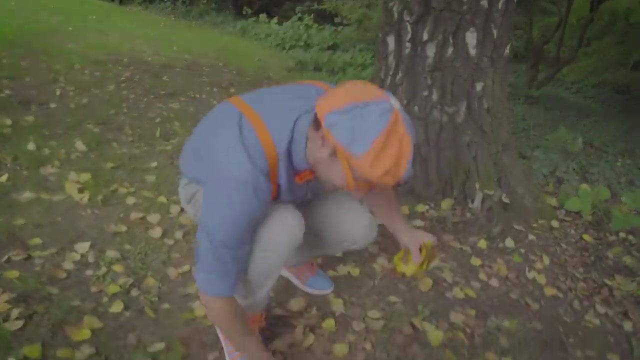 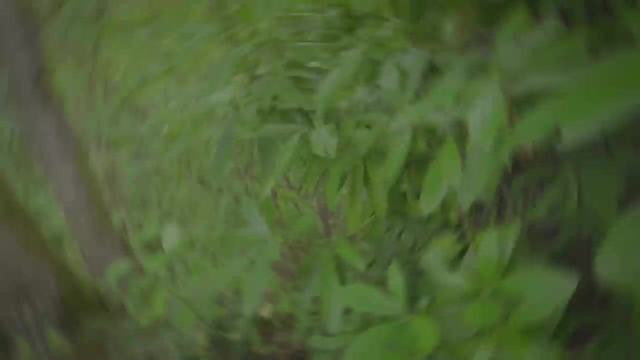 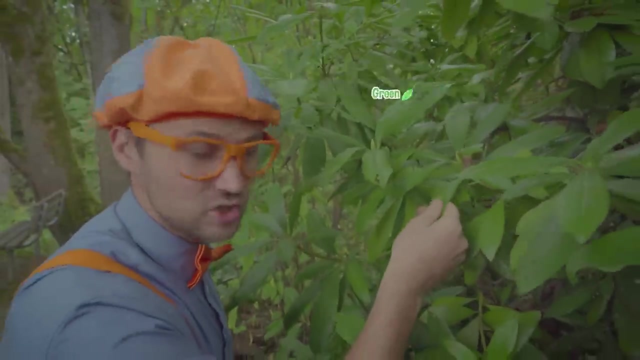 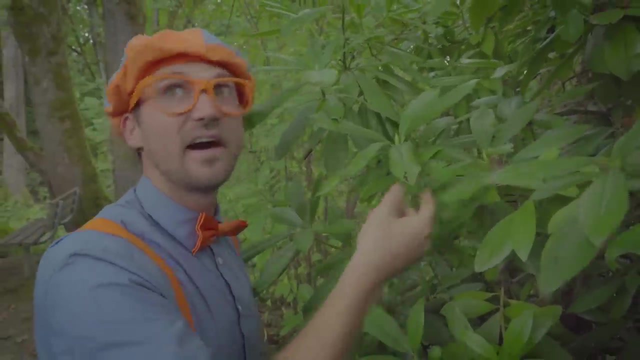 from all the leaves we collected earlier. Good job, That was so much fun being crafty with you. Whoa, Check out these leaves. They're so green, Hey. and when I touch them gently, yeah, nothing happens. They're just so soft and moist, Wow. But this leaf over here, Whoa, This leaf looks. 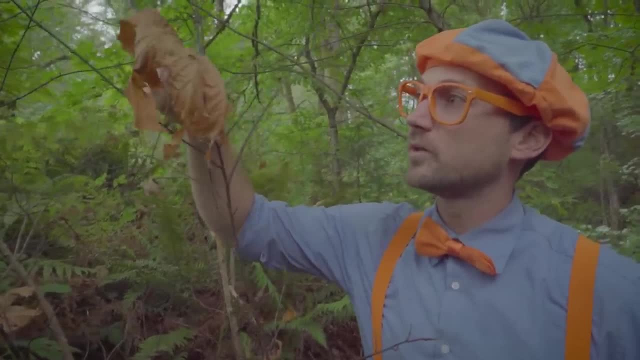 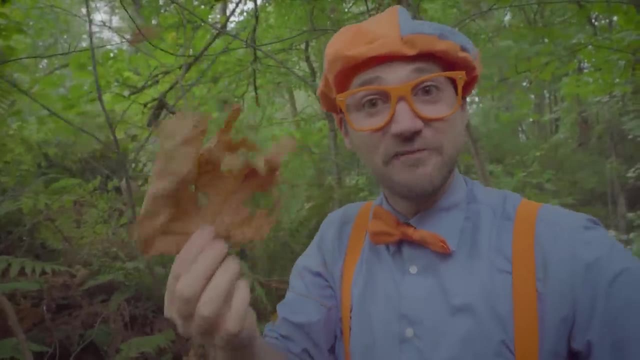 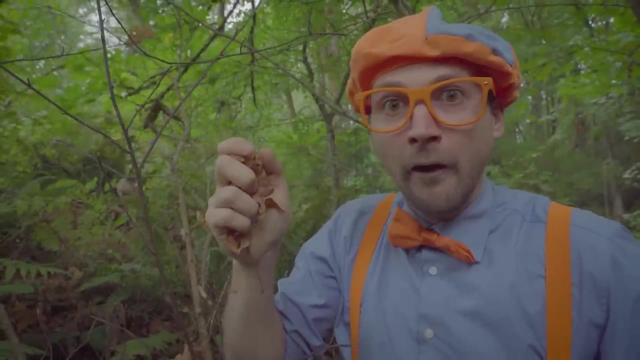 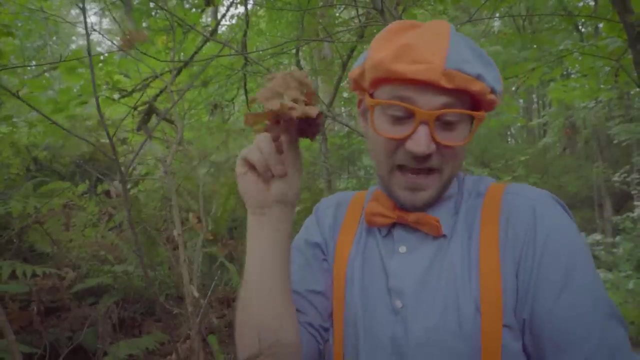 like it fell from the tree above. Let me pull it out. Yeah, You see this leaf? Yep, It definitely fell, because it's fall and it turned brown. I wonder what happens when I touch it. Yeah, Did you hear that It crunched because it's so dry? Okay, We'll keep this one for later. 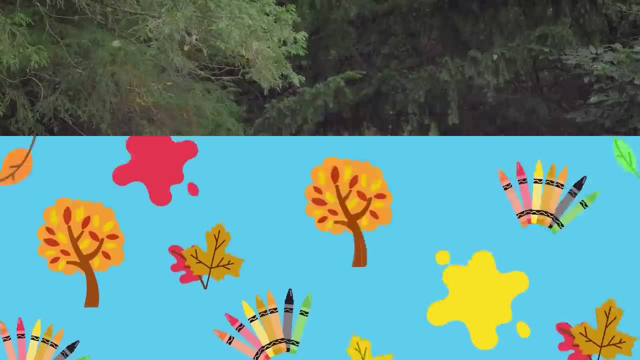 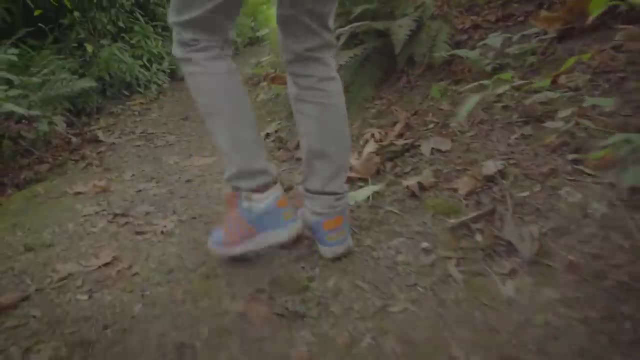 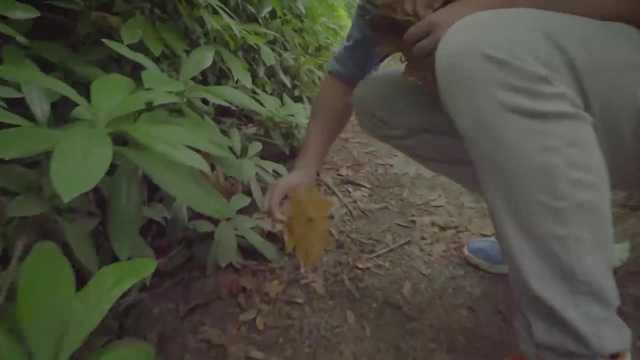 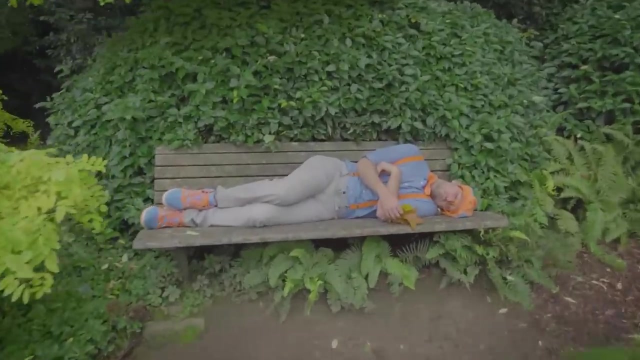 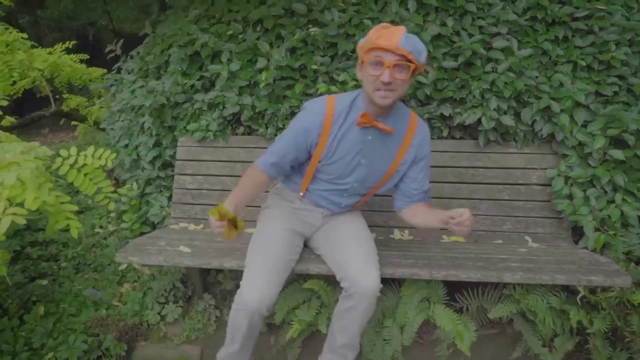 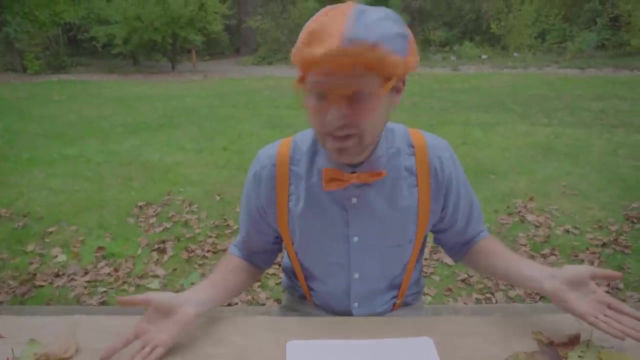 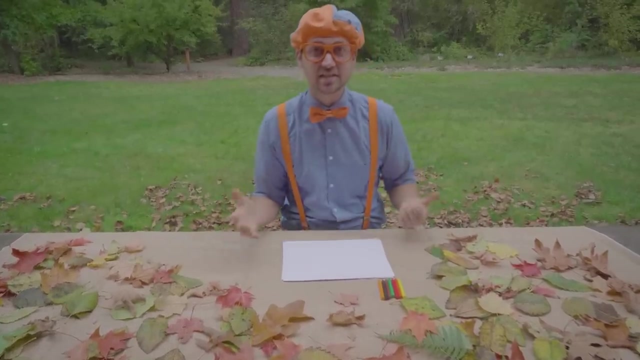 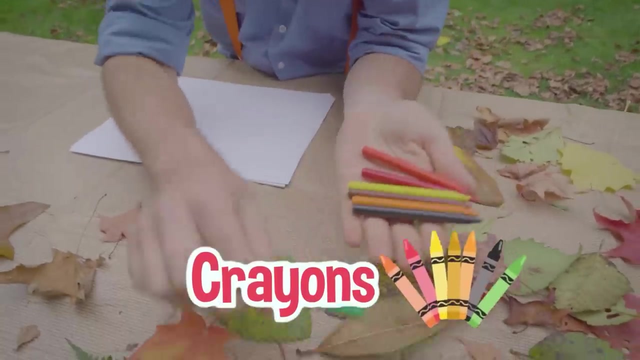 Leave no leaf behind, No time for sleeping. It's time for a cruise, It's time for a craft. Yeah, Look at this, Another art piece. I am so excited. I love leaves and I love the season of fall. All right, So for this art piece, we need some crayons- Whoa, I dropped one, Ooh. 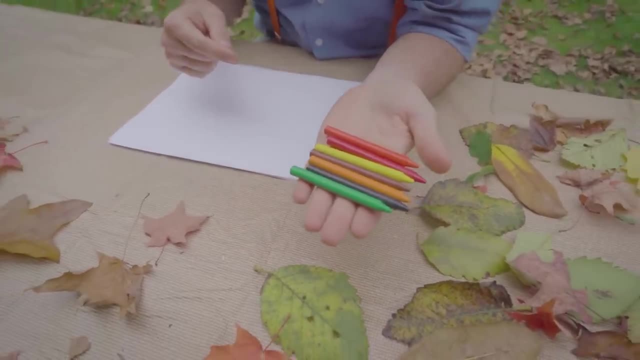 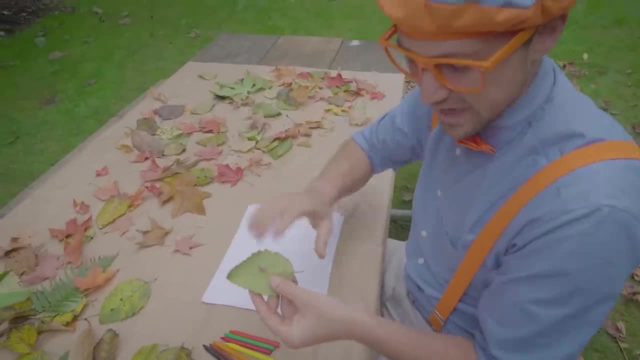 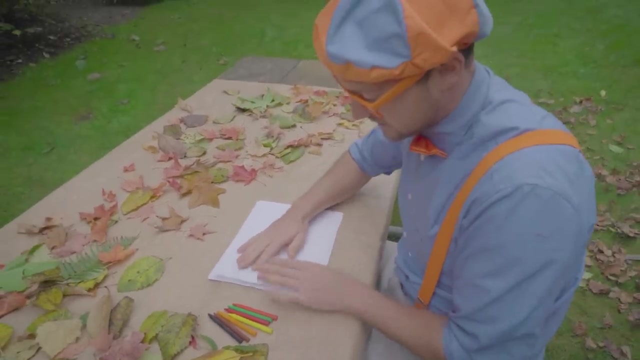 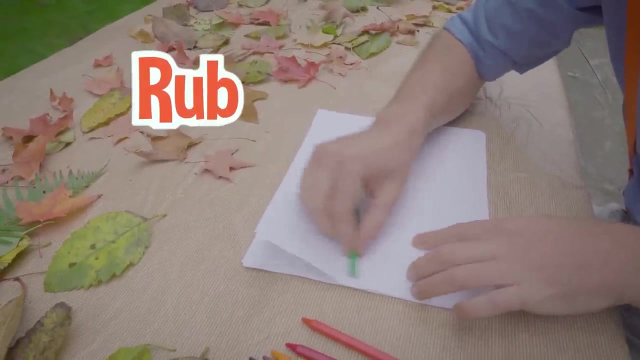 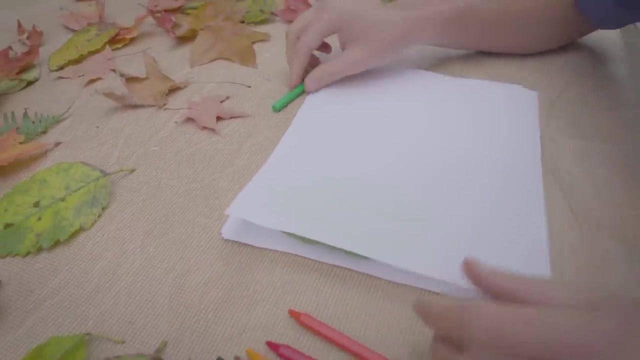 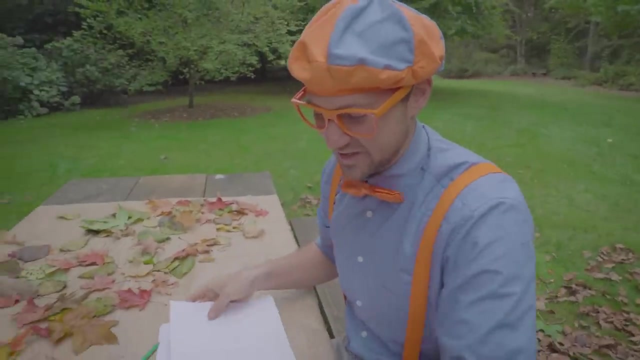 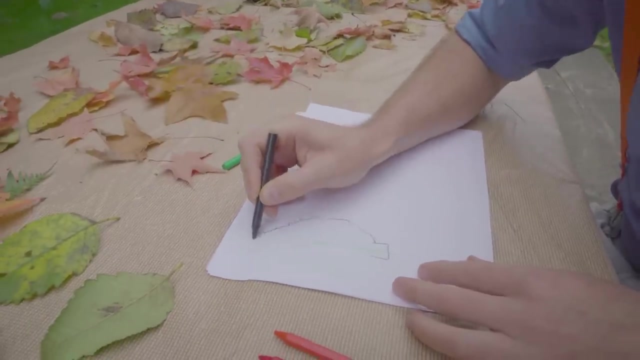 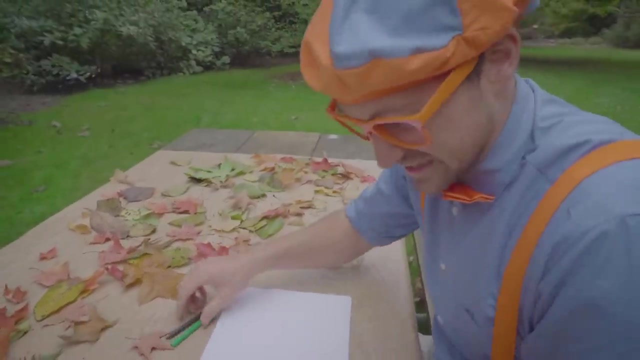 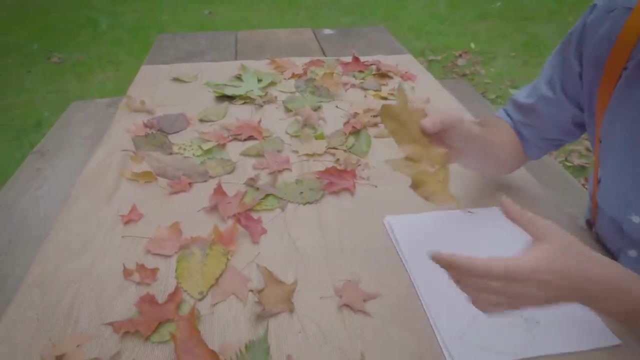 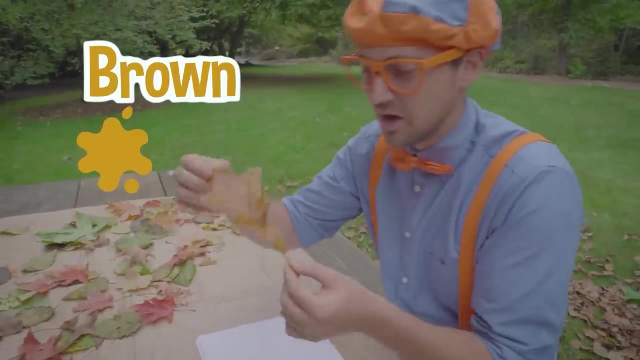 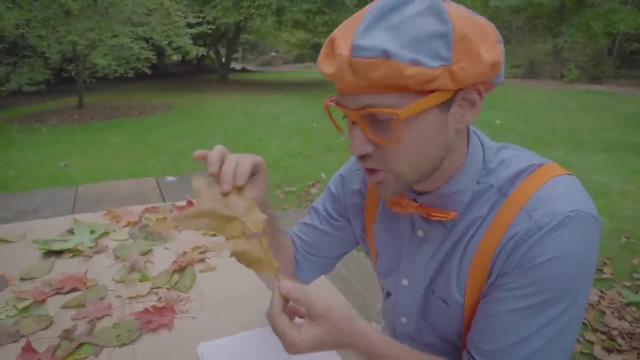 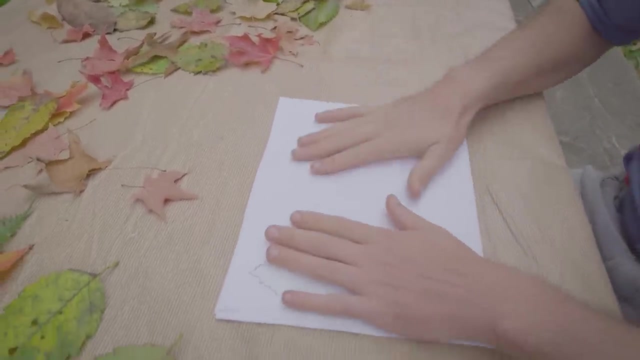 Okay, it has a hole in it, That's okay. It's gonna be really tricky, but I think we got this. Okay, I'm gonna put it to the side, like that. Yeah, at an angle, There we go. All right, then let's do the color brown. 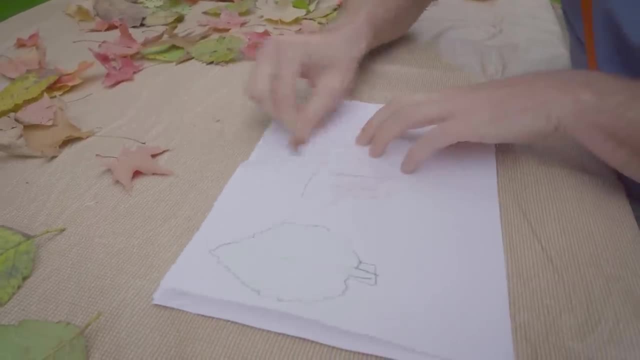 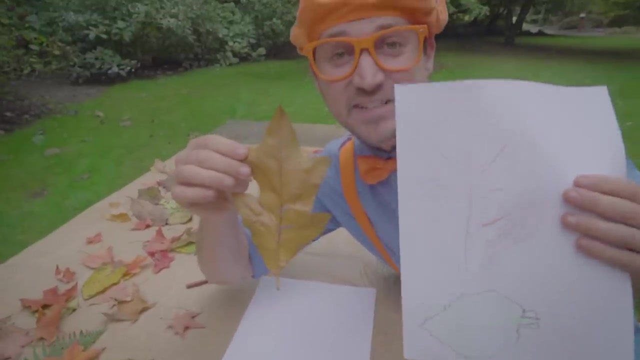 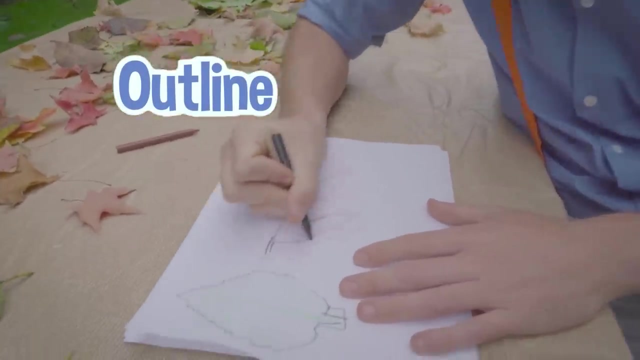 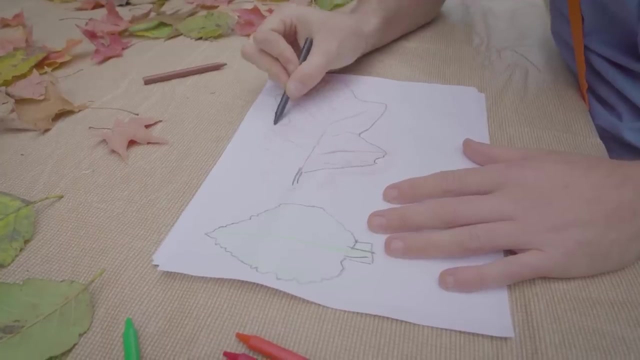 Ready Whoa. look, Do you see what we did? Isn't that cool? Okay, I'm gonna outline this one. Yeah, I love outlining them. Yeah, you don't have to, but I'm just going to because it makes it a little bit more apparent. 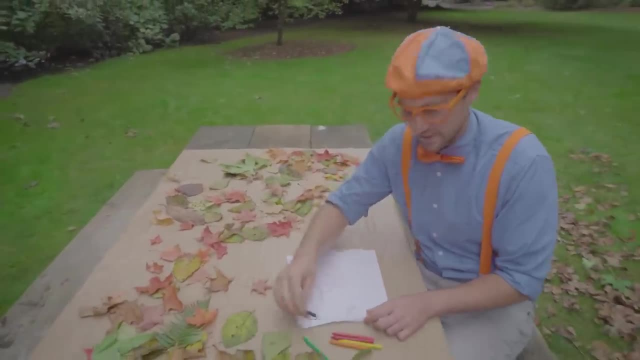 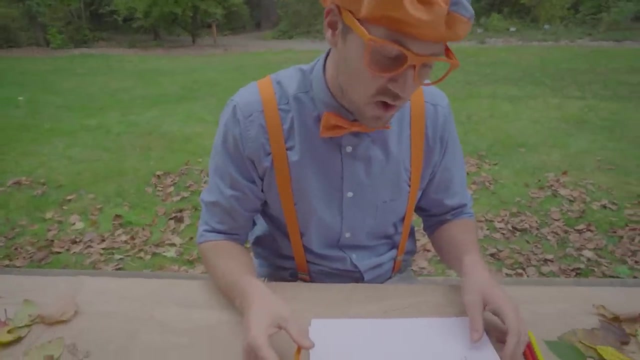 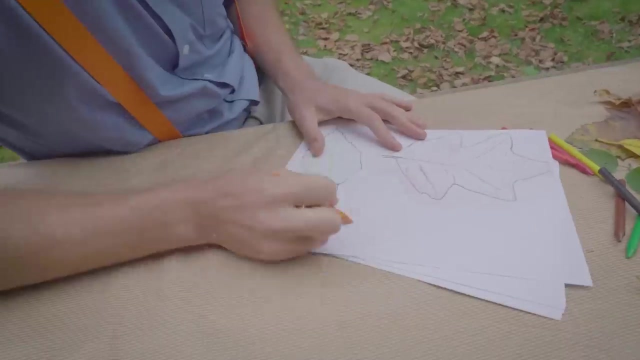 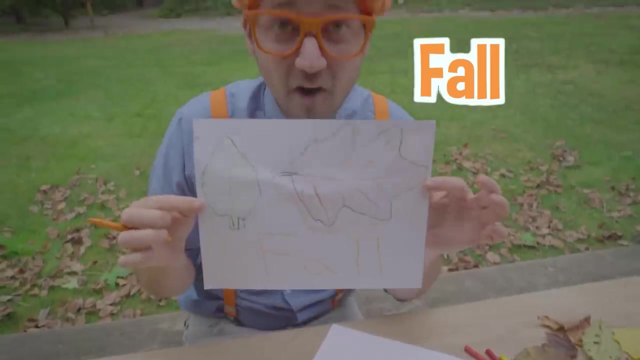 Yeah, hey, I have an idea. Why don't we take a third color, like the color orange, yeah, and write a word on the bottom? How about the word fall? Okay, ready, Spell it with me. F-A-L-L. fall. 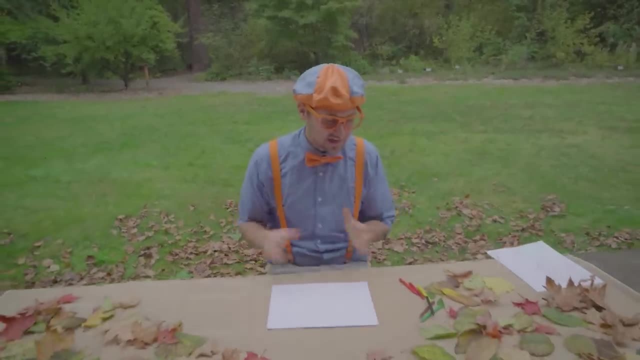 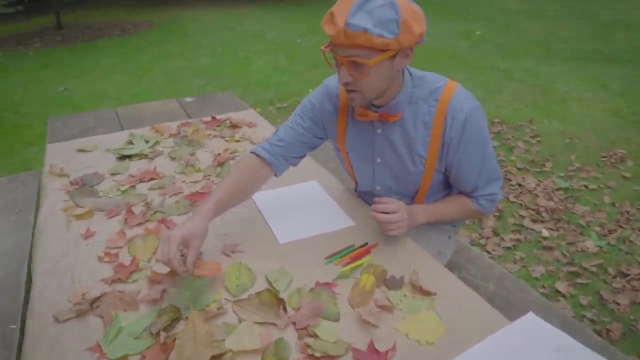 Good job. Okay, let's put that right over there, and then let's do another leaf. Hmm, let's see So many leaves to choose from. Hey, look at this one. This one is a unique one. Yeah, this is from a fern. 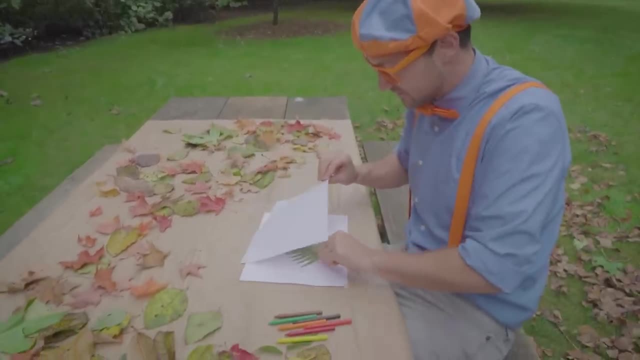 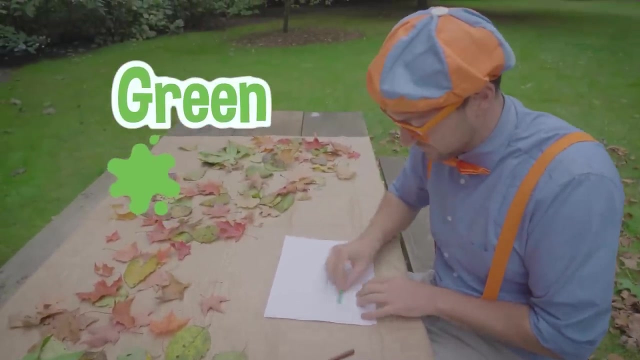 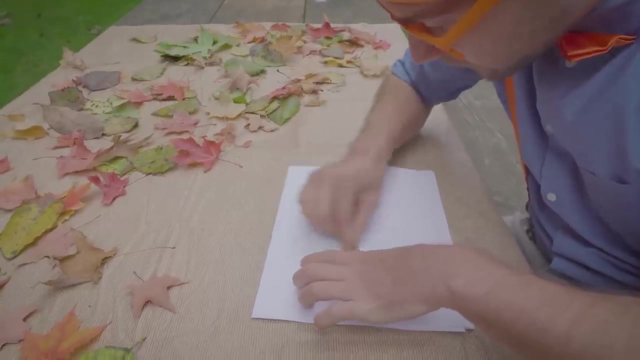 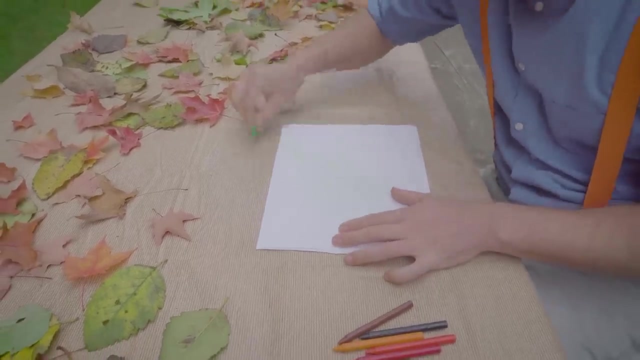 All right, I'm gonna put that right here. Then let's use the color green again, because the leaf was green, but you could actually use any color you want. Whoa, this is looking really, really cool. Wow, do you see that? 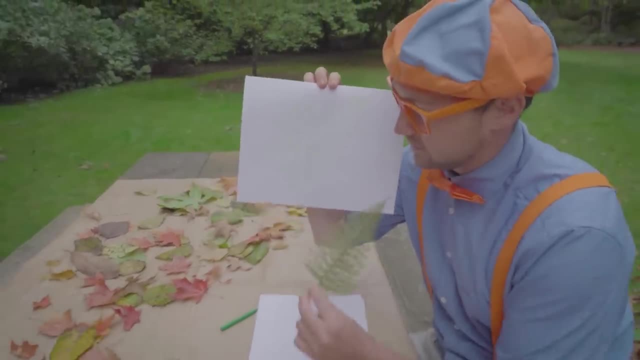 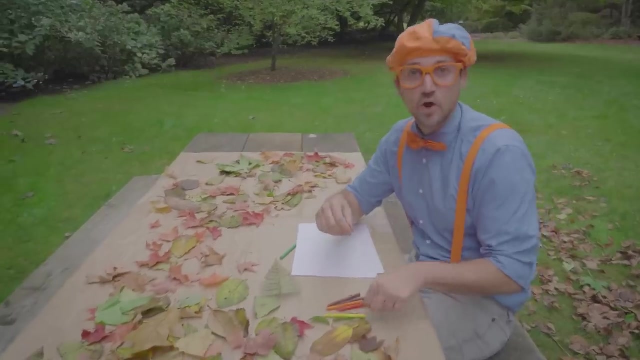 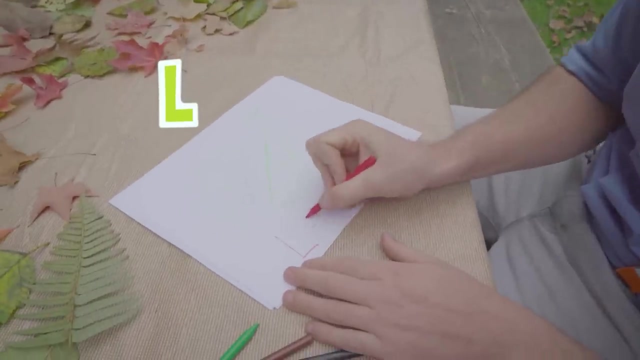 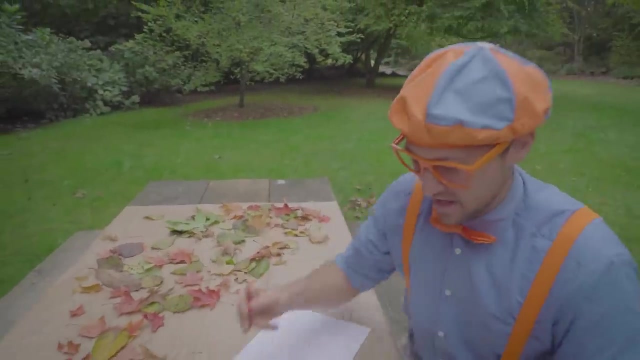 It's hard to see, but it's really cool. Yeah, Look, looks the same. huh, All right. Now let's take the color red and write the word leaf Ready L-E-A-F leaf- All right. 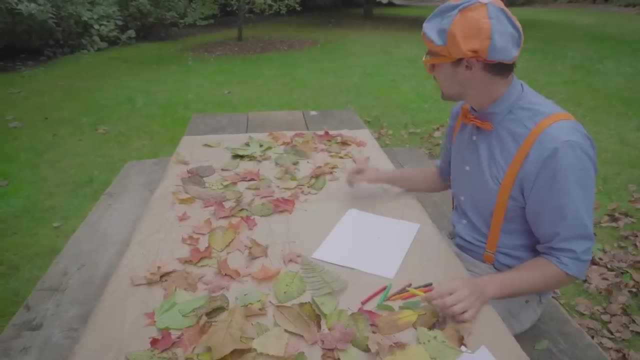 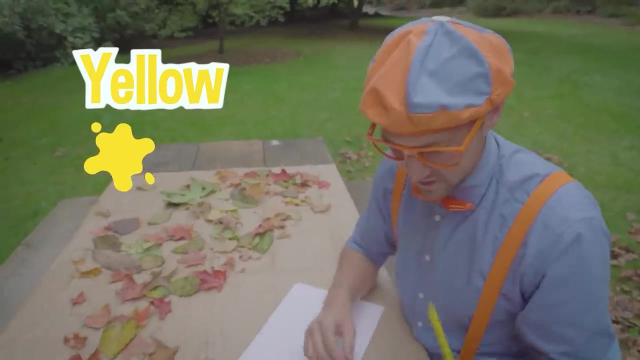 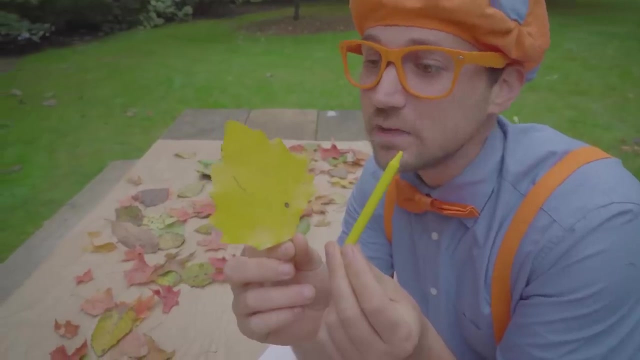 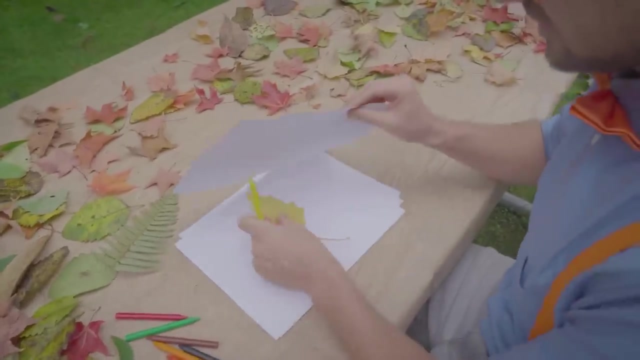 Let's do one last leaf. Um, hey, I know We haven't used the color yellow yet. Yeah, let's use the color yellow. Let's find a yellow leaf. Whoa, look at this. Yeah, that's a bright yellow leaf. Okay, All right. Okay, Put this leaf right in the middle. 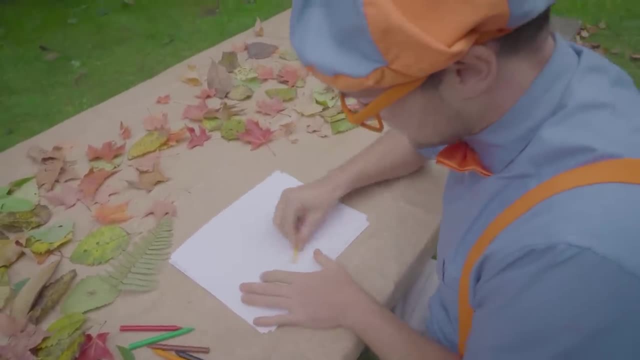 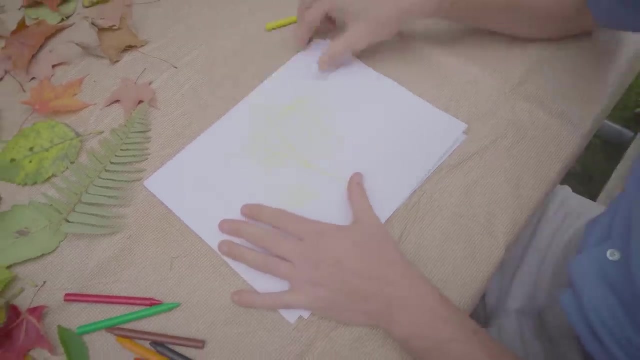 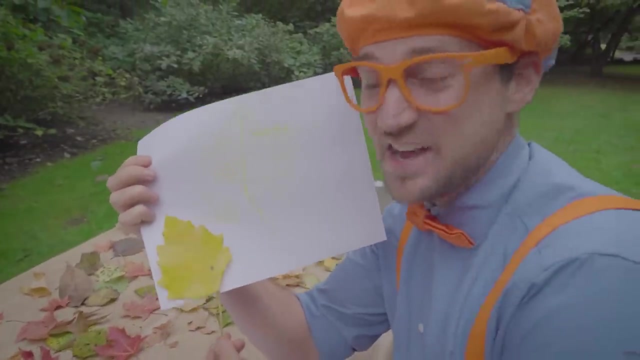 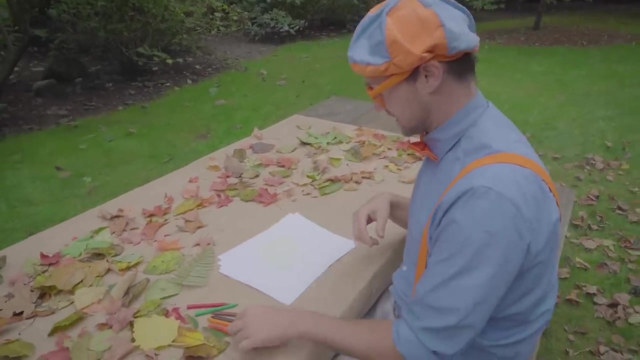 There we go And here we go. Wow, Look at that, Whoa, Another great leaf. Okay, Let's spell one last word. Let's use the color. Let's use the color black, since we didn't outline this, Let's. 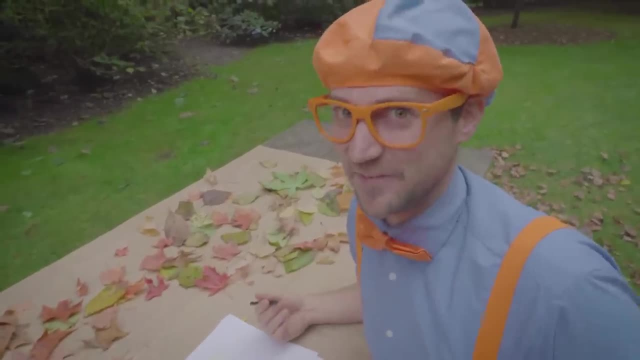 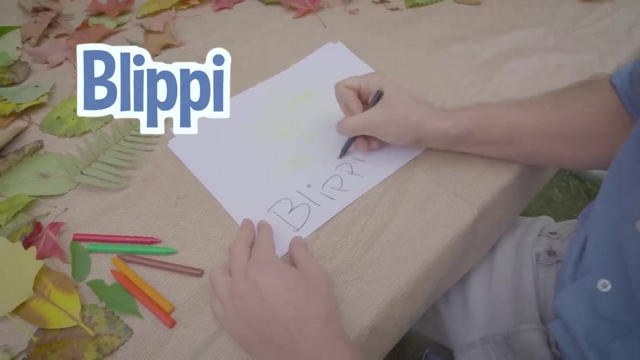 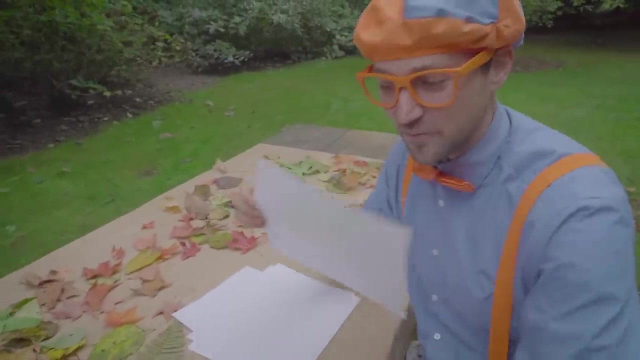 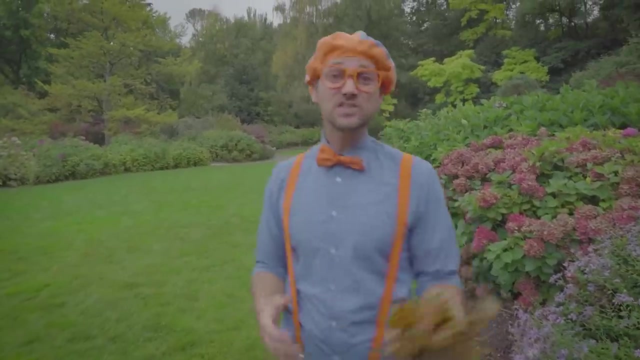 spell. I know Let's spell my name Ready B-L-I-P-P-I Blippi. Good job. This is so much fun doing all this fun art with you. Wow, Wow, That was so much fun learning about the season of fall with you. 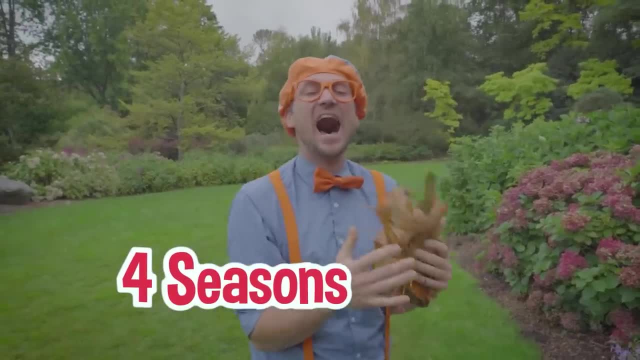 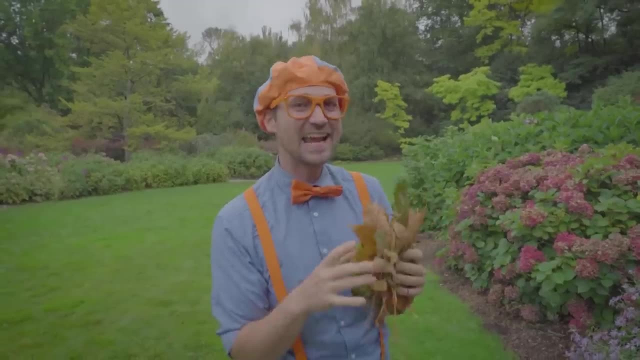 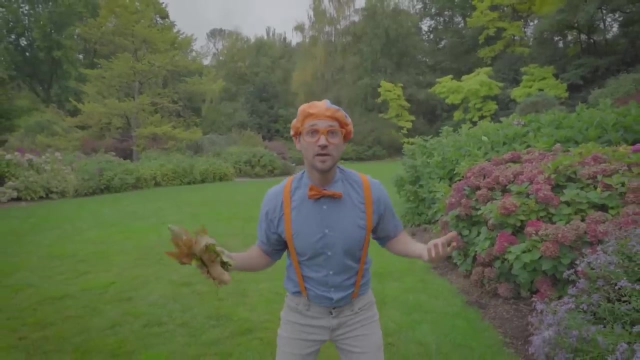 It's one of my favorite things to do. Four favorite seasons. We learned some counting, some colors, some size comparisons, textures, and we were really crafty. Well, this is the end of this video, But if you want to watch more of, 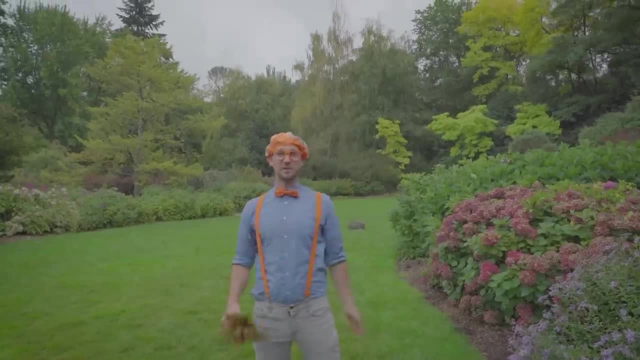 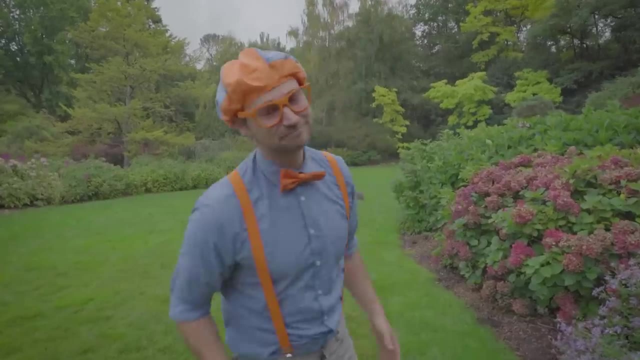 my videos. all you have to do is search for my name. Will you spell my name with me? B-L-I-P-P-I, Blippi, Good job, All right, See you again, Bye-bye. Bye-bye. Three, two, one. 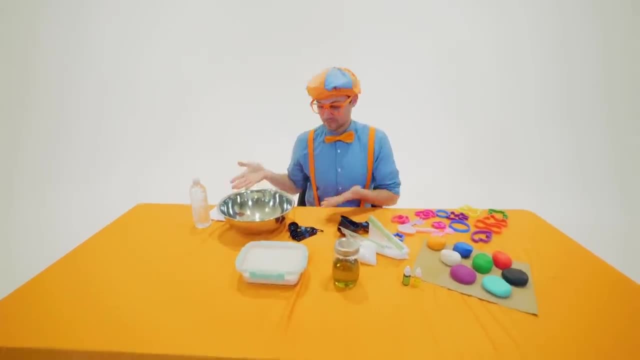 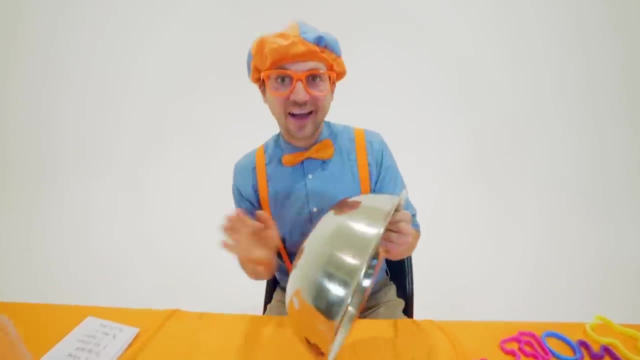 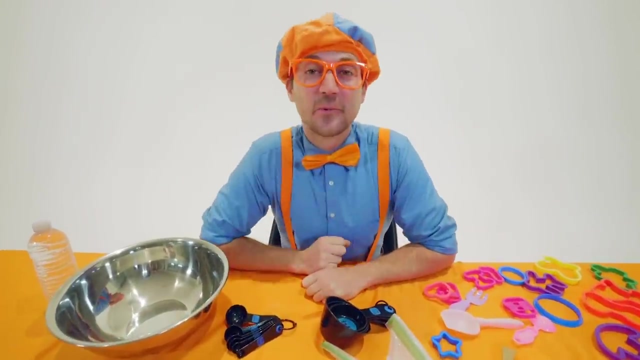 Hey, it's me Blippi, And I was just making some sweet tunes with this bowl, And do you like that? That's funny. But hey, today we're not going to learn about tunes, We're going to learn about, yeah, how to make. 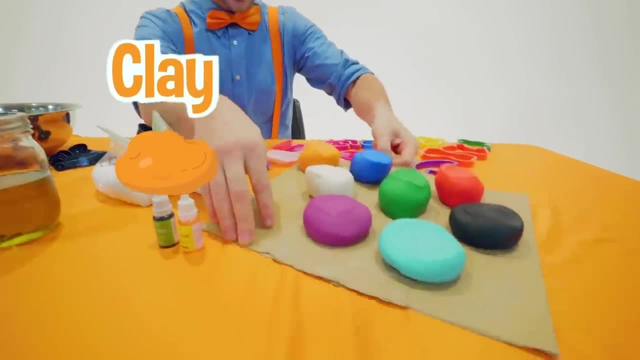 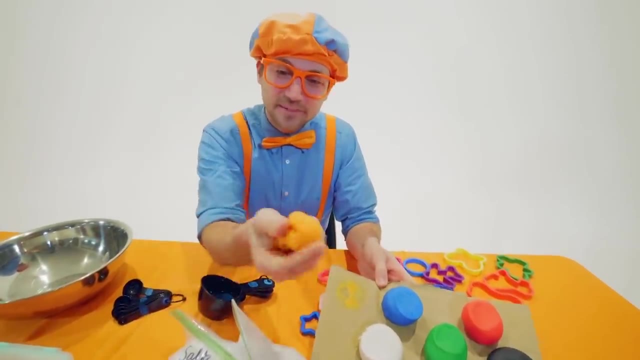 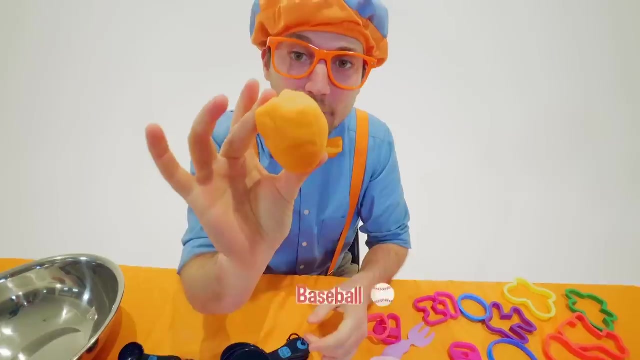 clay: Hey, yeah, look at it. Look at how many cool colors I have. Whoa- Look So much fun to play with Whoa And you can roll it up and make things with it. Look, I just made a baseball. 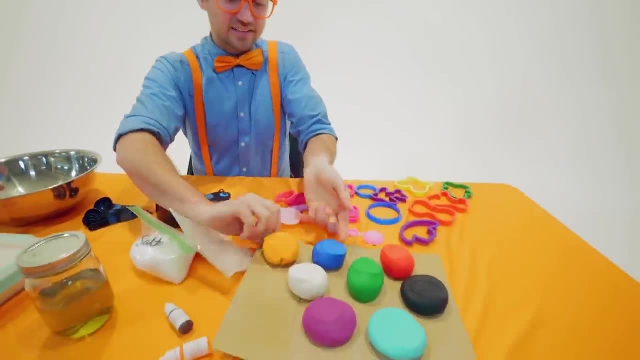 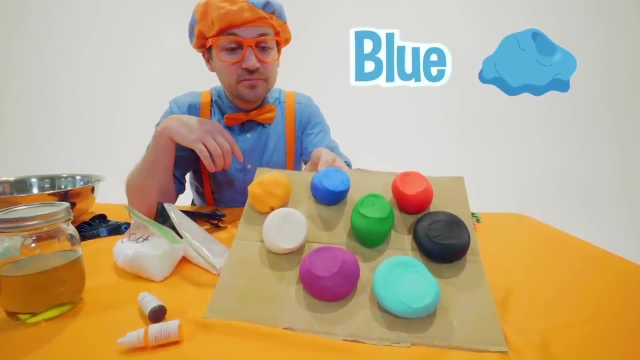 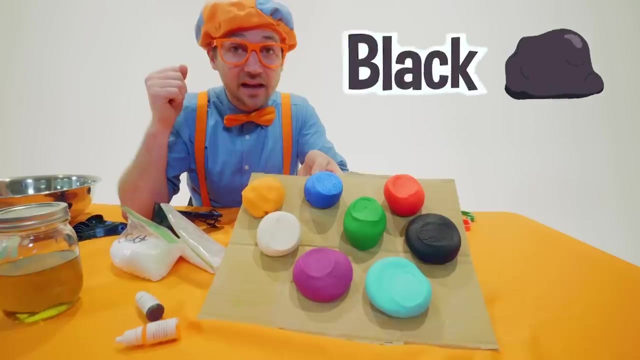 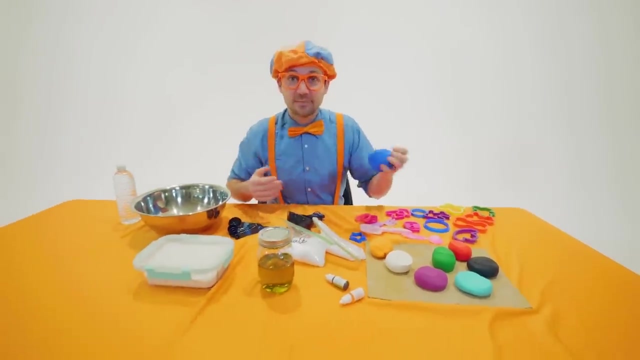 Wow, All right, Let's look at all the colors we have: Orange, white, blue, purple, green, red, black and light blue, Whoa. And today, yeah, you and I are going to make some of this. 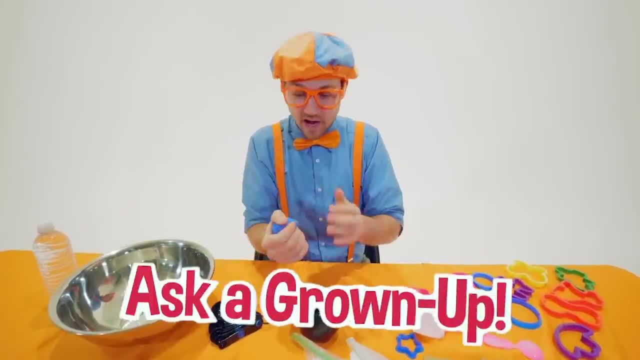 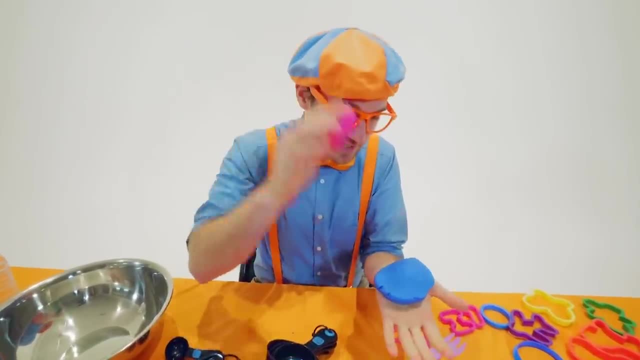 Yeah, And this recipe you can make at home with a grown-up- Yeah. And then, after you make it, you can squish it nice and flat, And then you take some of these and eat, And then you cut it out. 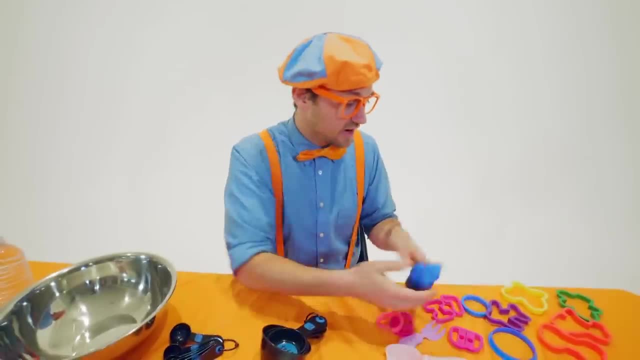 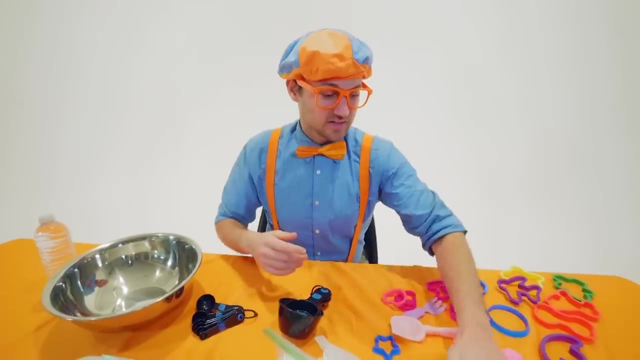 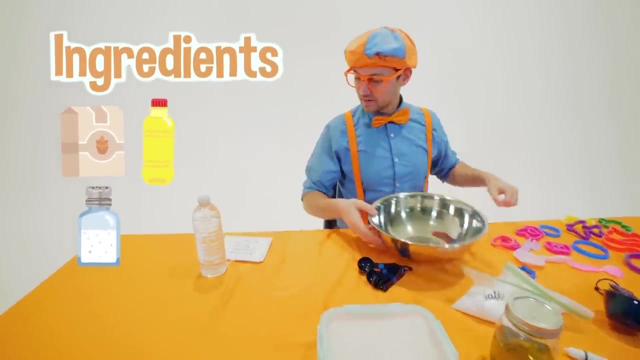 Whoa, And maybe we can spell some words. Maybe we can make an airplane together. Whoa, This is going to be so much fun. Okay, So the first thing we have to do is have all the ingredients for this clay. Yeah, Here we go. 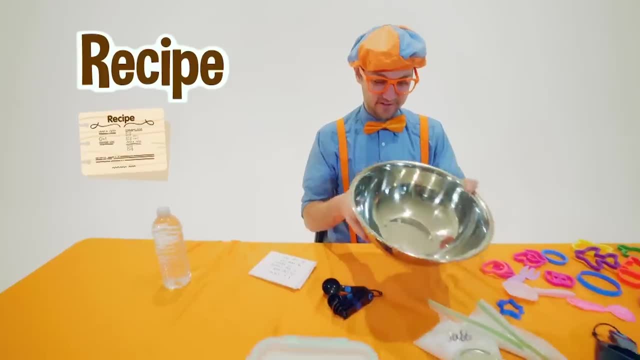 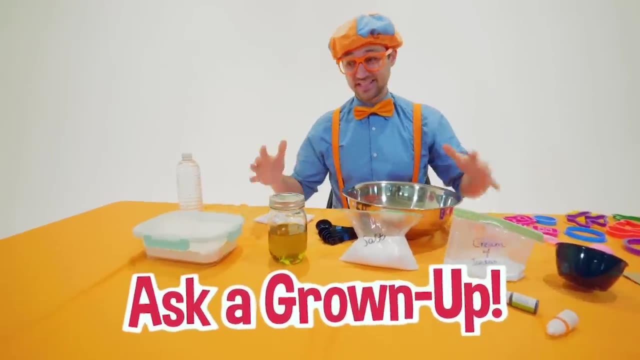 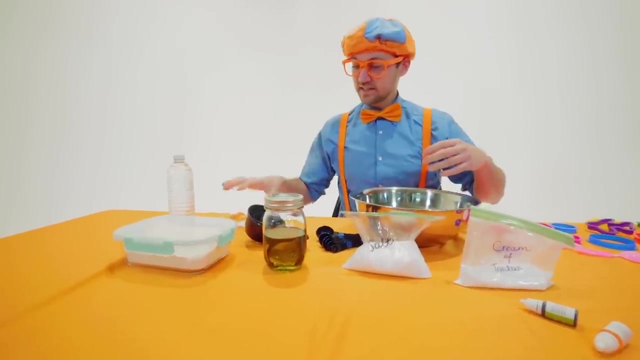 And I have my recipe right here. First we need a bowl, And what I would do if I was you, I would probably have a grown-up help you, because this can get really messy And there's a lot of ingredients, Yeah, All right. So first we need to start with one cup of flour. Whoa, Okay, Let's. 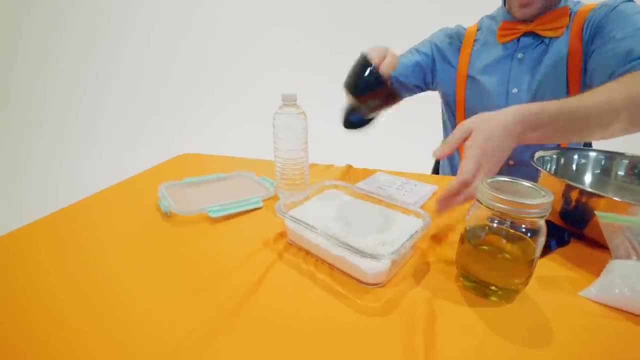 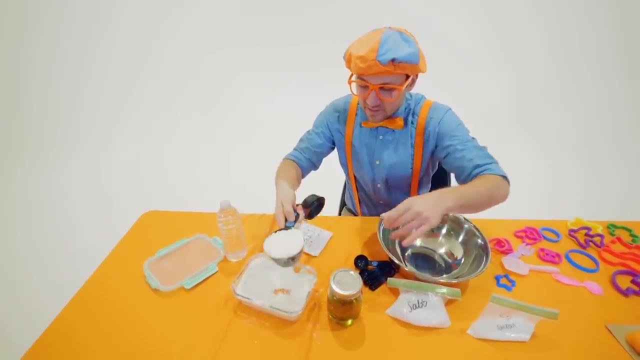 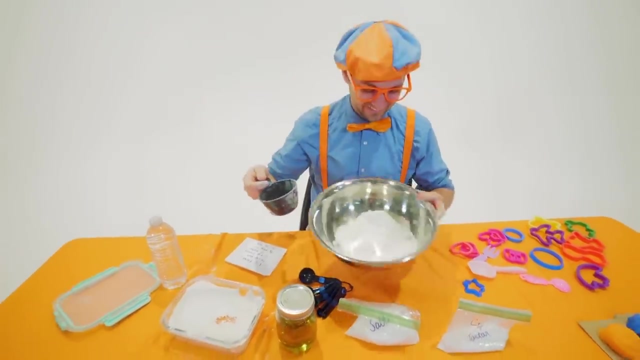 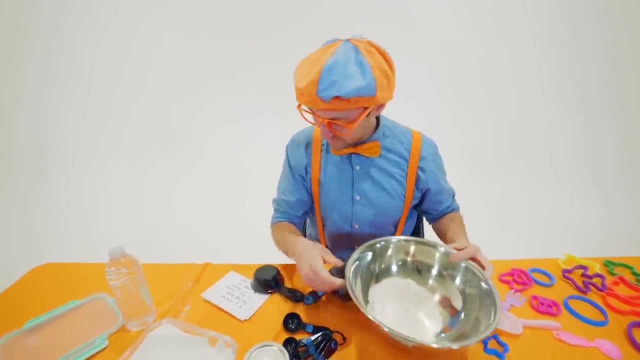 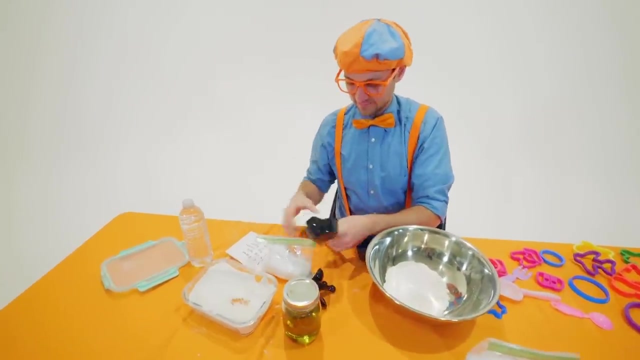 open this up. There we go, And it doesn't need to be exact. Yeah, That is one cup of flour, Here we go. Whoa, Wow, That is a great bake. Okay, All right, Let's see. One quarter cup of salt. All right, It is definitely already getting. 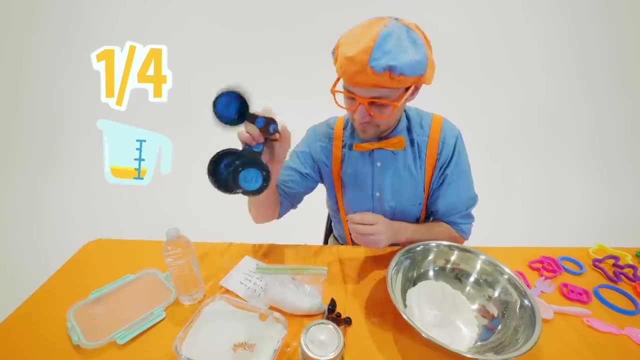 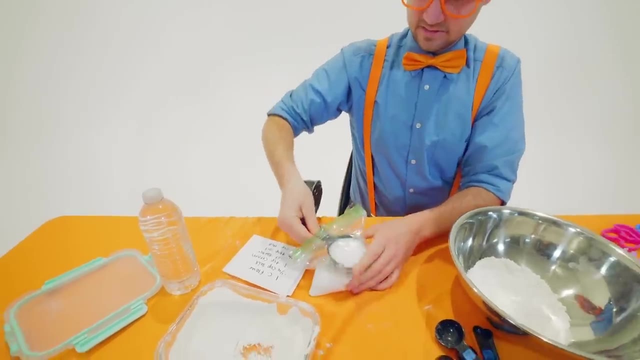 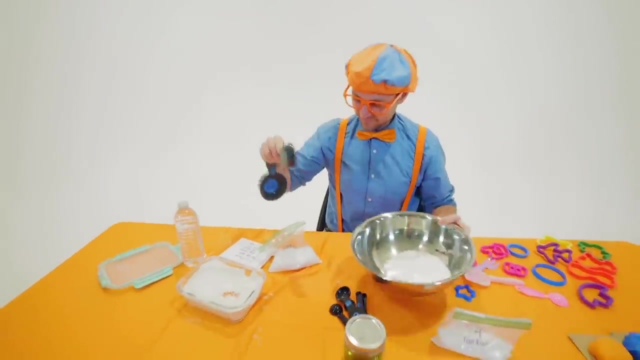 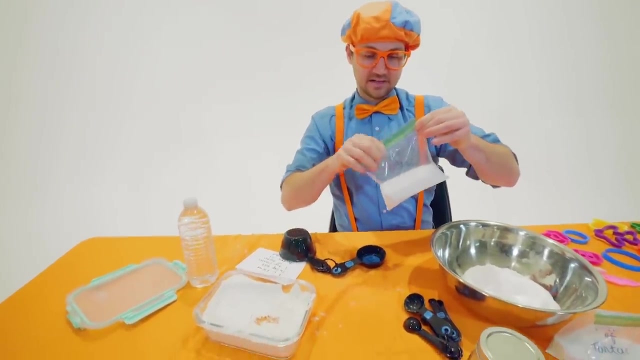 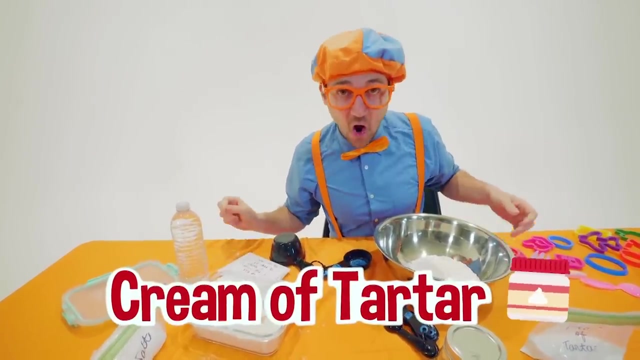 really messy. Okay, One quarter cup, And then we need to grab some salt. Here we go: Perfect, Ready, Three, two, one, Whoa, Perfect, All right. Okay, Let me zip this back up. Yeah, Then we need one teaspoon of cream of tartar. 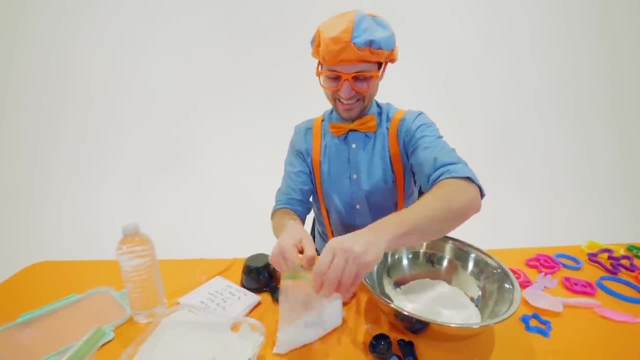 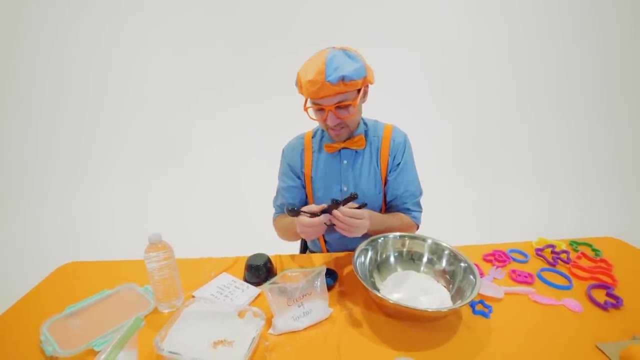 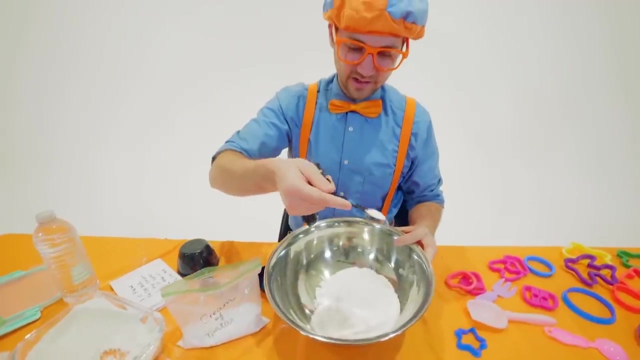 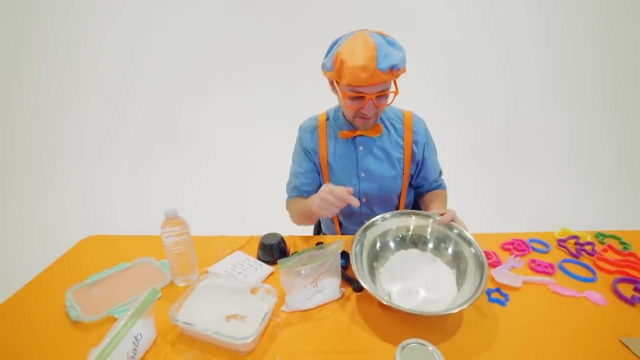 What a silly name. That's so fun. Cream of tartar: One teaspoon- Oh, there's so many. Okay, Here we go. Here's one, Here we go, And we're going to mix all this up in a little bit, But for now let's pour all the. 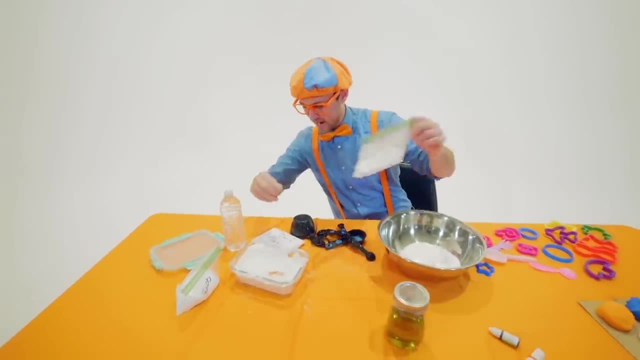 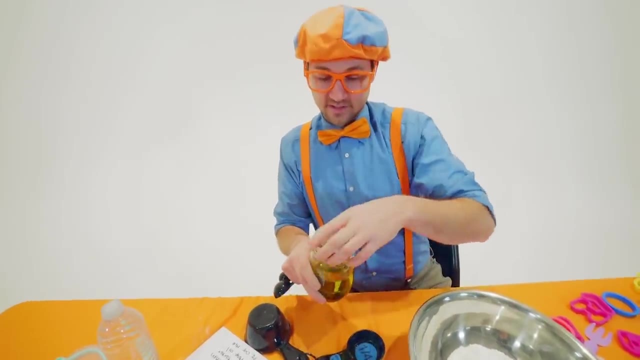 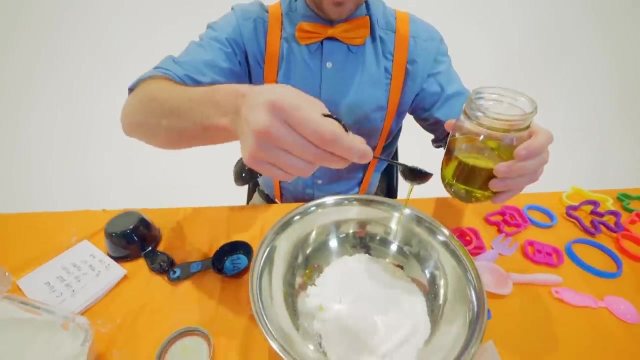 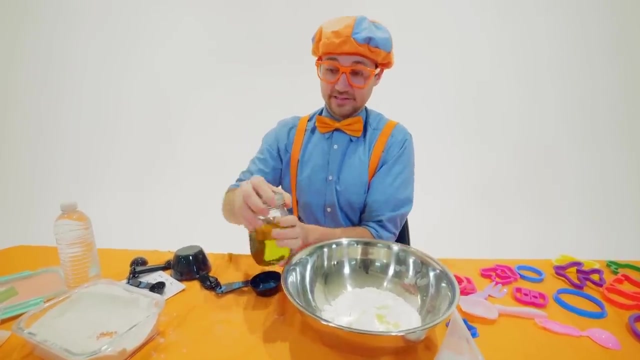 ingredients in here. Then we have a half a tablespoon of oil. Okay, Whoa, This is where it might get a little messy. Okay, Perfect, All right, Put the lid back on, Just so it does not spill. That would be bad news, Barry. Okay. 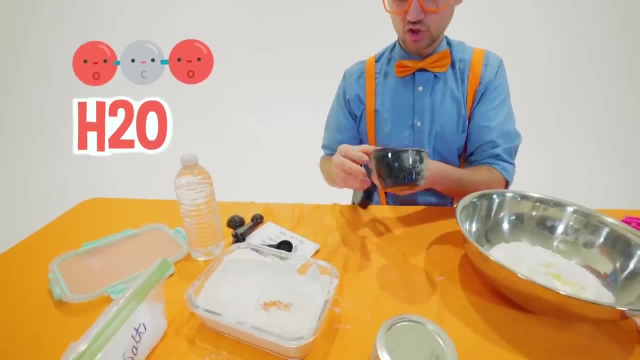 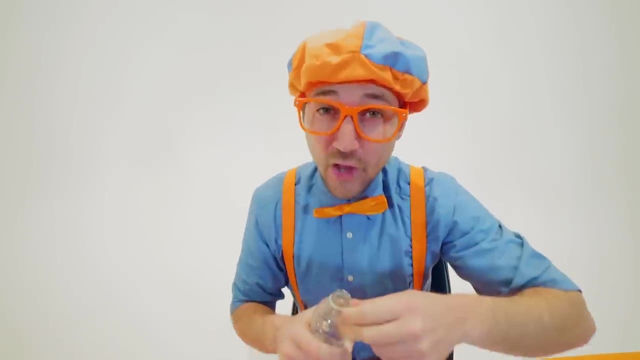 And then we have a half cup of H2O. Do you know what H2O stands for? Yeah, Water, I love water. All right, Half of a cup, Perfect, All right. Oh, hey, look at all that. 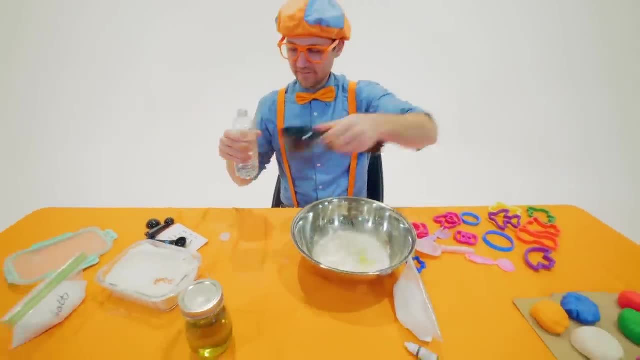 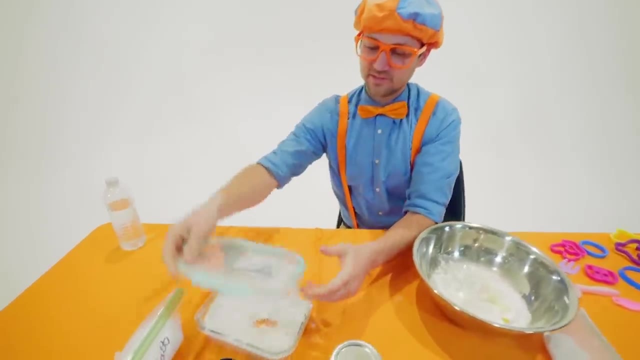 Nice and clean. Nice and clean, That's nice and teachy. I like it, You like it, You like it. How do you like it? Look, I forgot to close up the flower. You should probably do that. All right, let's push all that stuff to the side. 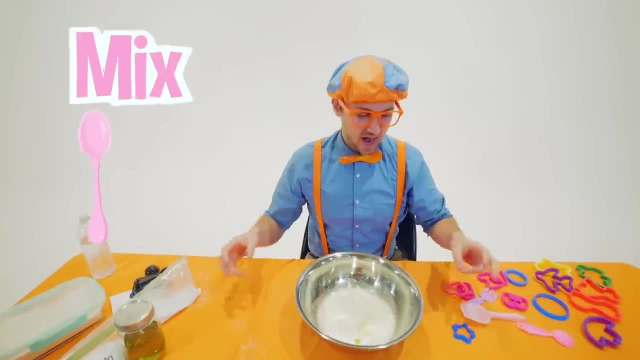 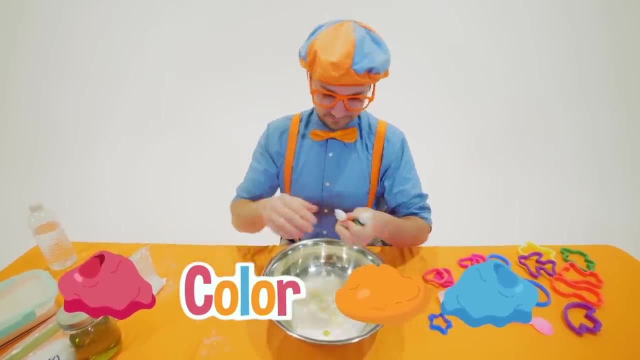 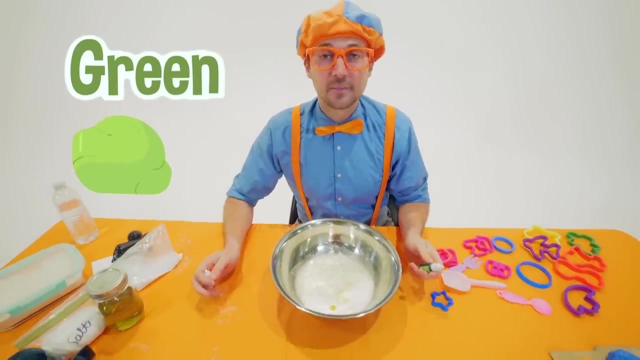 because now we're ready to mix it up, But what we need to do is put in some color. You can make any color you want, But what we're gonna do, although we already have a green color, I think we should make another green. 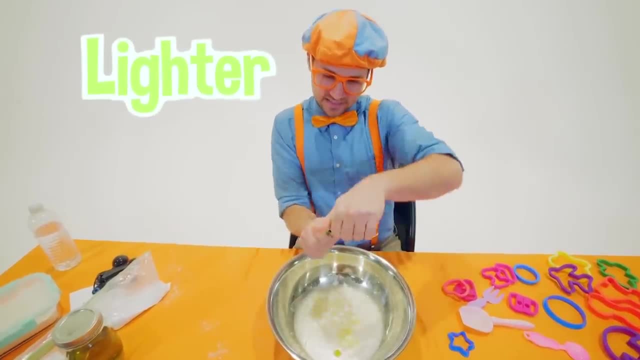 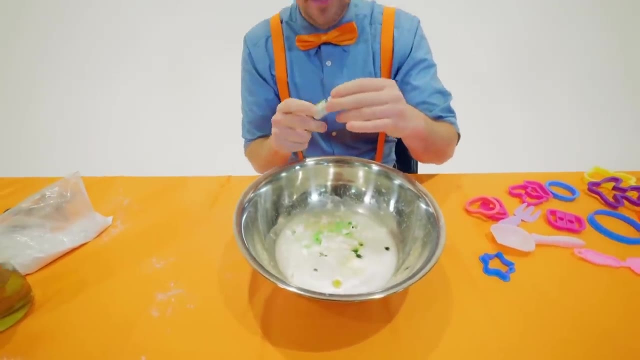 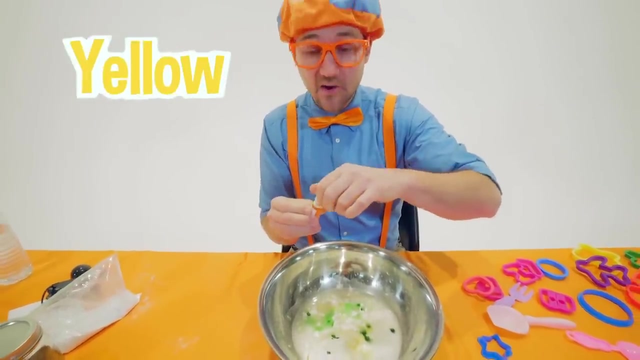 But this one will be a little bit lighter. So let's open this up, add some green. I don't know how much to add, but that seems like quite a bit. And then also I'm gonna add a little bit of yellow. 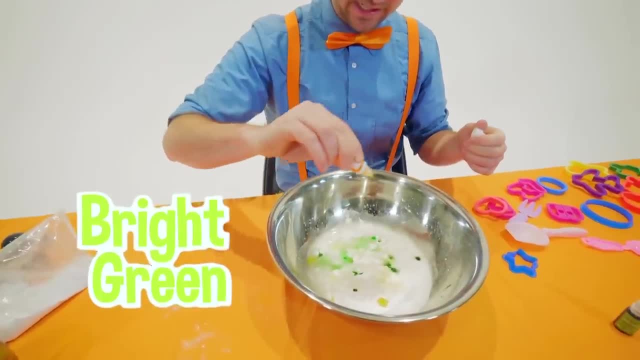 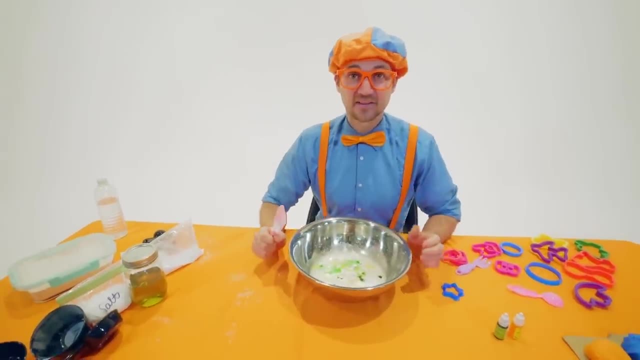 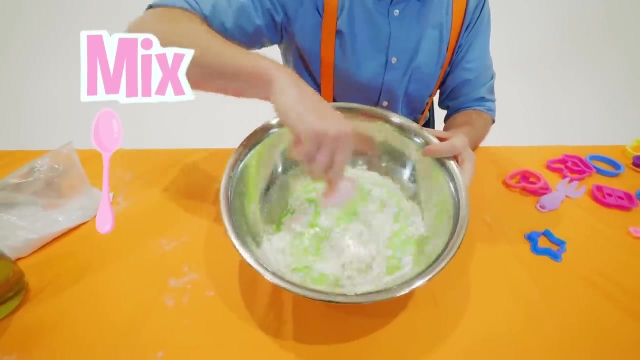 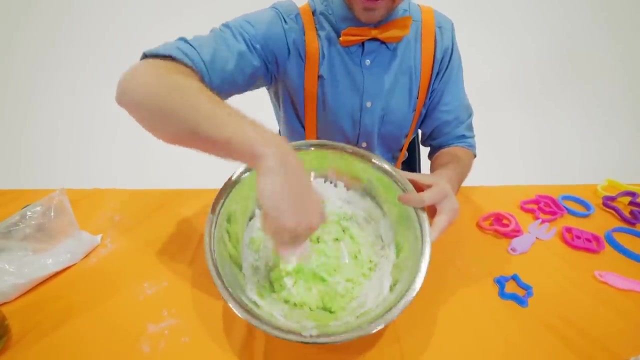 Yeah, it's gonna make it more of a bright green. Let's close that up. Whoa. that was a fun recipe to make, But now I gotta mix it up. Whoa. it's looking so good. Wow, You see it. 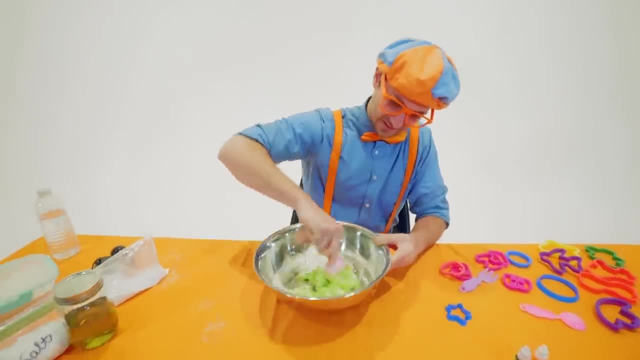 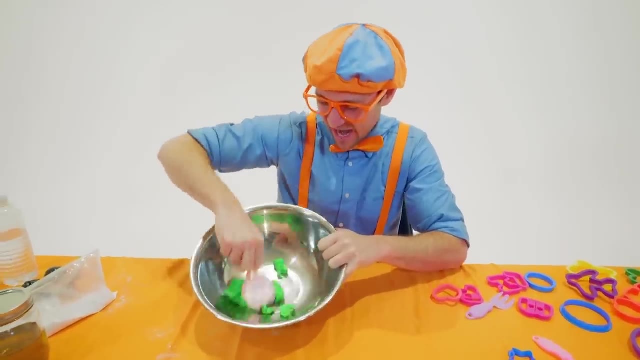 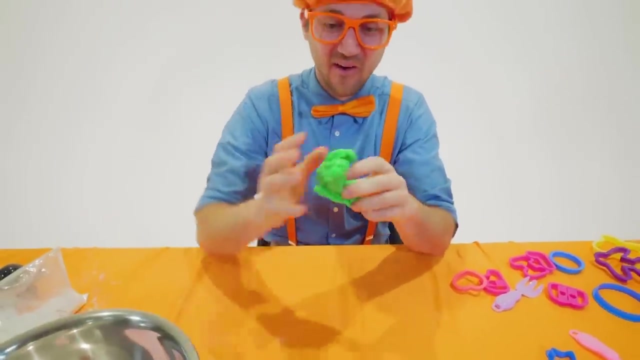 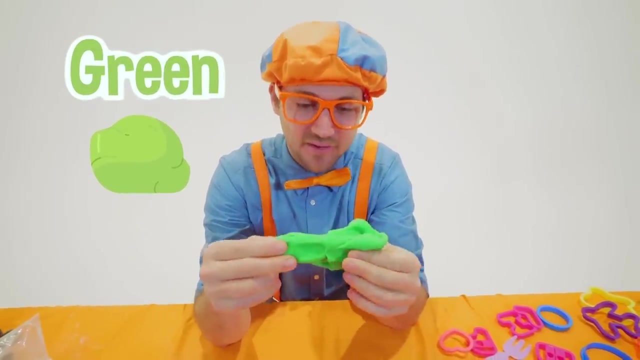 Whoa. all right, let me keep mixing it up. Whoa, yeah, we did it. Whoa, check it out. Wow, whoa, homemade clay. wow, What a pretty green color. we made good job. I wonder what color you're gonna make at home. 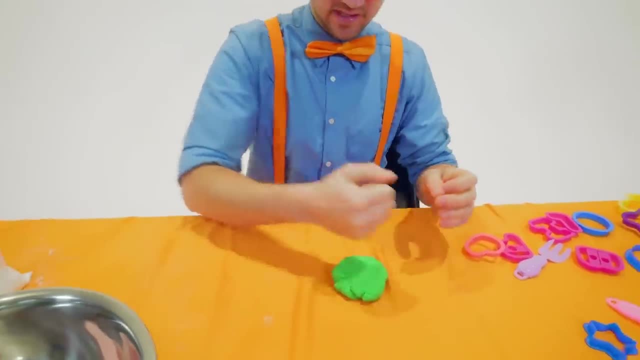 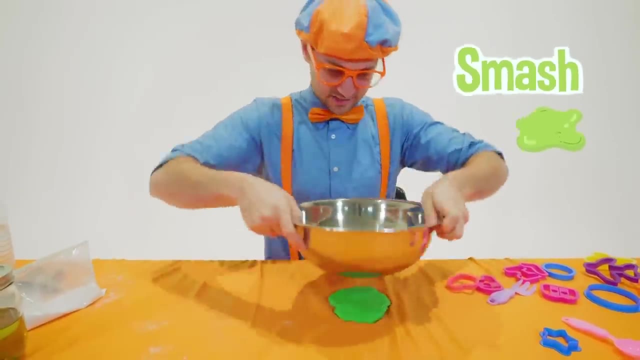 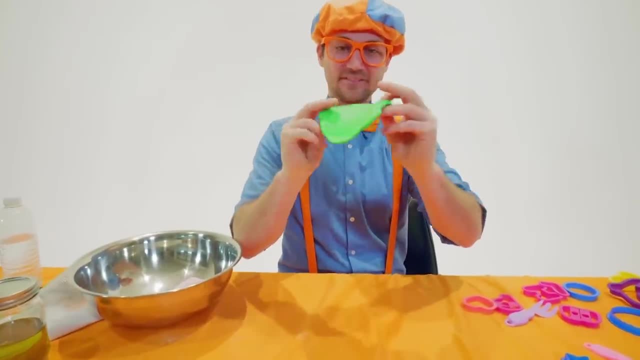 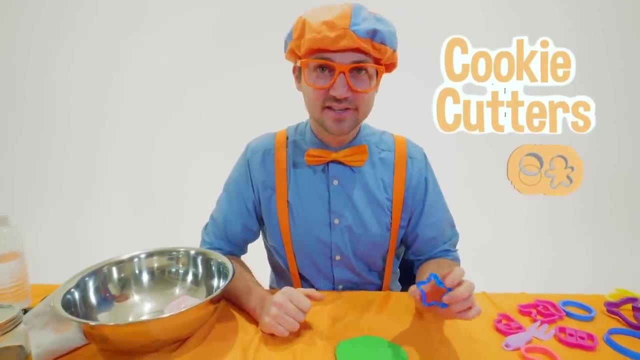 Oh, that's silly. Okay, let's peel it off. Wow, perfect. And then now you can use these. Yeah, they're like cookie cutters, But these are definitely not cookies that we're making. I would not eat this. 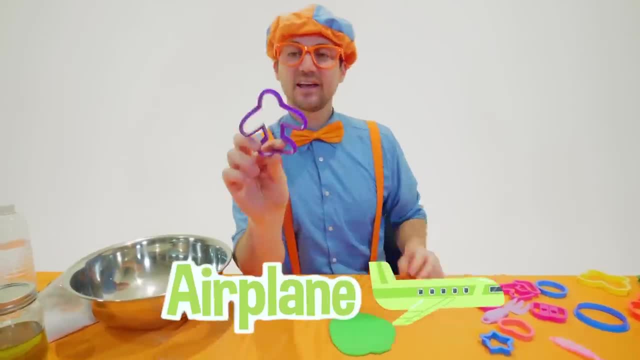 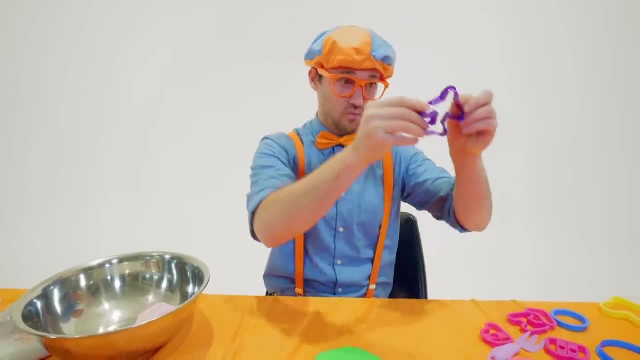 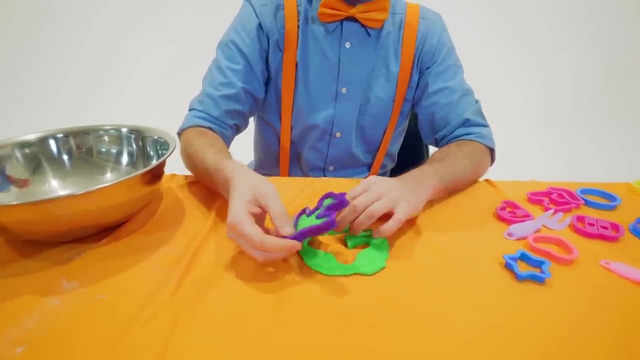 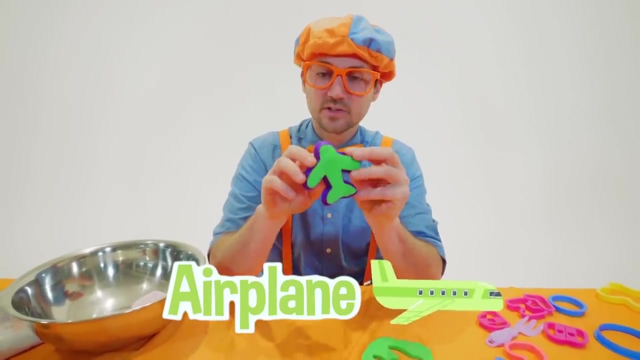 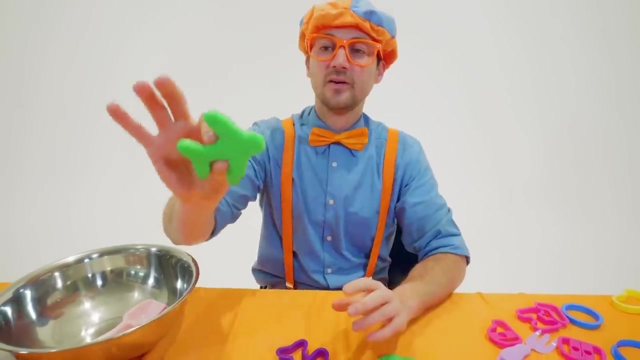 Okay, all right, okay, Yeah, remember that airplane. Pew pew, pew, wow, yes, yeah, check it out. okay, now you push it down. whoa, look, cut an airplane out, but first let's push it out of here. wow, yeah, we did such a good job. 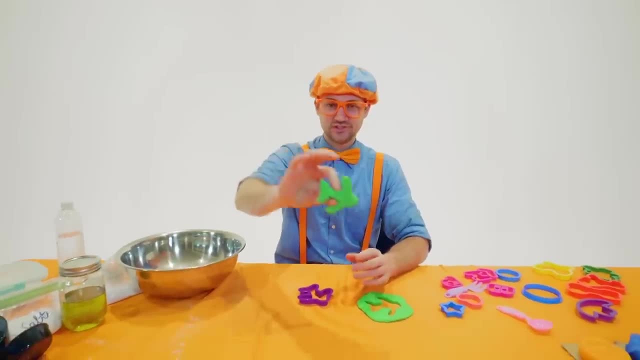 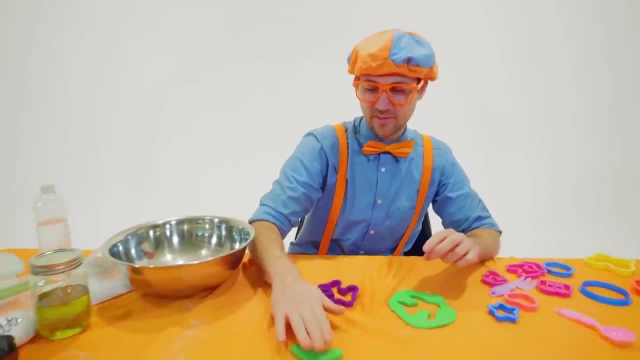 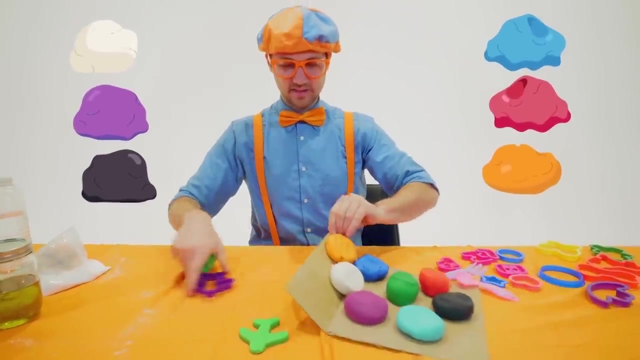 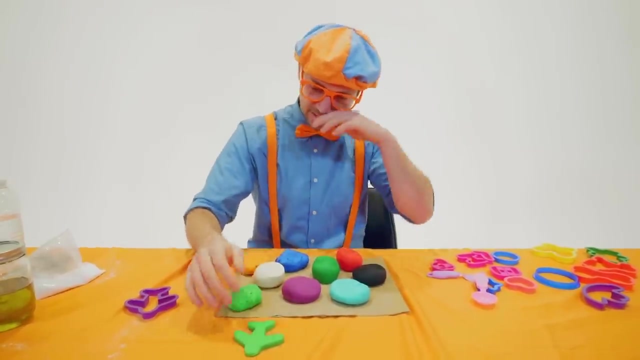 wow, okay, i'll put that airplane right there now. let's bring all the colors that we have out and then let's see what we can make together. okay, so let's put that green back and we have the airplane right there. what else? oh, we have some. 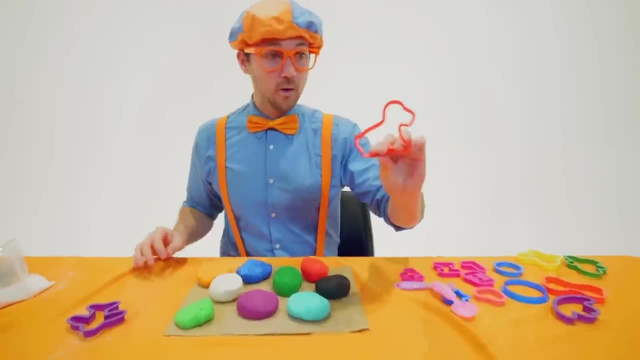 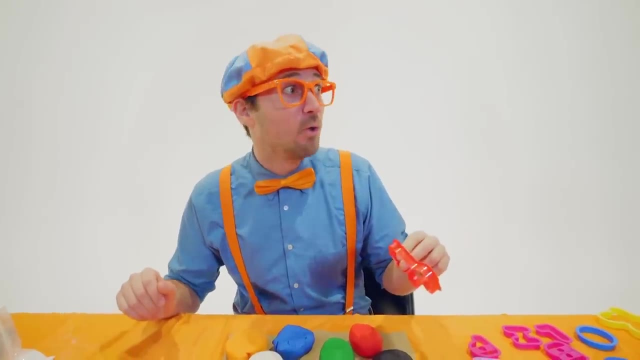 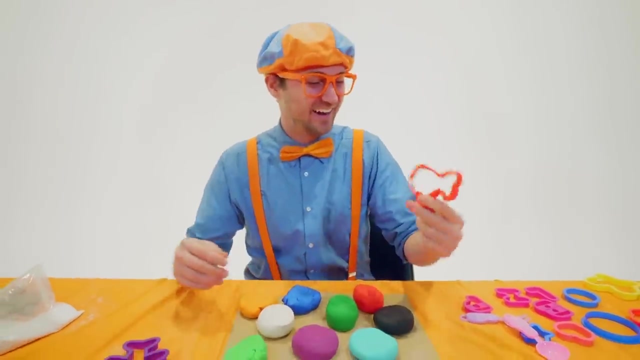 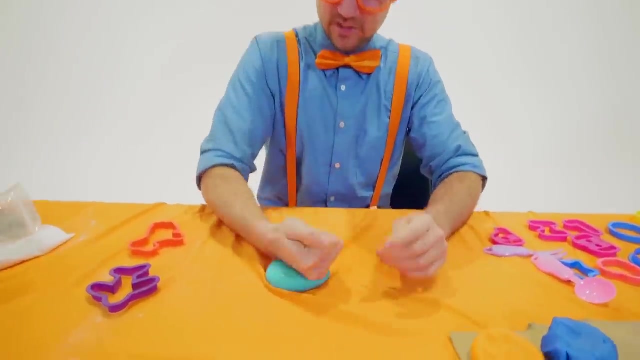 okay, so let's put that green back. okay, so let's put that green back. letters. We have, ooh, a dog. Will you act like a dog with me? Ready, Wow, Dogs are so cute. Okay, let's make a blue dog. That sounds pretty silly, doesn't it? Okay, you know what to do: Smash out. 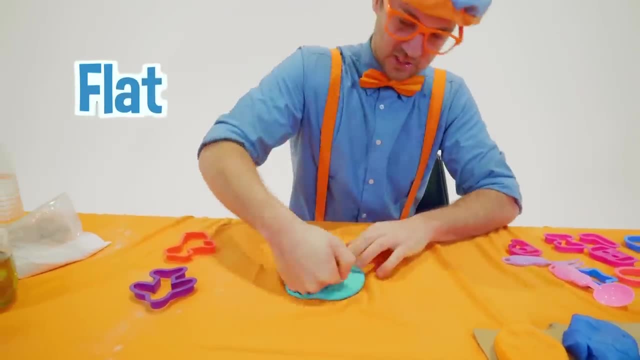 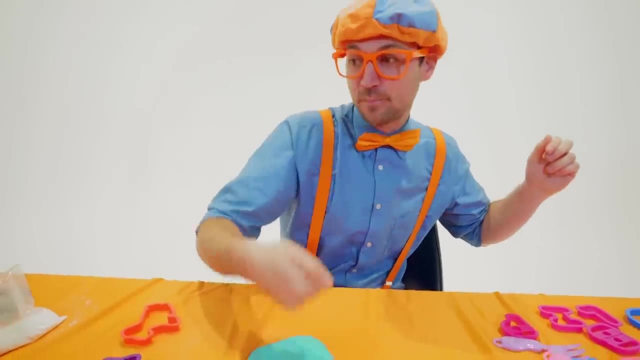 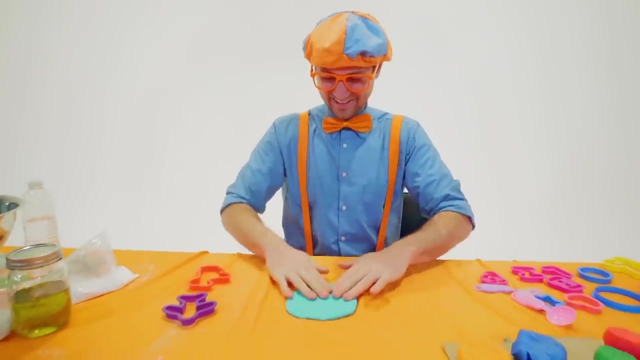 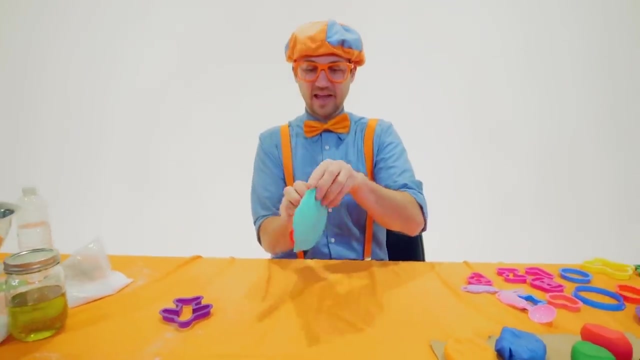 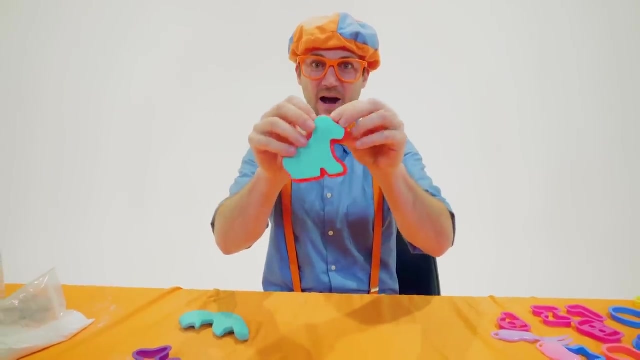 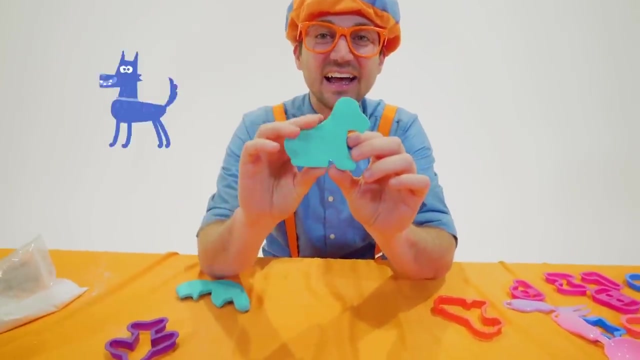 your clay nice and flat. Okay, here we go. All right, push it down. All right, Whoa, look at that. Whoa, Pull the sides away, Wow, And now? oh, that's silly, Look what is that. Yeah, it's a little poochie. 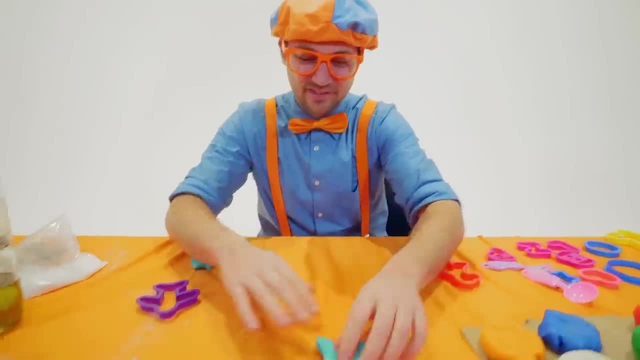 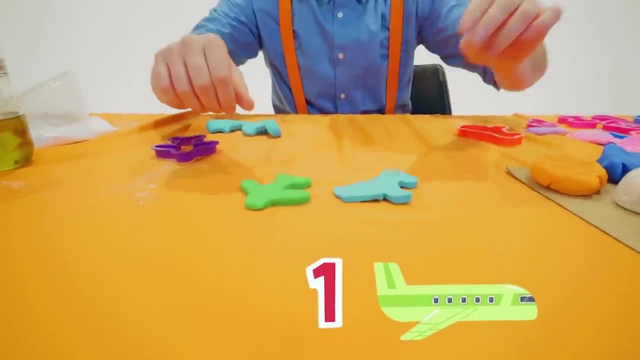 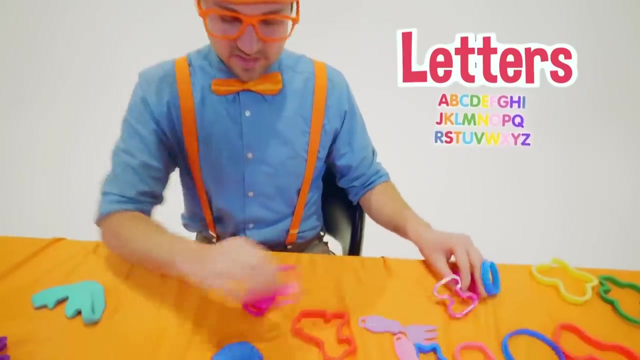 Okay, we'll save you, We'll put you right there. Perfect, All right. One pooch and one airplane, Perfect. Oh hey, I think we have some letters over here. We can spell something out. Okay, Looks like we have a, B, a, P. 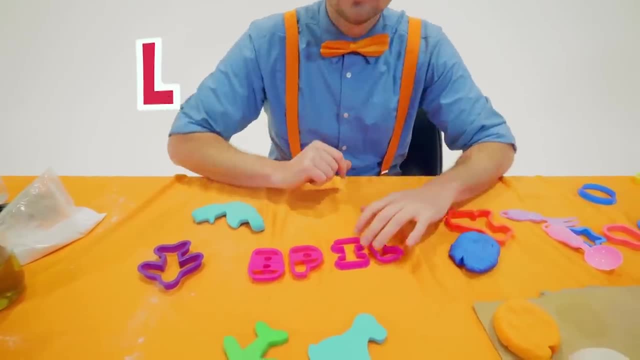 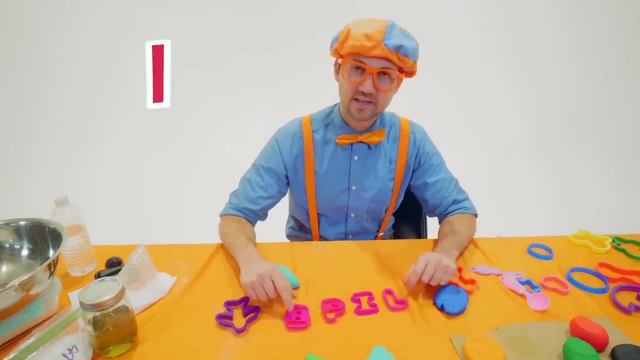 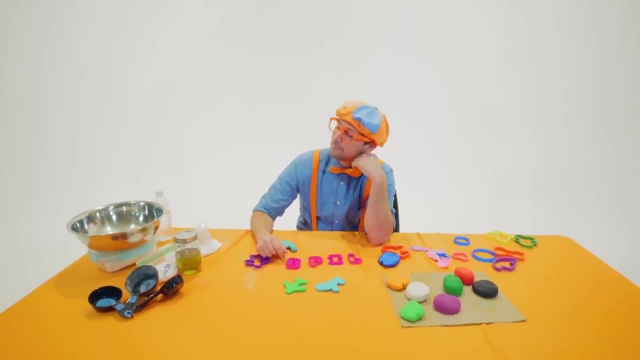 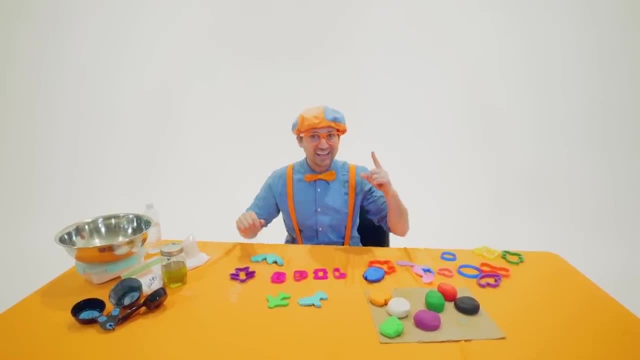 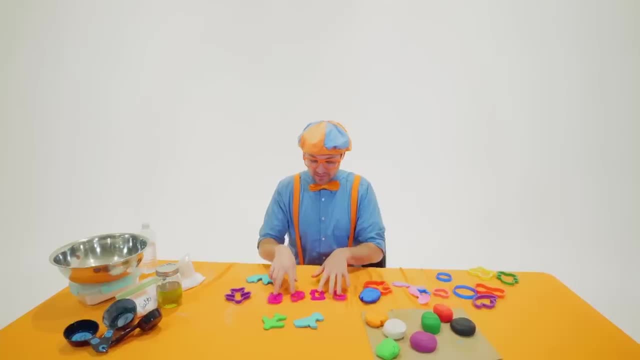 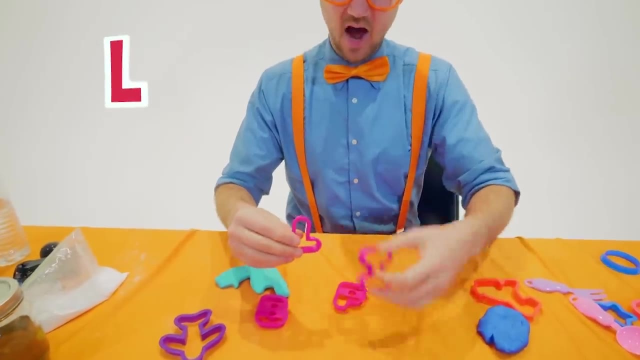 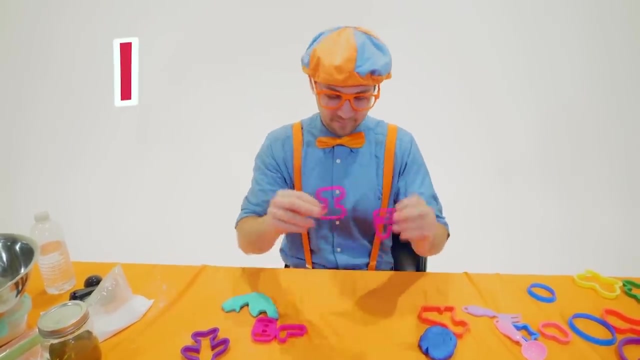 Yeah, We can actually spell my whole name out just with these four letters. See, We would go like this: We would use a, B, an, L, an, I, We would do two Ps And then we would use another, I. Perfect. 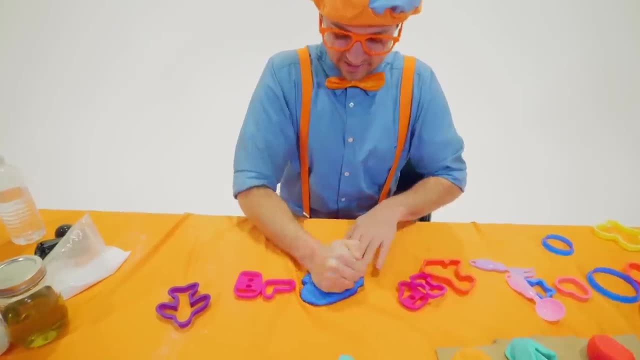 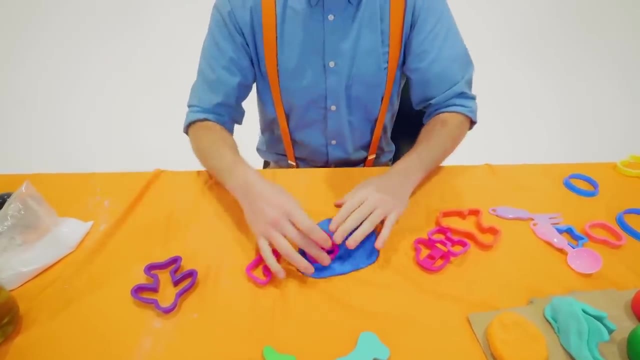 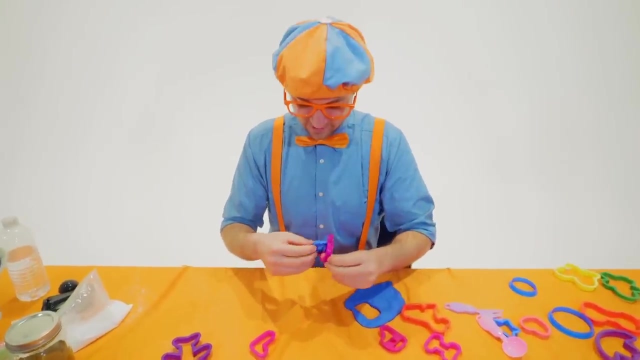 All right, Let's do that. All right, First we need some colors. So Let's use this blue color. Yeah, there we go. Let's do a, B right there. Perfect. Well, this is gonna be so cool. Yeah, and if you use some of this at home, maybe you could spell your name. 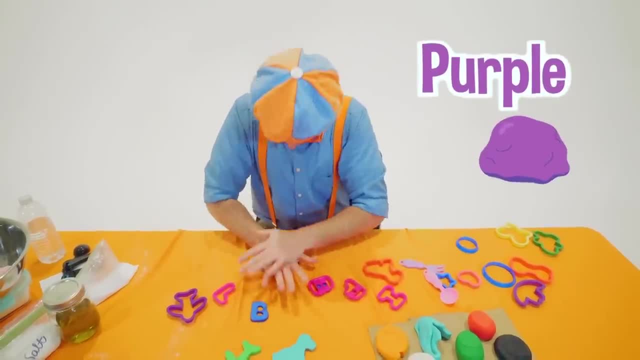 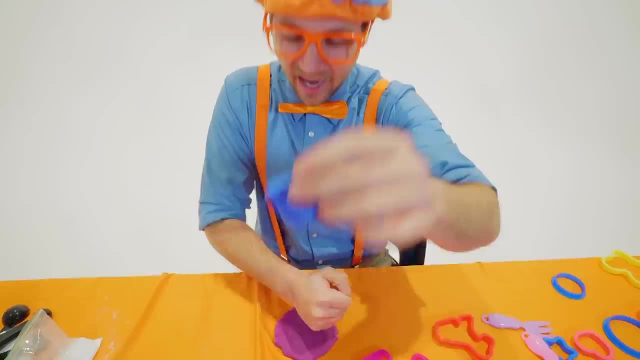 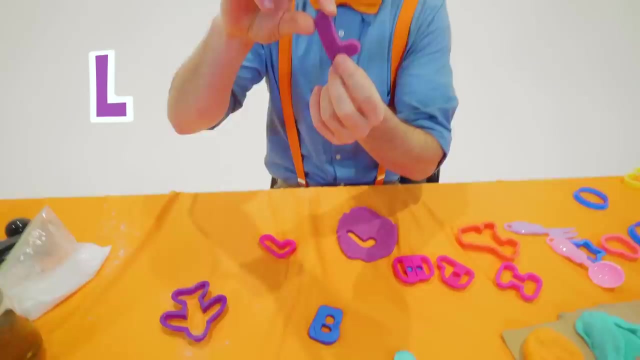 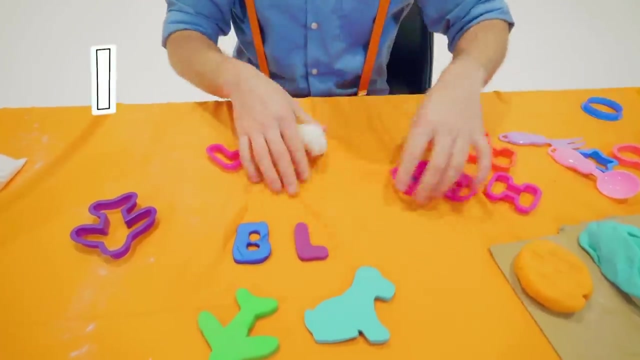 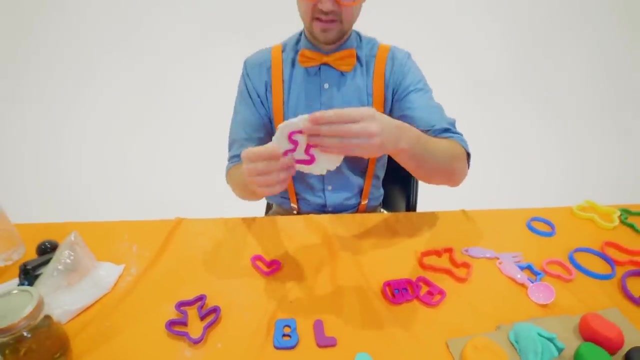 Okay, let's use some purple. Alright. so we've got a blue B right here, Yeah, Okay. and then we have an L. Alright, nice little L right there. Yeah, it's a B L. then we need an I. How does that look? yeah, whoa. 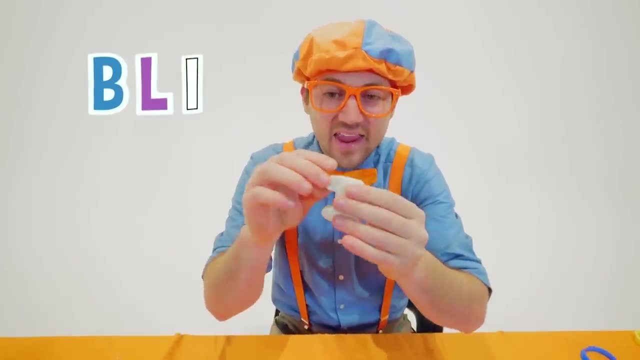 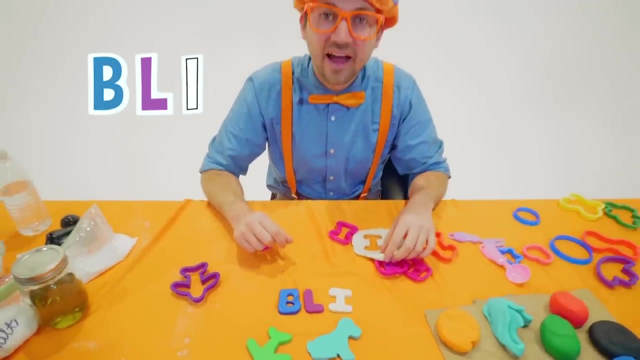 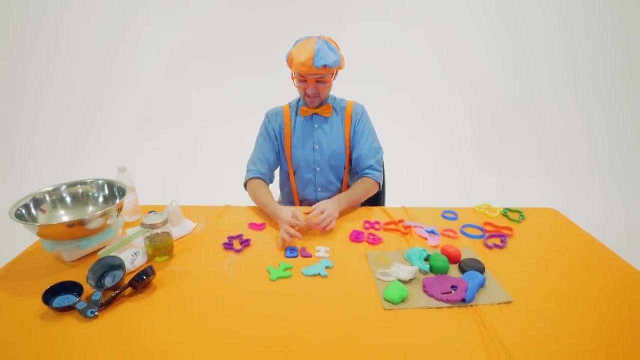 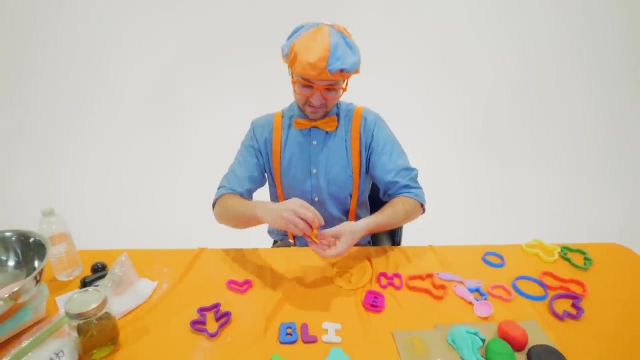 Okay, B L I. Yeah, B L I. What's the next letter? Yeah, P, and there's two of them. Let's use one of my favorite two colors: Yeah, the color orange. B L I, P. we need another P. We'll use the color black. 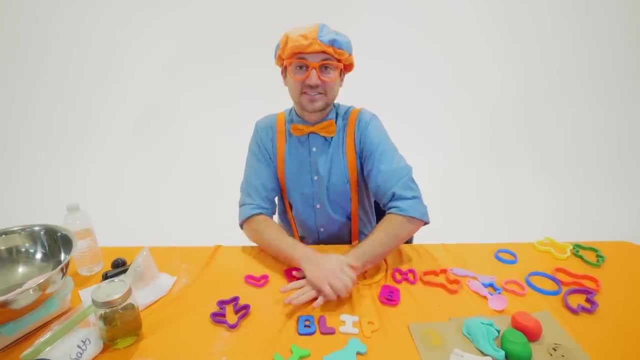 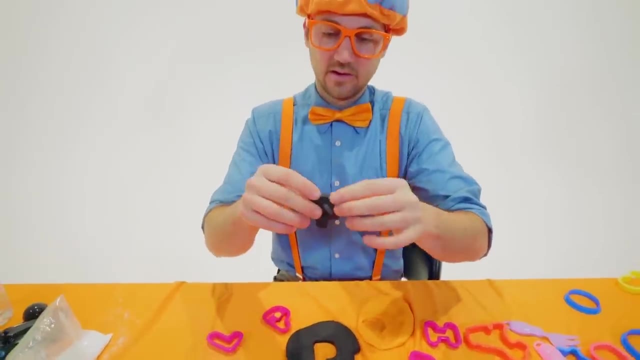 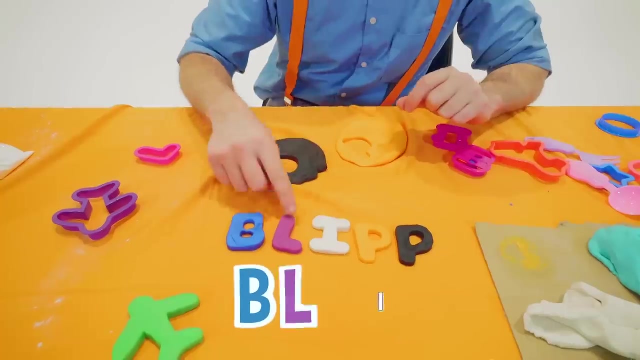 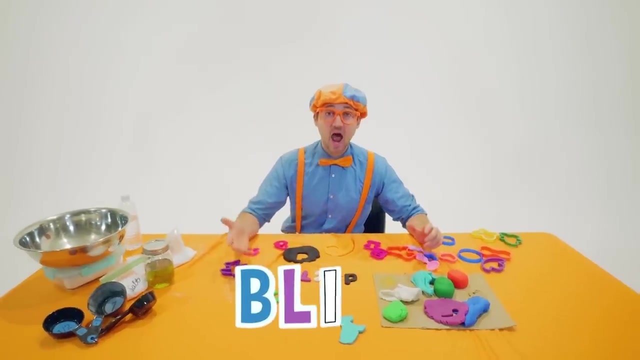 Huh, This is so much fun. It feels so cool on my hand. Ooh, another P, Yeah. so we got Here, we go. We got B L I P P. What's the next letter? B L I P P, Yeah, I. 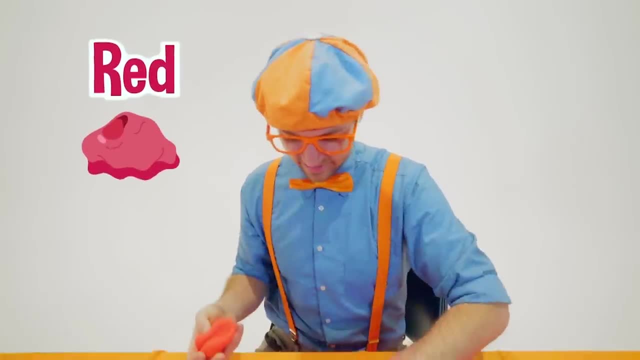 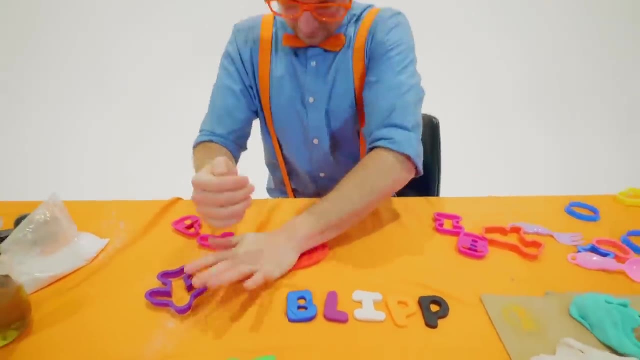 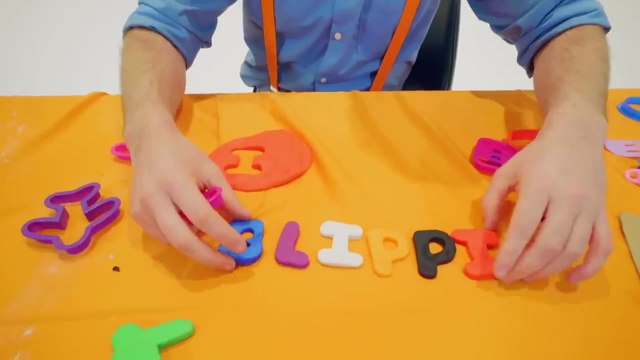 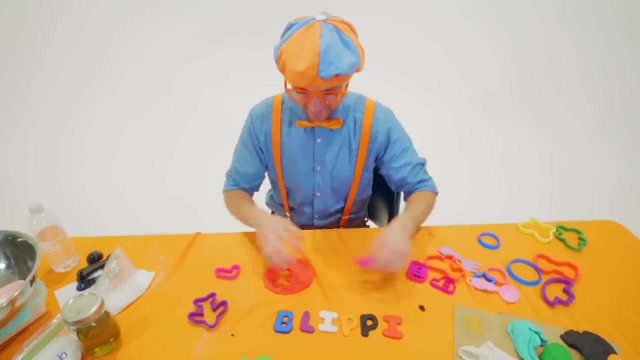 And let's use this bright red Pillar. All right, here we go. B L I P P I. Here we go. Oh, How does that look? B L I P P I. Yeah, good job, All right. Okay, let's put these down here with the dog and the airplane. 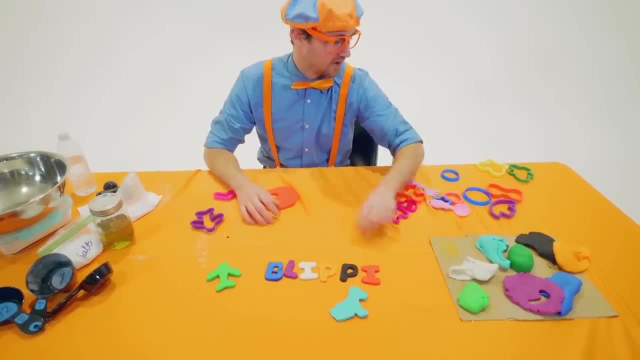 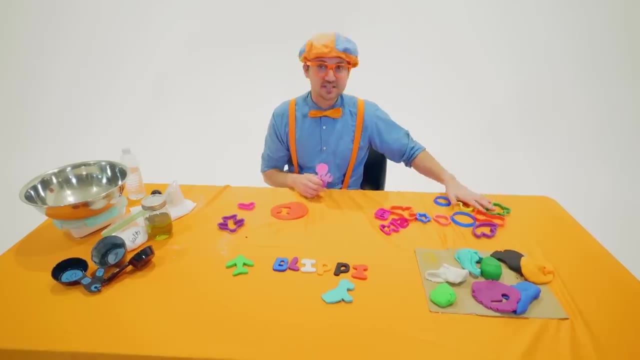 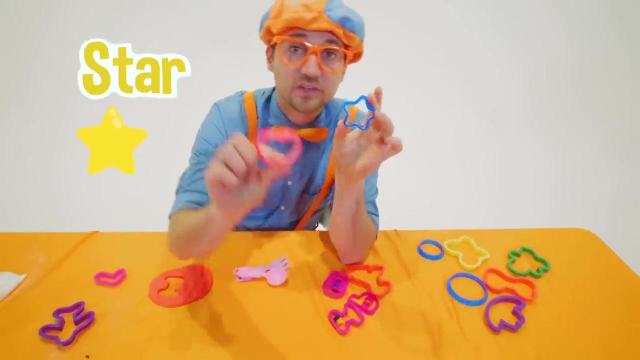 There we go. All right, Now let's make one more thing, Huh, Hey. well, since we have all these stencils and these cookie cutters, Yeah, you could actually use a lot of them. You can make a star, You can make a heart. 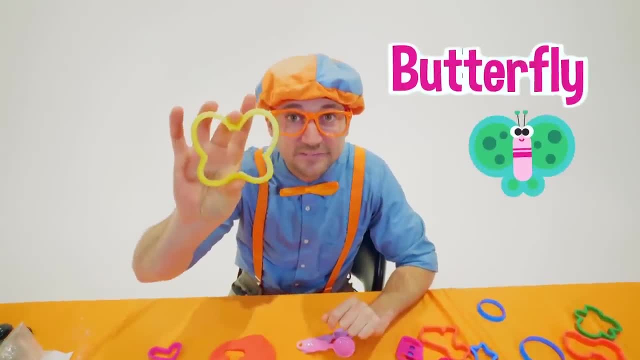 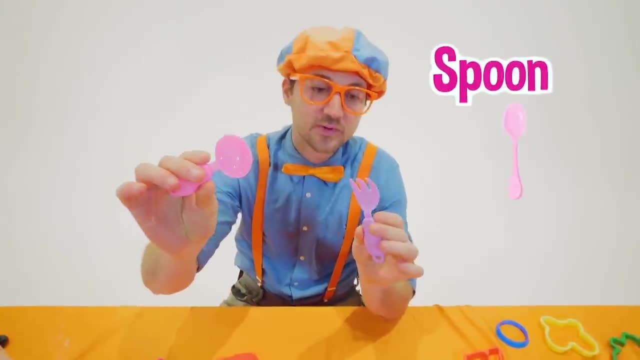 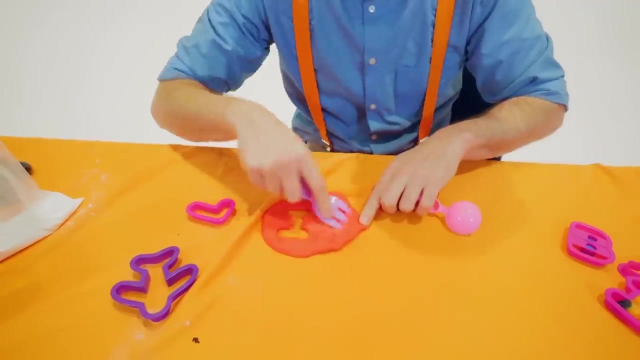 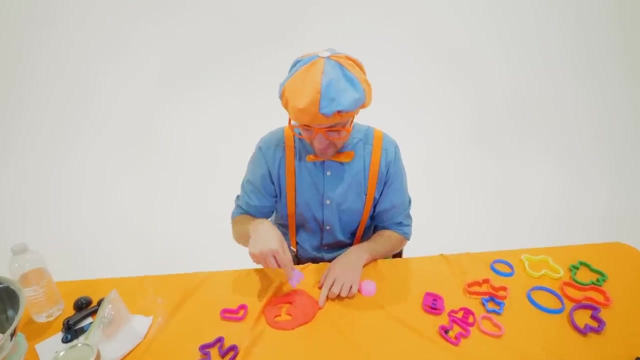 You could make Butterfly, Yeah. or you could use some other tools, Yeah, like this spoon or this fork, and see, Look at this, see, you can Use the fork and, yeah, act like you're in the garden. Yep, gotta make the soil nice and soft, so then you can plant some plants. 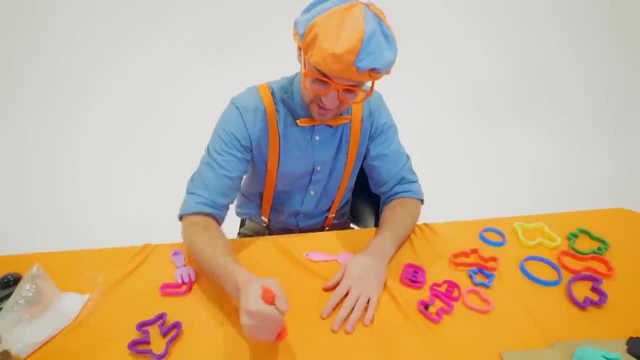 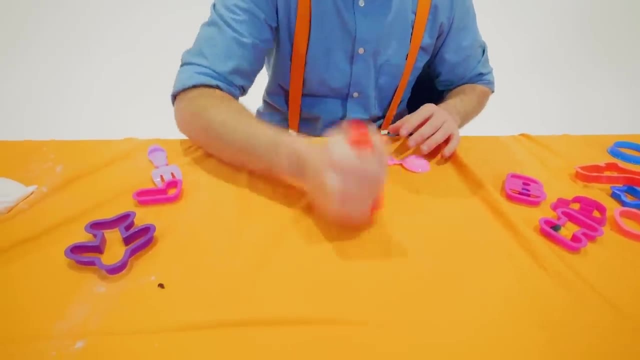 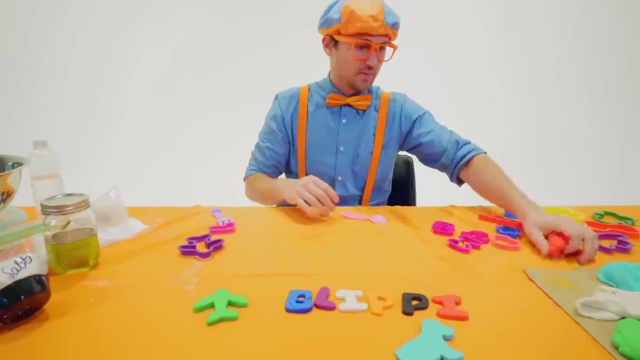 But I'm definitely making a mess with all these small pieces. This is a cool trick that I learned. see, you can actually pick up a lot of the pieces by smashing it. Yeah, it's kind of fun. Huh, Okay, but watch this. Hey, we haven't used this color of green yet. So if you take the spoon and 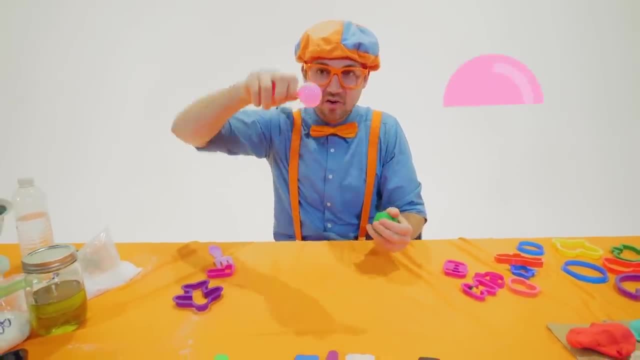 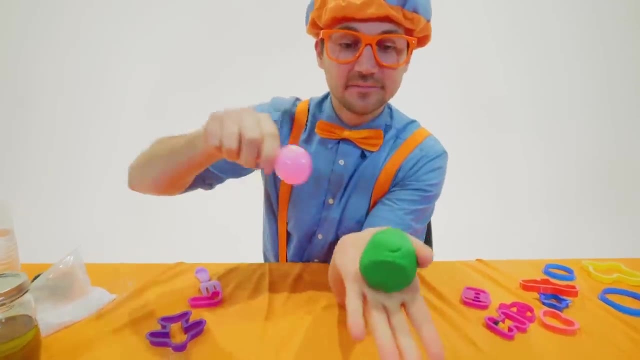 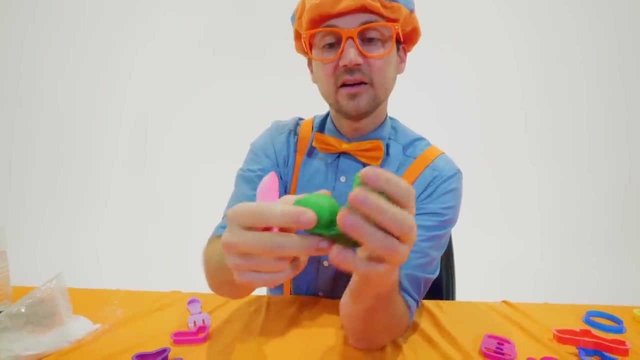 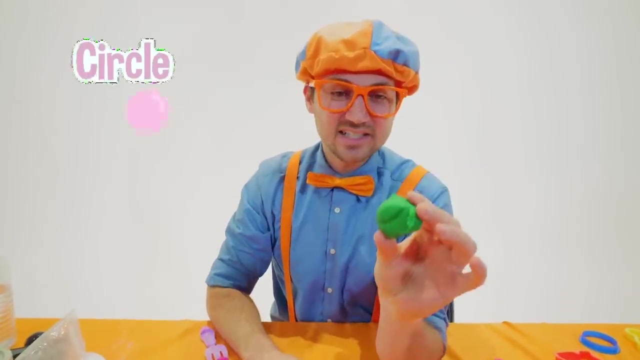 You scoop it. although it's a half of a circle, We go all the way around. you actually might be able to scoop a full circle. Okay, let's try it ready. Yeah, look, There we go. Whoa, It's like a circle, Wow. And then you can put it in your hands, roll it around. 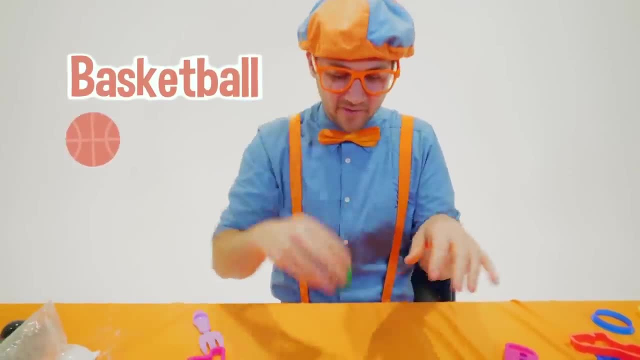 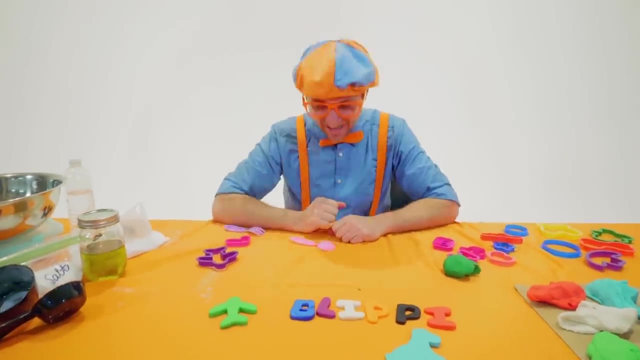 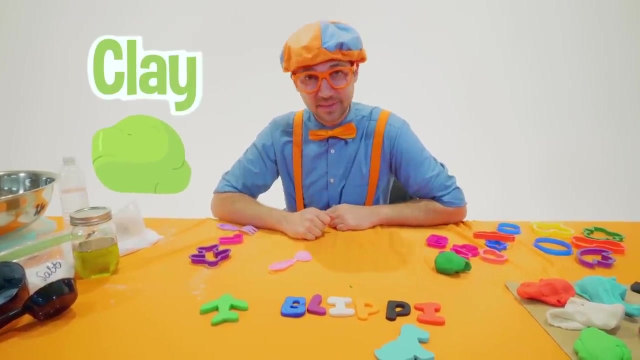 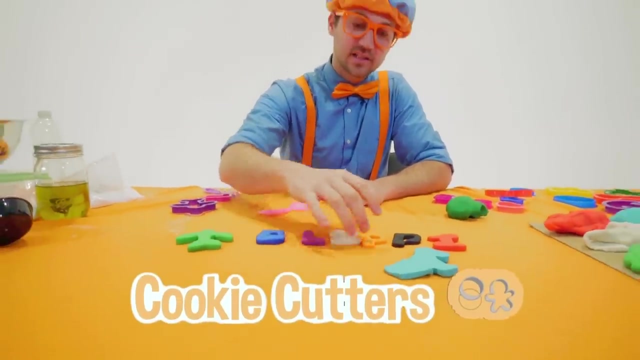 Yeah, look, It's like a basketball. That was silly. Well, this has been so much fun making this clay with you. Did you have fun making clay with me? Yeah, and it was really fun. Yeah, using those cookie cutters to cut out some of the clay into an airplane. 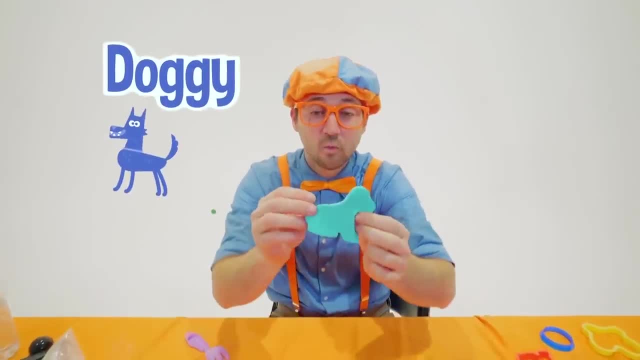 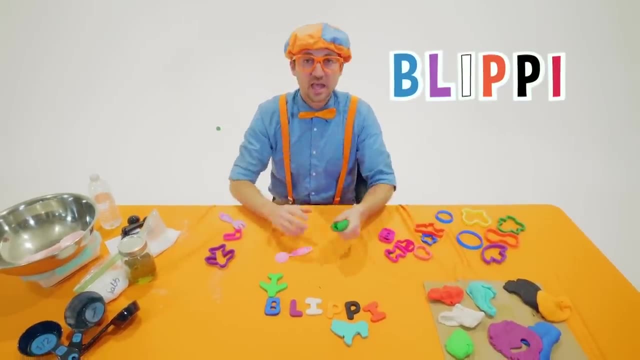 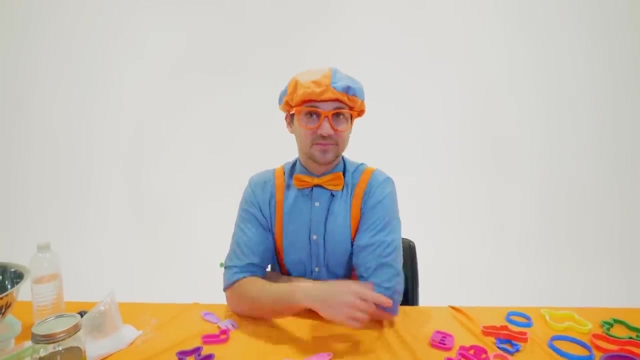 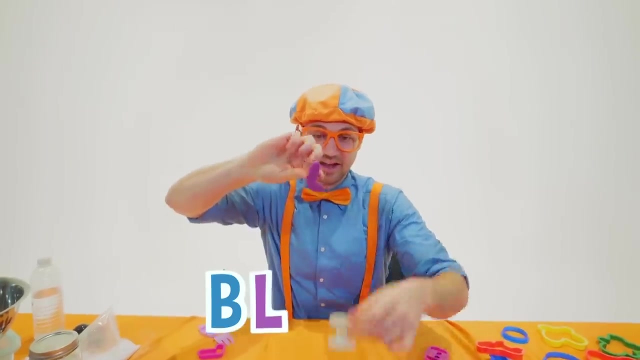 Yeah, a doggy And my name Blippi. well, this is the end of this video, But if you want to watch more of my videos, all you have to do is search for my name. Will you spell my name with me? Ready B L. 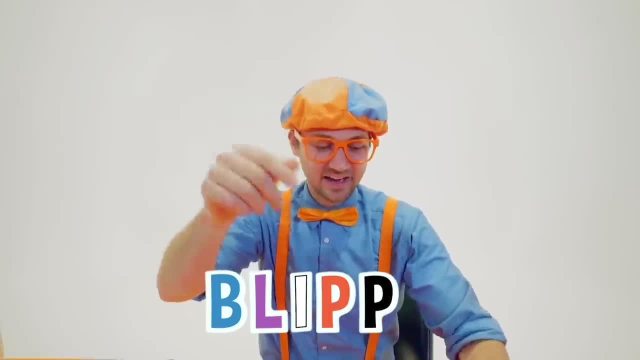 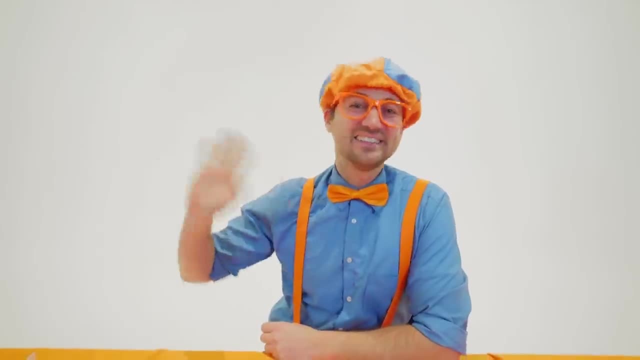 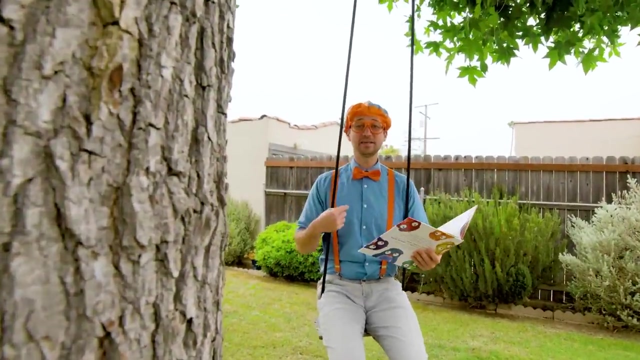 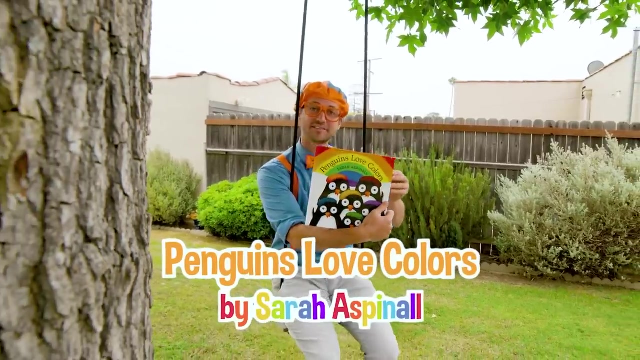 I, P, P, I, Blippi, All right, Thank you so much for being my friend. See you soon, Bye, Bye, Hey, It's me Blippi, and I'm just reading this really cool book- Yeah, it's called penguins, Love colors by Sarah Aspinall. 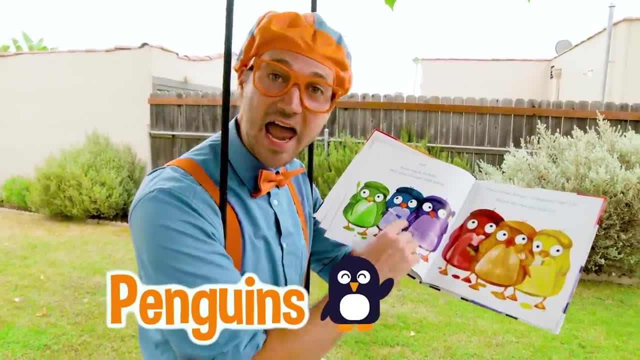 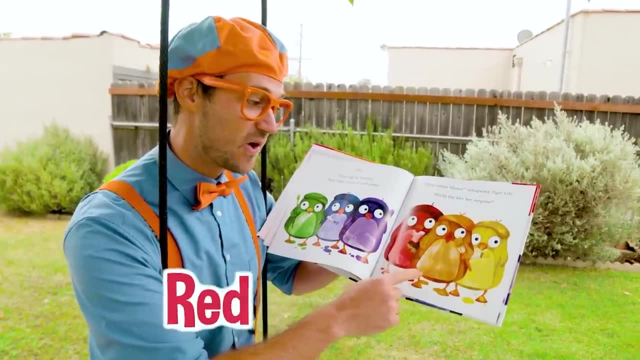 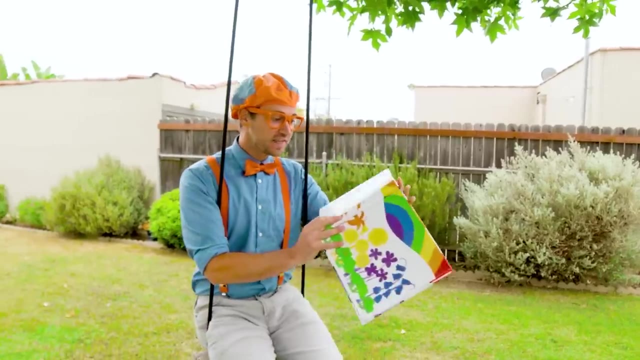 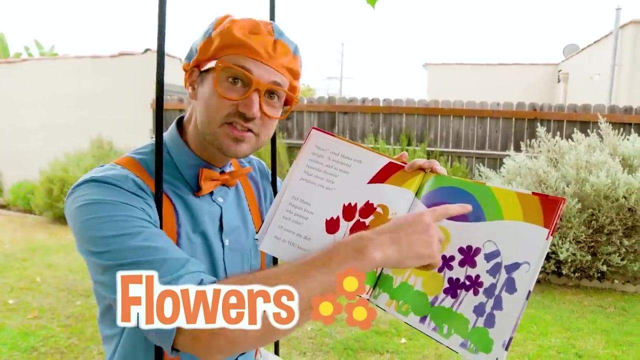 It's about all these penguins that have a different favorite color: green, blue, violet, red, orange and yellow. I love this book. Oh, Check this page out. Yeah, it looks like a garden. There's so many flowers and so many colors, Whoa, even a rainbow, Hey. 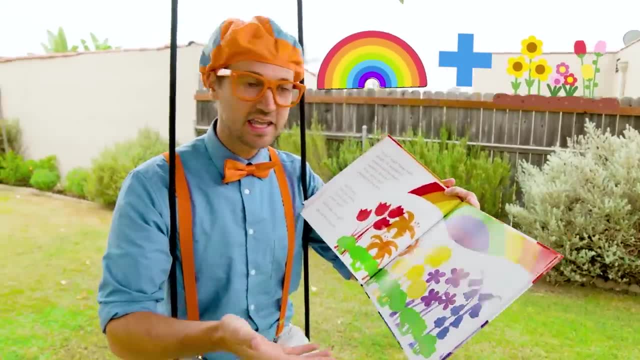 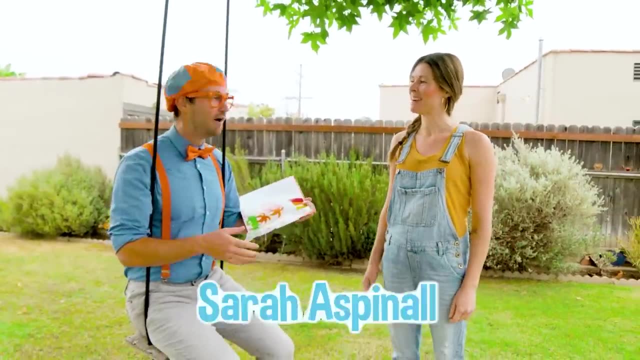 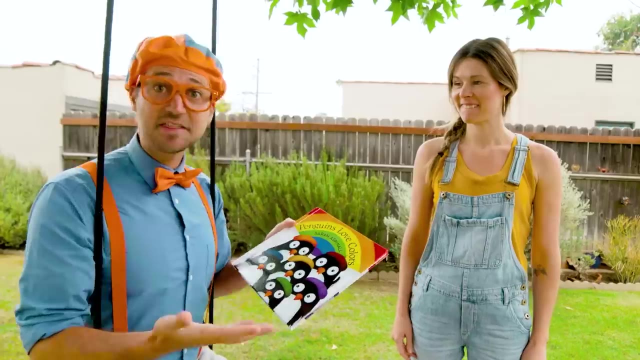 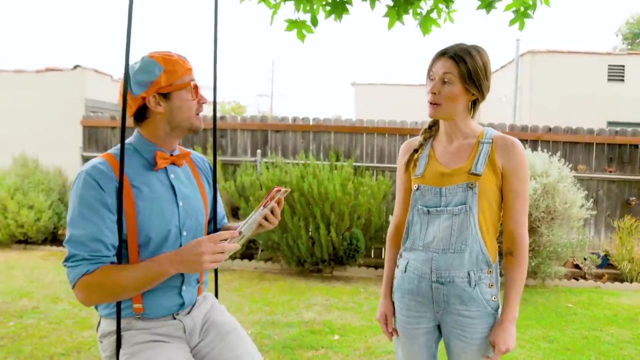 rainbow plus garden equals rainbow garden. Oh Hey, who are you? I'm Sarah Aspinall. Sarah Aspinall, Wait a second. Like the author and the illustrator of this book, That's me. Whoa, that is so cool. Would you like to make a rainbow garden of your very own? 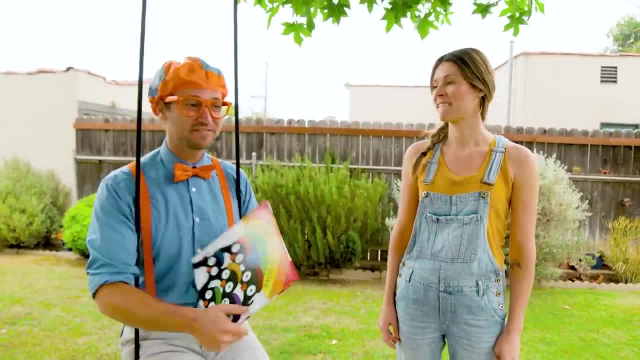 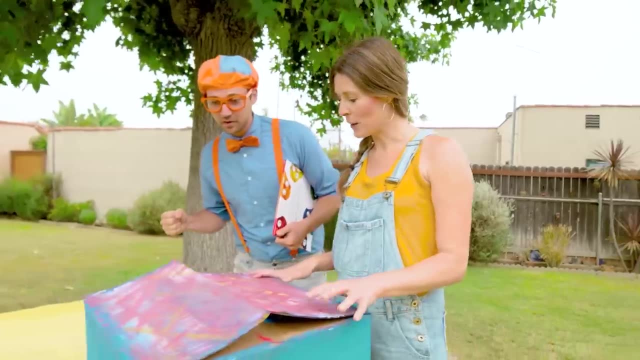 Blippi. yeah, I think that would be so much fun. Well, come this way, I've got all of the things you need. Oh, all right, Here is a box full of lots of fun art surprises for you to have your very own. 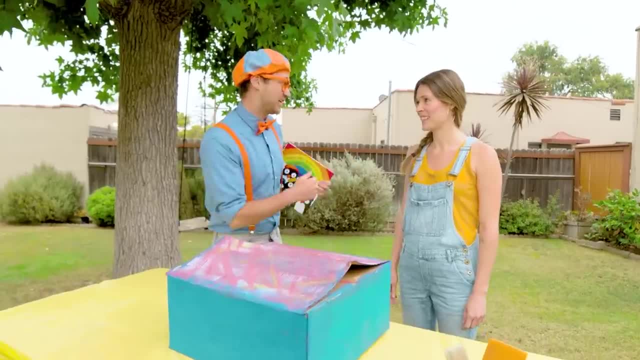 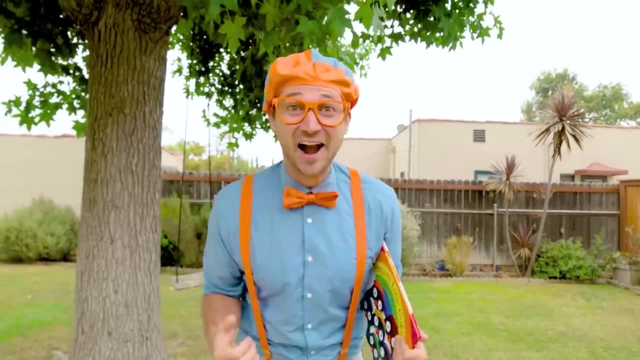 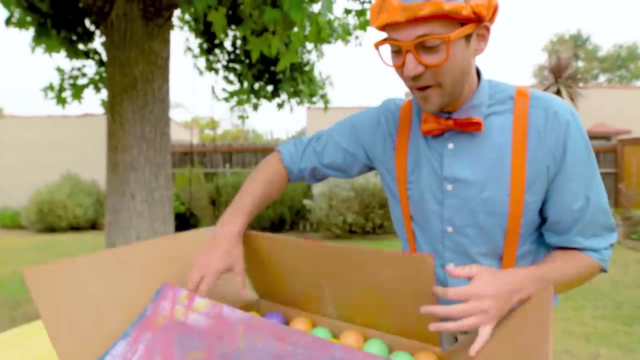 Wow. well, thank you so much, and we are very excited to make our very own rainbow garden. Have so much fun. Blippi, All right. See you later. Are you excited? Yeah, I sure am. Let's do this. Wow, All right, let's find all the things that we need inside this box. 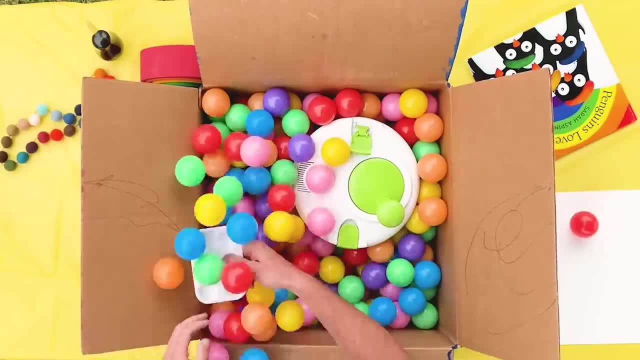 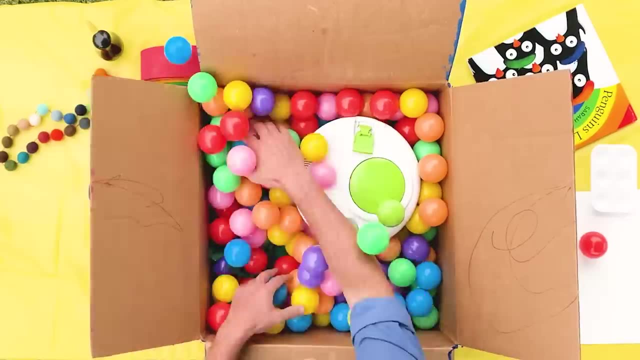 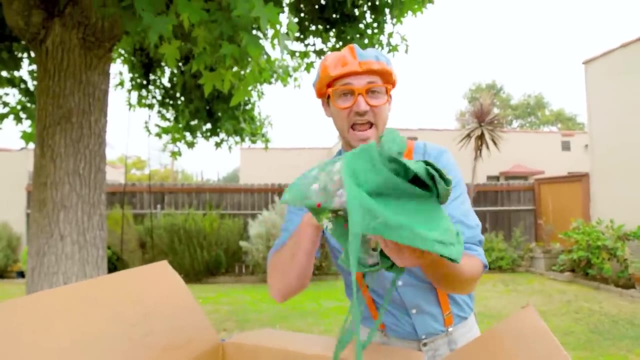 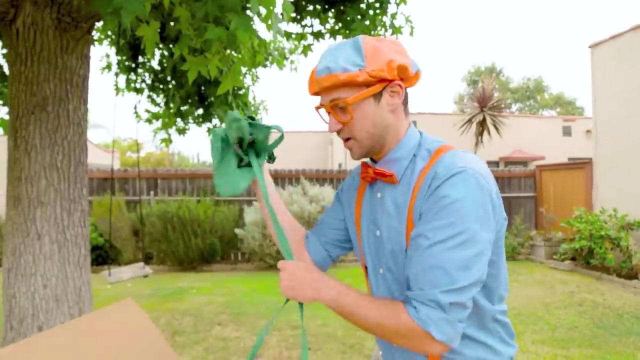 A green lamp. Here's one I actually love. haut Hier there. Wow, Look at this An apron. yeah, a green apron. It's really cute. Okay, A bolt of granite has right here over here, and we'll put that on before we start using all of the paints. 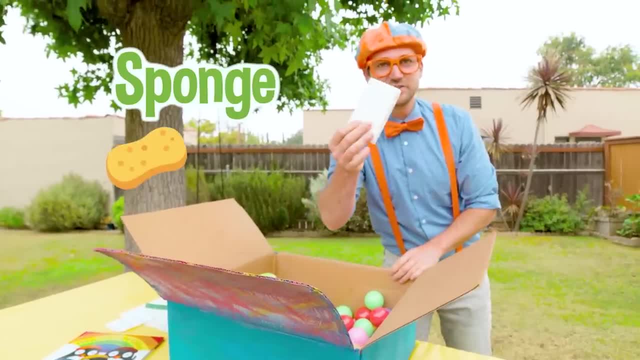 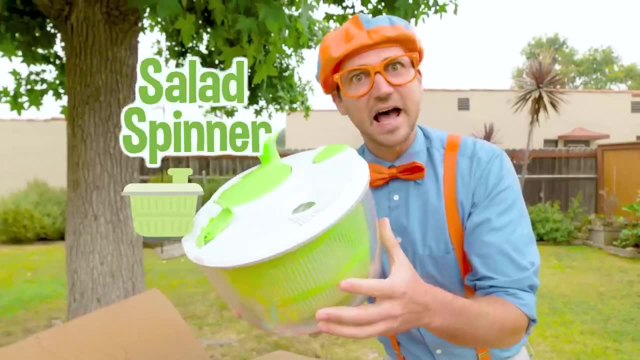 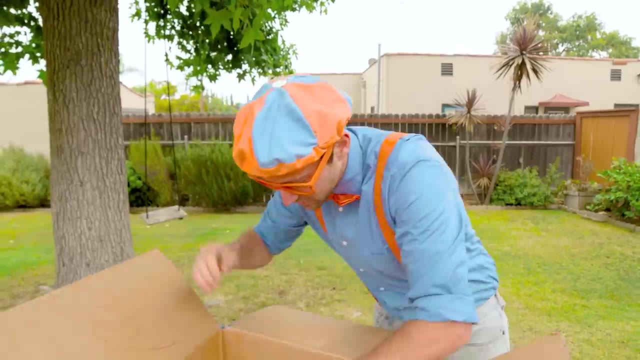 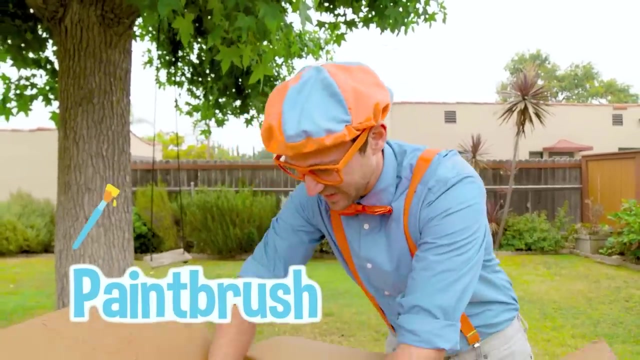 Whoa, hey, a sponge. Okay, put the sponge right there. Ooh, a salad spinner. Whoa, I know what this is used for. I'll show you really soon. Okay, and we have some scissors, a little paintbrush. 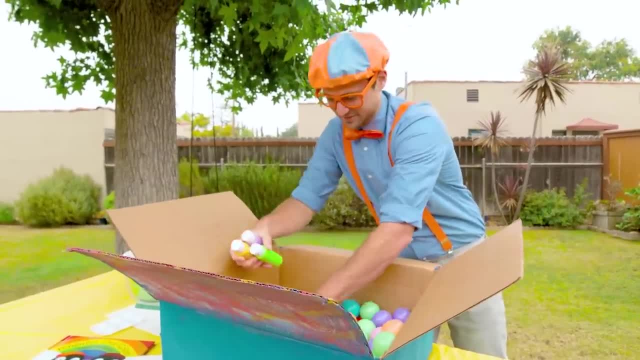 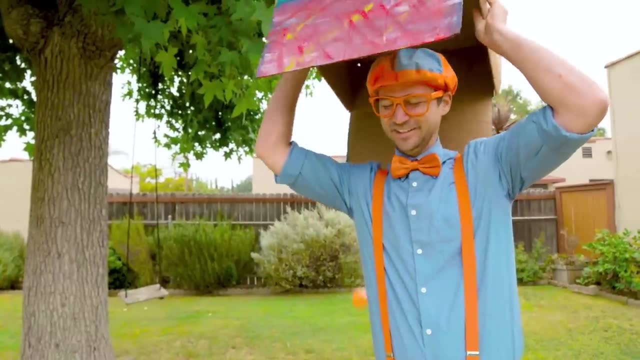 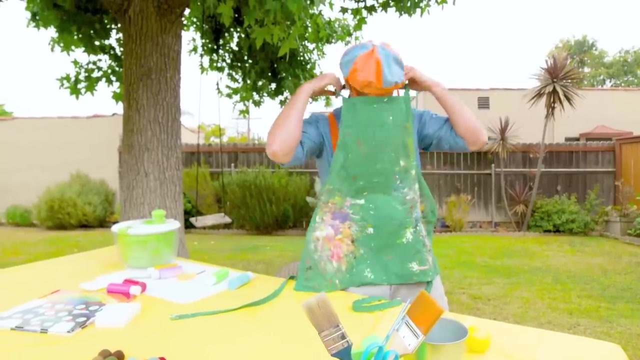 and, of course, a lot of paint. All right, I think that's all. Let's see. Yep, that's all. Okay, let's put on this apron. so then I don't get dirty. All right, here we go. 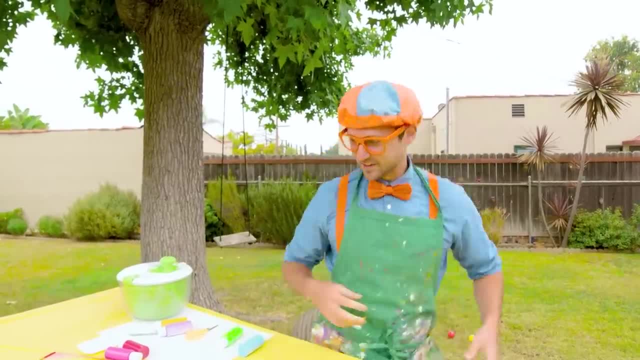 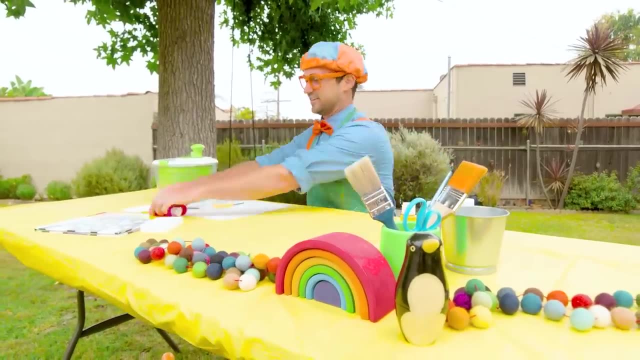 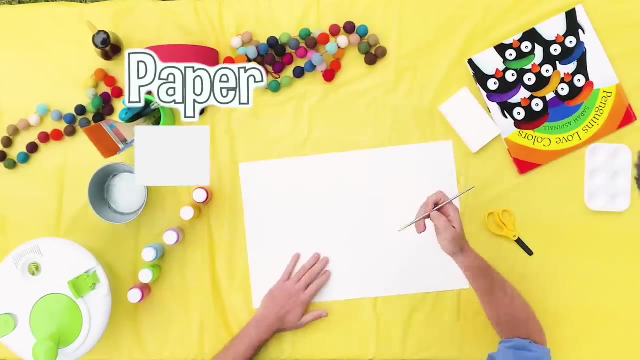 Tie it nice and tight. Perfect, there we go. All right, Okay, let's organize a little bit. Whee, All righty. Okay, so we have our paint over there, salad spinner right there, big piece of white paper. 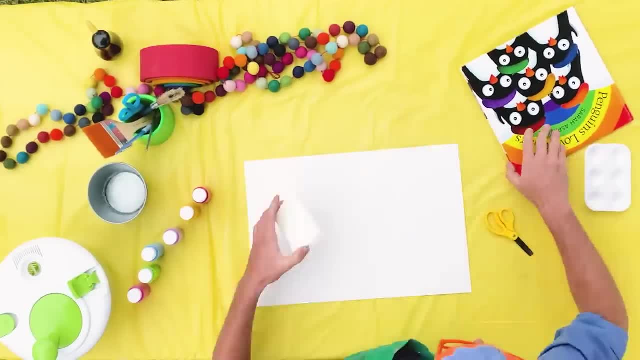 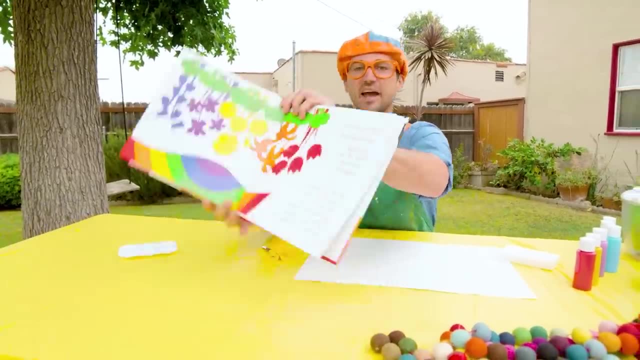 little teeny paintbrush. Put that in there. Can't forget about the book. so then we can reference what we're making. How about that? Yeah, perfect. Yeah, remember, we're making this picture- A rainbow garden, All right. 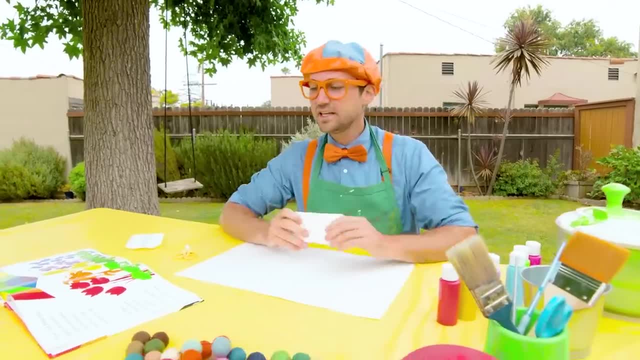 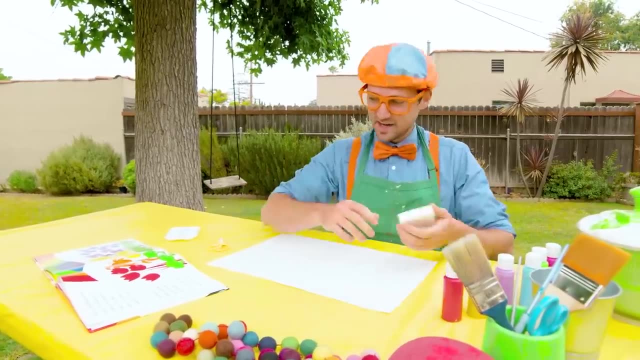 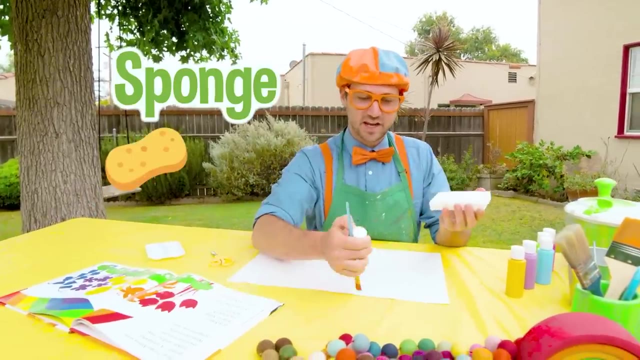 All right. So first we need to make a big piece of paper of rainbow colors. So let's take a little bit of red and a paintbrush and we're gonna put it on the sponge, okay, So let's actually just squirt it right here. 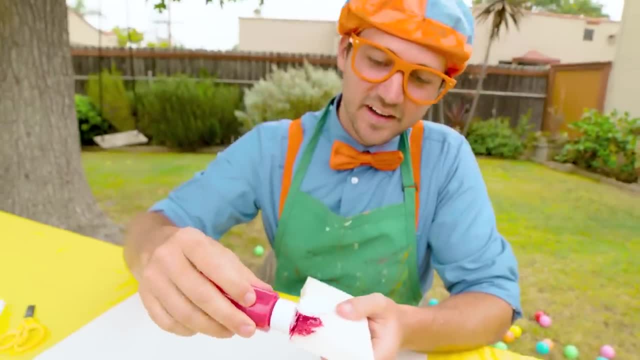 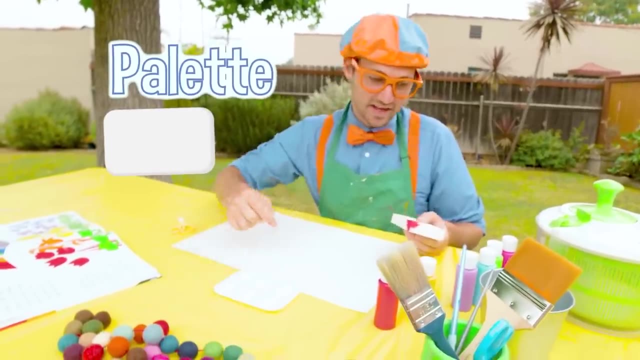 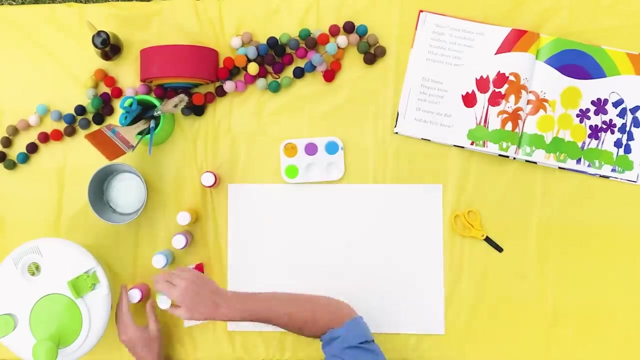 Okay, and now that we have a lot of red right there, we need to do all the other colors. But I actually have an idea. I think I should use this palette and fill it up. Might make it a lot easier, Perfect. 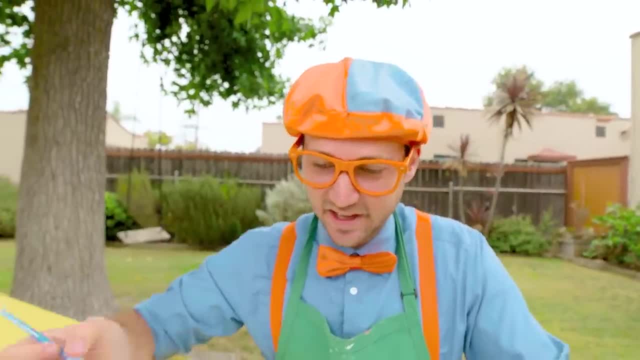 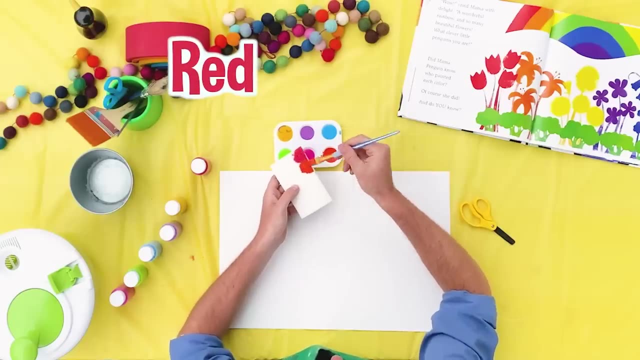 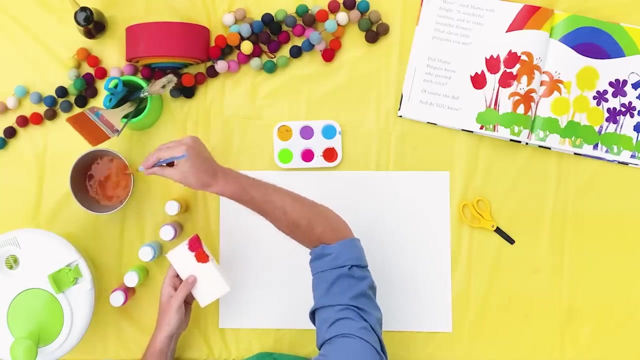 Okay, now let's take the paintbrush, All right, and let's put some orange right here. Yeah, so now we have red and then orange. We need to wash off our brush, Ha ha, Perfect, And we need some yellow right here. 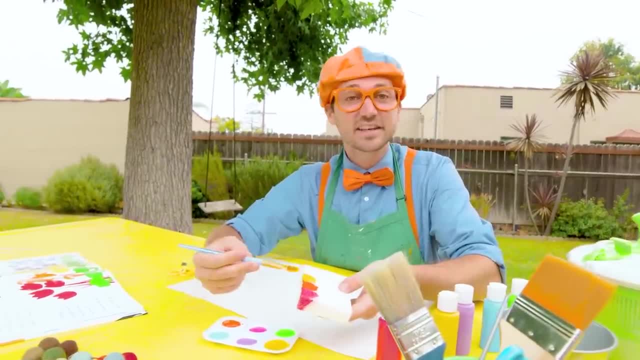 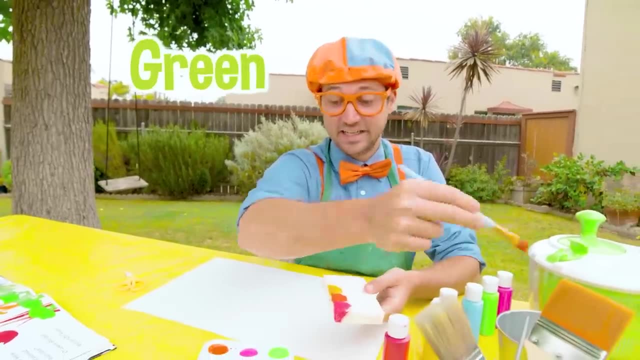 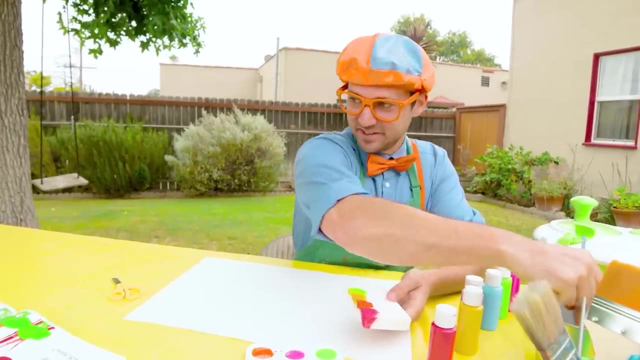 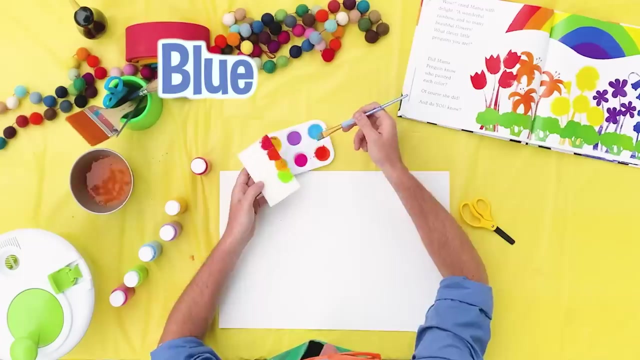 Wow, Yellow is so pretty. It's like the color of the sun. Okay, lots of yellow right there. Now we need some green. Okay, Whoa Green. Perfect. After green, we need some blue. Yeah, perfect. 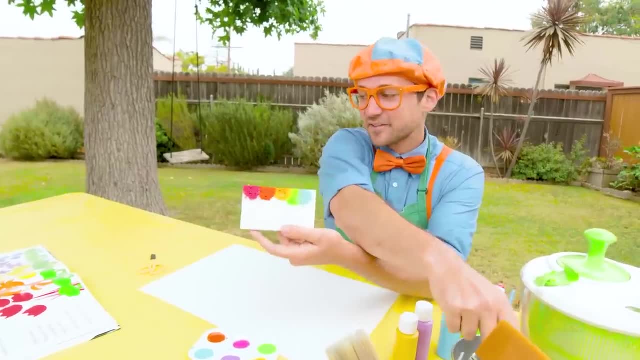 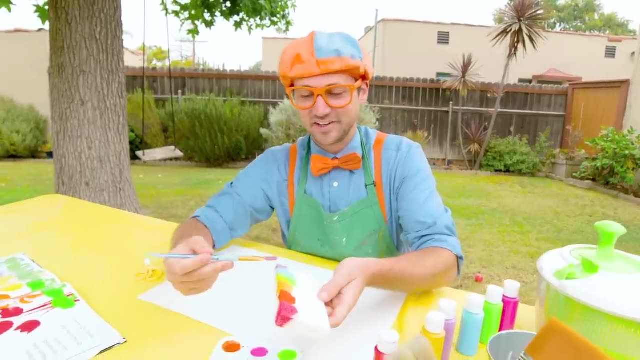 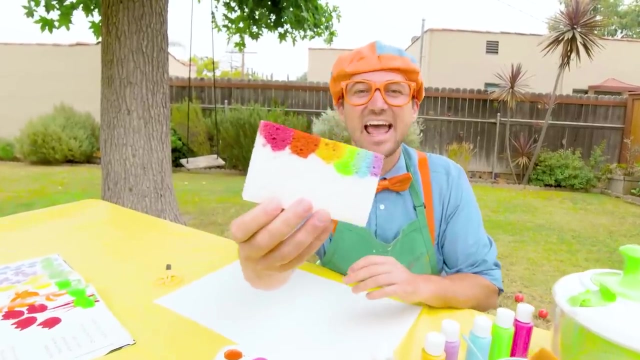 Good amount of blue right there. Do you see this? We're almost done And now we need some violet or purple. They're very similar in looks. Wow, There we go. How does that look? Ha ha, yeah, like a rainbow. 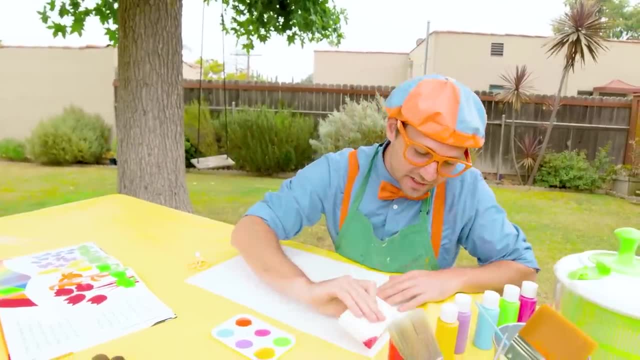 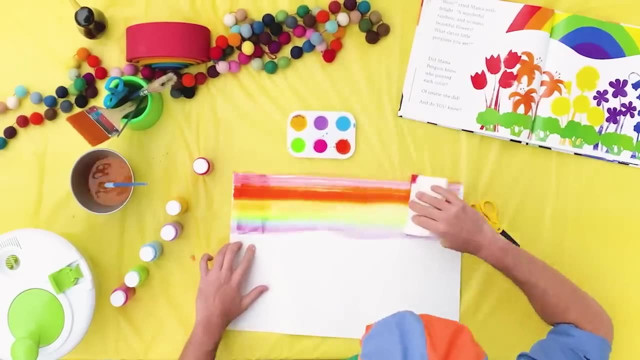 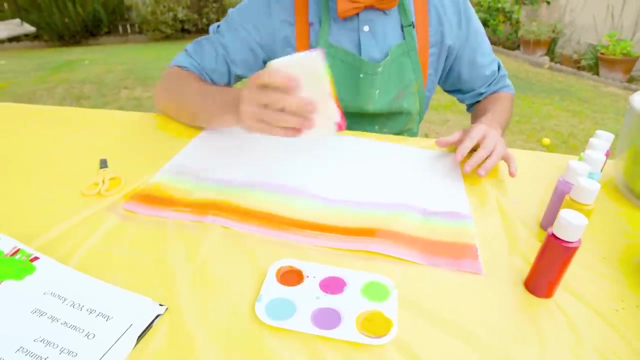 All right, now for the fun part. Push it down right here. Yeah, Whoa, Whoa, Look at that, Wow, Yeah, And you do that same thing many times in a row, all the way down. So I'll do that now. 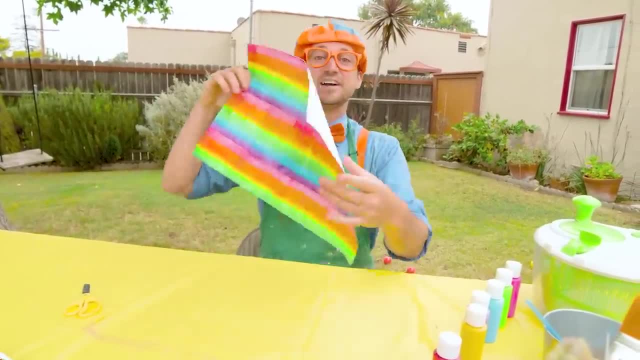 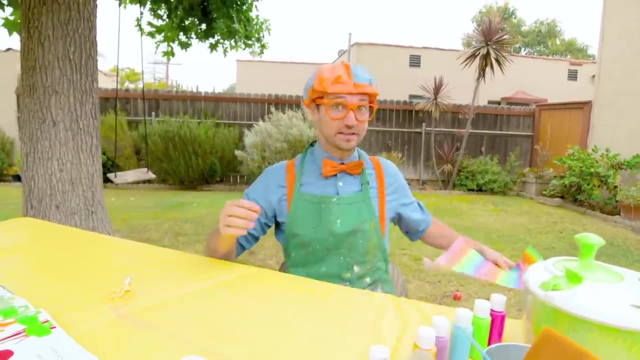 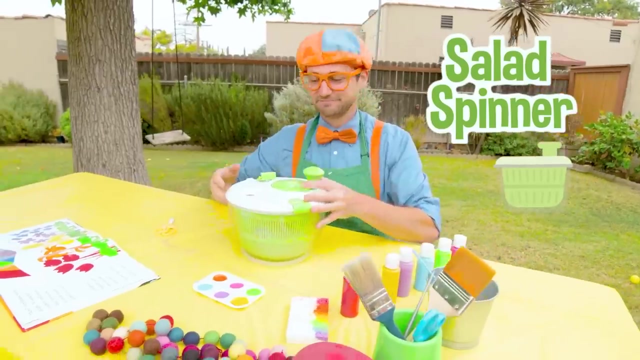 Whoa, That is so beautiful. Check it out, Whoa. Okay, I'm actually gonna set this over to the side so it can dry. It's a little wet still, Perfect, Okay. Now what we need to do is take this salad spinner. 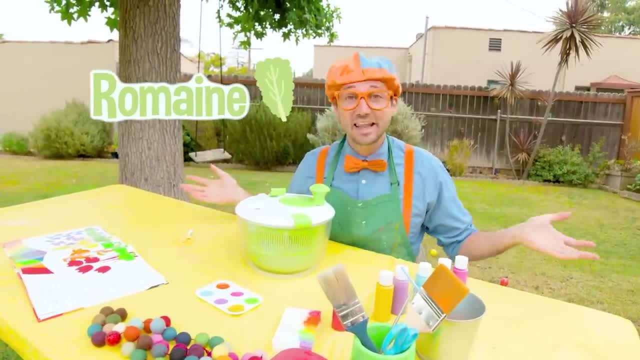 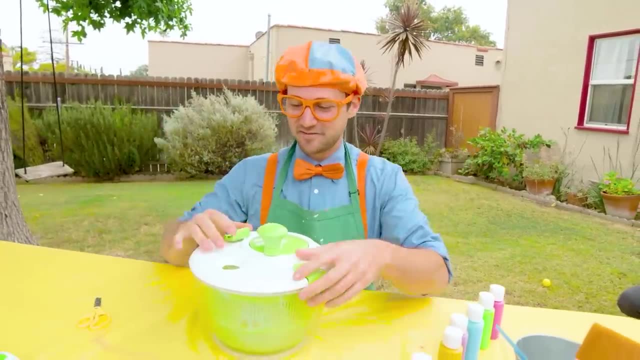 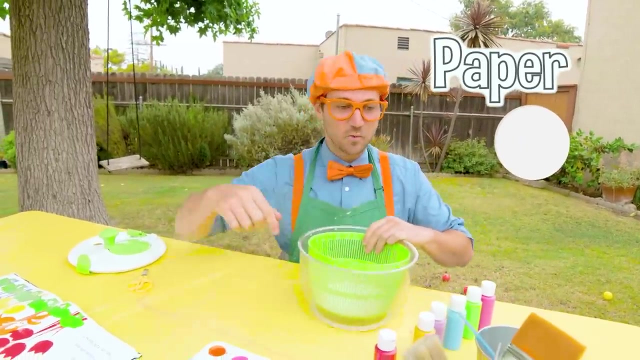 Yeah, You normally put salad, kale, romaine lettuce inside here and you spin it around and it flings all the water off of it. But today what we're gonna do is we have a white piece of paper right there and we get to put some colors in here. 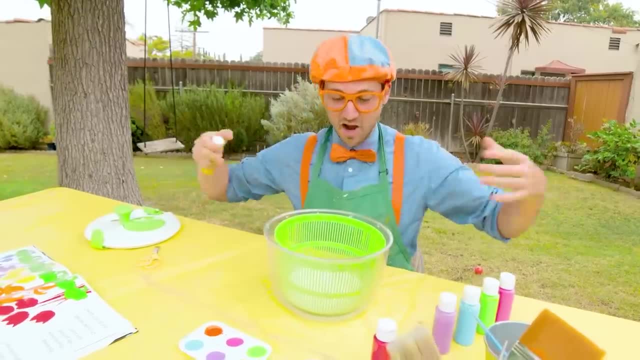 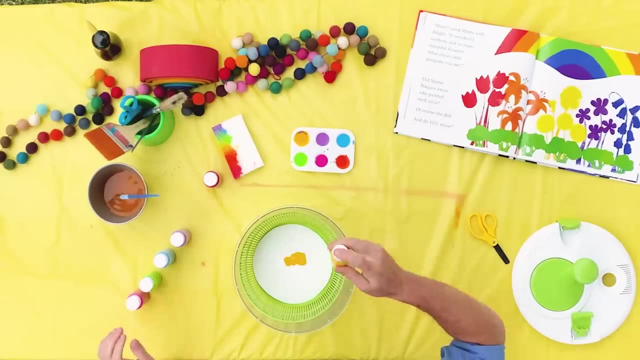 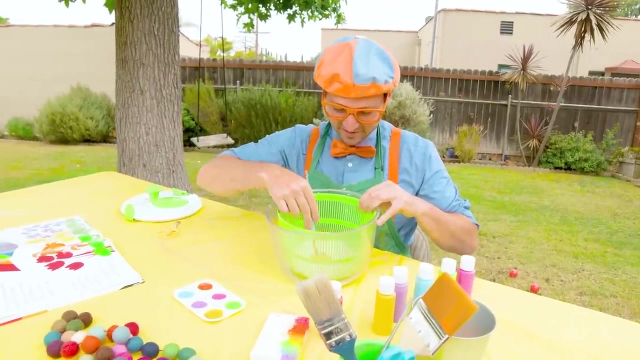 and then spin it and then it pushes all the paint off to the edges. Okay, Ready, We'll put some yellow. Yeah, That looks really good. And then, how about we put some orange? I love orange. Yeah, Just like that. 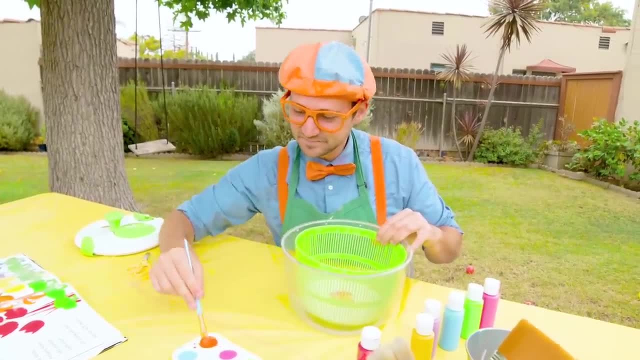 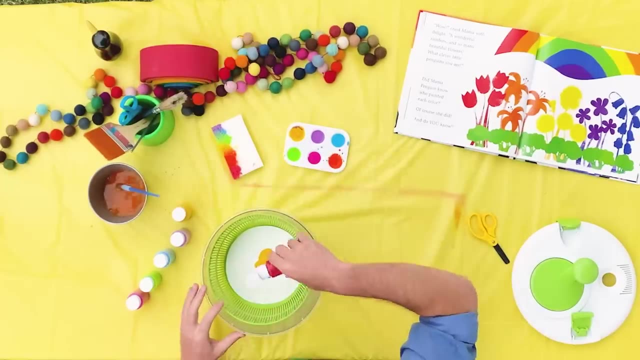 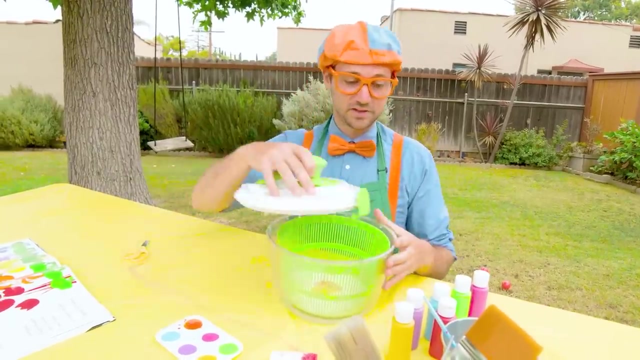 Wow, Yellow and orange. And how about a few drops of red? Yeah, How about that? Just a couple? There we go. Perfect, All right, Now let's put the top on. It's all sealed, Here we go. 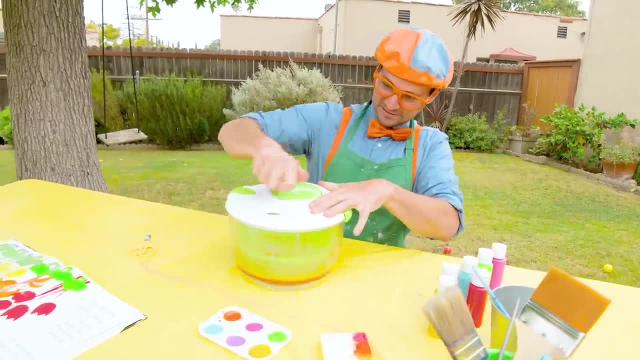 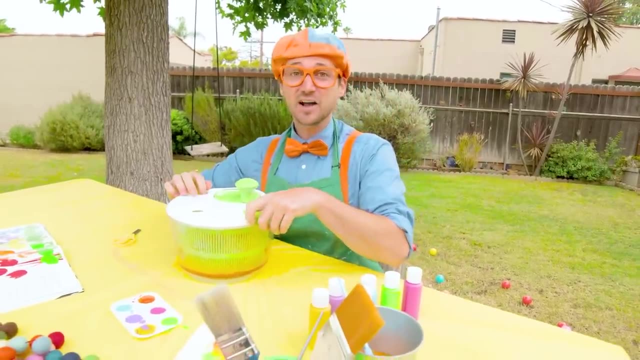 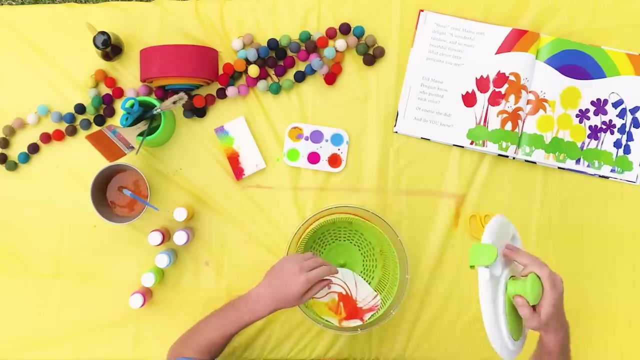 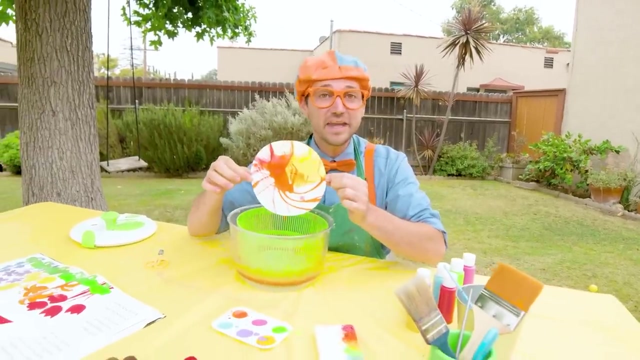 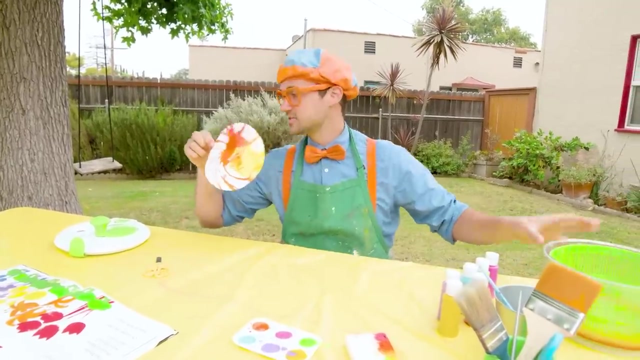 Wow, That was awesome. I just spun it so fast. Let's open it up and see what we have inside. Wow, That is awesome, Awesome. Wow, that is amazing. We just made that by spinning this around really quick. Okay, it's pretty wet, so let me put it off to the side. 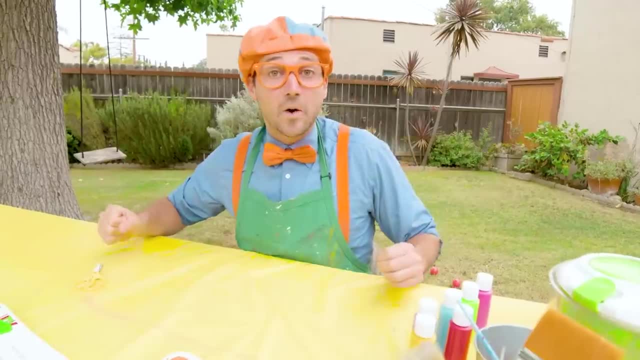 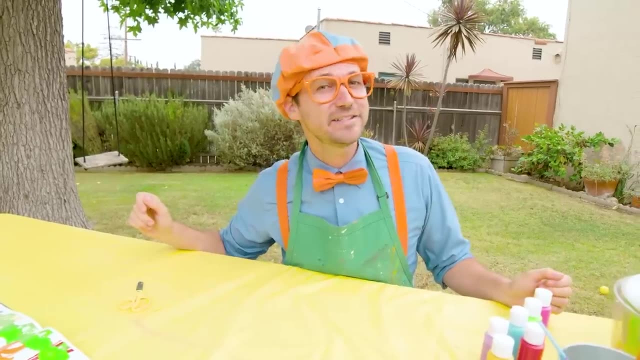 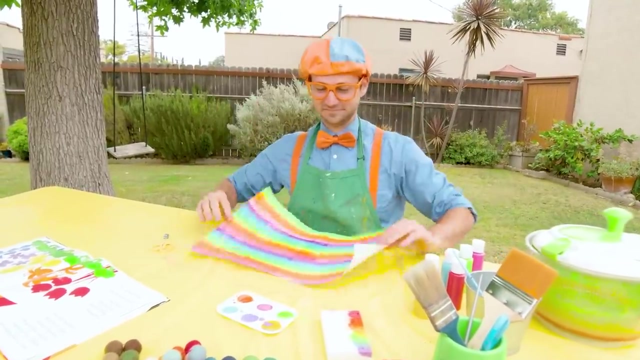 so then it can dry. Okay, now that I put that off to the side to dry, the original rainbow is probably ready to use, So let me get it. Yep, it's nice and dry. All right, so now what we need to do. 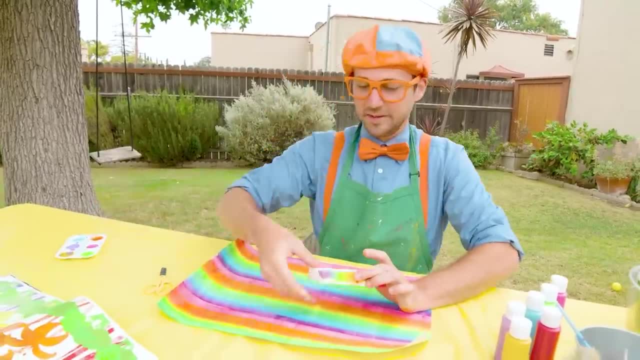 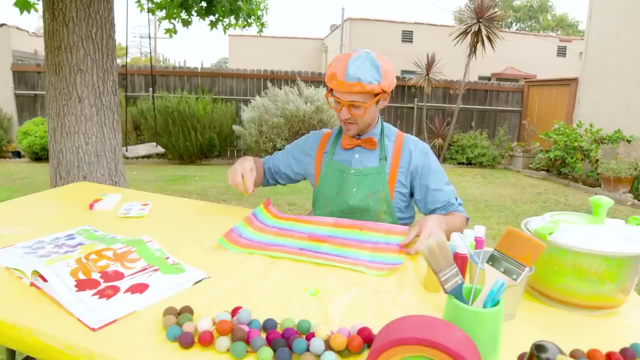 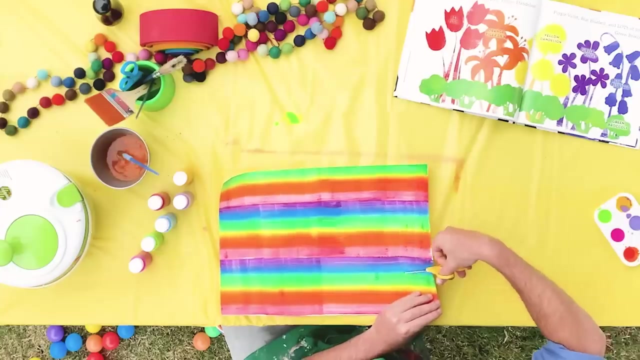 let me organize this paint. I don't want it to get all over me now that we're all done painting. So what we're actually gonna do is take this and make a little squiggly line while we cut Ready. Yeah, just like this. 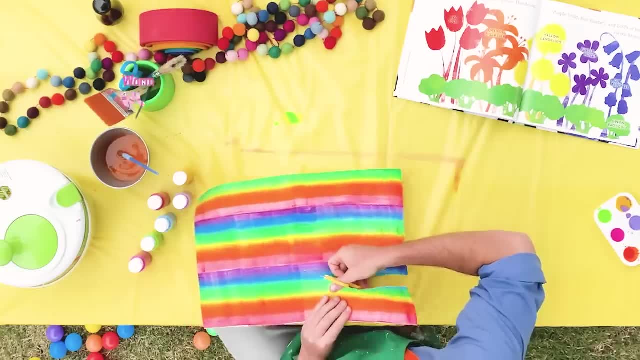 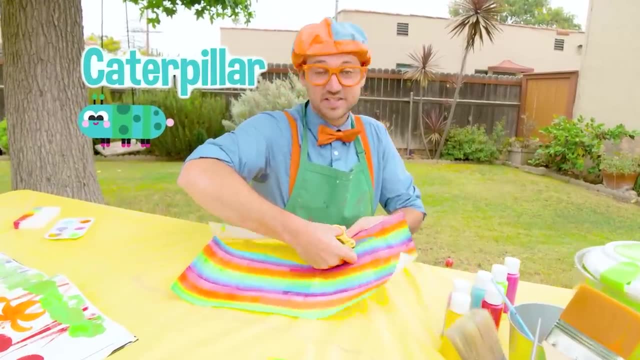 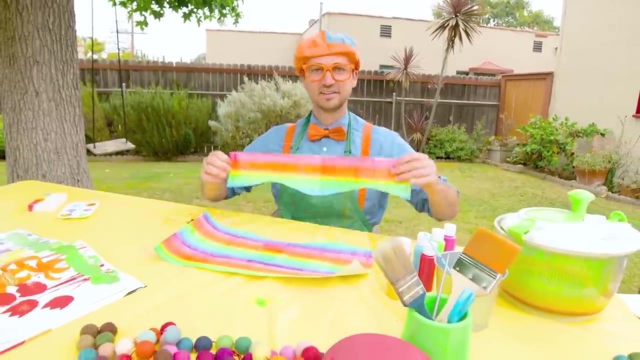 Oh, kind of like a worm- Worms squiggle around- Or a caterpillar or a snake. See this? Yeah, check that out. Okay, now what I need is a white piece of paper. I have one right on the ground over here. 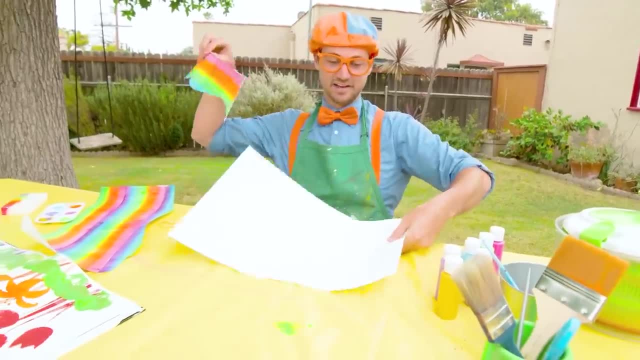 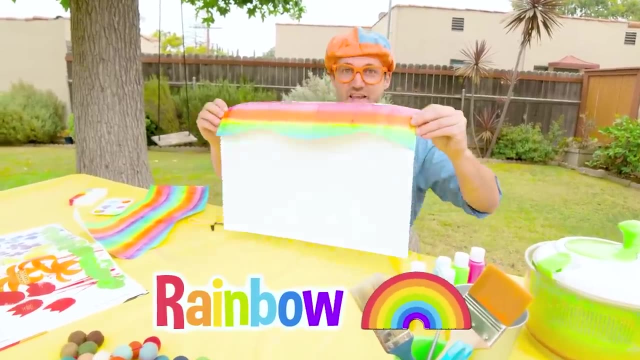 and then I put it on the top. Do you see that It's a white piece of paper? Do you see that? Yeah, it's like a rainbow, Just like in Sarah's picture. So let me get some glue right over here. 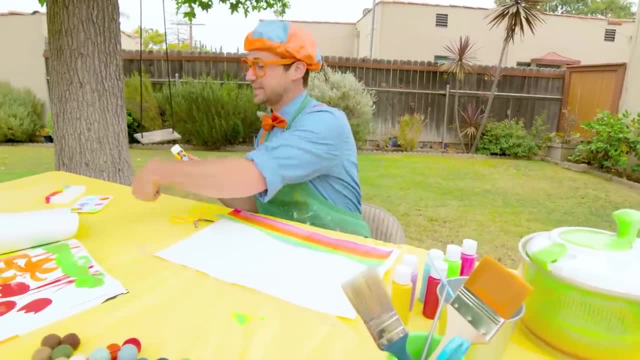 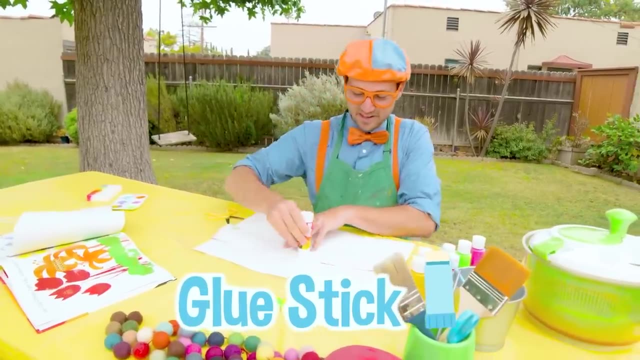 All right, now that I have this glue, I can glue it down. All right. Have you ever used a glue stick before? It's kind of fun. Yeah, it's not all liquidy like the normal type of glue. This is a glue stick. 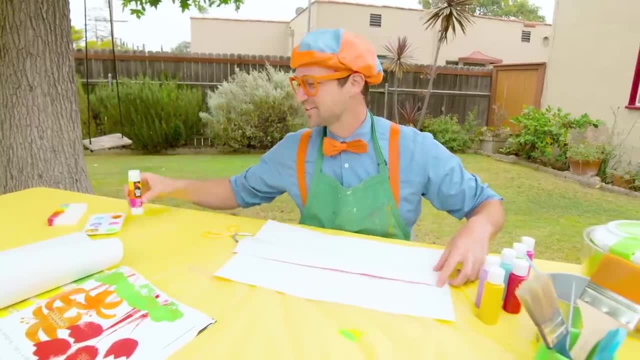 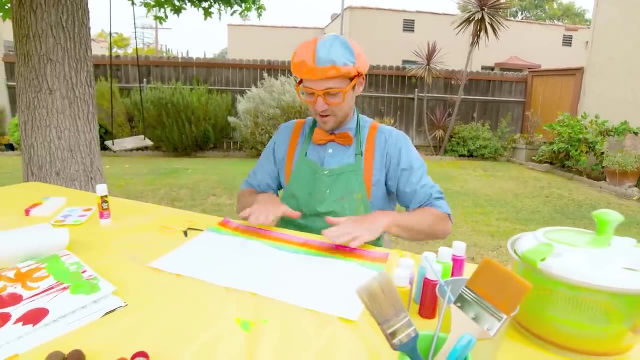 You just kind of like color it on, But it's no color. You know, like as if you're coloring. Yeah, there's no color to it. It's clear, Perfect, Wow, This looks amazing. You and I are doing a really good job. 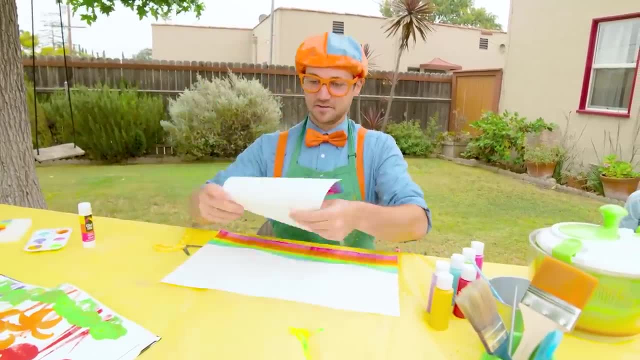 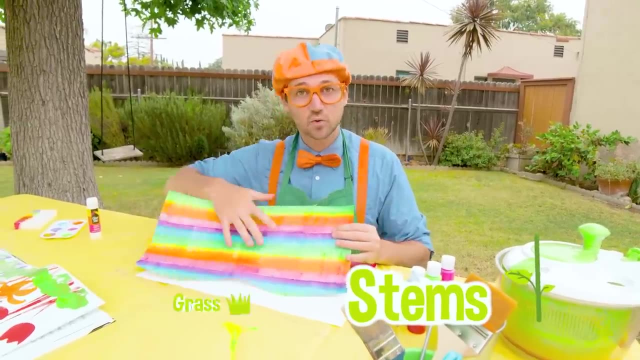 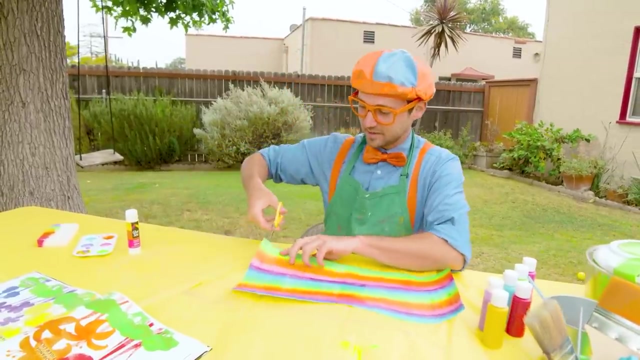 All right. Next step is to take this- Remember The rainbow- And cut out some stems and grass from the other side. I'm gonna set this down right over here, So then I can start cutting. Okay, Let's cut a nice long stem. 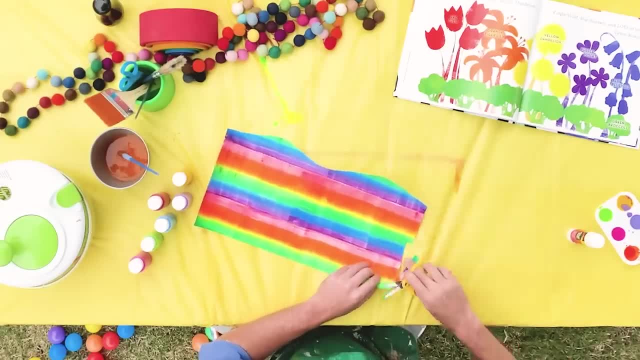 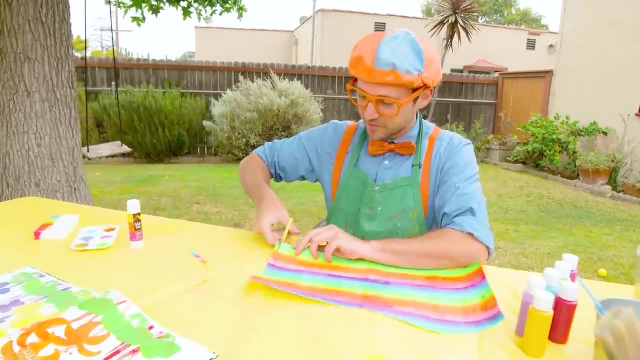 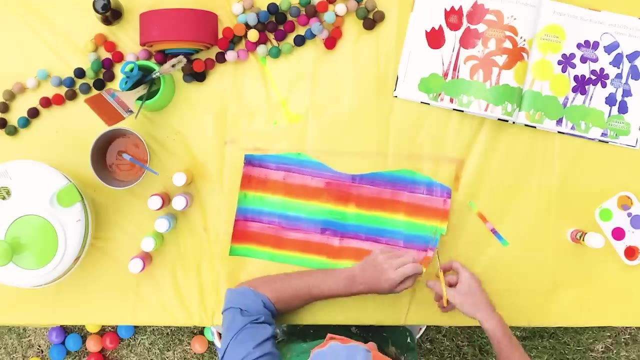 Yeah, just like that. It's like a really thin long rectangle. Perfect, Let me do another one. Yeah, I'll start with two. How about that? Yeah, Oh, whoa, There we go. We have two long rectangles. 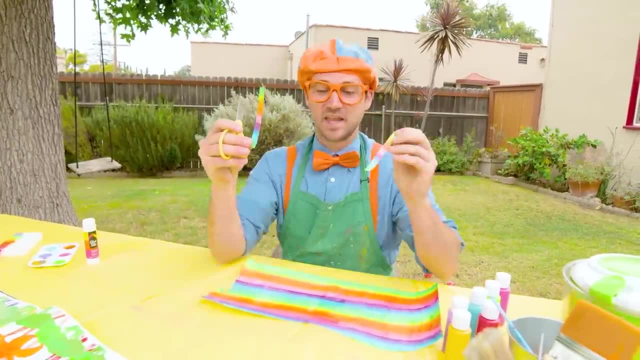 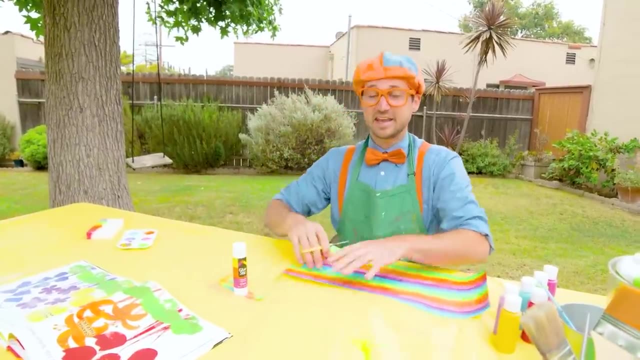 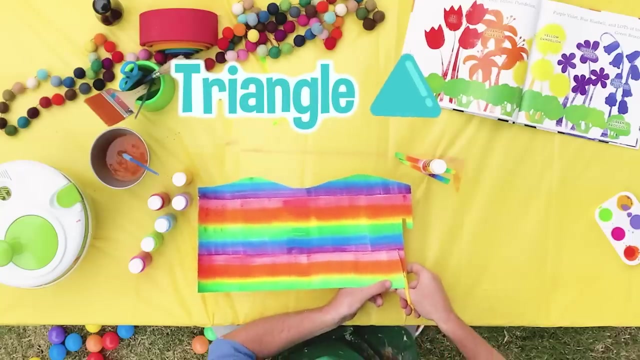 Yeah, One, two, And these are gonna be the flower stems. Okay, Put them right under there. Perfect, Now we need some blades of grass, So what we're gonna do is some triangles, Just like that, Some nice tall blades of grass. 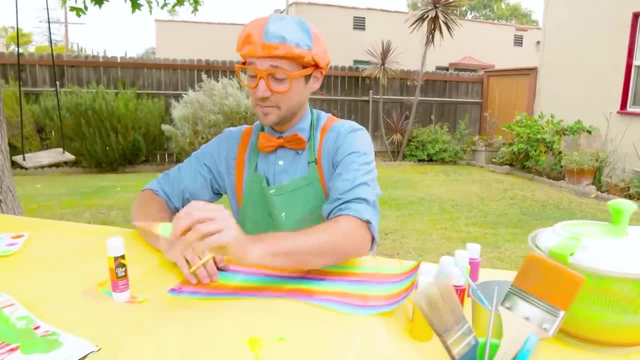 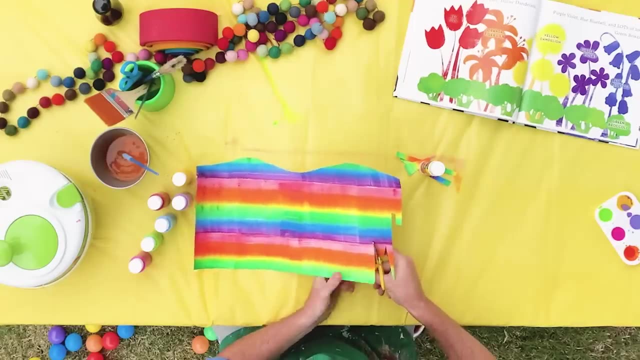 As if you might need to mow your lawn. Yeah, And these blades of grass I'm cutting. they're gonna be long. Yeah, Triangles, Just like I said. Whoa, How does that look? Do you like that blade of grass? 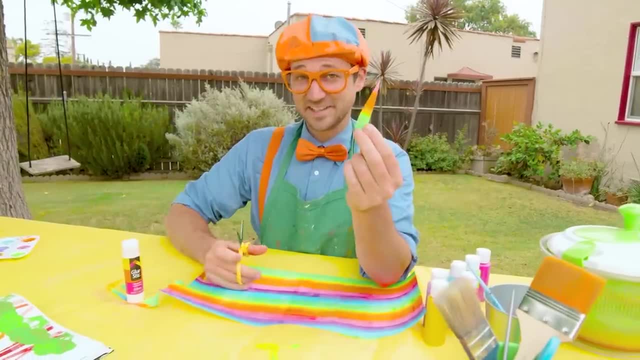 I sure do. All right, Put those right here. I'm gonna set this aside And grab my piece of art that had the rainbow on the top, And then here we go, I'm gonna be able to put these on the bottom. 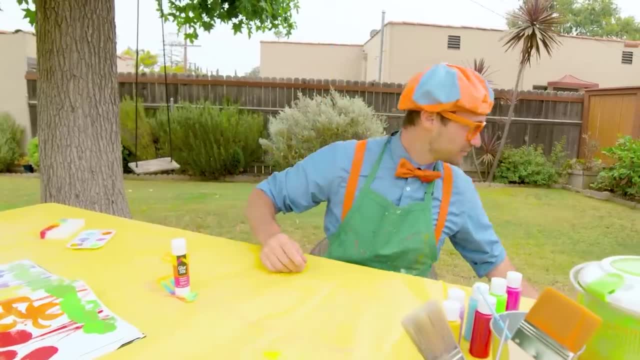 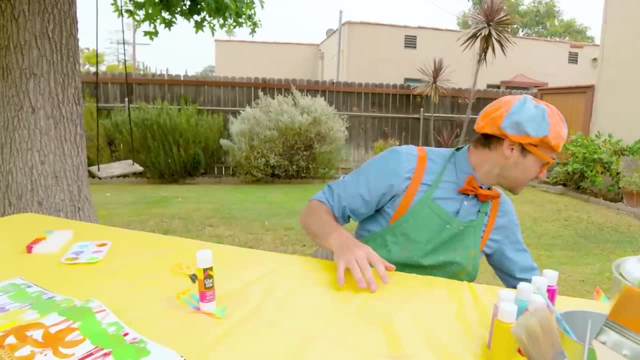 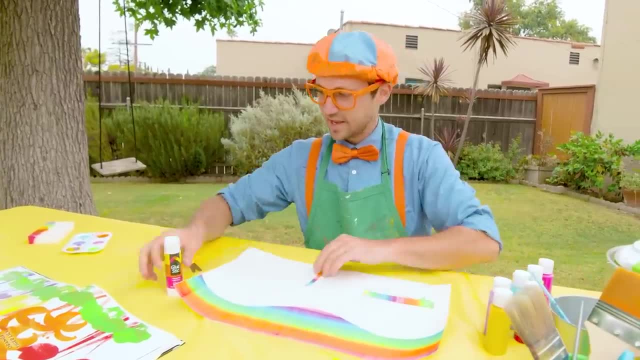 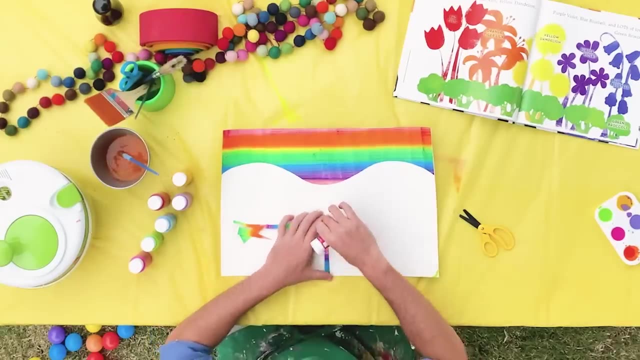 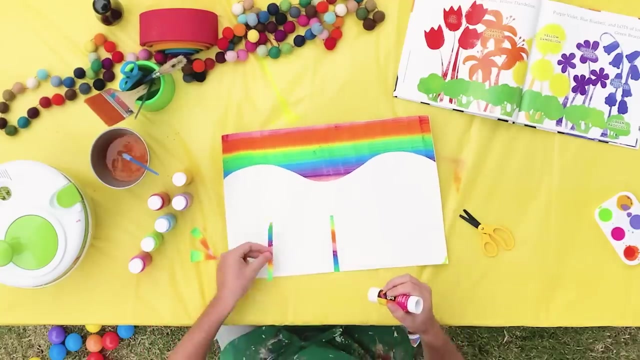 All right, I got some more, But let me flip this around and take my glue stick again. Whoa, Get one right in the center. How about one to the side a little bit? huh Yeah, There we go. I love doing art. 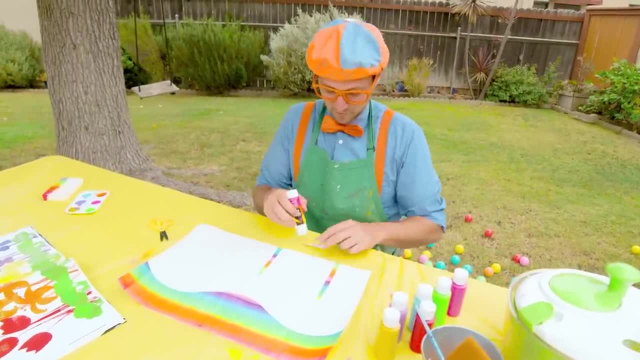 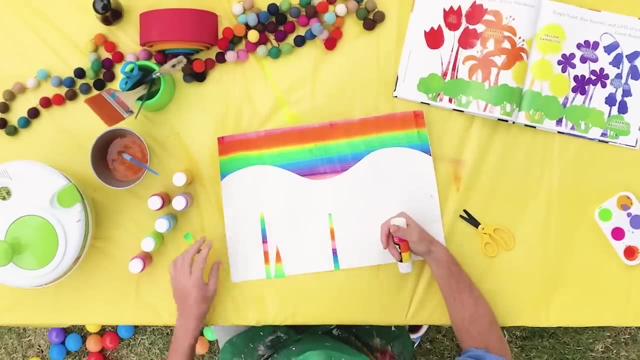 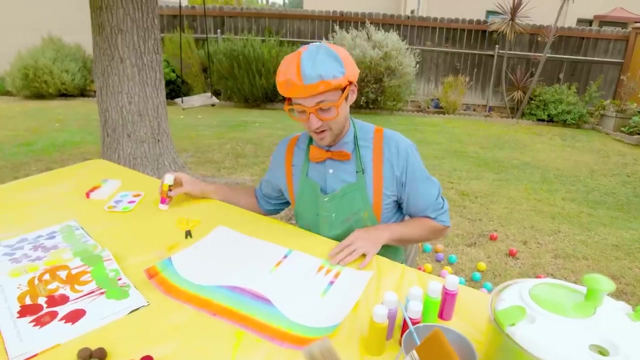 Yeah, How does that look? Yeah, and we'll do the blades of grass too. It's so colorful. Wow, Look at that. Oh, here we go, All right. okay, All right. looks like I need to cut some more. 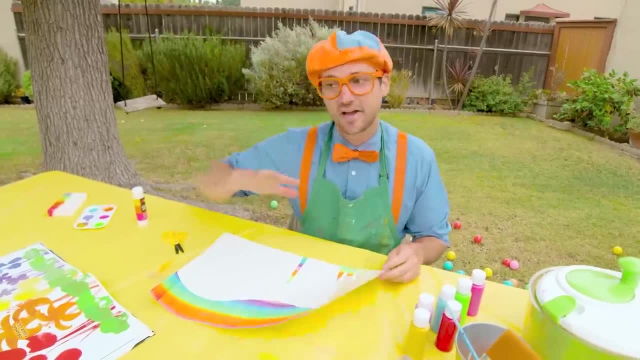 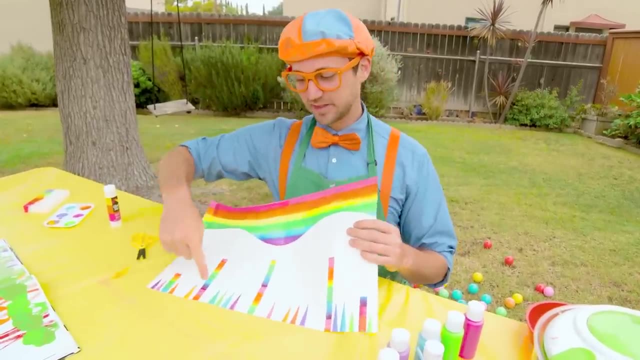 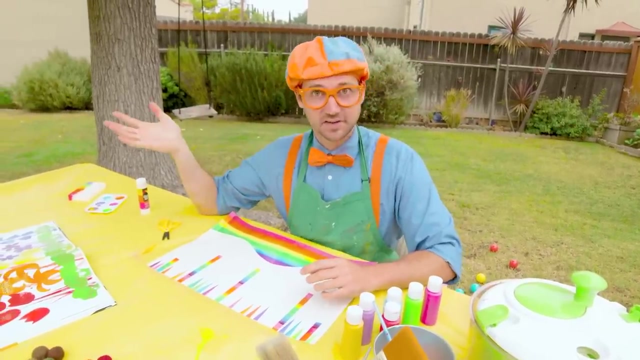 and then glue it all down. So let me grab the piece of paper and I'll cut a bunch. all right, Whoa, check it out. All right, I did all the blades of grass and all of the flower stems. Now we need to do the tops of the flowers. 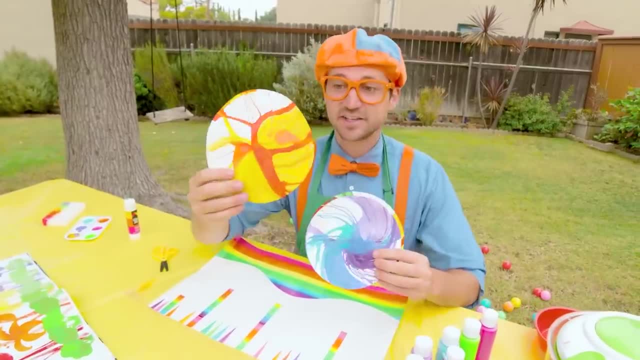 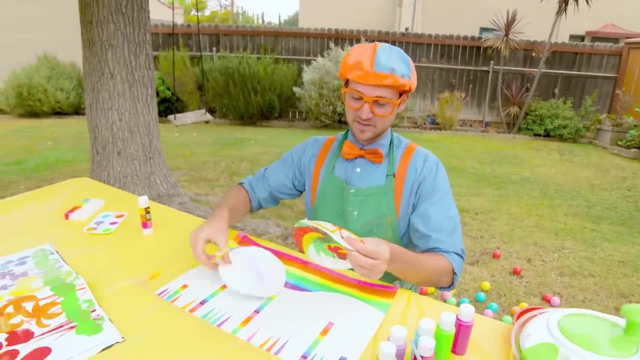 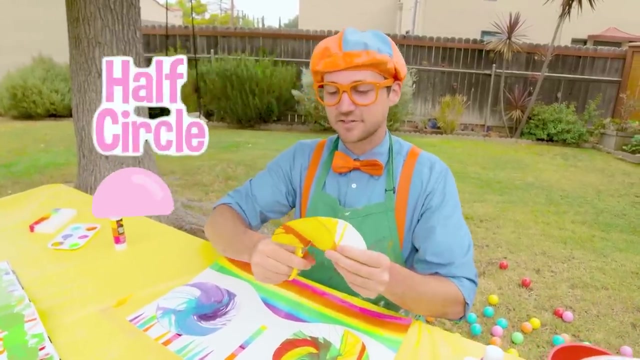 So remember earlier we did the salad spinners. Yeah, look at all these other ones that I have. Okay, so let's cut them up, So then we can use them for the flower petals. Let's do a half circle. 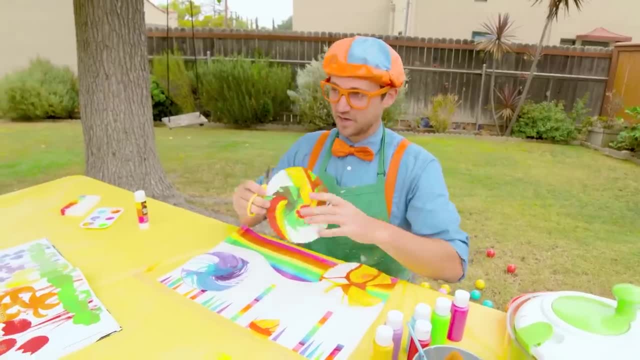 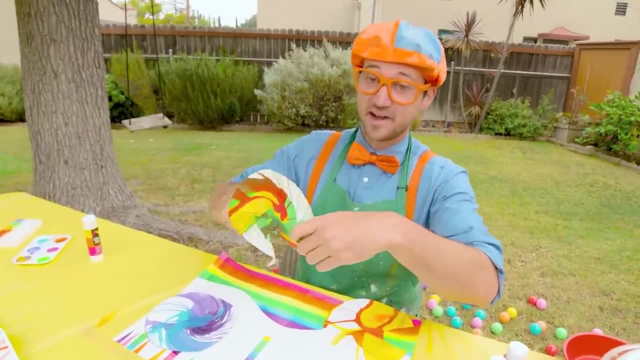 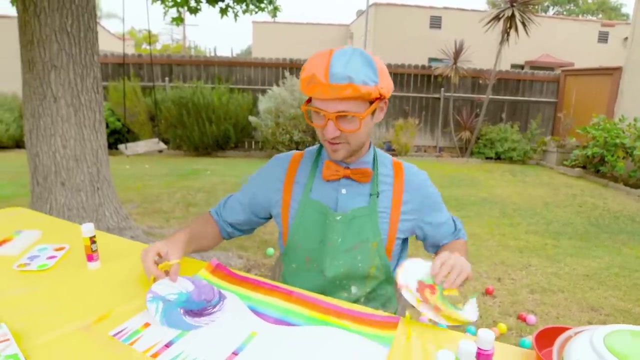 Yeah, like that. how about that? And then we can also do, yeah, something really big, because this one is gonna be a very big flower. yeah, Perfect, how's that look? All right, and then we need some leaves on this one. 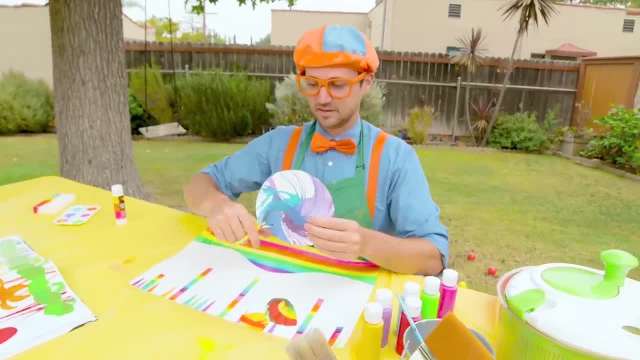 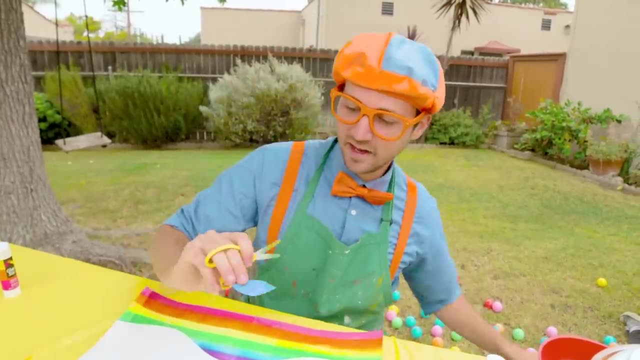 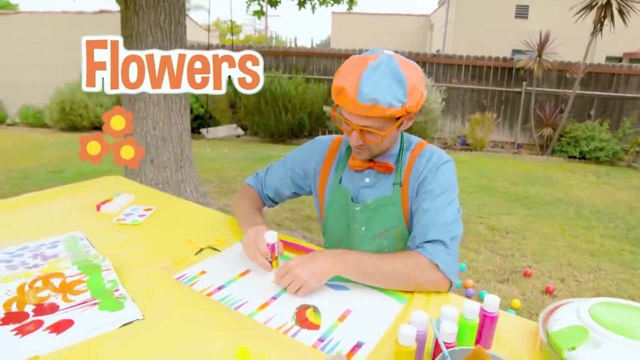 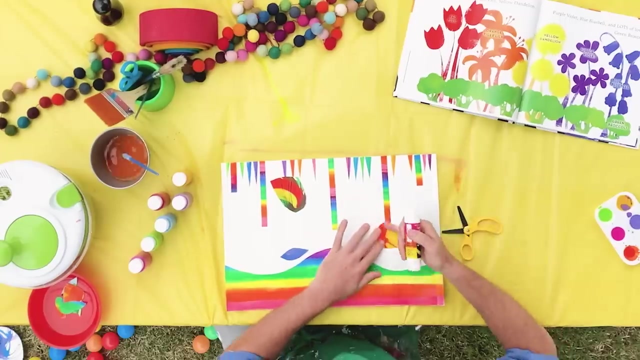 So let's go like this: yeah and perfect. Yeah, just like that, and then we can start gluing them down and making our flowers. So let's go like this: How does this look? Yeah, that's a beautiful flower. 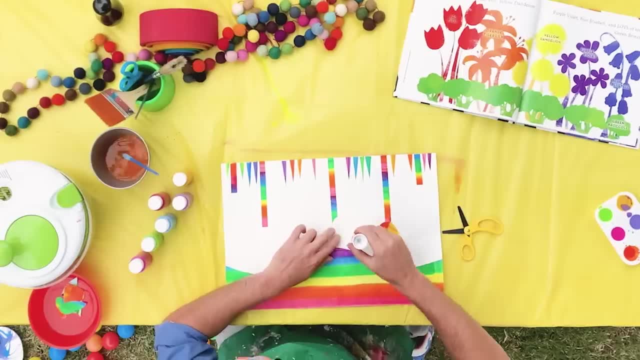 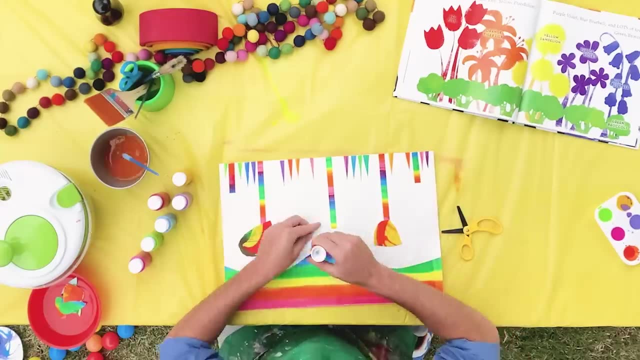 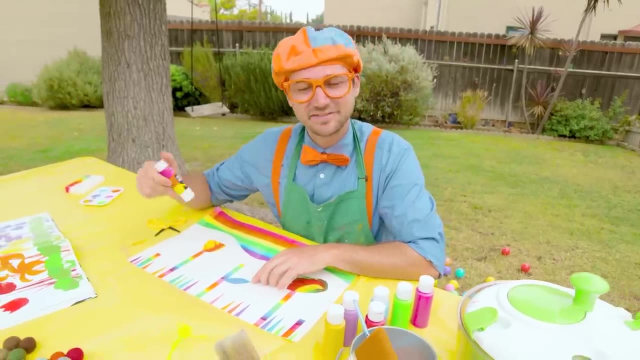 I love the smell of flowers. Then this one will be another flower. Yeah, and a stem. Okay, let's do a. actually not a stem, a leaf. We already have a leaf. We already have the stems right there. 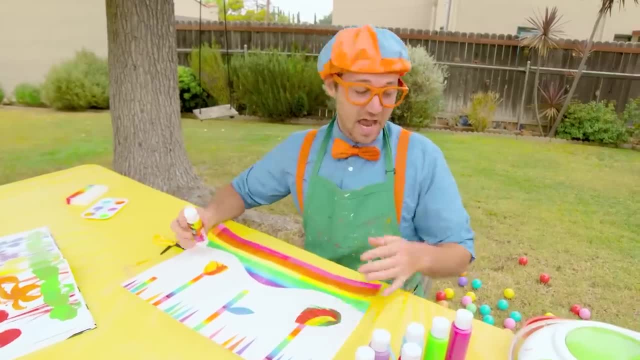 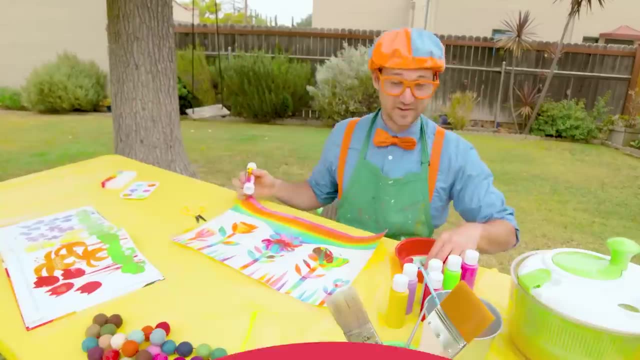 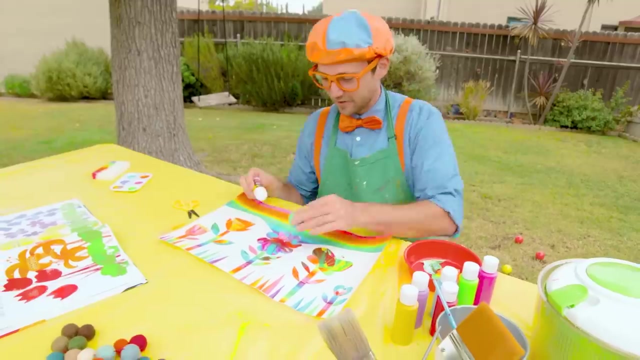 So a leaf right there, right in the center. Okay, I'm gonna cut some more and continue to glue them down. Here I go. All right, last but not least, let's put the center of the flower. Yeah, that's like where all the pollen is. 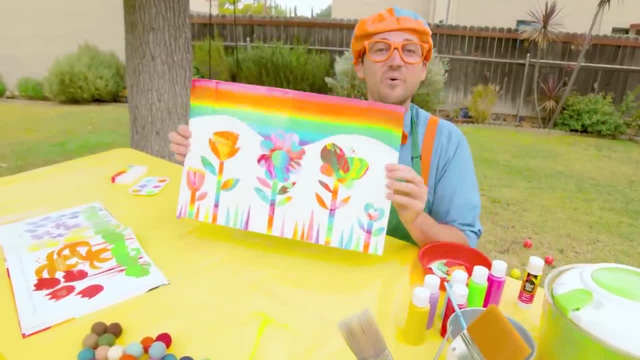 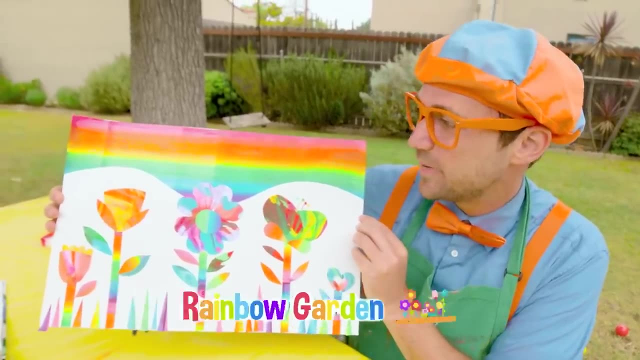 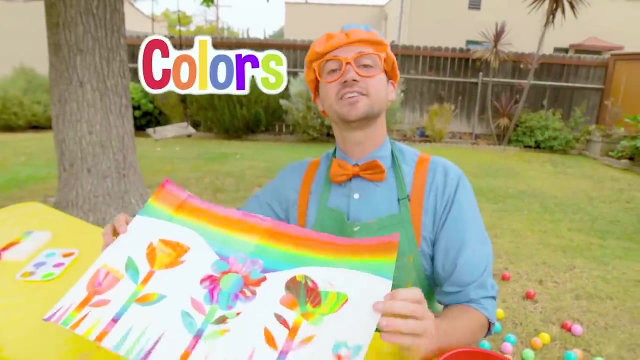 All right, how does that look? Wow, It looks like it's gonna look like a rainbow garden. Wow, what a beautiful picture. Whoa Well, thank you so much for learning about all the colors of the rainbow today with me. 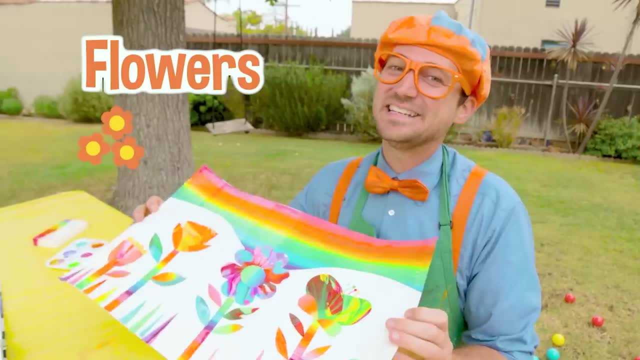 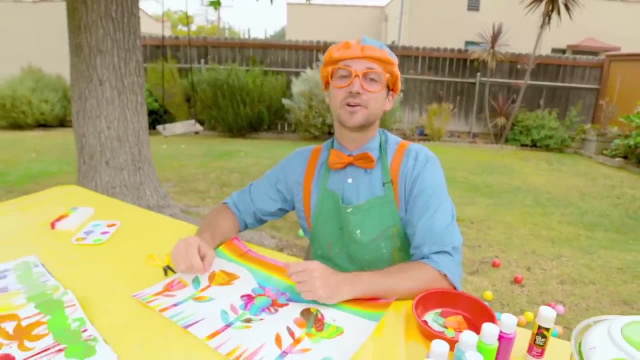 and about flowers, and also that amazing book about penguins by Sarah. Well, this is the end of this video, but if you wanna watch more of my videos, all you have to do is search for my name. Will you spell my name with me? 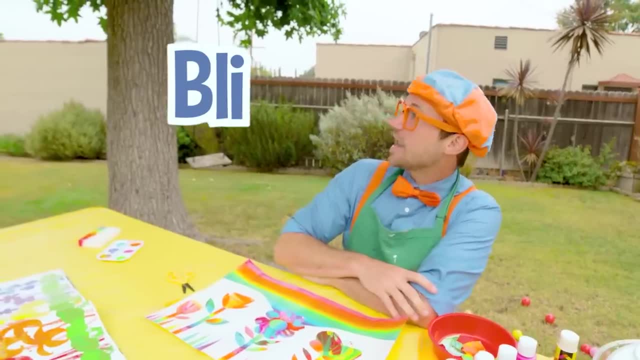 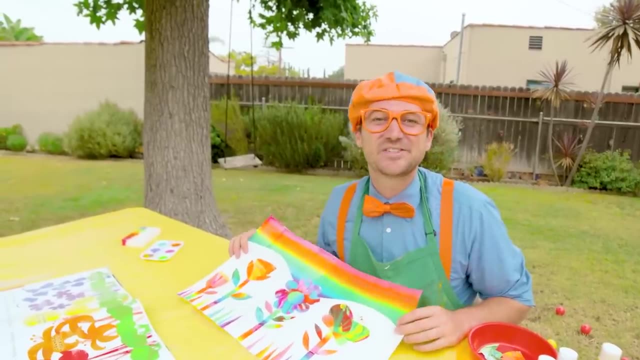 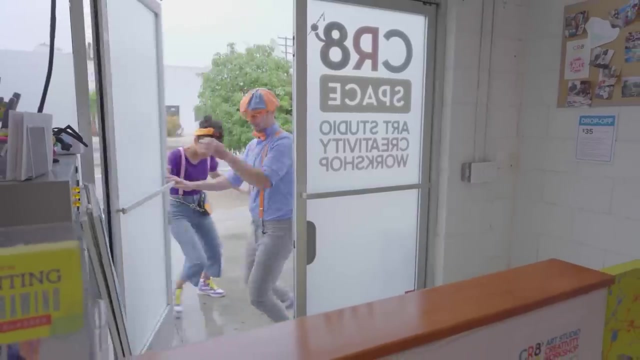 Ready B-L-I-P-P-I Blippi, Good job. All right, I'm gonna go frame this and put this in my tree house. All right, see you later. Whoa, Whoa, Whoa, Whoa. 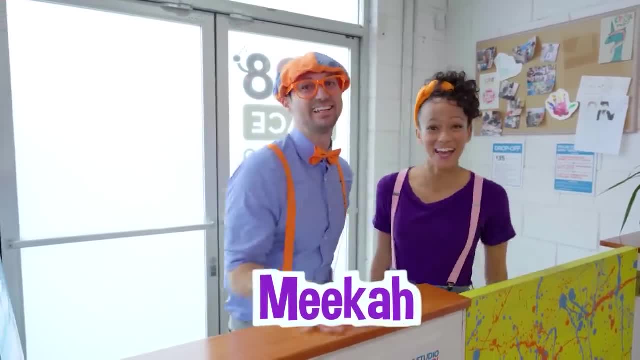 Wow, Hey, it's me Blippi. Hi, I'm Mika. Yeah, and it's sure raining outside today. Yeah, super rainy day, but luckily we are home. Yeah, super rainy day, but luckily we are home. 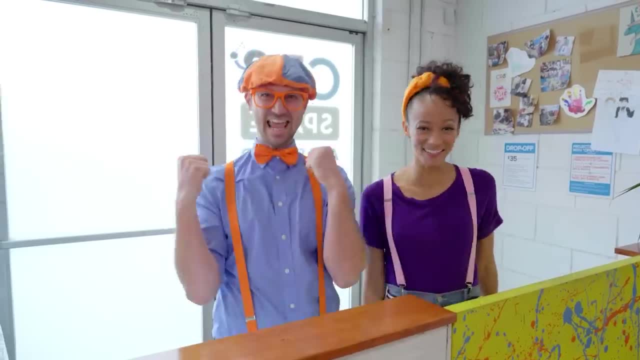 Yeah, super rainy day, but luckily we are home And we are indoors for some inside fun. And we are indoors for some inside fun- Yeah, Today we're at Create Space in North Hollywood, California. Yeah, and I'm so excited because we get to make art here. 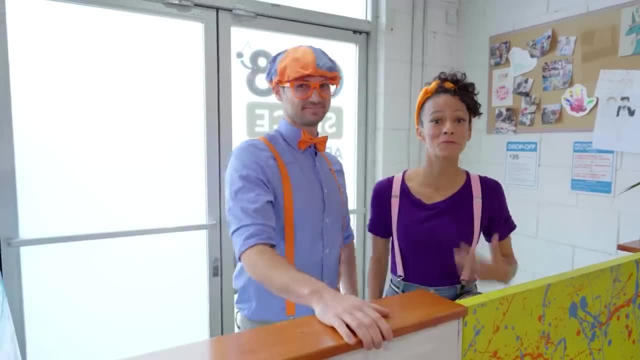 And we're so excited because we get to make art here. Yeah, art is awesome. Yeah, I love it. Shall we? Yeah, let's go, Whoa, Whoa, Look at all these paintings. Yeah, there's so many, and they're all in frames. 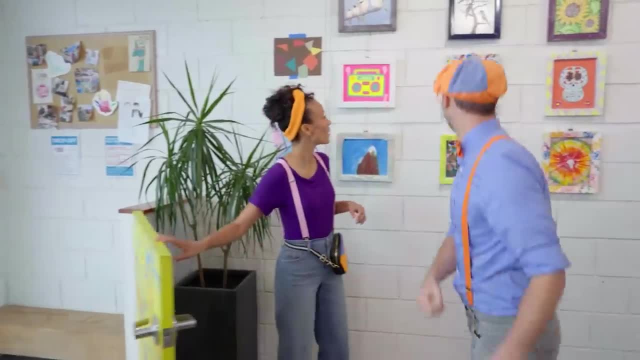 Oh yeah, All the frames are the same shape. Yeah, do you know what shape that is? I don't know. It's a unicorn, What about it? It's a unicorn, It's a unicorn, It's a unicorn. 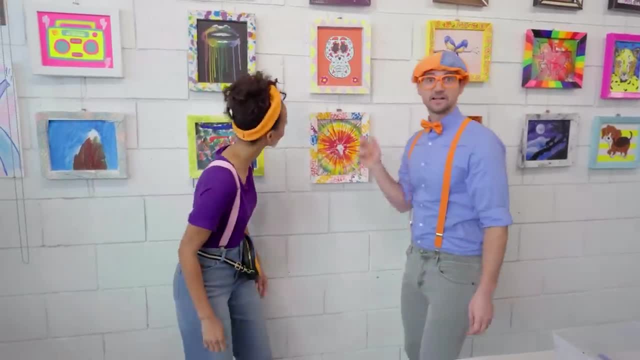 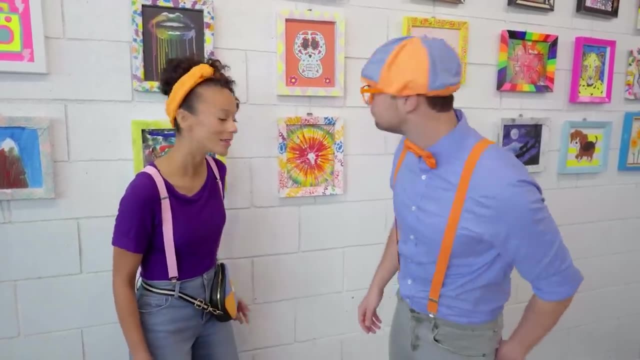 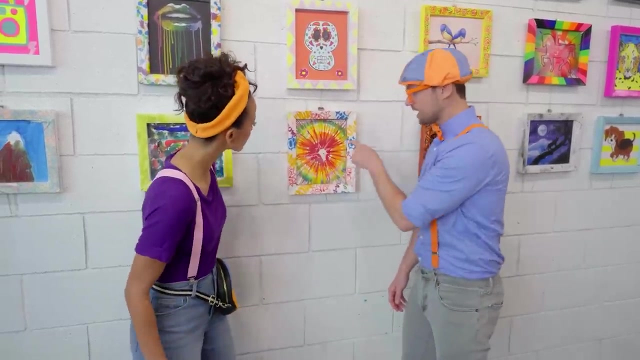 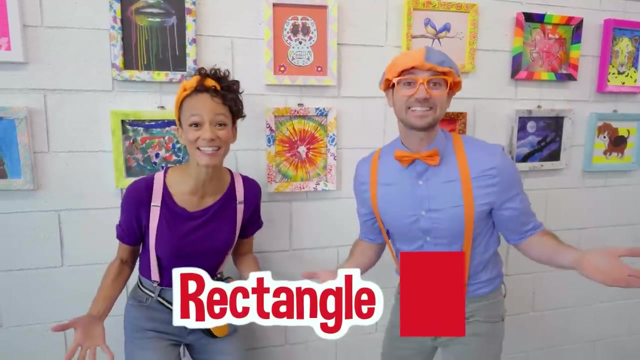 I know it, It's a unicorn. yeah, all the frames are the same shape. yeah, do you know what shape that is? hmm, that kind of looks like a square. that's right, because there's one, two, three, four sides. yeah, but look, mika, these are longer than these. you're right, which means it's a rectangle. 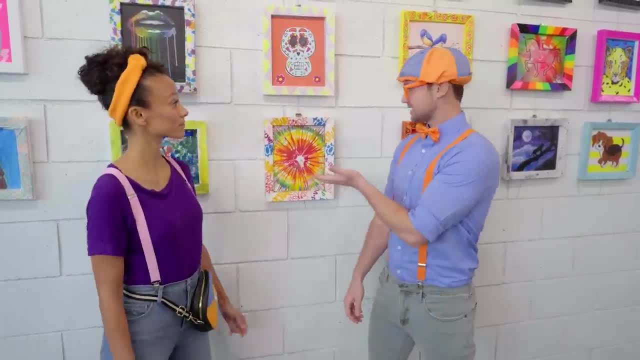 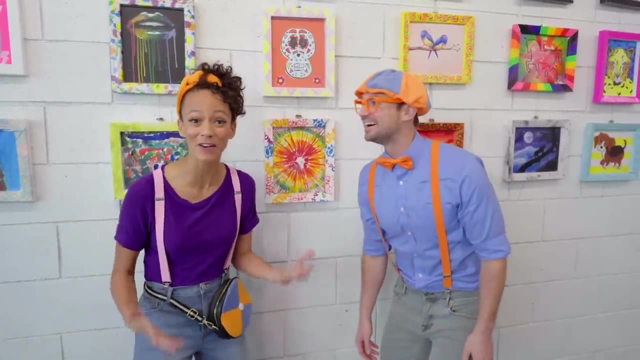 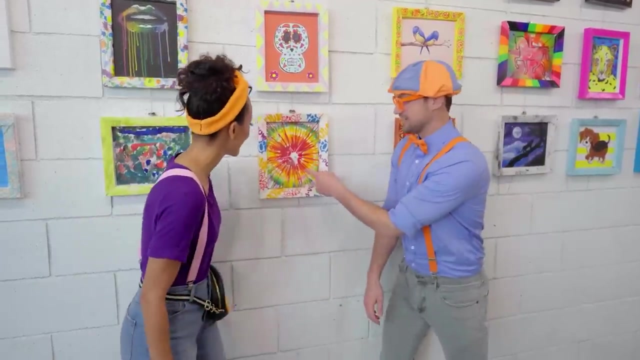 oh, wow, okay, all the frames are the same shape, so they're all the same. yeah, but look, all the paintings are different. yeah, that's the cool thing about art. it's such a fun way to express yourself and everyone comes out with different pictures. yeah, like this one so colorful. oh, look at this one. 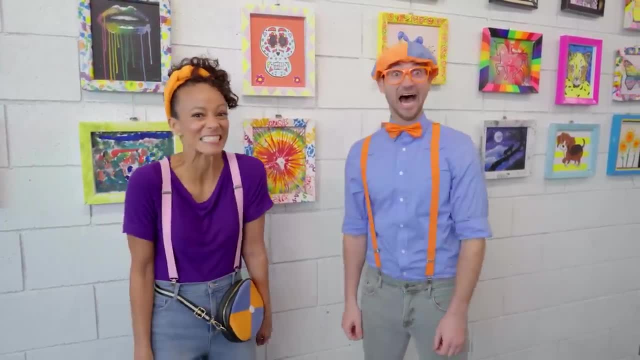 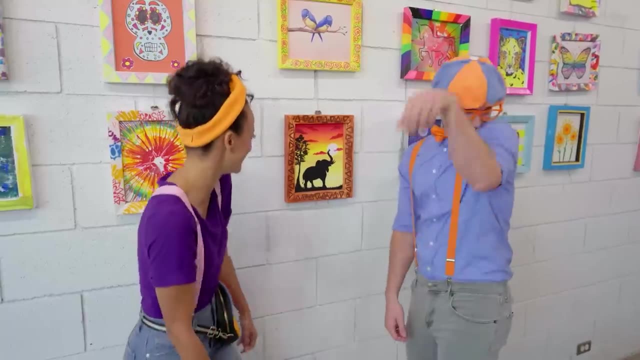 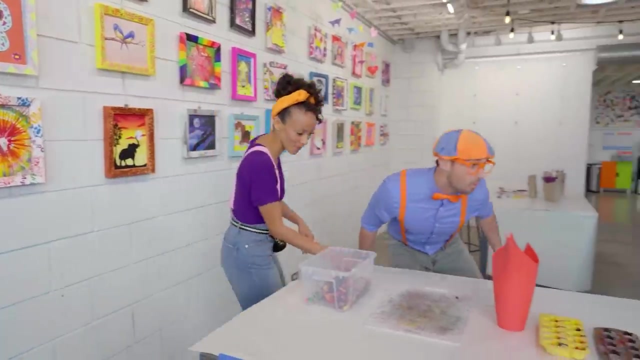 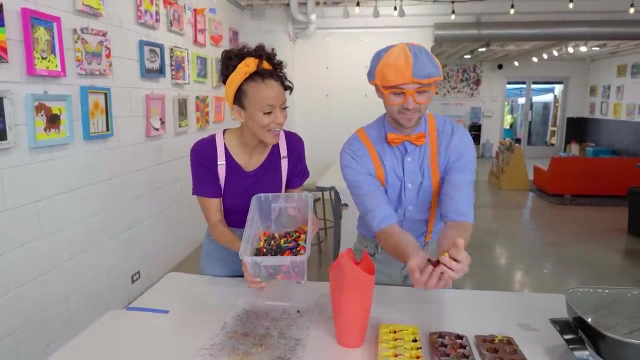 whoa, it's kind of spooky. yeah, i love the teeth. oh. and look an animal, an elephant, oh, cool. and look at the two little birds, oh, what's on this table? oh, looks like a lot of cool things, yeah. oh, look crabs. whoa, so colorful. so many different crayons. 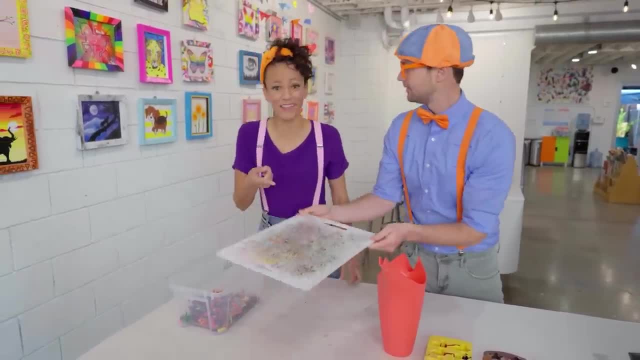 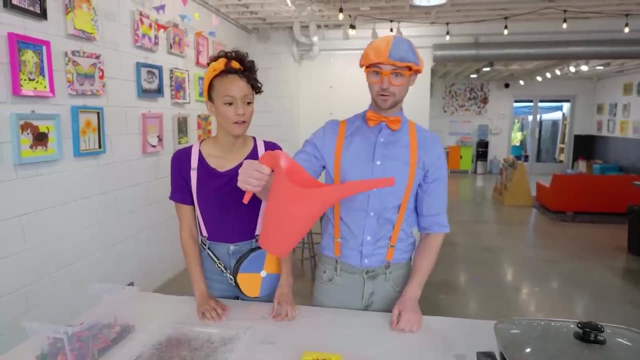 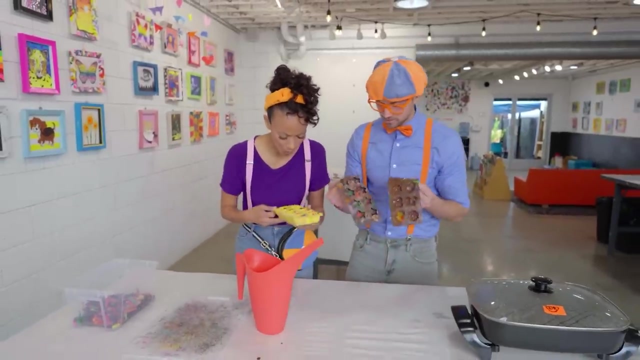 whoa, look at this. a cutting board. usually find that in a kitchen. yeah, i know interesting. oh, what's in there? oh, looks like one of those things that you use to water plants with there's water in there there. oh, yeah, probably shouldn't pour that out. whoa, look at these molds. something else you might. 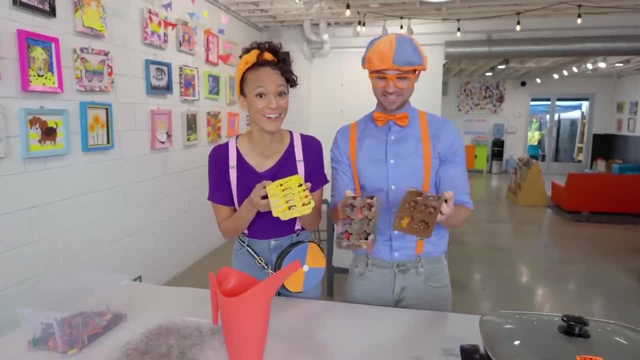 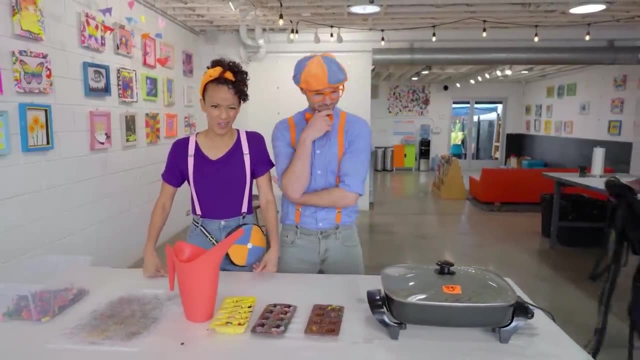 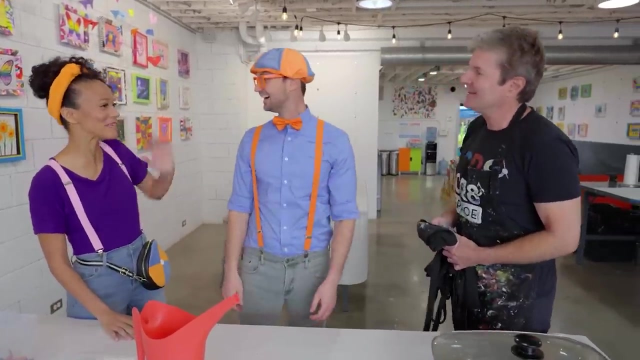 find in a kitchen. yeah, you can even put chocolate in these, oh yummy. whoa, hey, in a skillet. we must be cooking today. yeah, cooking art, hi, oh, hey, who are you? i'm david. wow, nice to meet you, david. i'm blippy, hi, blippy. i'm mika, hi, mika, what do you do here? well, this is my art studio. wow, cool, we love. 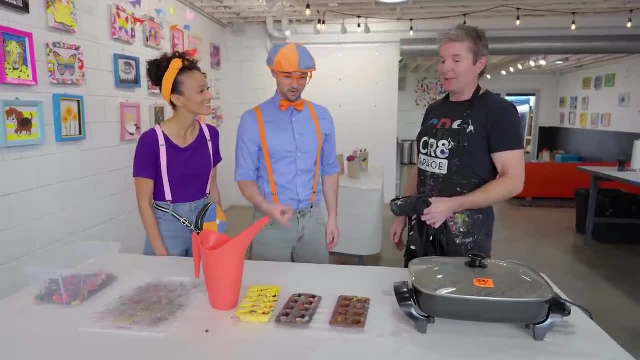 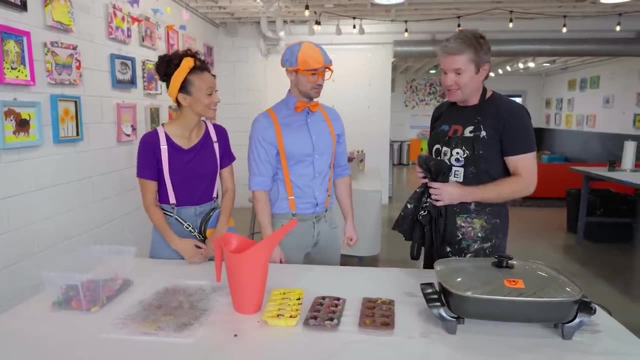 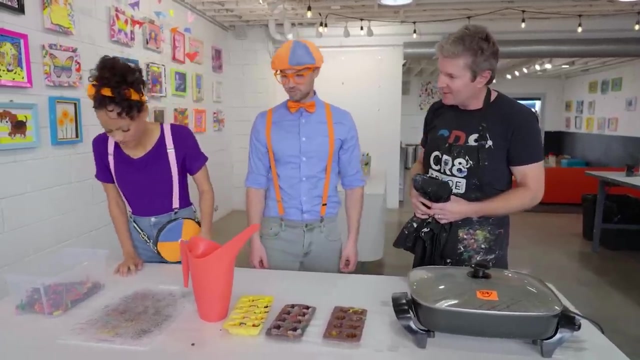 it here. it's really cool, thank you. yeah, it's been a dream of mine to do this forever and my dream came true. i would love for you guys to try a little project with us today. wow, did you figure out what all this stuff is for? no, we couldn't figure it out, but we saw everything that was here. 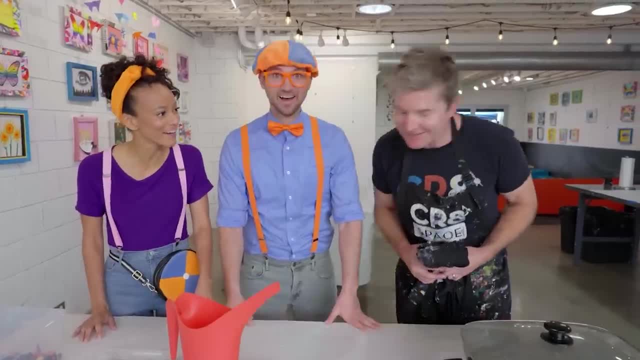 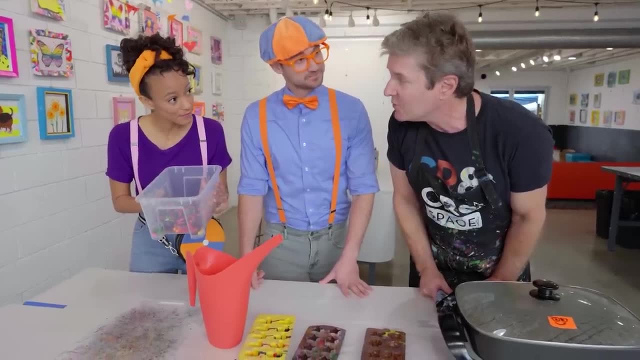 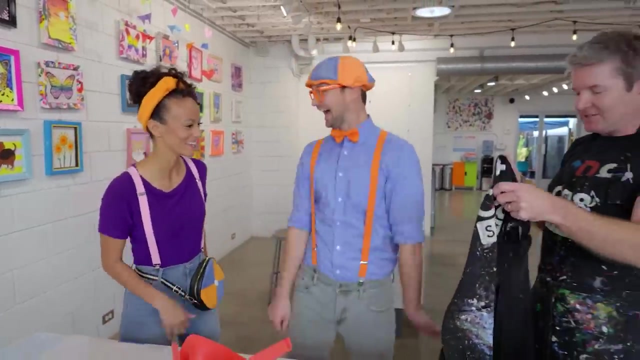 looks like we're going to cook. yeah, surprise, we're going to cook crayons- cooking crayons. you can't eat crayons. yeah, so these crayons are going to be reused. we're going to turn them from something old to something new. oh cool. how are we going to do that? let's get started, okay, first of. 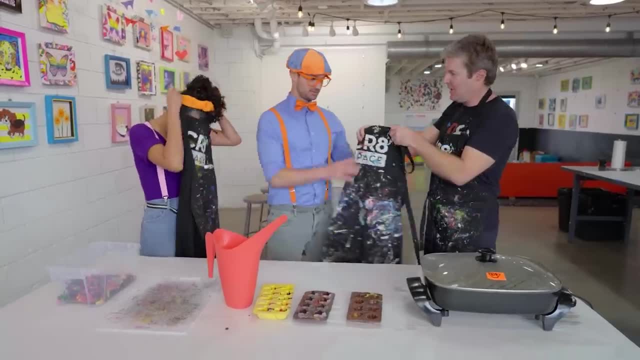 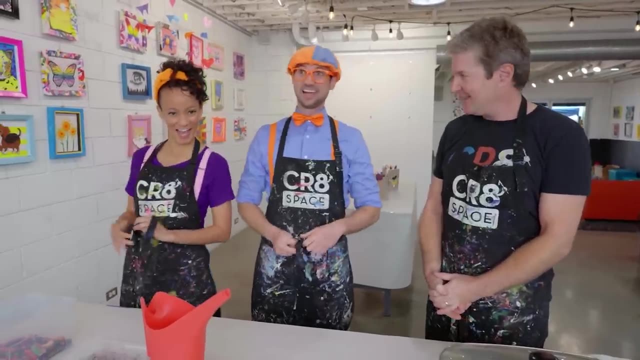 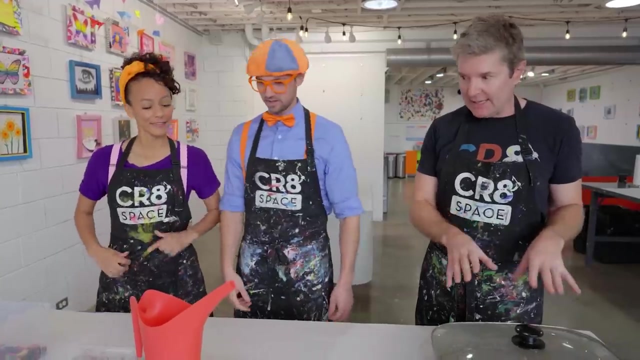 all here. here you go our aprons. you can put them on. keep your your cool clothes nice and clean. thank you for saying that we look so cool. yeah, we try every day, okay, so, so we're going to pour water into this skillet. it's going to get hot and while it's 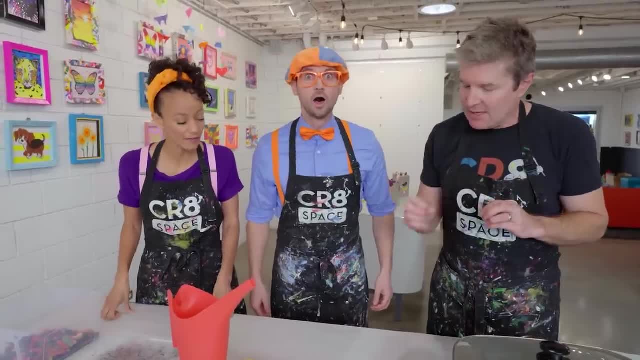 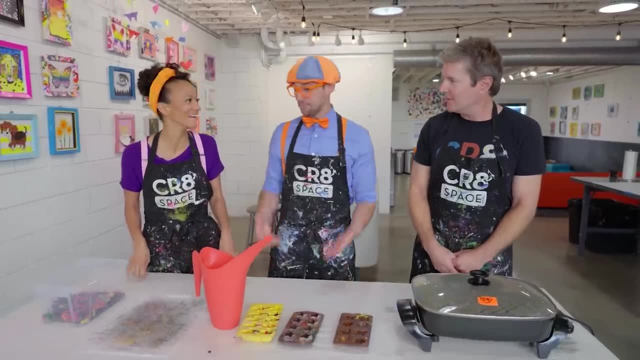 heating up. we're going to take those crayons and break them into pieces. okay, sprinkle them in the molds, put the molds into here, uh-huh, and then we're going to cook them. so we're going to mix these cranes together. they're going to melt, we're going to put them in there and then we're going to. 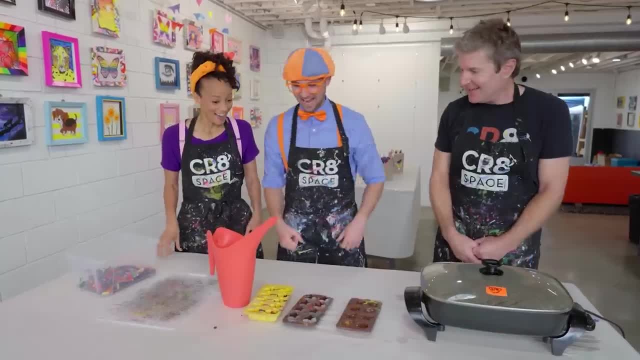 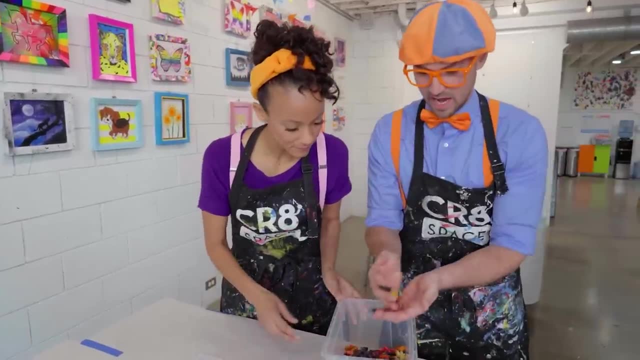 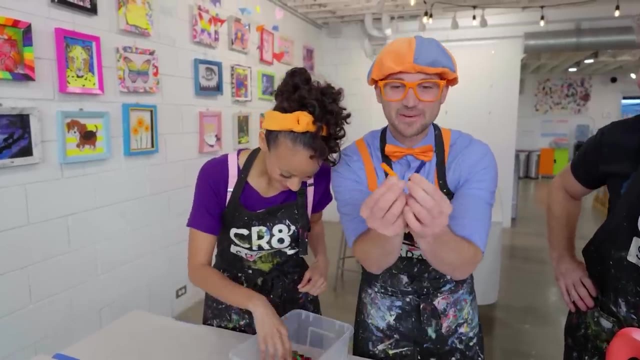 make rainbow crayons. yeah, love it. well, shall we sure? all right, pick your favorite colors, okay, right, ooh, let's see. well, i like blue and orange. oh yeah, he really does. okay, and i love purple and yellow. yeah, take it out. blue and orange. oh, there's some yellow. i like orange and orange. 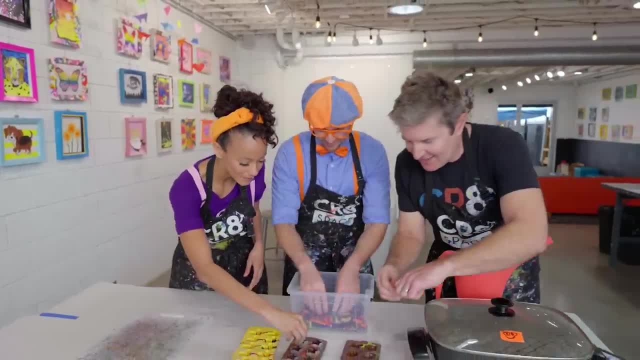 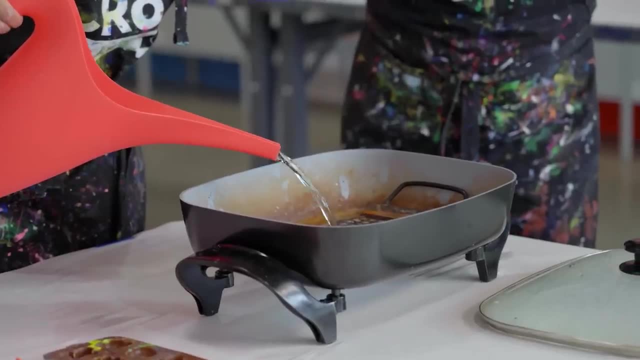 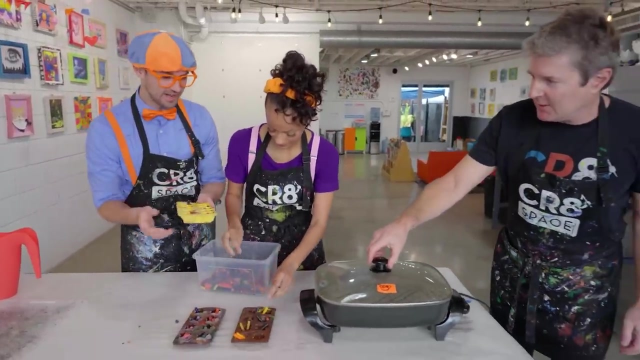 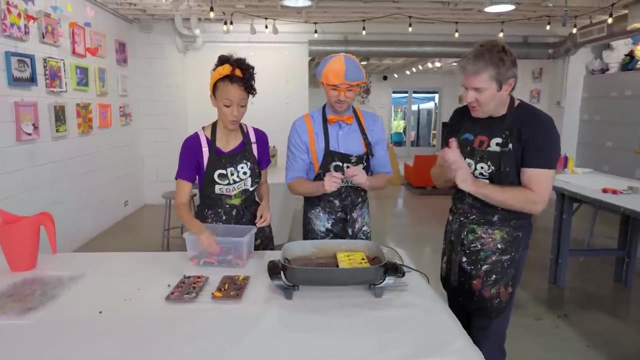 here you go. thank you okay, break them in there. okay. okay, you ready? yeah, come on, we put it in there now. yeah, all right, go ahead. and uh, if you don't mind, it's gonna get hot. so, okay, just be really careful. okay, all right, this hot, it's a good idea to do it with a grown-up. yeah. 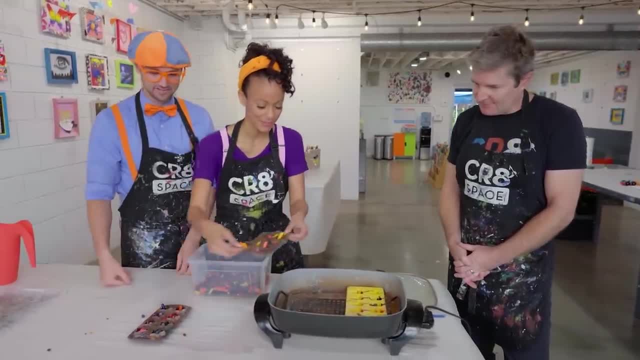 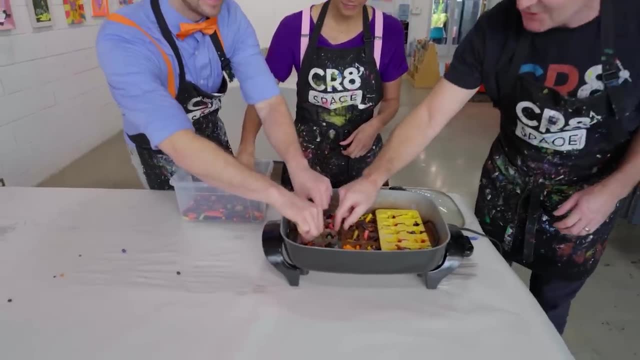 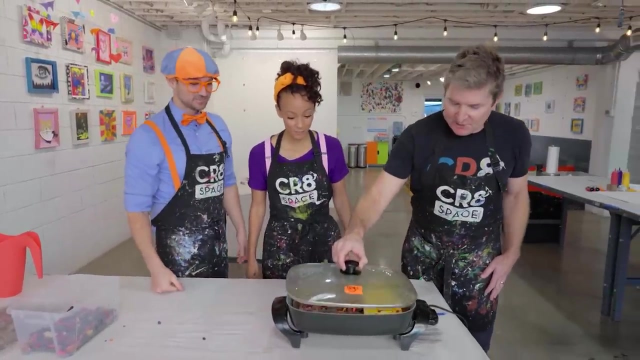 yeah, all right. and here's another that looks great. just set it right in the water, okay. and then this one: perfect. oh, you guys, these are gonna be so cool. i'm so excited. nice work, i love your colors, thanks, um, if you guys don't mind, i'm gonna stay here and watch this cook. okay, okay, and if you want, 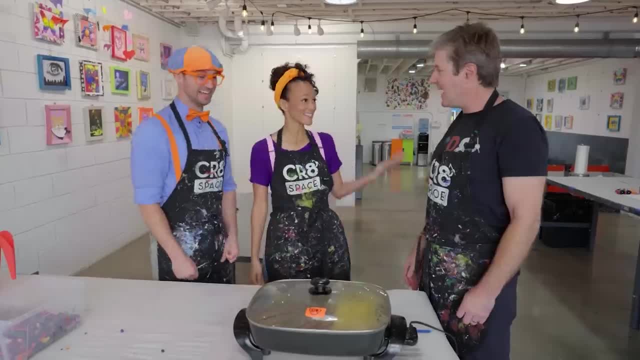 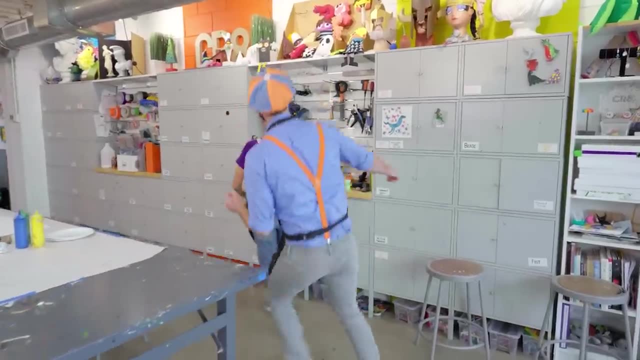 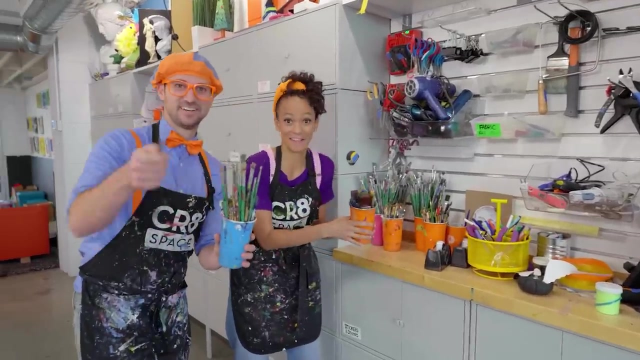 go and explore the art studio. all right, that sounds like fun. okay, yeah, thanks so much. have fun, wow, oh, look at this place. yeah, oh, look at all these scissors. whoa, oh, and look. paint brushes- yeah, a lot of paint brushes, wow, sizes, yeah, oh, and some tape. 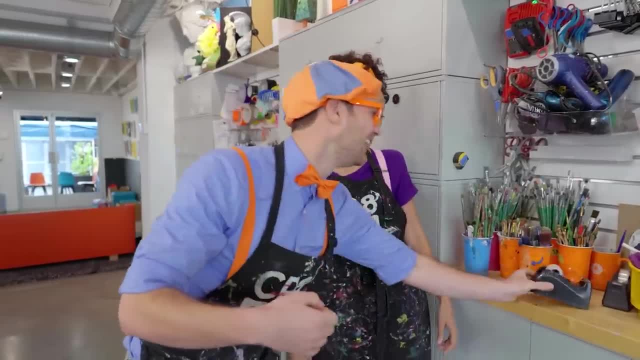 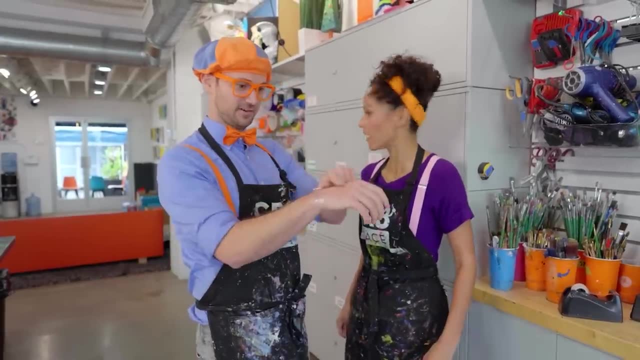 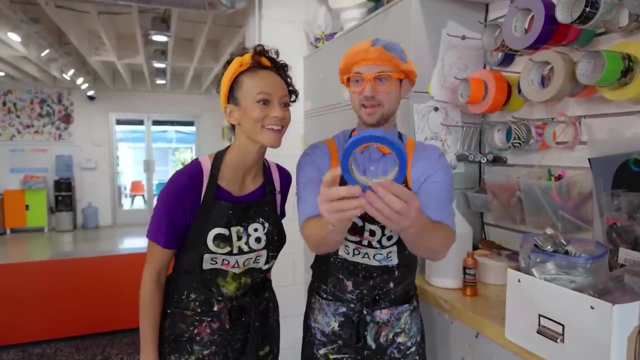 oh, stick things together. whoa, yeah, it's really cool how there's a lot of different materials to use for art. that's right. oh, and there's even more over here. whoa, whoa, check it out. more tape, oh, some blue tape, one of my two favorite colors. yeah, oh, and look. purple tape, my favorite color. 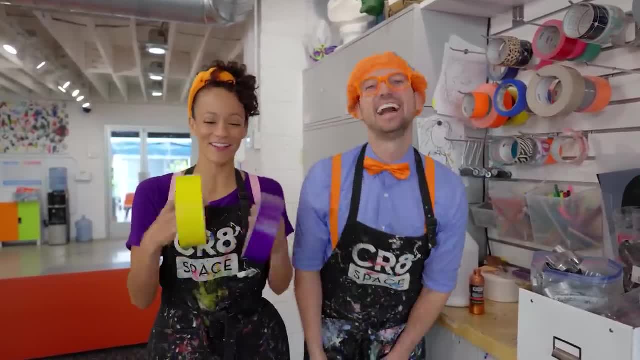 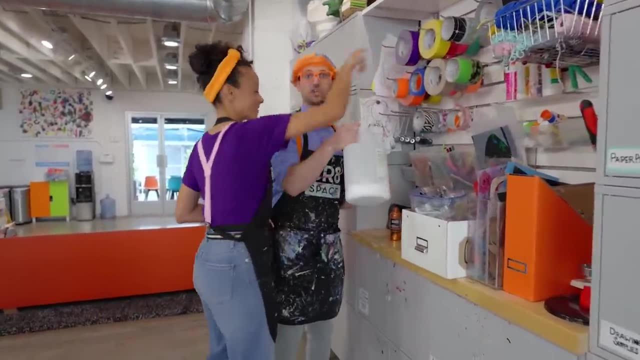 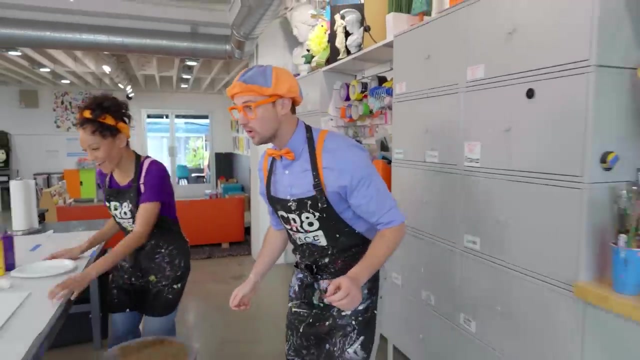 yeah, and look, mika, my other favorite color- you know me so well- yellow. wow, this is so cool. it looks like we have a bunch of glue. whoa, that's a lot. wow, whoa, mika, check it out. whoa, look at all of this stuff. it looks like it's all set up for. 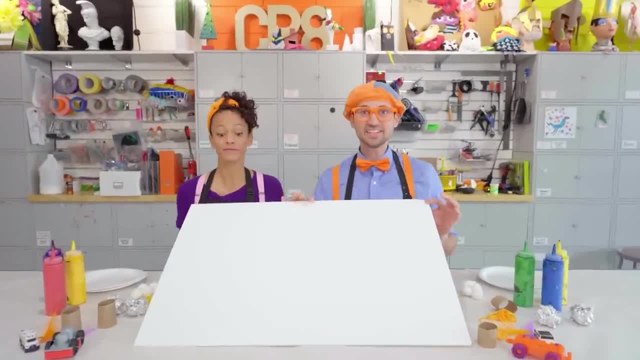 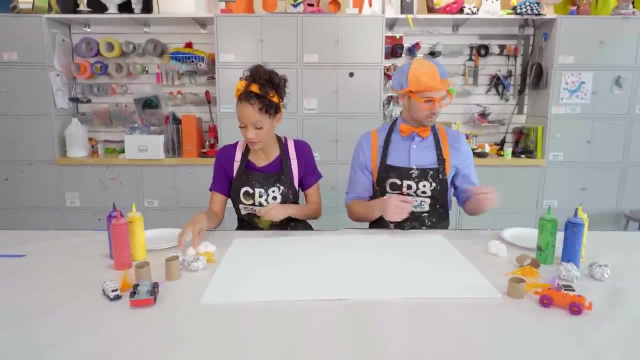 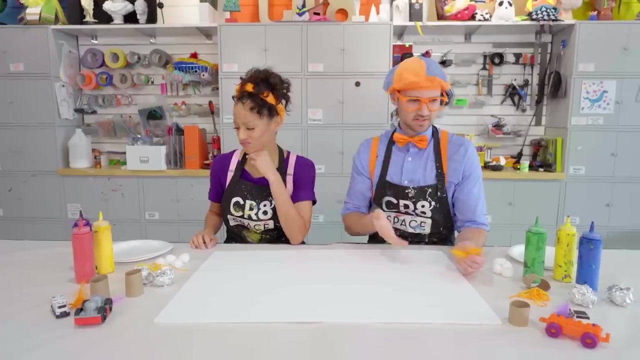 us to make a picture together? yeah, check it out. this is our canvas. should we make a picture together as a team? yes, okay, we have paint and, oh yeah, cotton balls. huh wait, some feathers. where's the paint brushes? there's nothing on the table. i know what we use these. 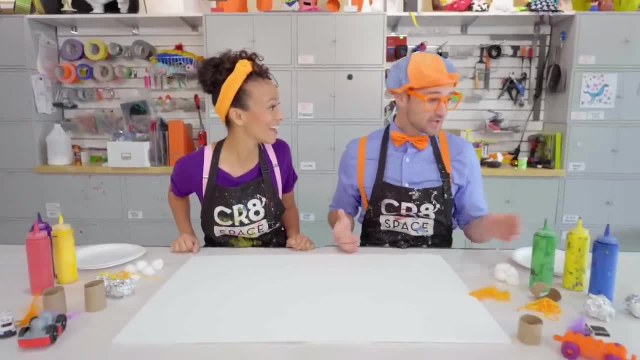 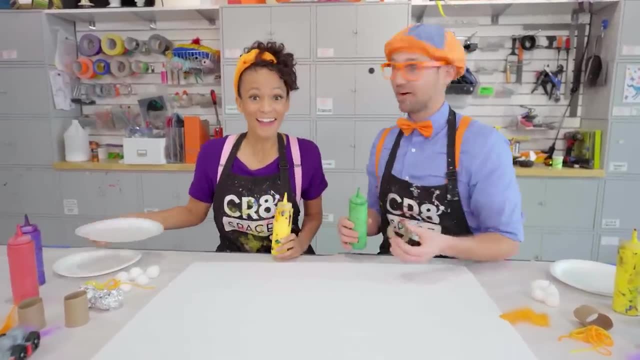 things to get the paint onto the canvas. oh yeah, you're right. so you're basically saying we can use, say this green, and then put it on this cardboard and then smash it down. yeah, all right, yeah, okay, okay, let's see, i'm gonna start with a yellow. 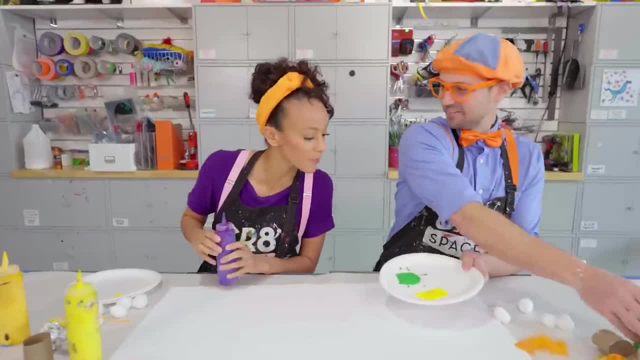 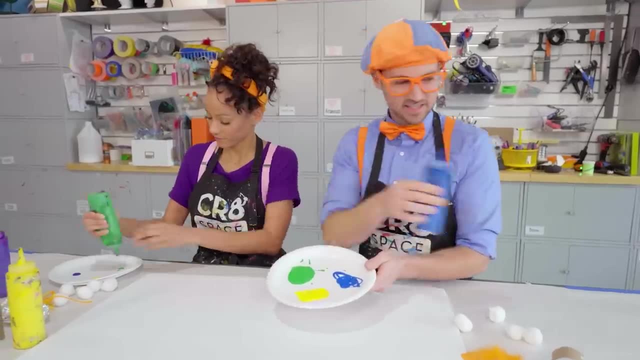 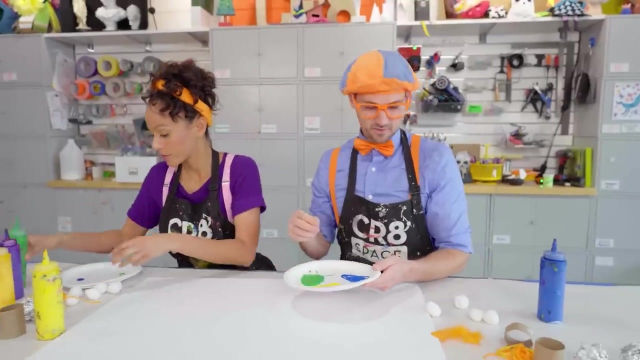 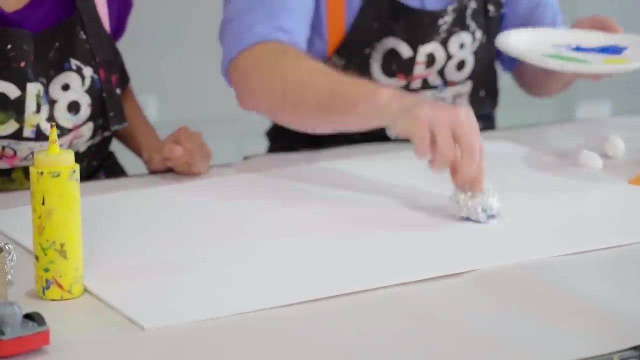 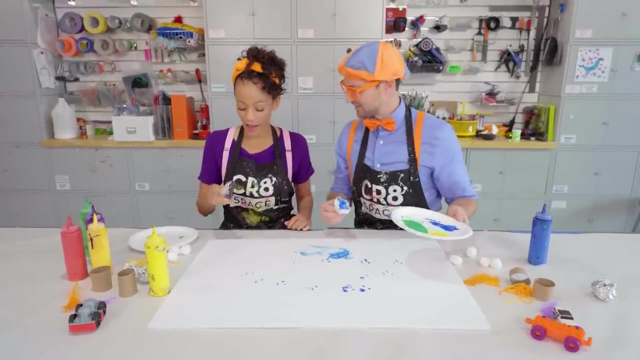 and here we go, all right, and here's some blue. what are you gonna use first? um, let's see. well, i have yellow, green and blue. okay, i'm gonna use some blue. i'm gonna use some aluminum foil. all right, now your turn. i want to take this car and i want to put it in the green paint here. 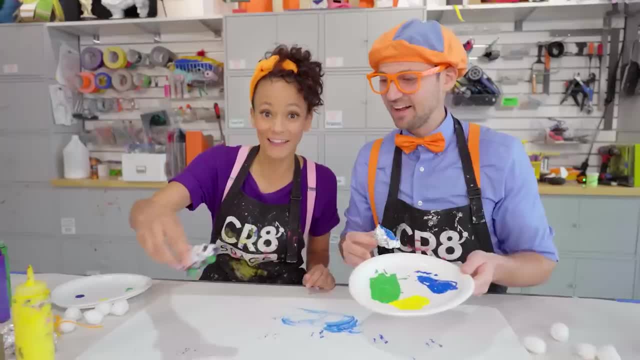 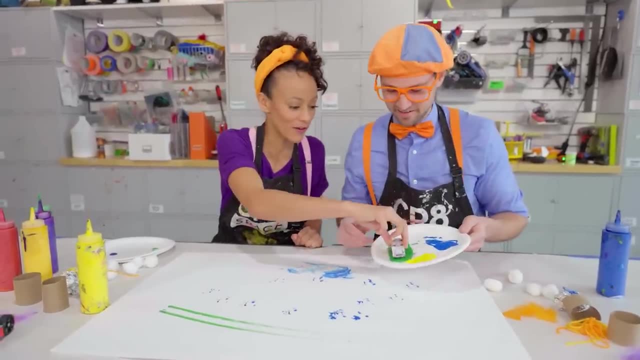 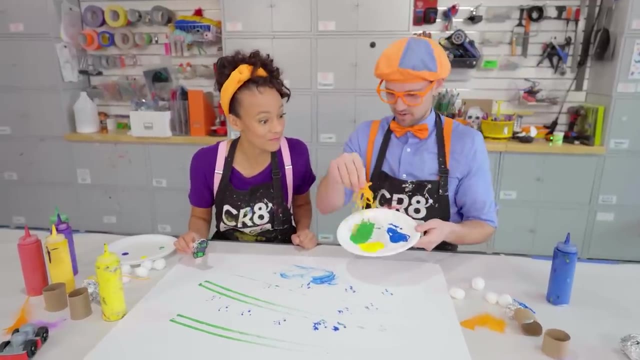 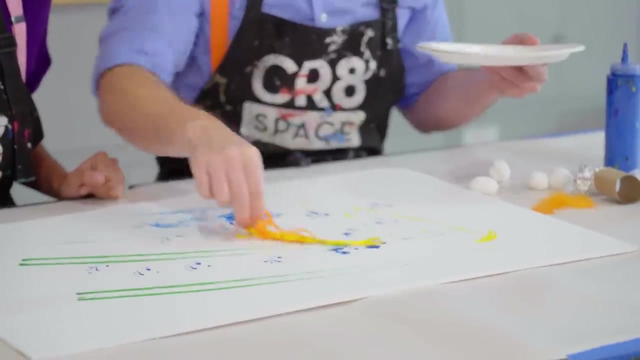 thank you, blippy. oh, you're welcome. whoa, all right, see what it looks like speed painting. whoa, yeah, that looks cool. wow, yeah, more on there looks like some mud tracks. yeah, you want to try? oh, oh, sure, oh, i'm gonna use some yarn. whoa, that's gonna look silly. yeah, okay, here we go. whoa, now, this is a masterpiece, it sure is. 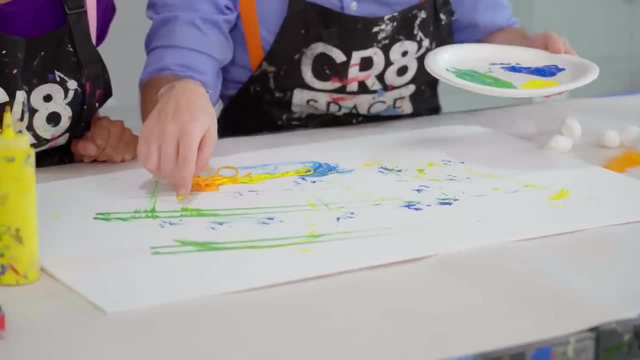 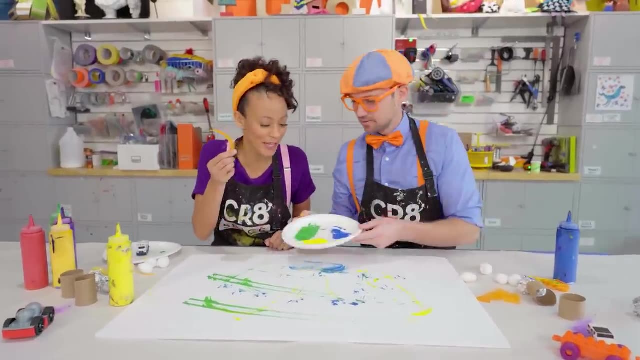 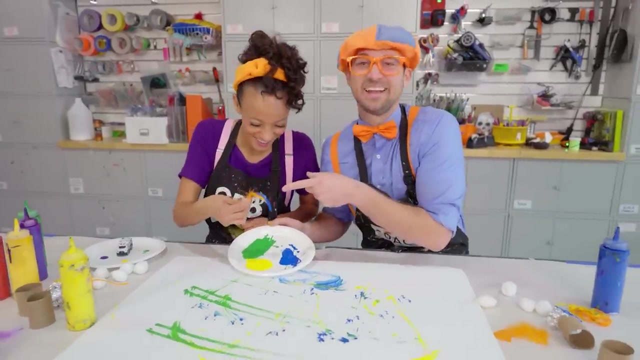 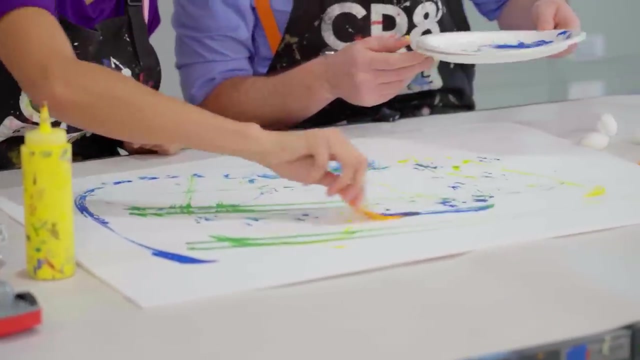 it went over the wet paint. it looks like the vehicle is sliding around, slipping and sliding. i wonder what a feather would look like. oh, you want to try some? trying some blue here? okay, now that's my kind of burn. all right, let's see. okay, whoa, whoa. that looks so pretty, mika, thank you. wow, oh, i have an. 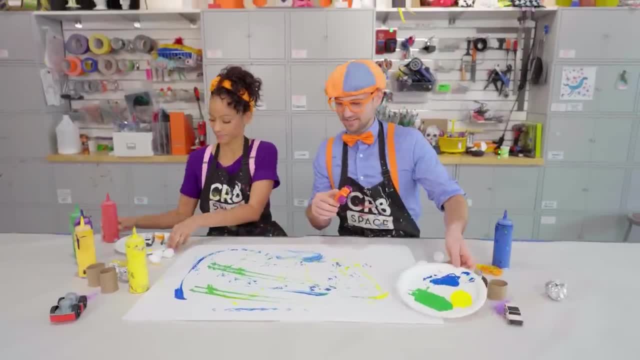 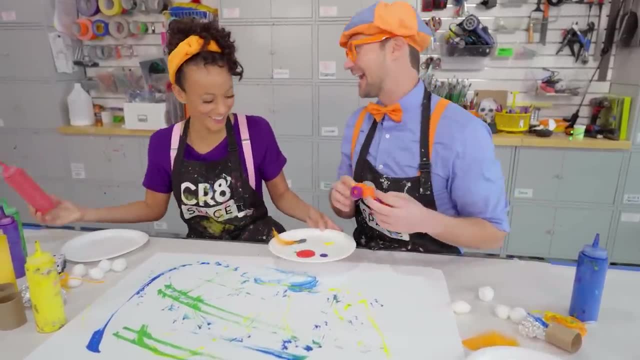 idea. do you think that red works? let's try it. all right, okay, this is gonna be so silly. okay, it works. it works really well. all right, i'm gonna need your help for this one. okay, okay, you see this. yeah, okay, will you pass me the red, sure, okay. 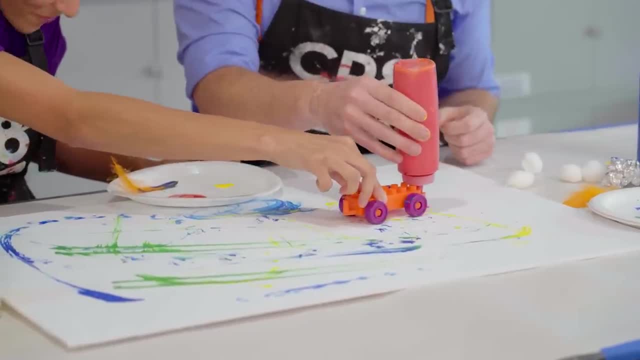 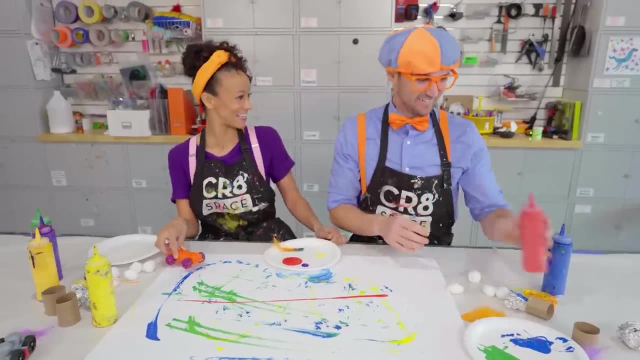 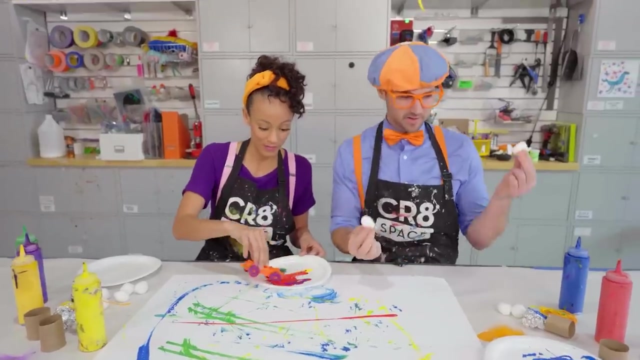 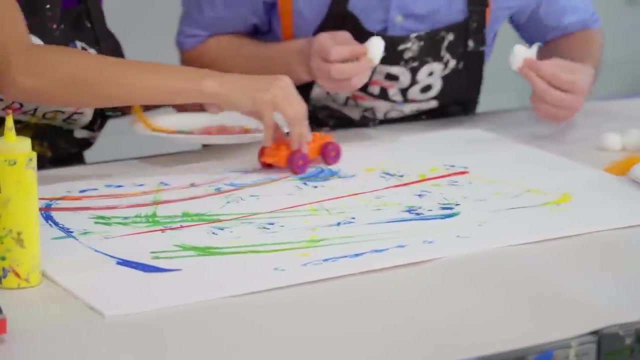 let me do a tie knit. thank you so much. now i want to put the wheels through the red here. whoa, oh, and some cotton balls. all right, i'm going gonna mix all the colors together. let's go override. مالج, oblاء مالج. 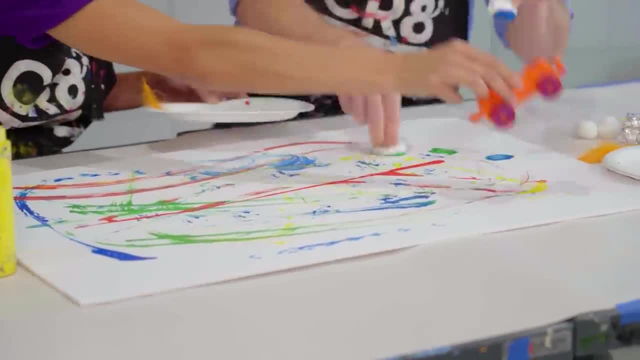 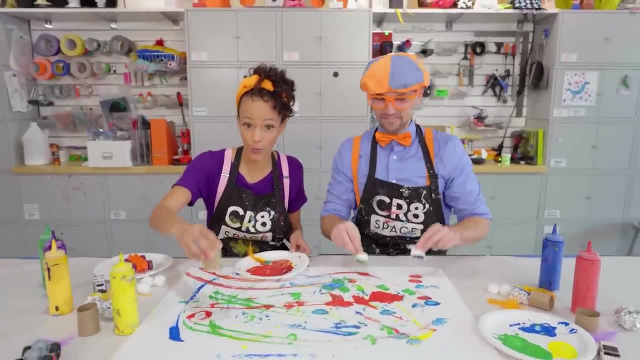 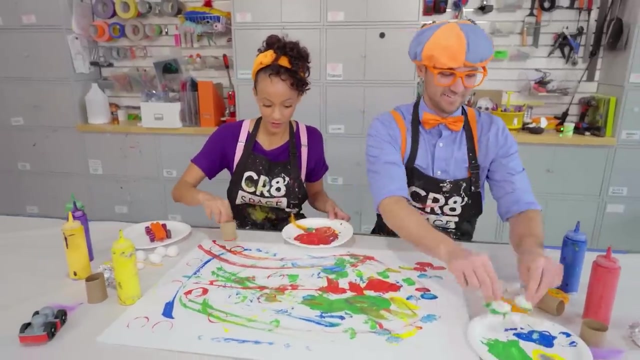 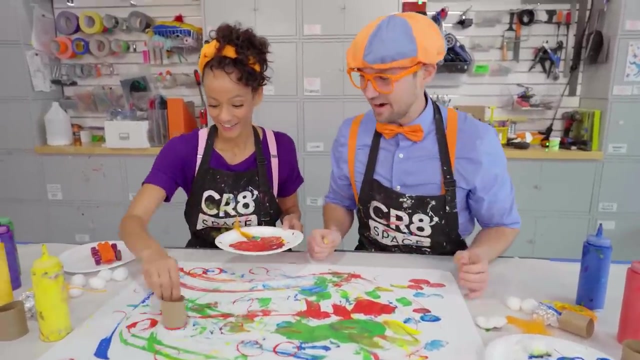 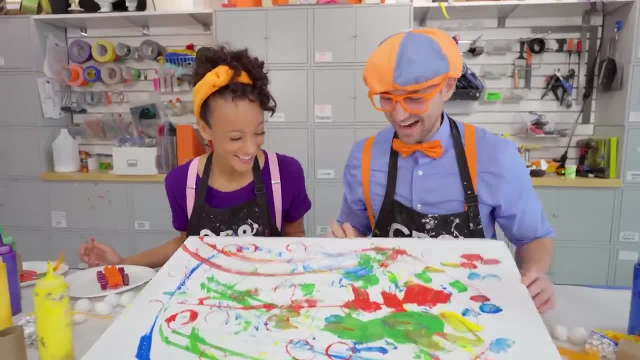 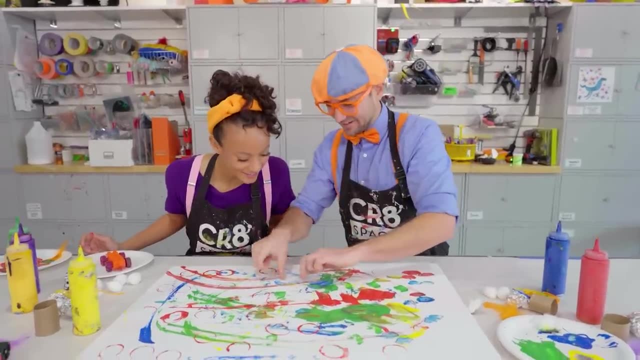 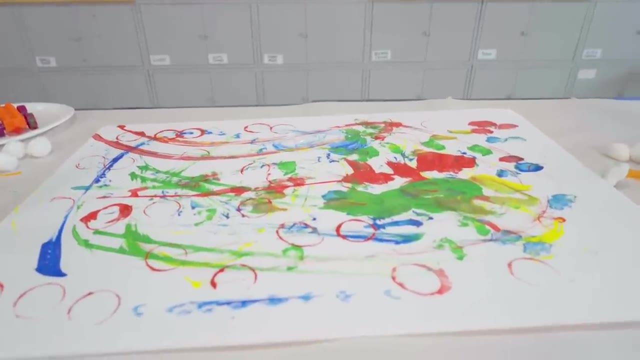 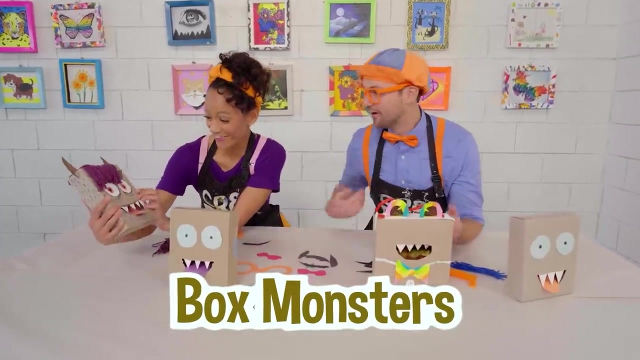 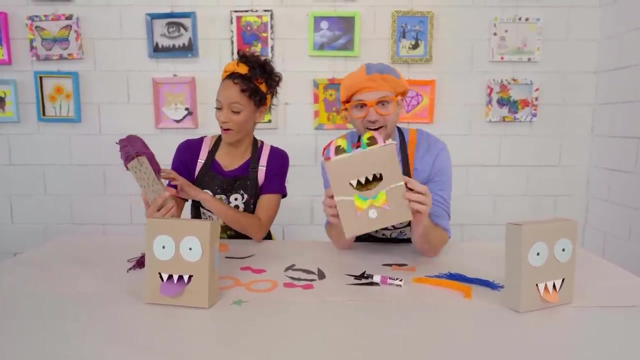 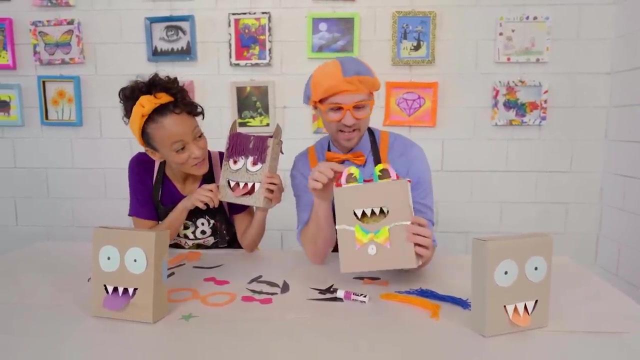 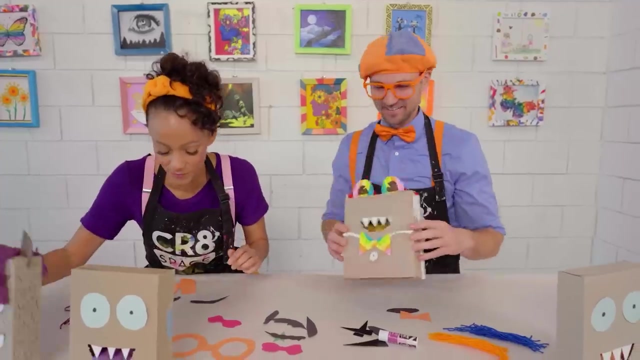 good, it looks amazing. wow, shall we let it stay right here to dry? yeah, let's go find something else to do. okay, here you go. wow, looks like box monsters. wow, they're so silly looking. oh yeah. oh look, the eyes are on top of that. and this one has rainbow eyes and a bowtie, just like me. button rainbow colors, it looks like. 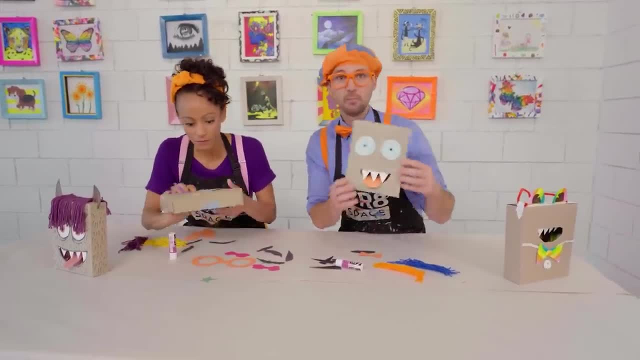 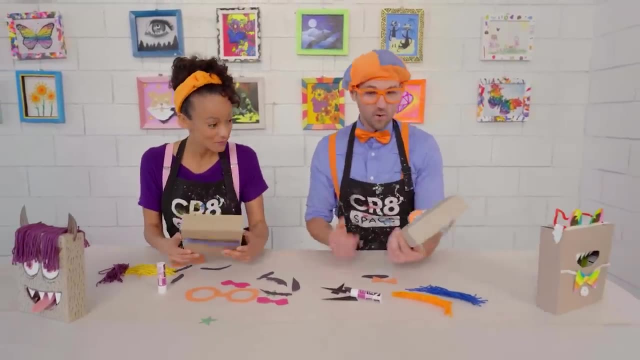 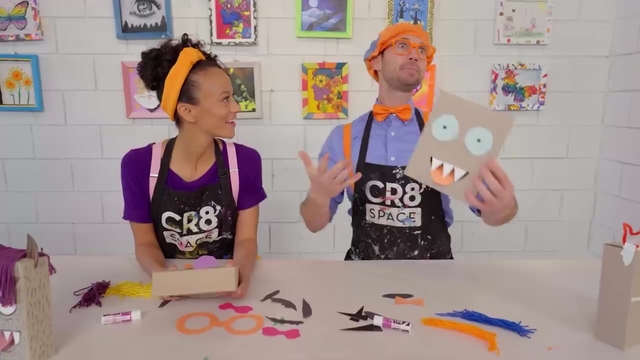 there's other bow ties and things here, oh, and some blank monsters. we can make our own monsters. oh, what kind of monster should we make? hmm, I know what I'm gonna make. what I'm gonna make: a Blippi monster box. oh, that's a great idea. 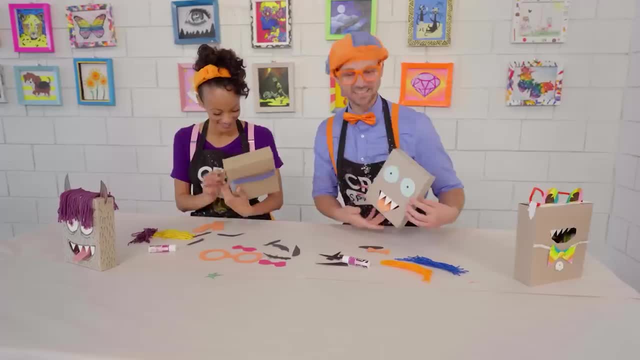 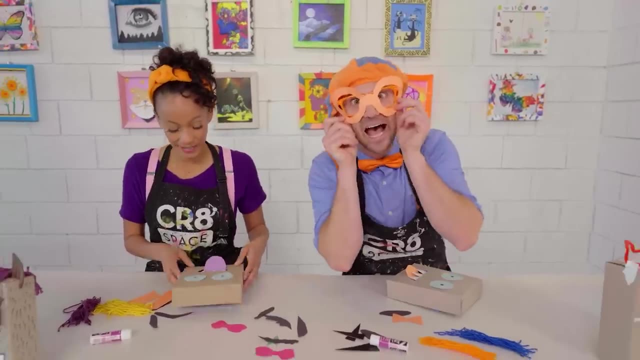 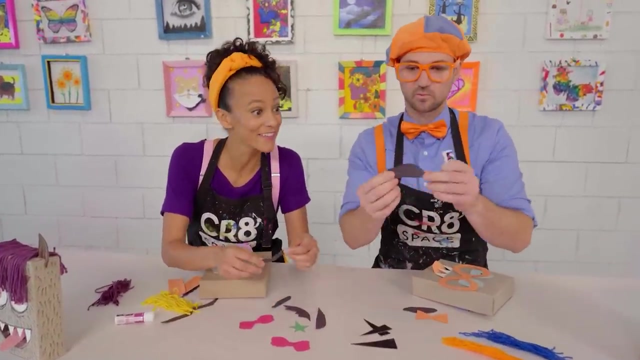 I'll make a Mika box. oh, that's a great idea too. whoa, look these. look like my glasses. oh, that's perfect. let's see what we have. oh, look, a pink bowtie if you want to pee. oh yeah, it looks like a really big, uh eyebrow. yeah, how do I look? I know. 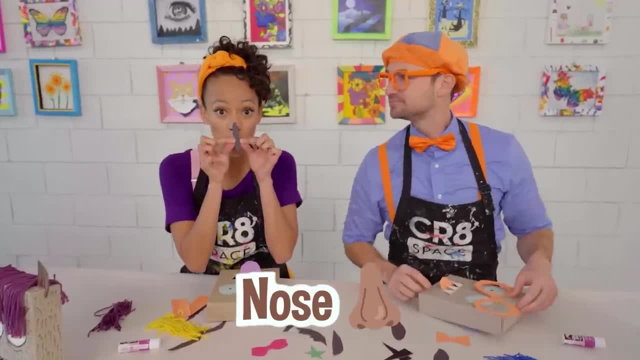 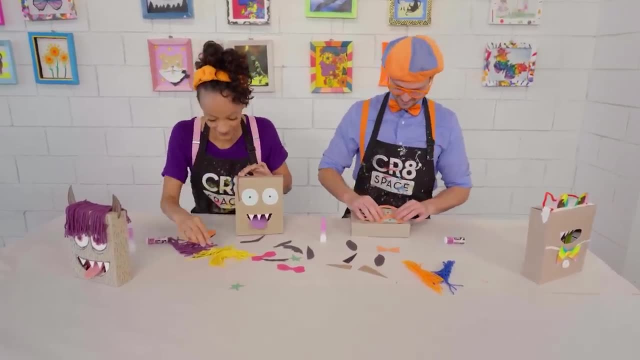 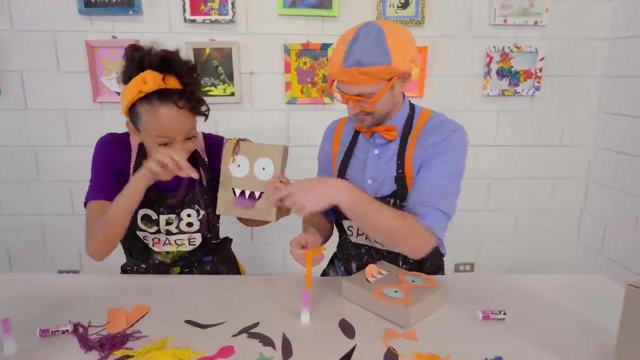 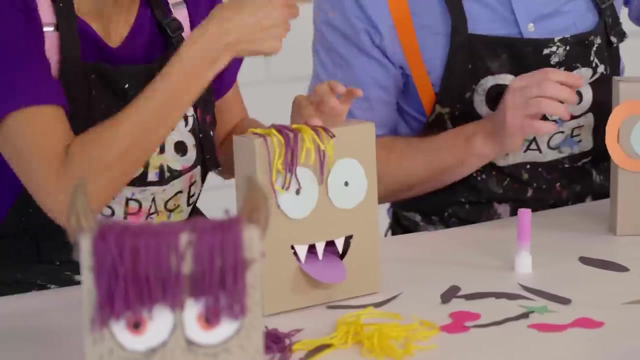 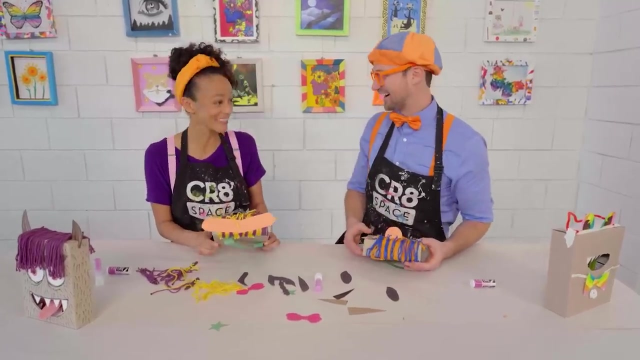 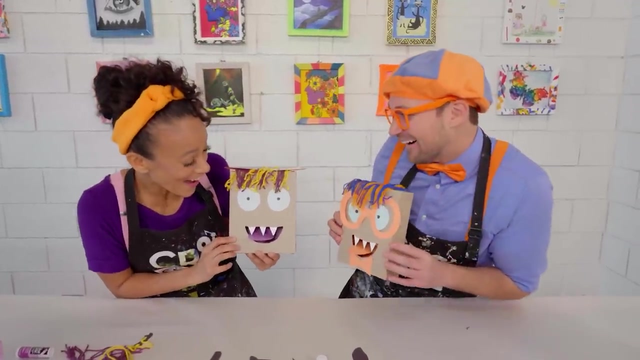 oh, very funny, but this could be a very long silly nose. whoa, now that is silly. yeah, okay, foreign, foreign, foreign, foreign. oh, all right, are you ready? yes, I'm so excited to see your monster. here we go. oh wow, it looks just like you, Mika. thank you, Monster Mika. 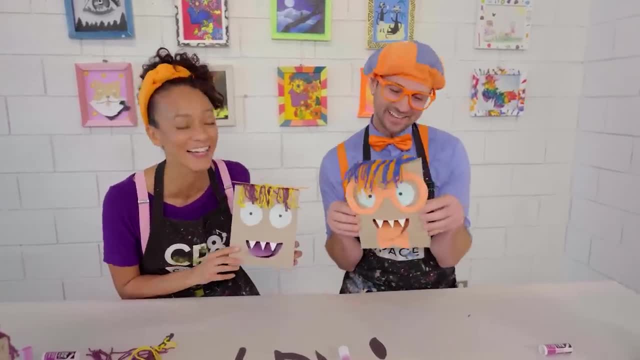 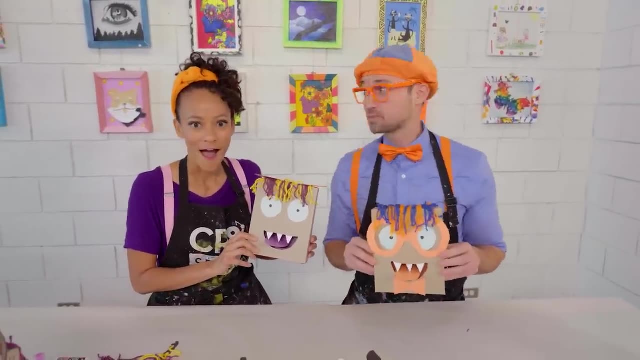 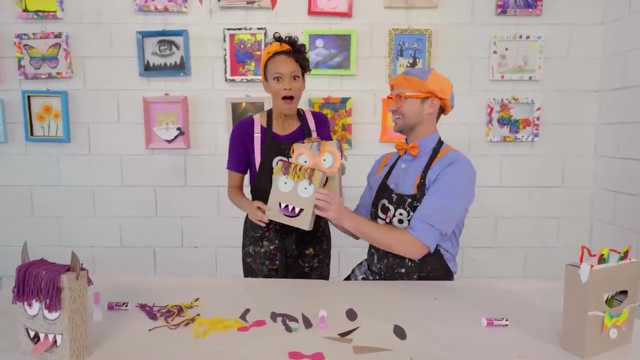 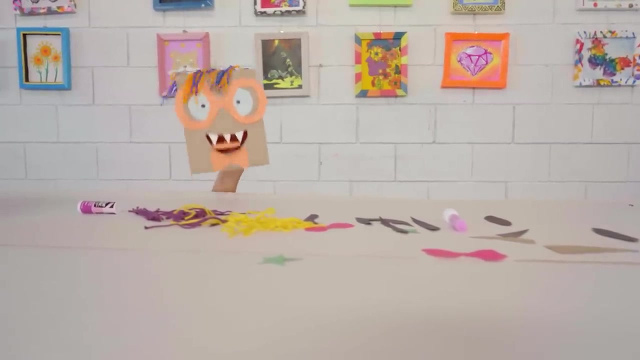 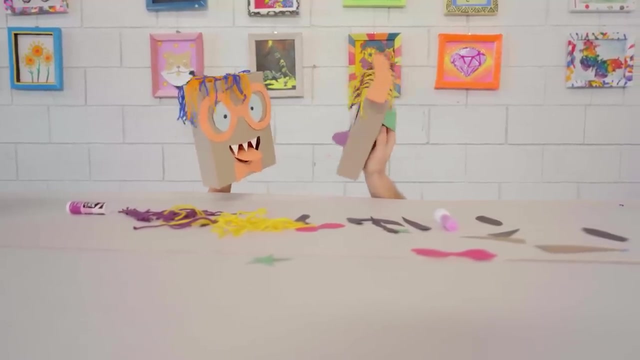 look at yours, Blippi. that looks amazing. oh, thank you, hello. so silly looking well. shall we have a monster box puppet show? yes, we shall. yeah, hey, I have an idea, though what shall we? Oh, I'm Monster Blippi, hello, Wow, hey, Blippi. oh, I mean Monster Blippi. you look fabulous. 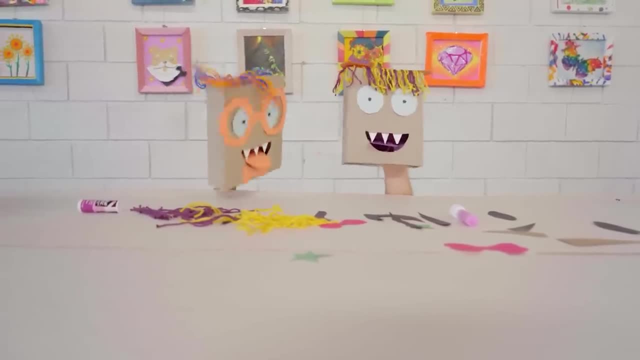 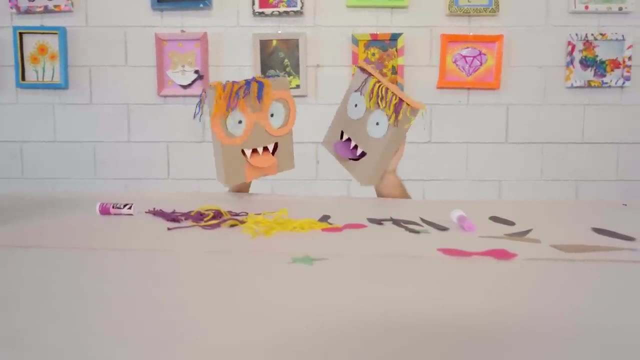 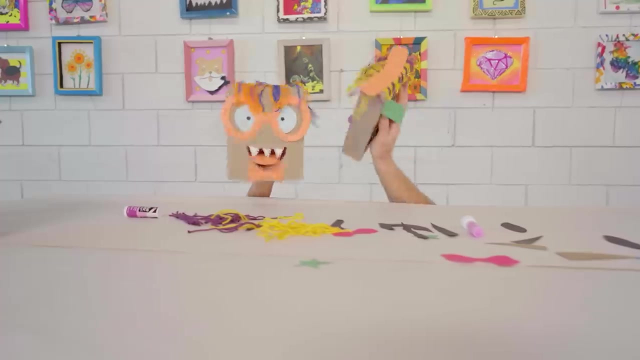 That's right. ha ha ha ha. I'm a silly monster looking good, Mika. Oh, thank you so much. Oh, did you notice my purple and yellow hair? Of course I did. it does look fabulous. Ha ha ha ha. you are so silly, Blippi. that's why you're my best friend. 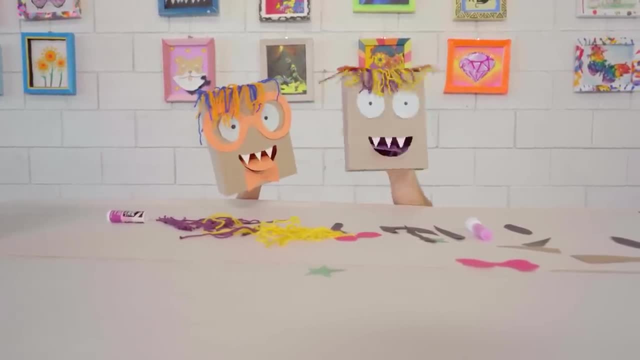 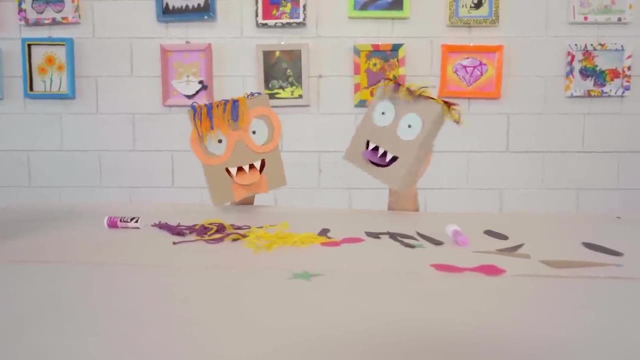 No, you're my best friend. Oh, no, you're my best friend. Oh, Mika Monster, we have fun together. Yeah, we do. we go on such fun adventures, That's right. hey, let's go on another one. 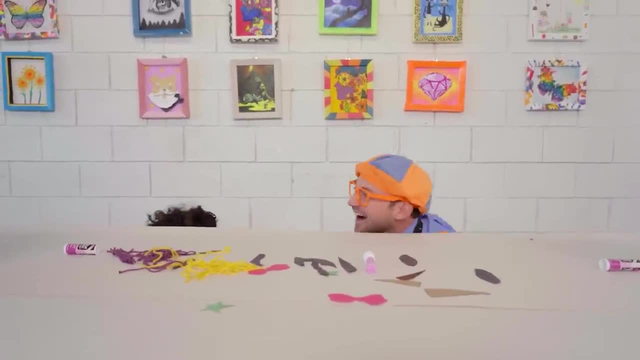 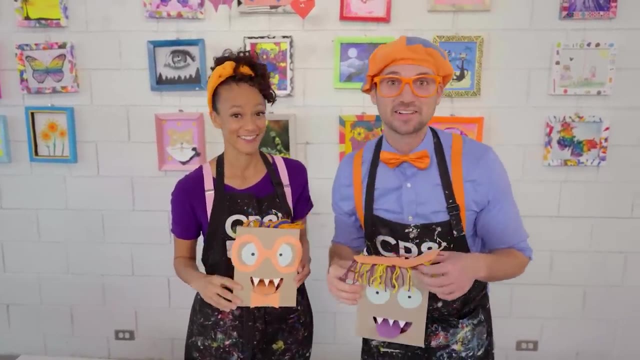 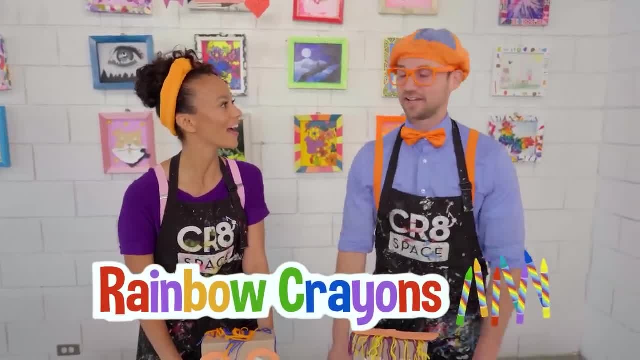 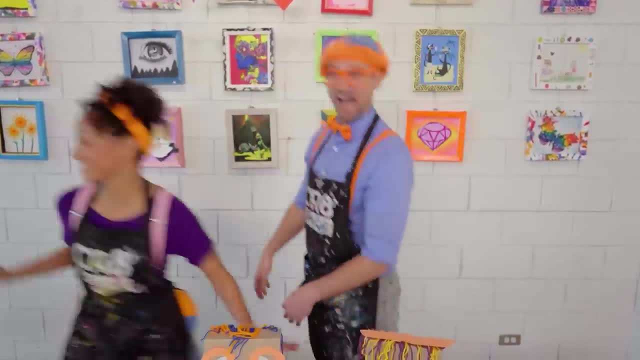 Yeah, and those rainbow crayons- wow, I bet they're going to be so colorful, I know, Hey, Oh yeah, Do you think they're finished yet? I don't know. let's go check, Come on Wow. 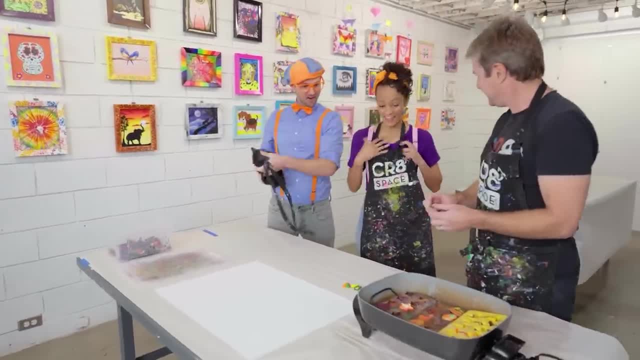 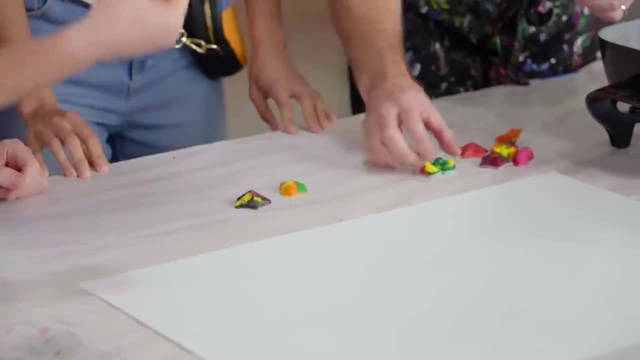 Oh, hey, Hi, Welcome back. Thank you. Oh, are they done? They are done. You want to see them? Wow, Whoa, Check it out. A star, Yeah, Isn't that cool. And a ladybug. 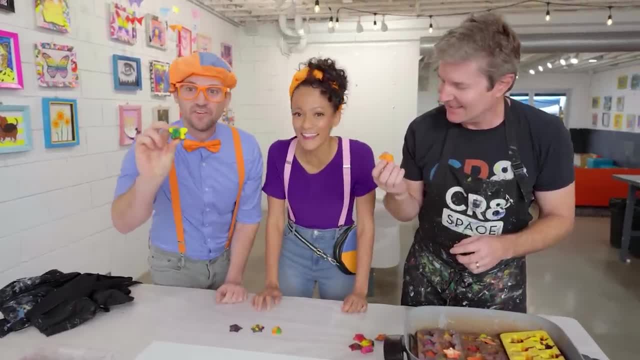 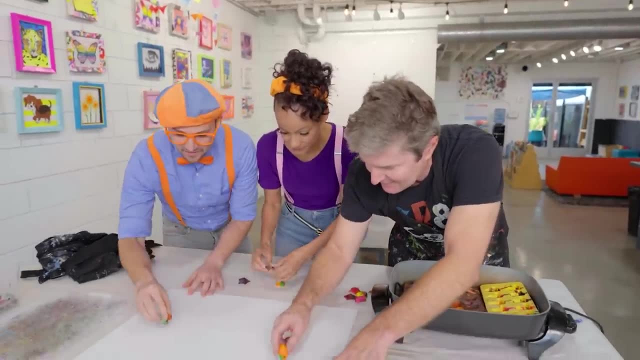 So cute And so colorful. Yeah, they look great. Wow, You guys want to try them out? Yeah, Yeah, Here, follow me ready, All right, Whoa, Whoa, Whoa. they do change colors when you use them. 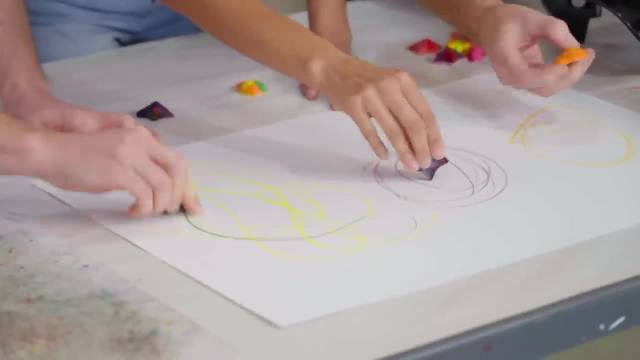 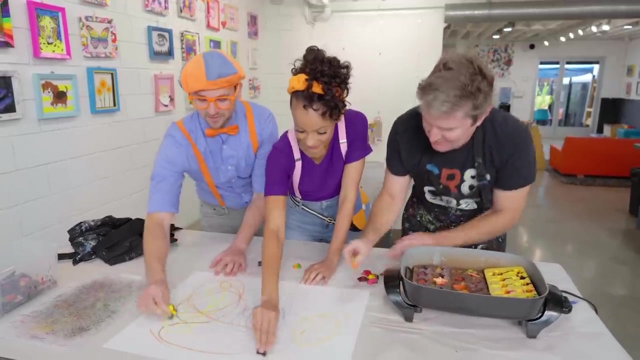 Whoa, Whoa, Whoa, Whoa, Whoa, Whoa. I can see blue and purple in mine. Whoa, Isn't that fun. Mine went from yellow to green to orange. Whoa, I can see yellow in mine now too. 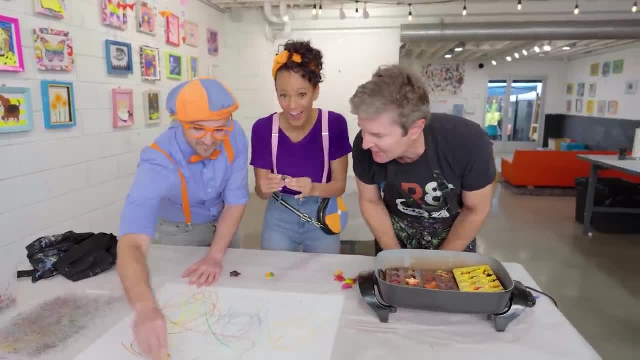 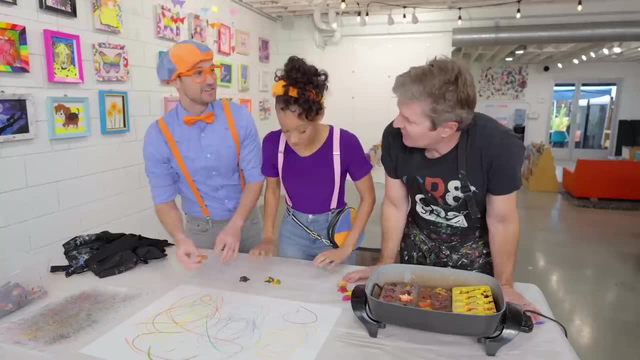 Woohoo, I love what you guys are doing. that looks fantastic. Whoa, So fun. That was so much fun making art today. Yeah, What else did you guys do at the studio? Oh Well, we made some really cool monster boxes. 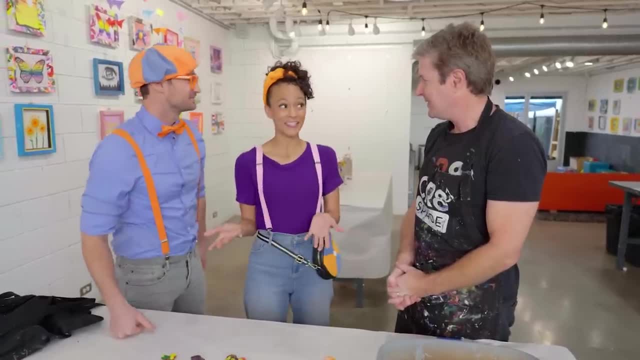 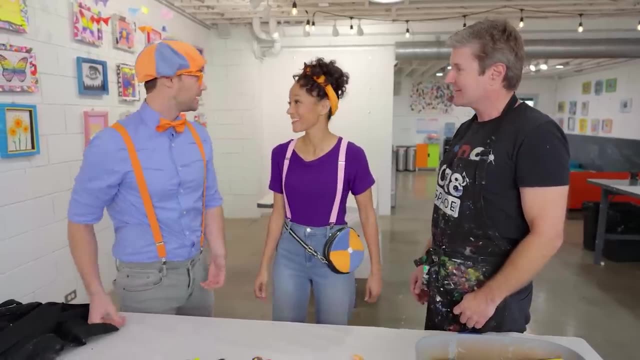 Yeah, I love monster boxes. Yeah, And we painted a canvas together. Great, Yeah, go ahead and clean this up if you guys want to go and see if your stuff's ready. oh yeah, maybe it's dry. yeah, all right, thank you so much. thanks for coming in. it was so nice to meet you guys. 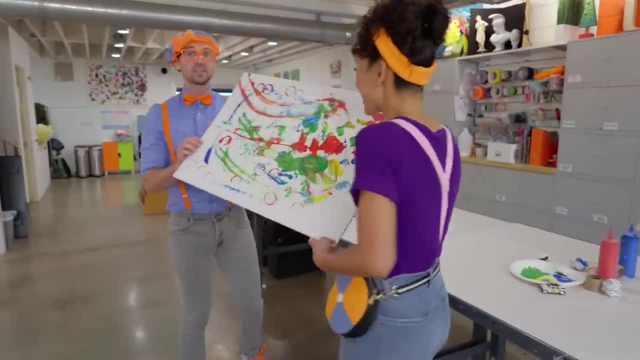 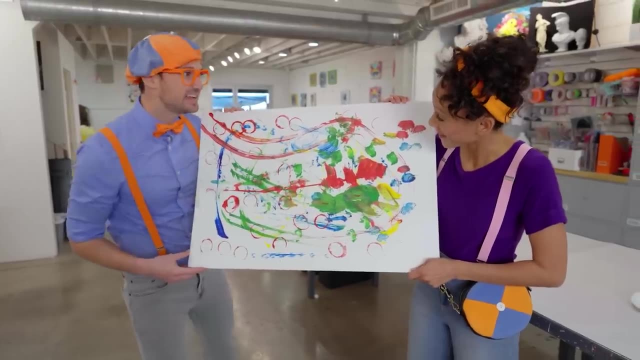 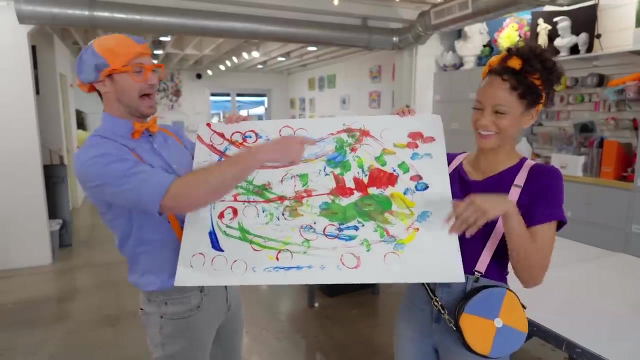 bye. wow, look it is dry. yeah, it looks really nice. oh yeah, i love the green and the tire tracks that you made. yeah, and here are the circles that we made with paper tubes. oh yeah, and you can't forget about my piece of tape. wow, should we go hang it up? yeah, let's do it all right. 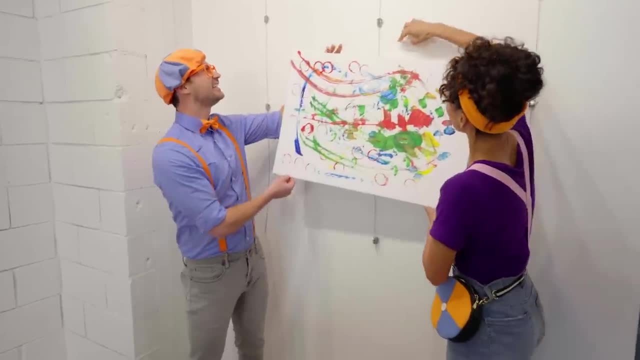 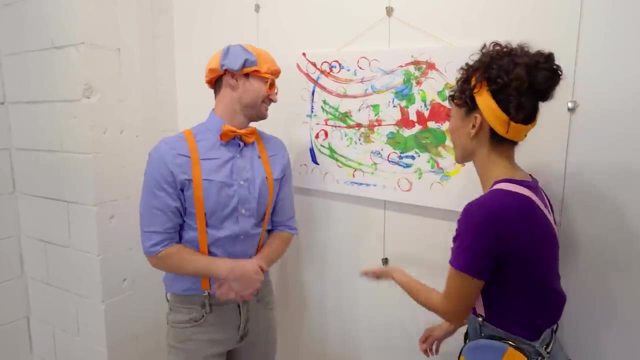 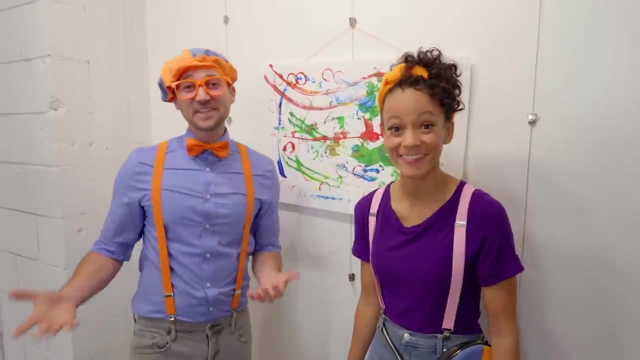 now everyone can see it. yeah, here we go. what a beautiful masterpiece. yeah, i really love all of the colors that we used and that we made it together. yeah, we did such a great job. yeah, i think so too. well, this is the end of this video, but if you want to watch more of my videos, all you have. 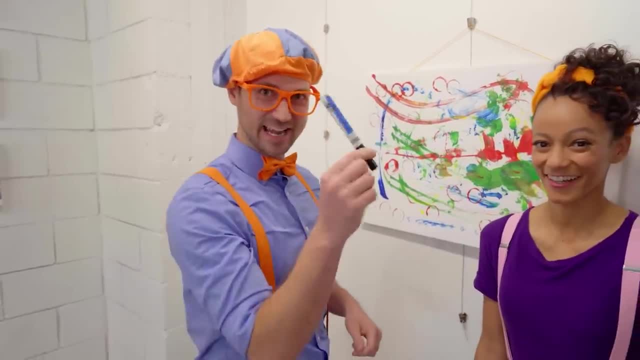 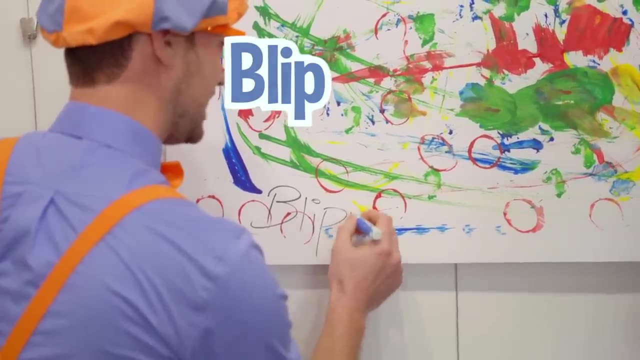 to do is subscribe to my channel and turn on the bell so you don't miss any of my new videos. subscribe to my channel and turn on the bell so you don't miss any of my new videos. do is search for my name. will you spell my name with me? yeah, ready, yeah, b l i p p i, blippy. 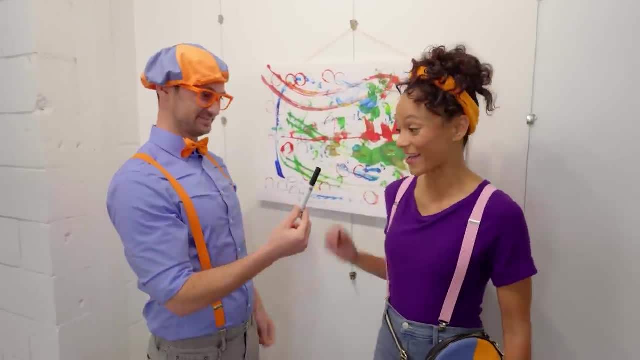 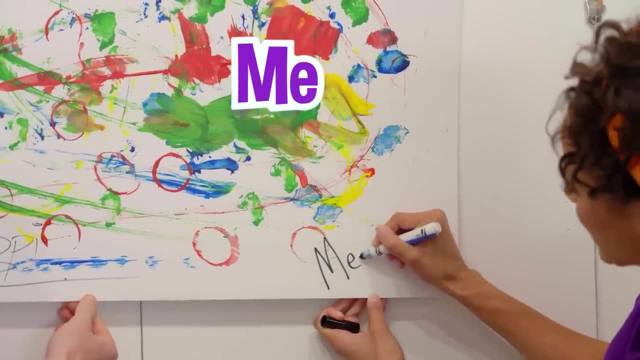 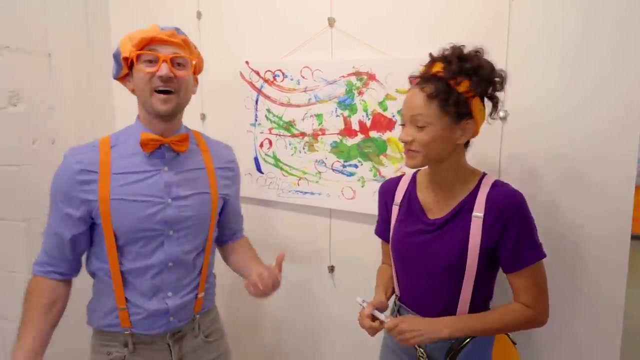 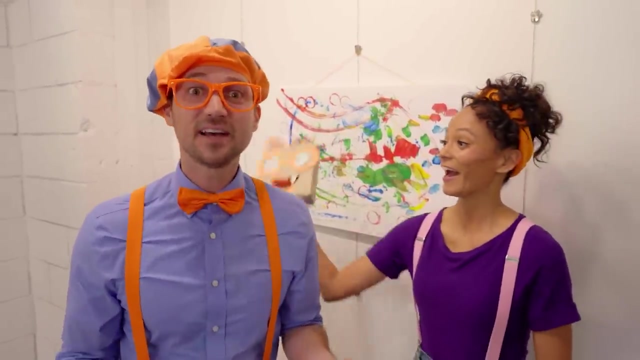 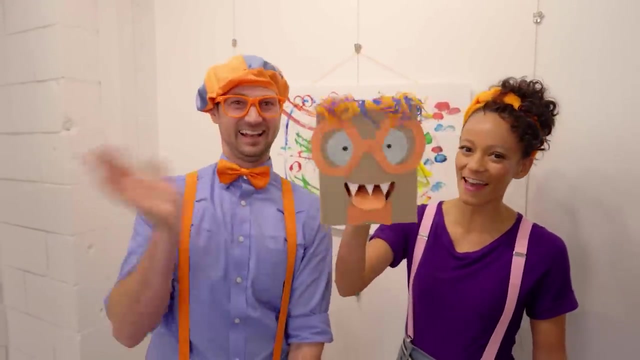 and if you want to search for me, you can spell my name: mika, you spell my name with me. awesome, what a fun video and it was so much fun making art today together. art is so much fun because it's all so unique. i love art too. blippy, whoa, hey, monster box. blippy, hello, hello. all right, see you. 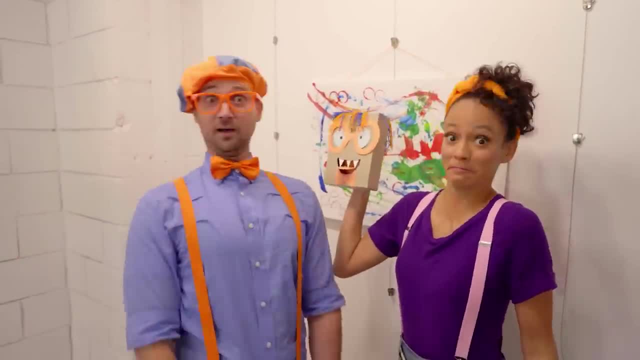 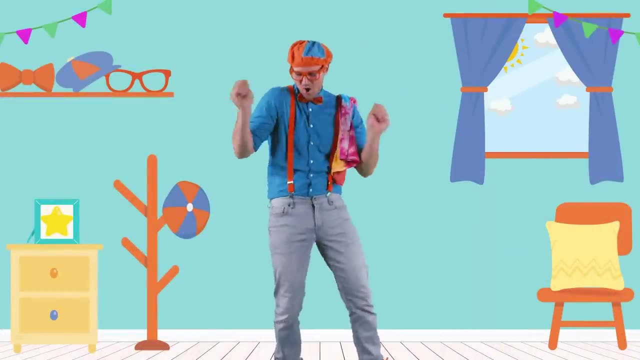 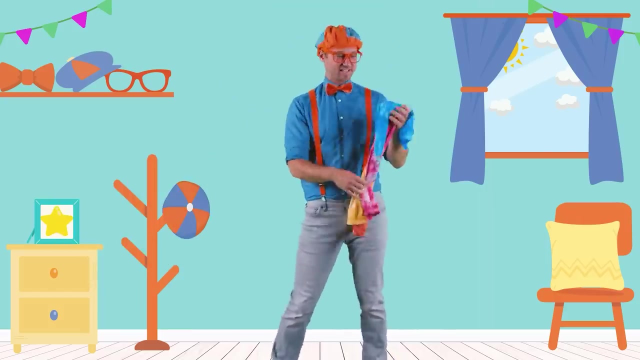 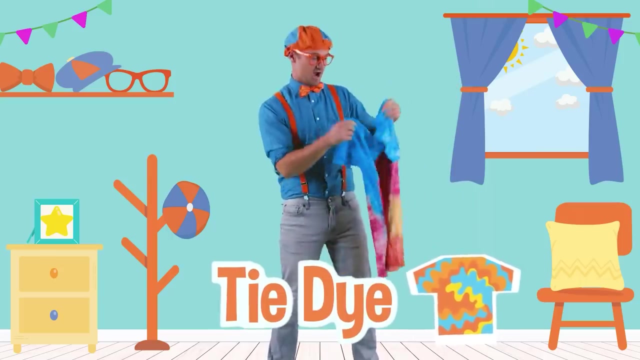 again. yeah, nice music. hey, it's me blippy, and i was just grooving to some tunes. check this out, though. do you see this? this is a tie-dye shirt, and today, you and i are gonna make a tie-dye shirt. wow, it's so colorful. 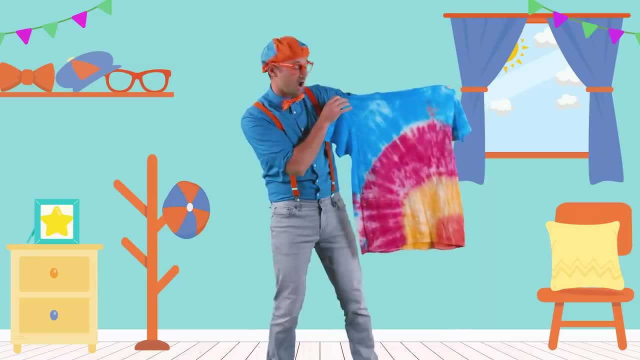 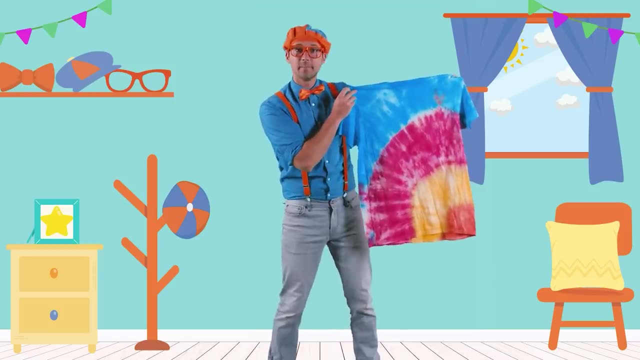 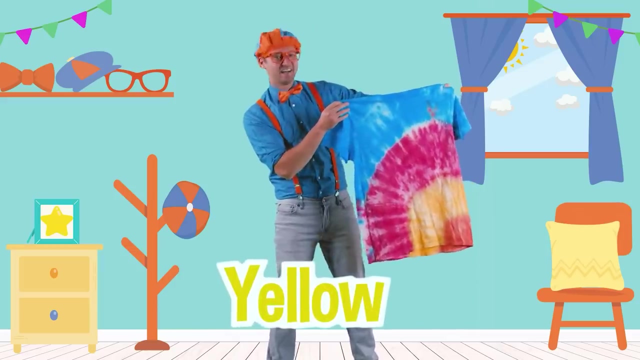 let's list all these colors. let's list all these colors. top there is the color blue. yeah, then below that looks like it's the color pink or red, pinkish red, and then we have yellow, like the color of the sun, and then we have orange at the bottom. do you see? 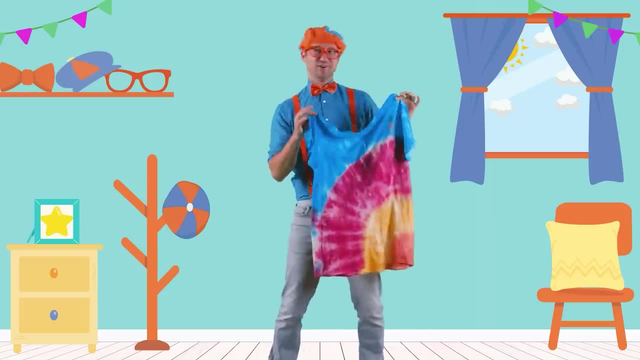 it. whoa, this shirt is so groovy. all right, let's go get some supplies and make our very own tie-dye shirt. whoo, this shirt is so groovy. all right, let's go get some supplies and make our very own tie-dye shirt. 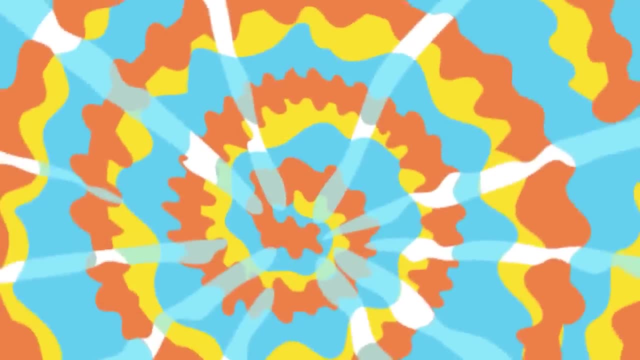 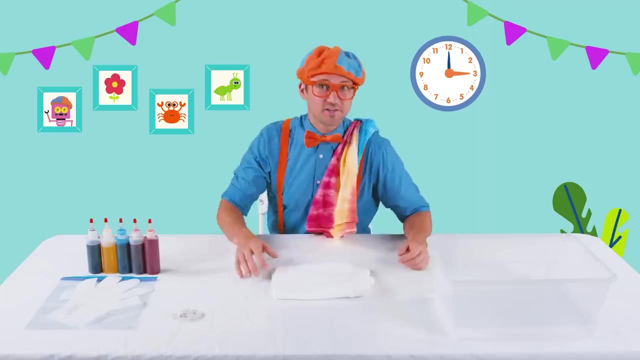 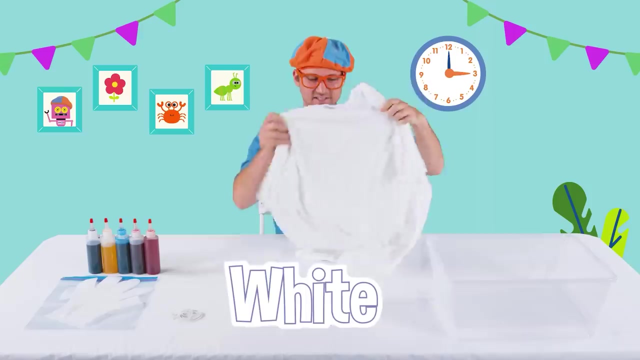 check it out. we have all the materials and supplies we need to make our tie-dye shirt. all right, we don't need this because we're gonna make one. so first you start with a white t-shirt- yeah, like this, see. and then you take a die- yeah, let's see. 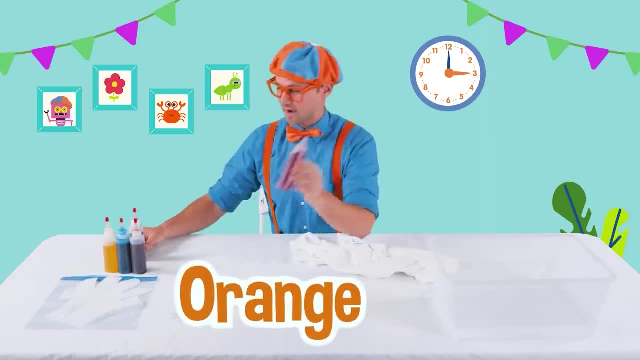 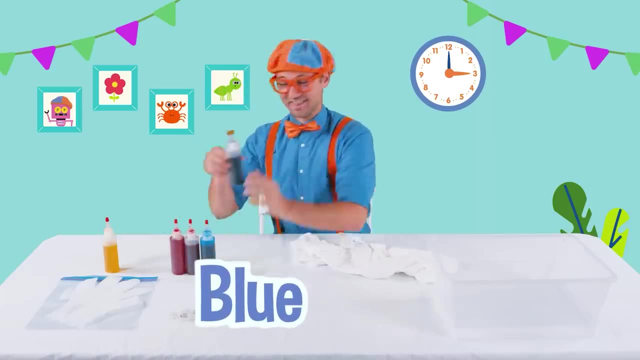 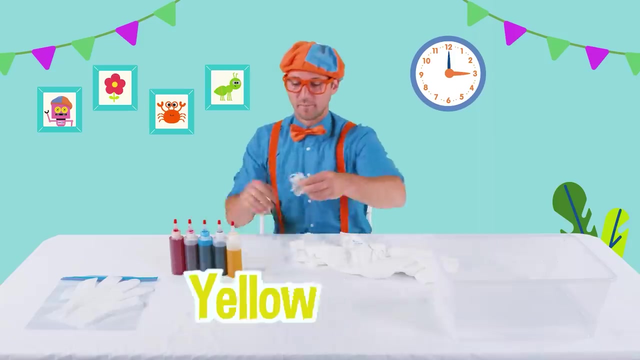 now, that's according to this person. i made enough bags. now let's switch to a fabric tie. uh, fabric die. this is the orange fabric die, this one is red, this one is blue, this one is purple and this one is yellow. and then we have some rubber bands. 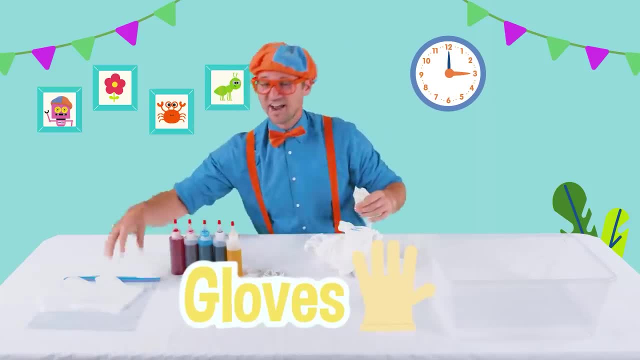 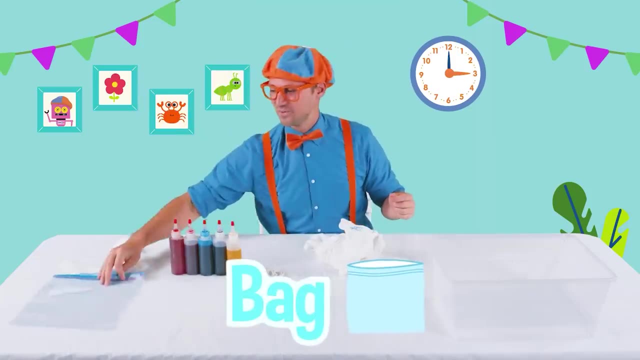 and you tie the shirt really tight, then you spray the die on it, but you have to wear your gloves And then we have a bag for later. I'll show you what that's all about. And the water. Okay, so first step, 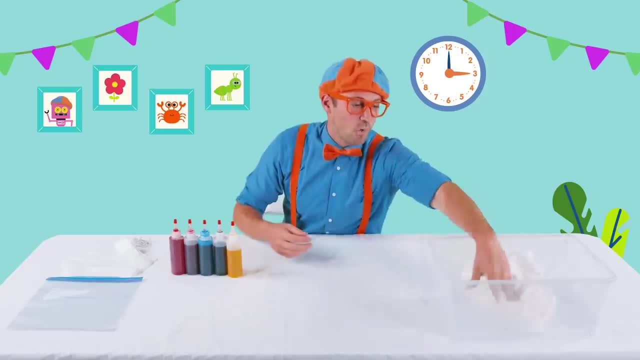 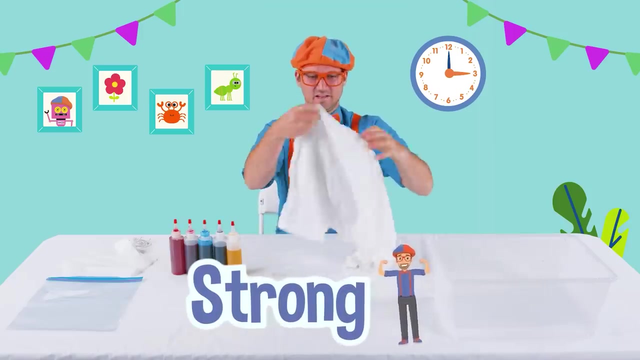 We need to get the shirt wet, Just like that. Let's get it nice and wet. Wow, The water's really cold. Okay, squeeze out all the water. Whoa, We're so strong. All right, And then let's lay the T-shirt out on the table. 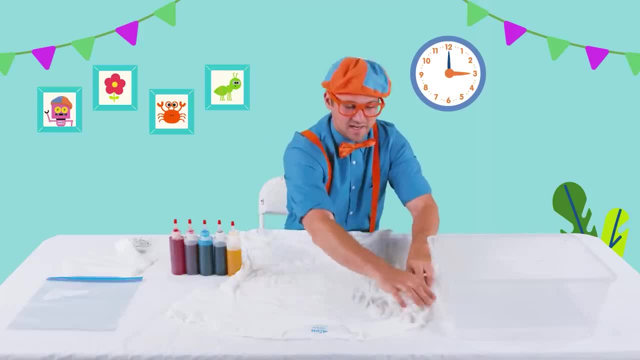 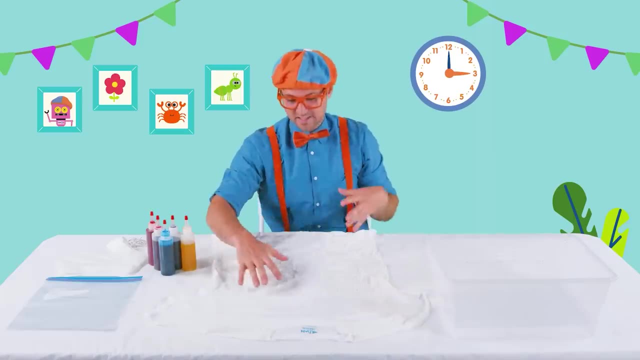 Yeah, And the cool thing about tie-dye is you can do so many different designs, And it's all about how you twist and crunch the shirt and wrap the rubber bands around it. So let's do a swirl. I love it. 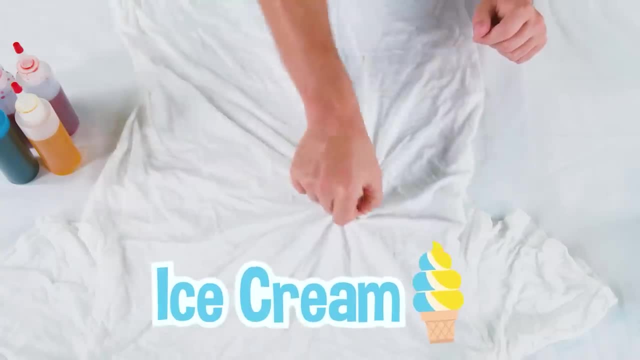 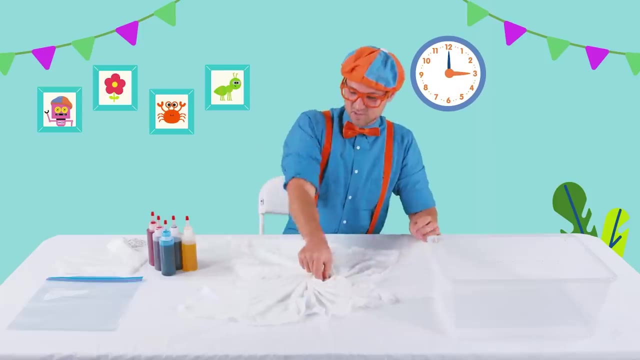 I love swirls. Yeah, kind of like ice cream swirls. I love ice cream. Okay, here we go. So you just twist it, swirl it, Oh perfect. Wow, I'm so excited to pick the colors. 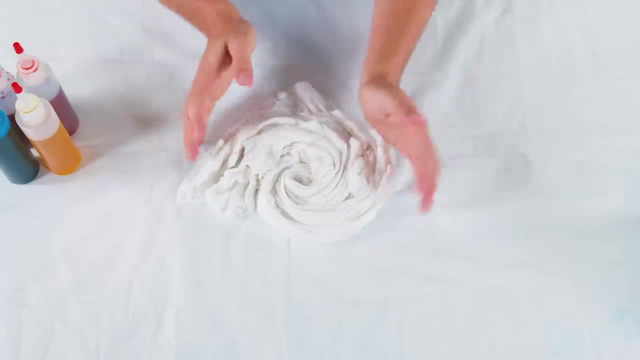 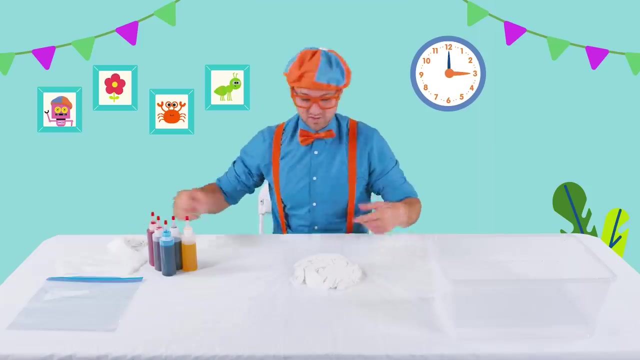 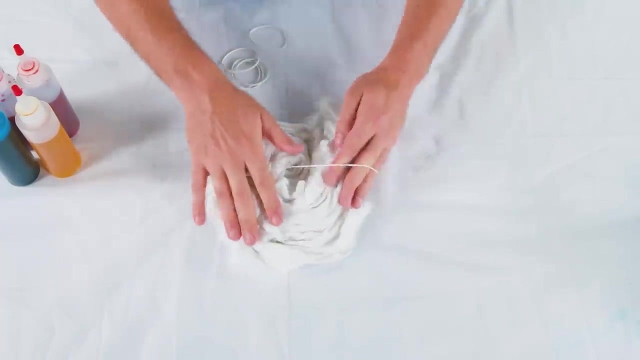 Okay, there we go. And then you have a nice bunched-up shirt. You could even bunch it, But I chose and swirl it. And then you take these rubber bands and wrap them around the top and the bottom of the shirt. 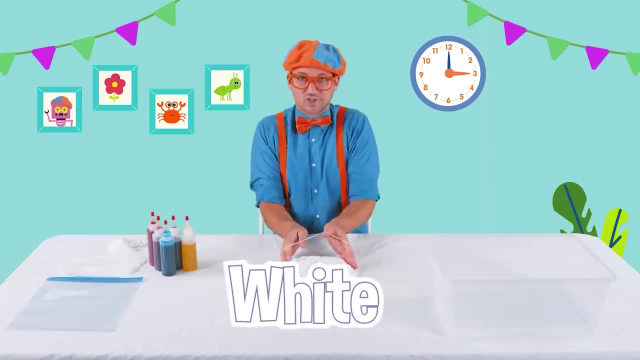 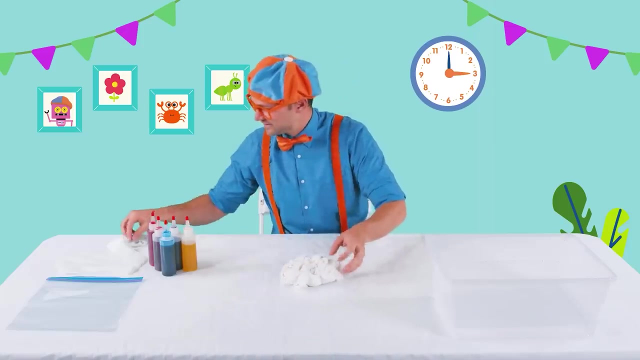 Just like this. Yeah, This white shirt is gonna be so colorful. All right, There's two rubber bands. Here is three rubber bands. Perfect, This is looking so good. And then there's the fourth rubber band. Wow, Will you count to four with me? 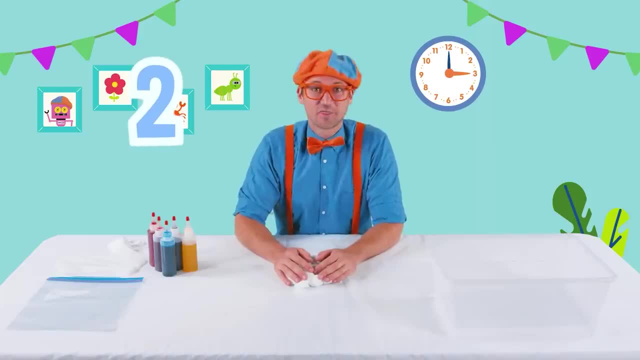 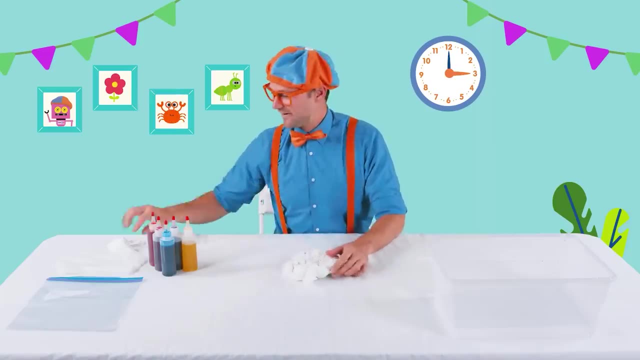 Ready. One, two, three, four. Good job, All right, Now we get to pick our colors, But remember, let's put on our gloves. Okay, here we go. One glove Okay. One glove Okay. 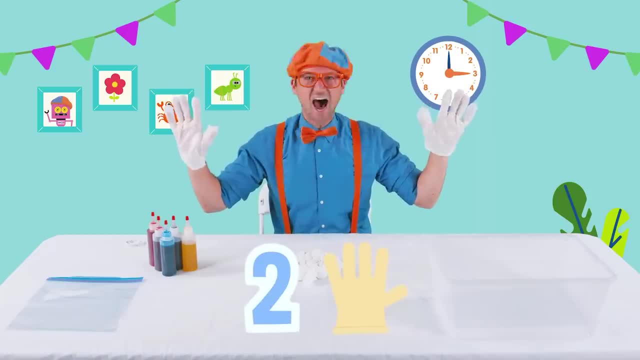 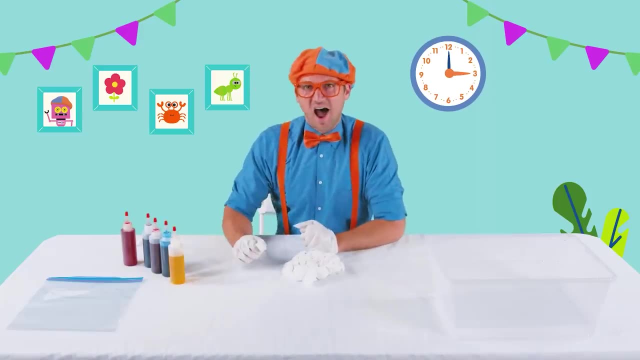 Two gloves, One, two. All right, Let's see, We have a lot of colors. I know I think I'm gonna choose two colors, My two favorite colors. Do you know what colors they are? Yeah, I bet you do. 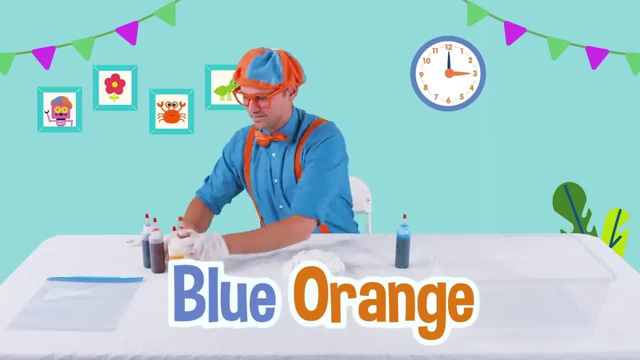 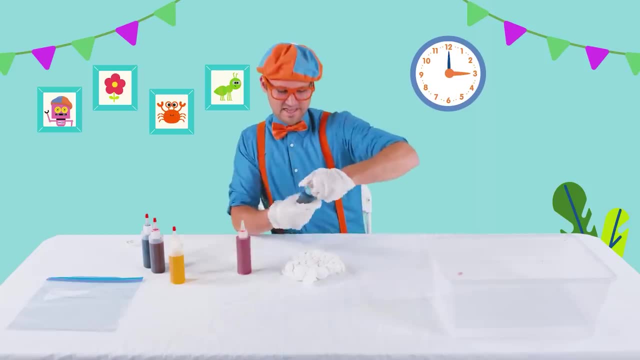 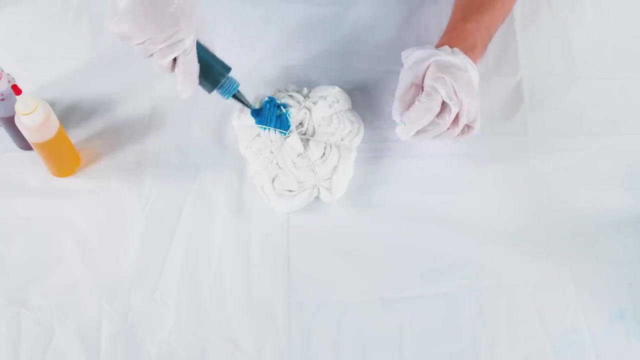 Yeah, blue and orange. All right, Here's the two colors. And then take the cap off And then you get to squirt the shirt in whatever way you want. I'm gonna squirt some blue right there. I'll skip some and squirt some blue right there. 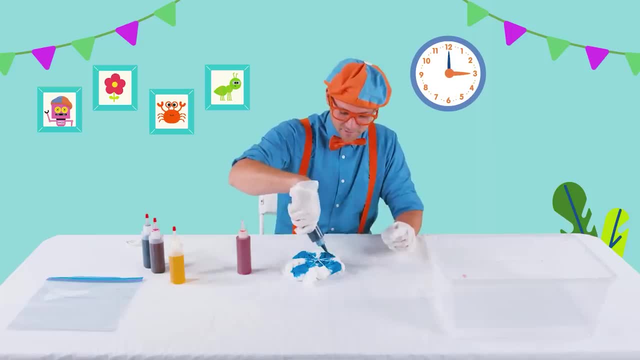 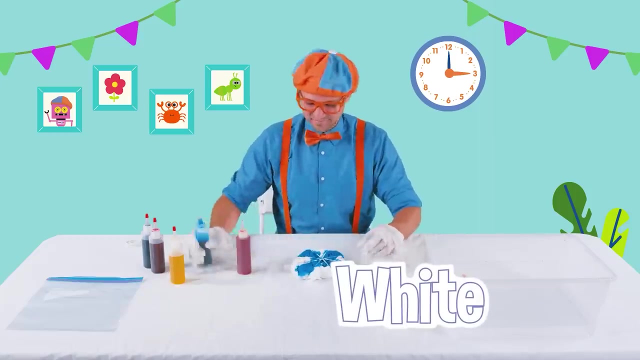 How about some blue right there And some blue right there? Wow, The shirt was all white, But now what color is it? Yeah, there's two colors: Blue and white. Yeah, All right, Let's give it a little more. 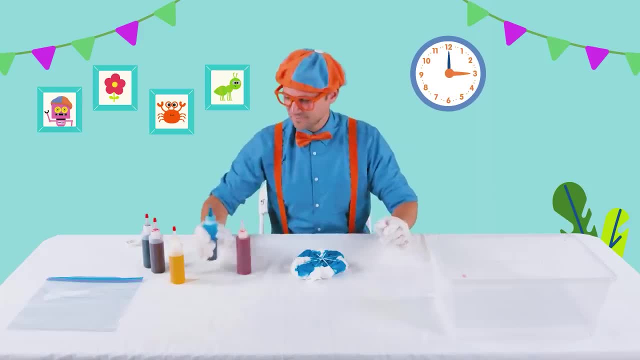 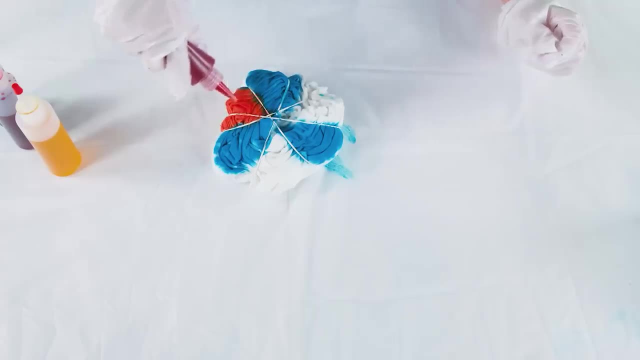 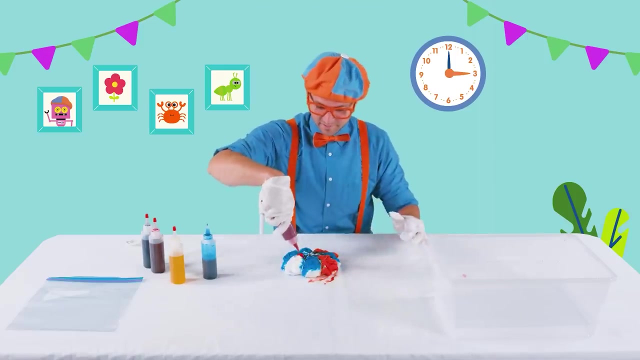 Wee, wee, wee. All right. So then the other color, like I said, is orange. So let's squirt that white and get it nice and orange. There we go. Wow, We are doing so good. There we go. 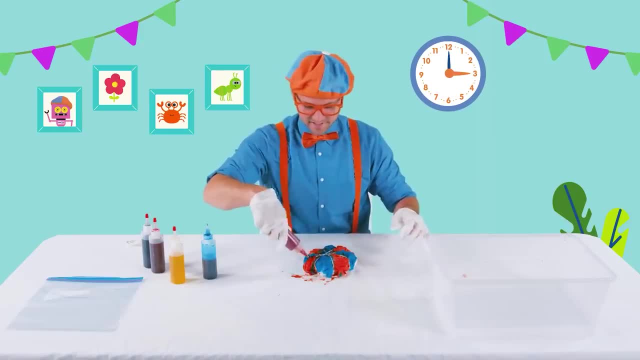 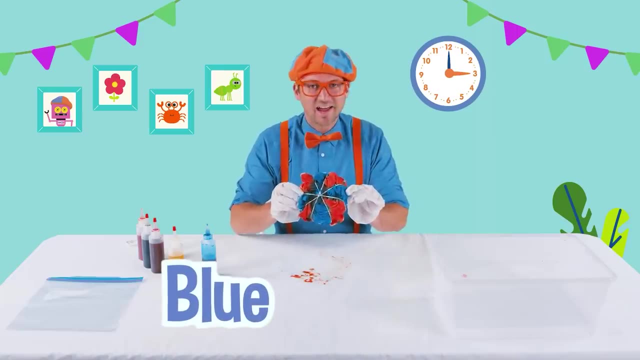 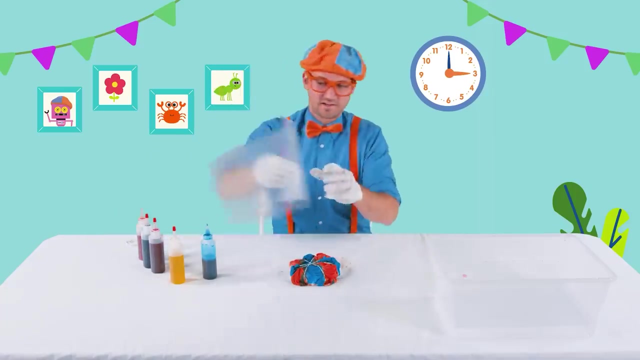 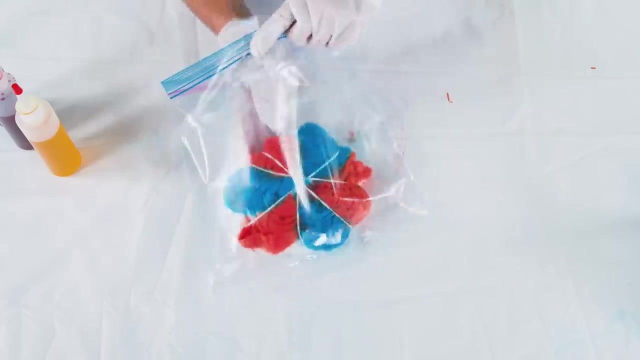 Perfect, Wow, Amazing, Wow. This looks so good. Do you see it? We have blue and orange, All right, Set that down. And now you take the big plastic bag and put the shirt in there And close it up. 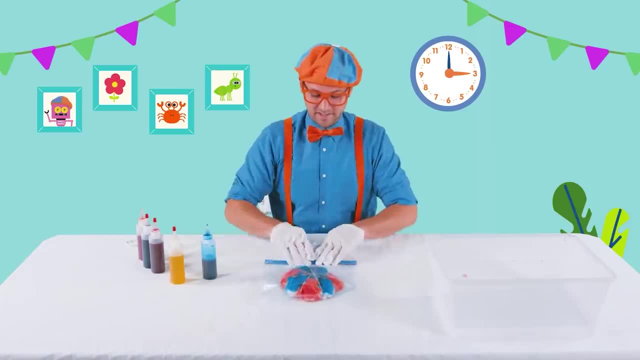 And now we get a weight, But you have to keep it in here for at least six hours. You can even do it up to ten. You can even do it up to 24 hours if you wanted to. The longer you keep it in this bag. 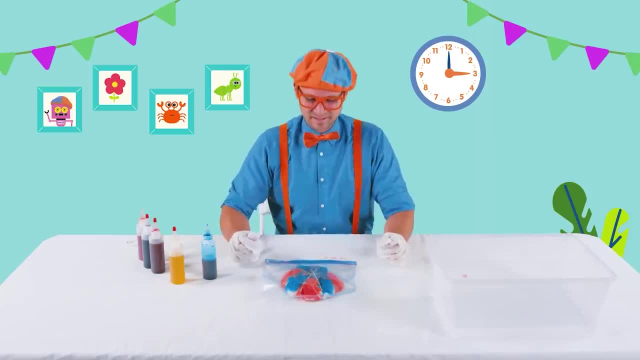 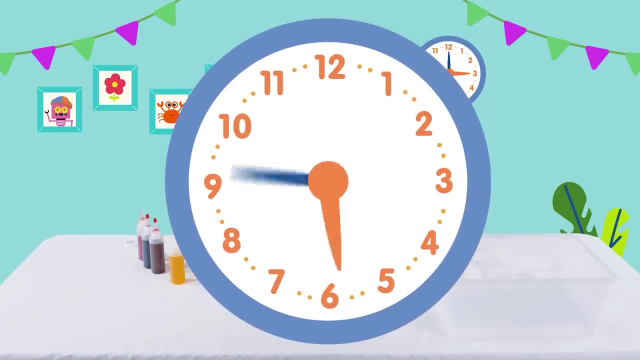 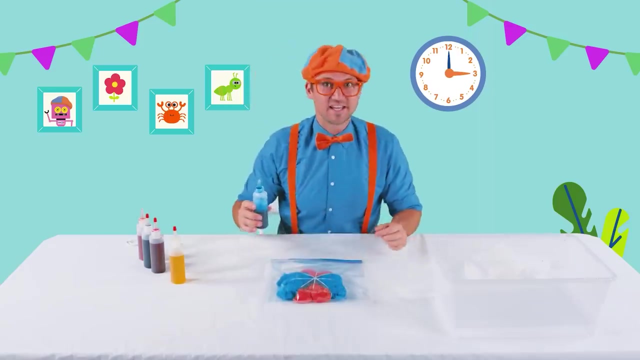 the darker and more vibrant the colors are going to be. I think we should probably wait eight hours. So let's wait. We're almost done waiting, But I think what we should do is mix two colors and see what color it makes. First let's take our blue. 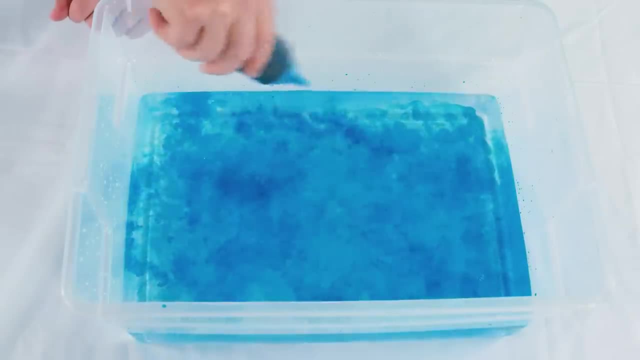 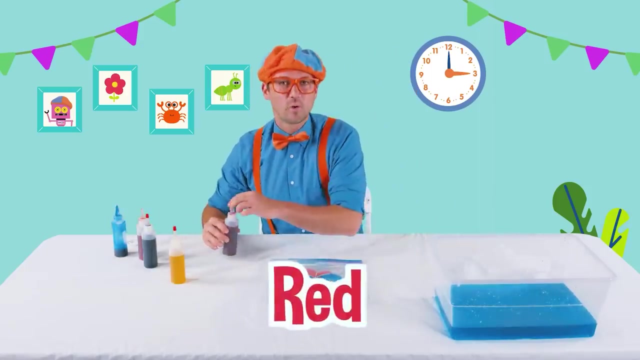 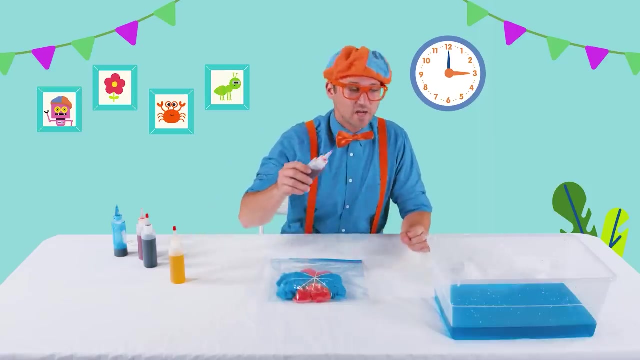 Whoa, Do you see that? Whoa, That's awesome. Wow, Blue water. And then let's take how about red? Hopefully it doesn't spill on me, because I don't have my gloves on anymore. All right, here we go. 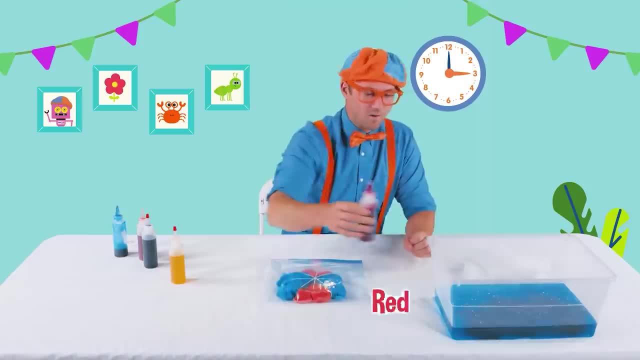 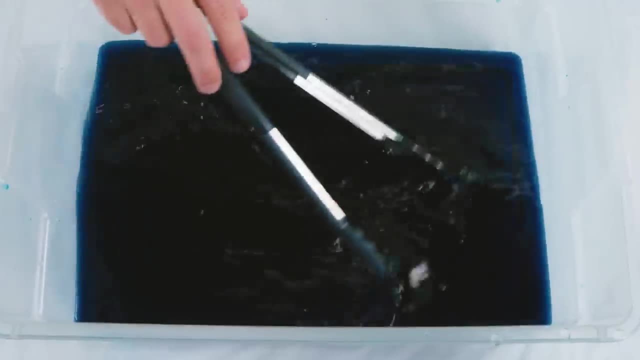 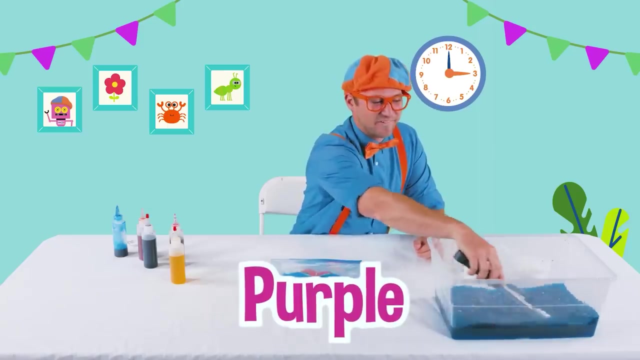 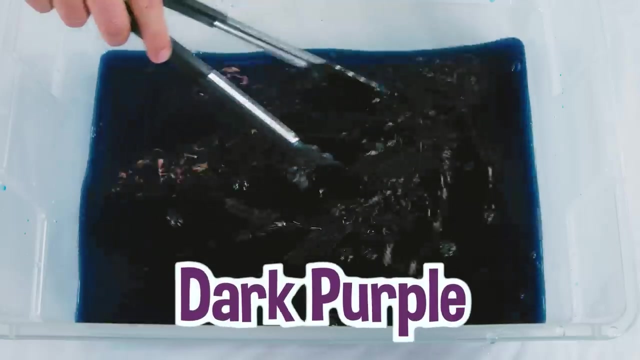 Blue and red. Whoa, What color is that? I have my mixing tongs, Wow, Yeah, Blue and red make the color purple. Whoa, Let's put a little bit more red in there. Wow, Now it's a dark purple. 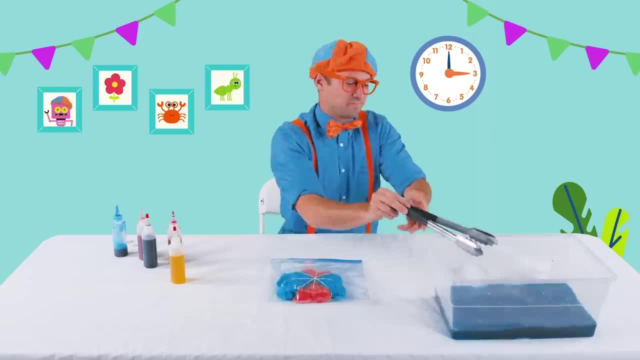 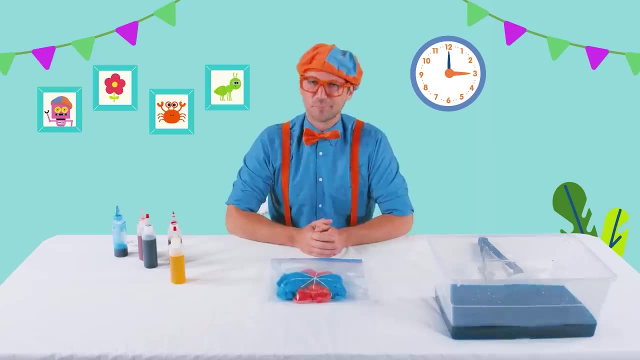 Whoa, That's fun. Okay, Well, I think our t-shirt has been in here for long enough. It's been about, yeah, multiple hours. So now I'm going to go and get it. I'm going to go take this to the sink, take the rubber bands off. 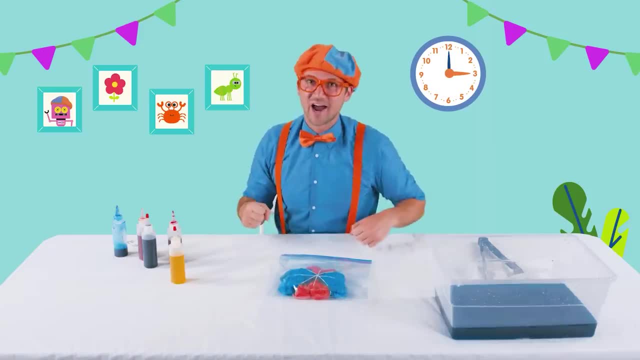 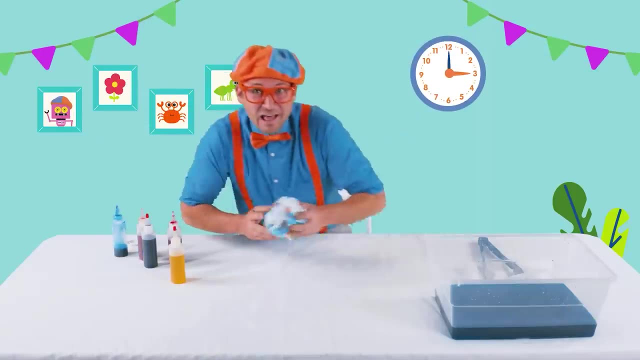 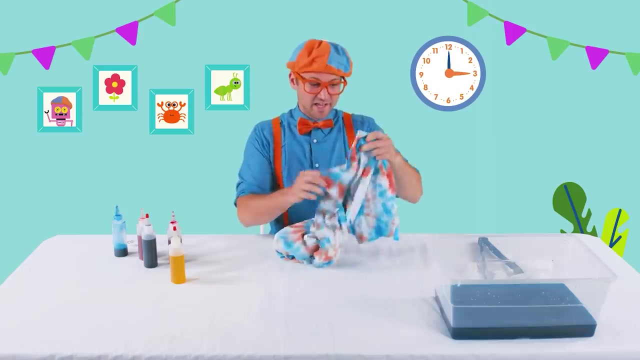 and rinse it off, and then I'm going to go put it in the dryer. I'll be right back, okay, Whoa, This is awesome. Our shirt is complete. Wow, All right, Here it is, Do you see it? 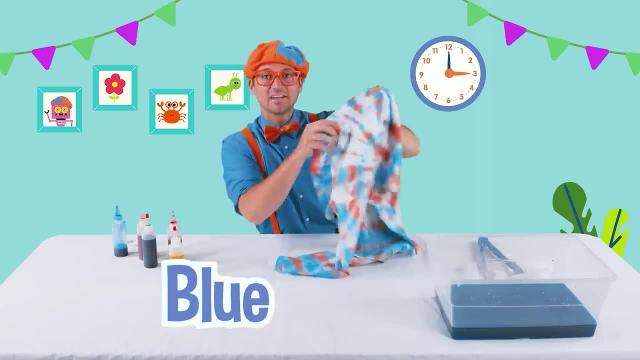 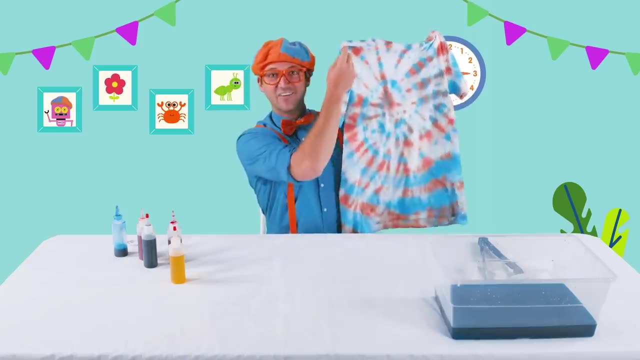 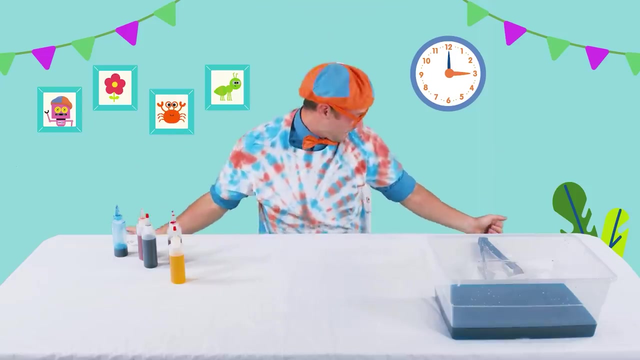 Wow, Yeah, It's blue and orange. Okay, Can you see how it where? I swirled it Right about there. Whoa, It's so cool. Time to try it on. Wow, How do I look? That was awesome. 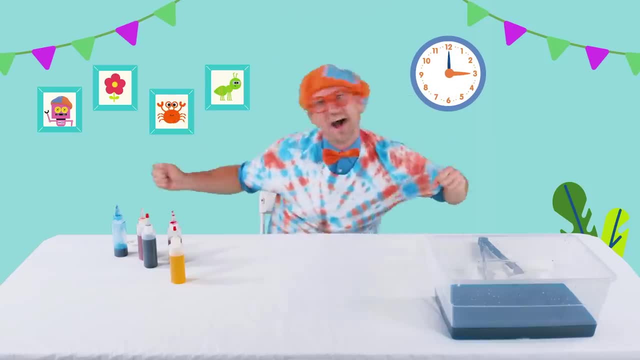 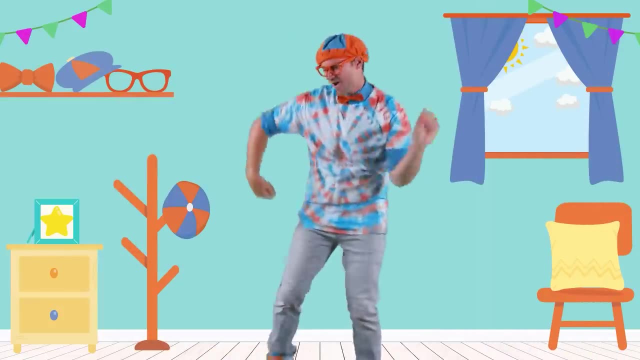 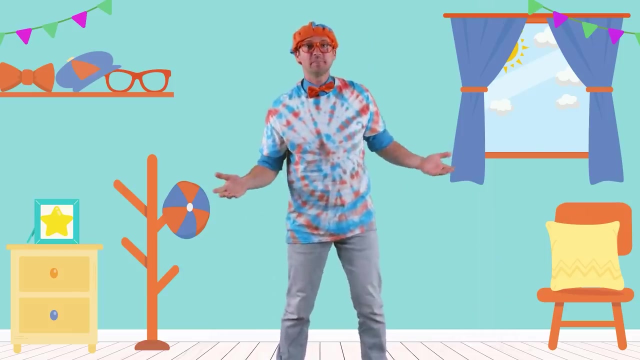 I love making tie-dye shirts. Woo Yeah, Woo hoo hoo, Woo hoo hoo. I sure do love tie-dye shirts, Tie-dye shirts. Whoa, Maybe now at home you can make your very own tie-dye shirt. 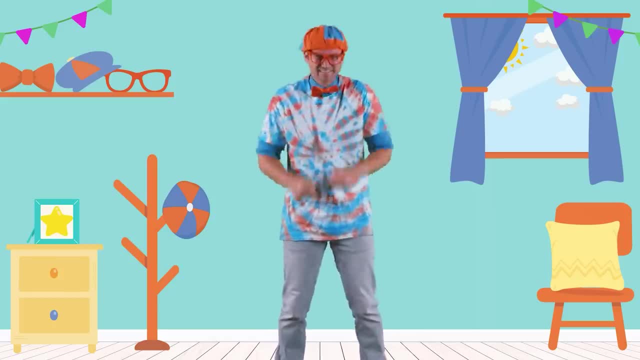 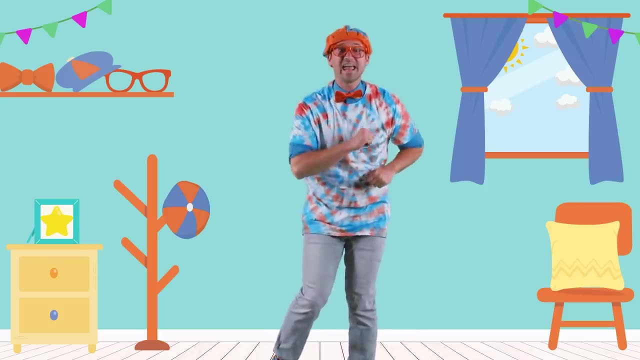 I am so excited to see the creation that you make. All right, Well, this is the end of this video, but if you want to watch more of my videos, all you have to do is search for my name. Will you spell my name with me? 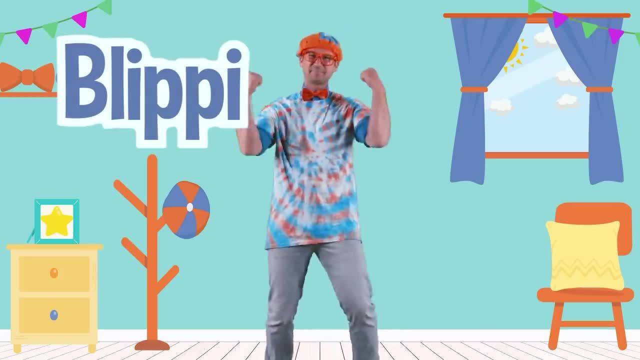 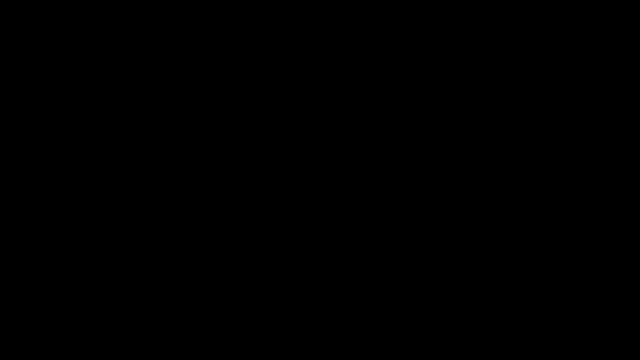 B-L-I-P-P-I. Blippi, Good job, All right, See you later. Woo hoo hoo. Woo hoo hoo. Oh, hello, It's me Blippi, and today we're on Amy's Playground. 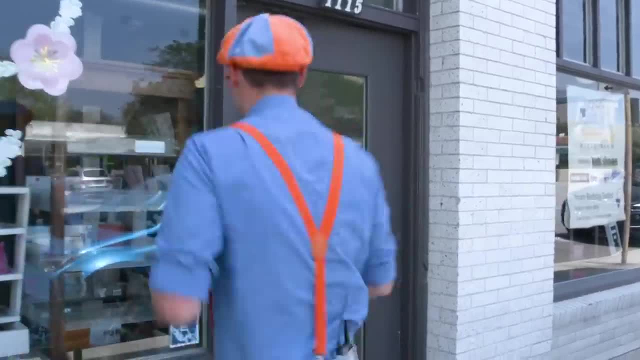 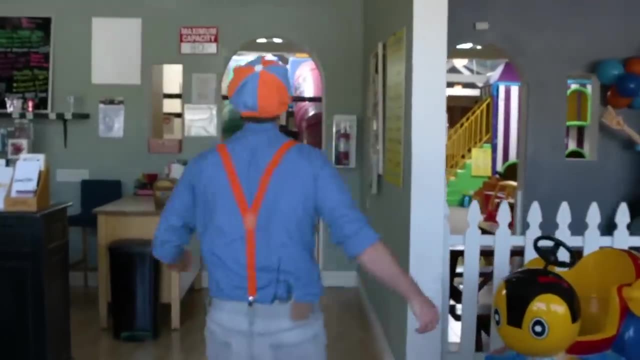 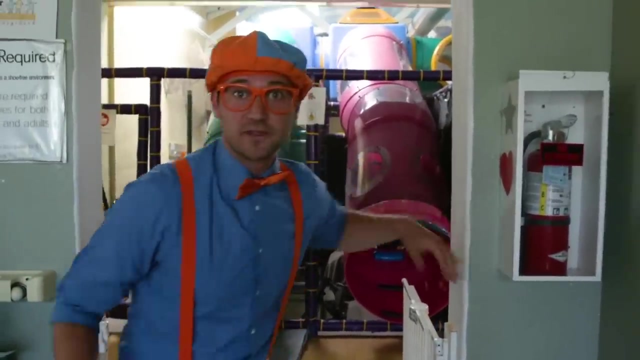 in South Pasadena, California. Come on, We're going to learn our colors. Whoa, Wow, This place is so cool. Whoa, We can't go past here without taking off our shoes. Here's one shoe And here's two shoes. 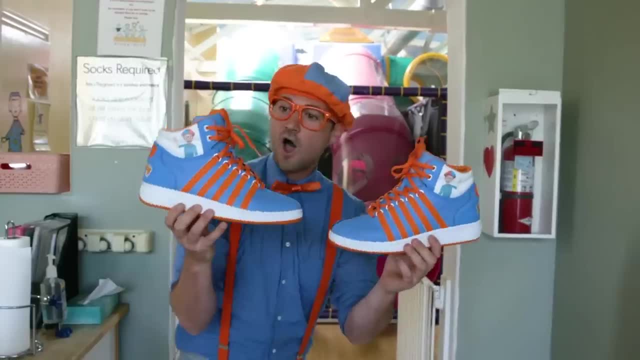 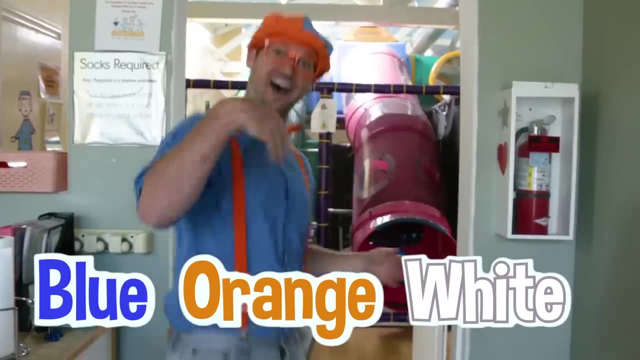 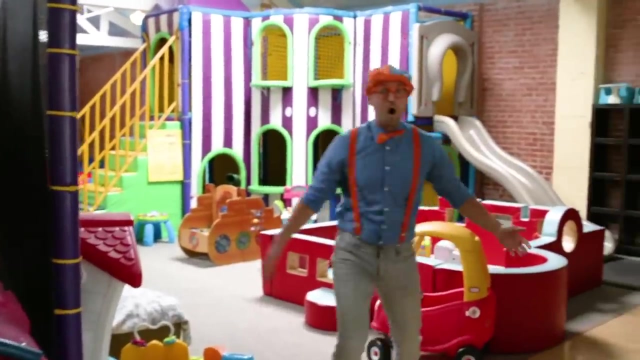 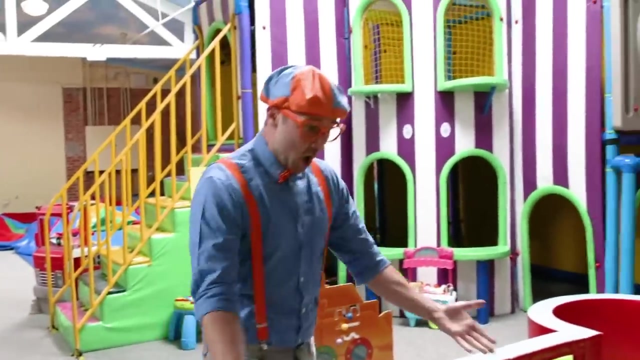 Hey, what color are my shoes? It looks like there is blue, orange and white. Woo hoo, Let's go. Whoa, This place is so colorful. Whoa, I love playing around here. Oh, this is pretty colorful. 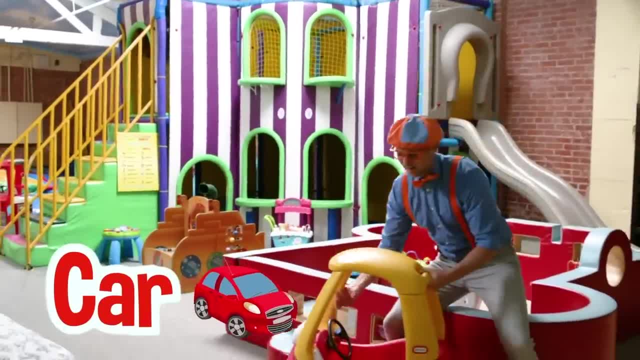 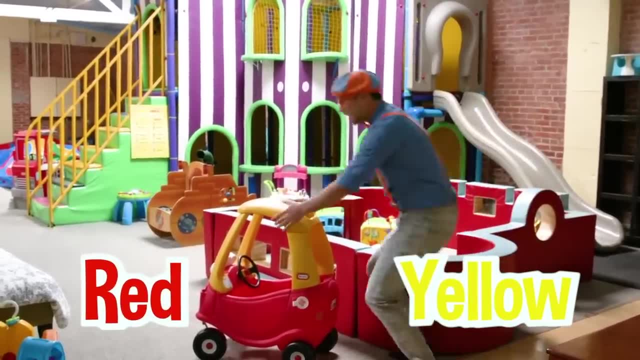 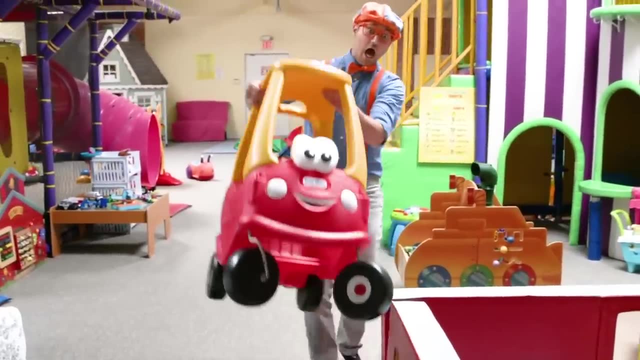 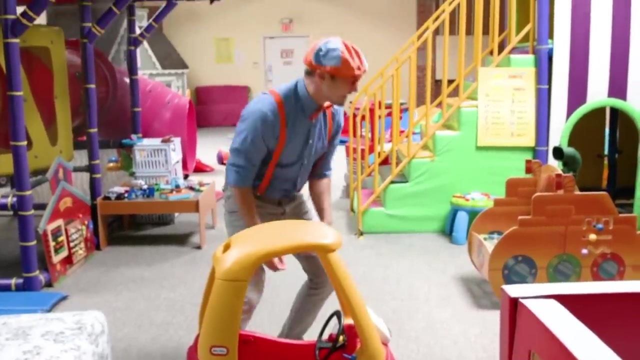 Whee, Whee, Whee. Look at this car. This car is the color yellow and the color red. Here we go, Whee, Whee, Whee, Whoa, Whoa, Whoa, So silly. Oh, what's in here? 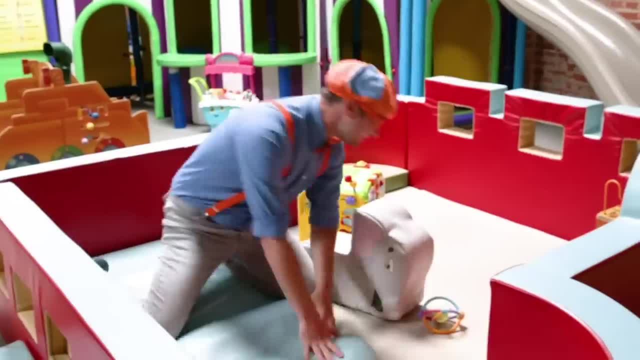 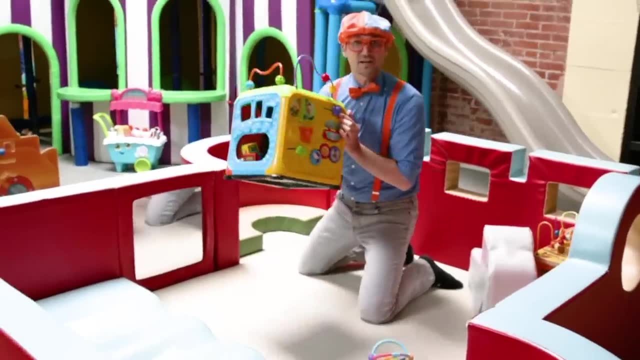 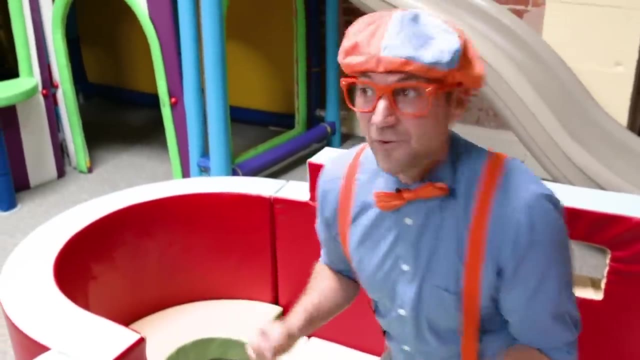 Whoa, It's so soft in here. Whoa, Whoa, Whoa. Hey, look at this. This box has so many colors on it. There's so many colors to name. Let's go continue to explore. Whoa. 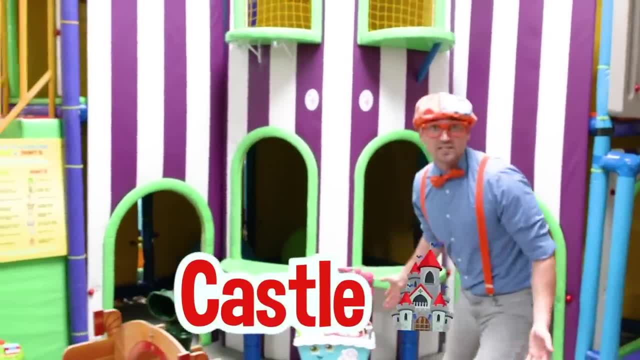 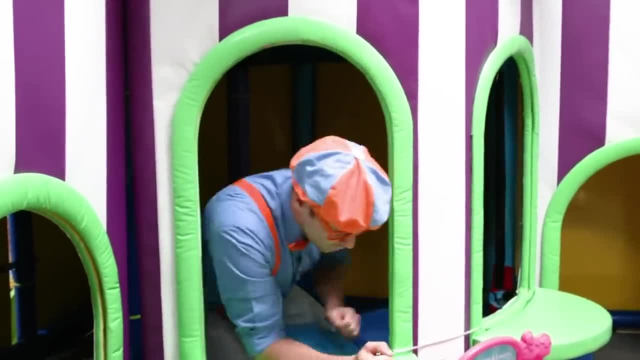 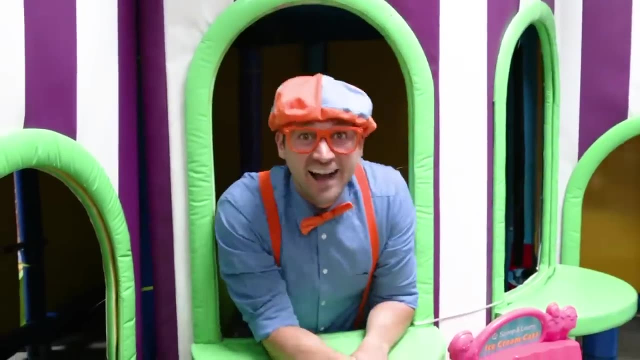 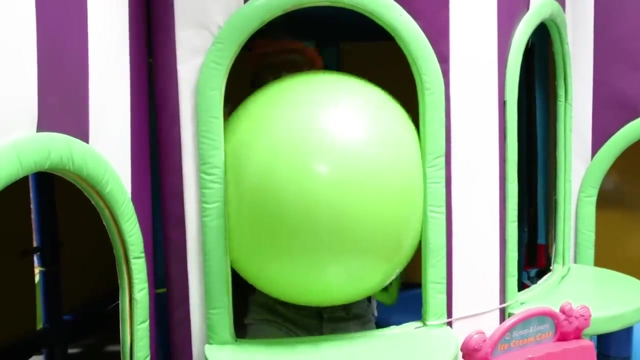 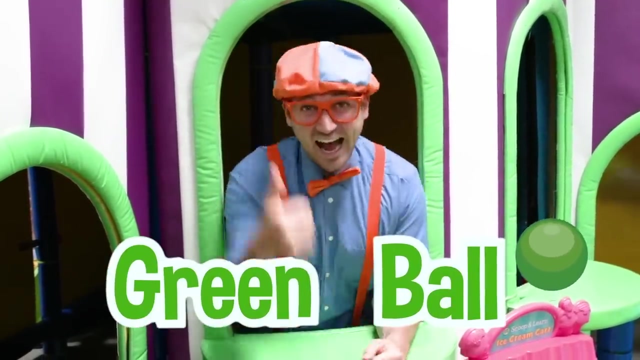 Whoa, It's like a castle. Let me go inside. Hello, Whoa, Let's take a look at this out. Whoa, That ball was the color blue. Hey, here's another one. That ball was the color green. 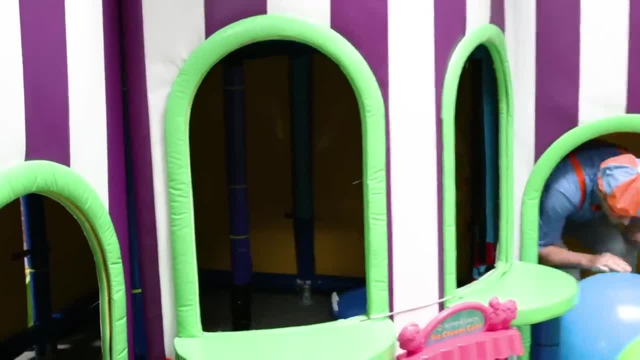 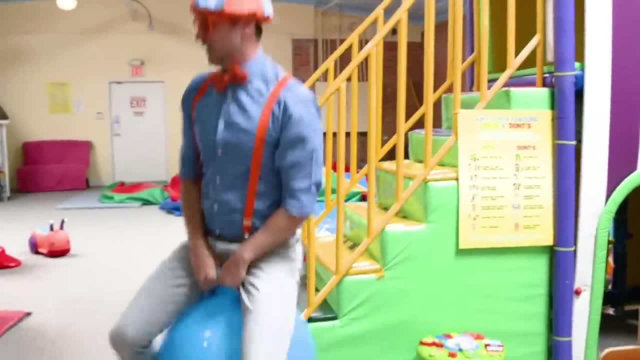 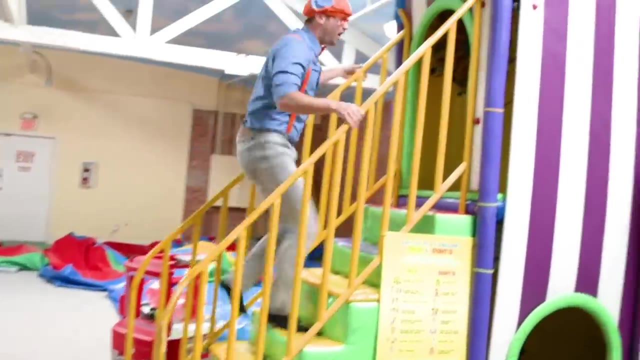 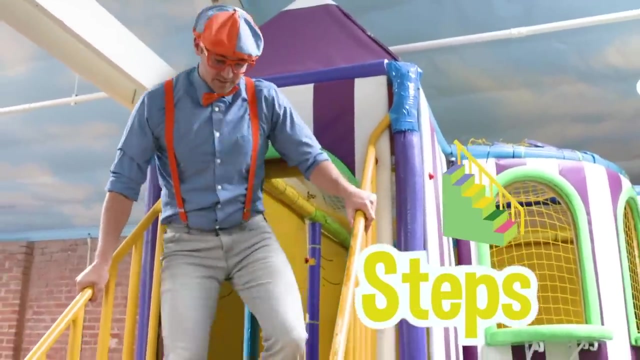 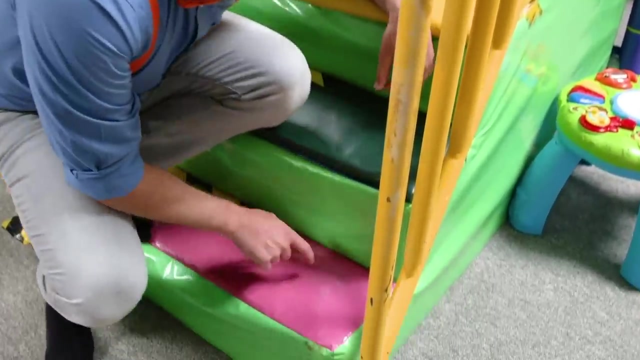 Good job. Whoa, hey, Boing, Whoa, Whoo, Whoa, whoa. wow, the castle is so tall. whoa, hello down there. hey, whoa, look at these steps. wow, do you see the colors? look at this color. what color is this? this is the. 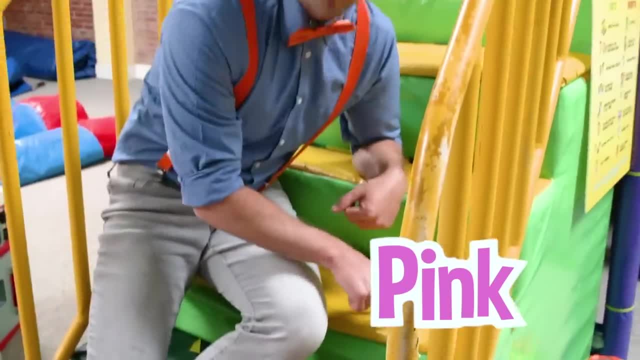 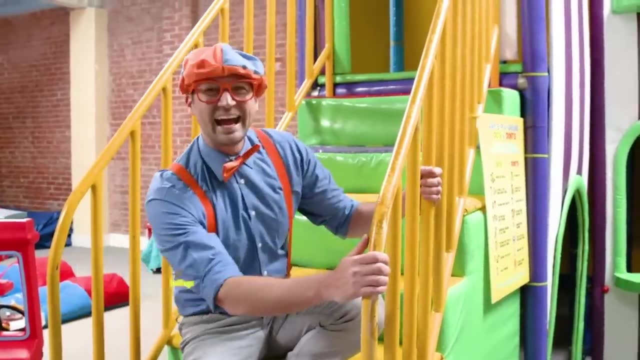 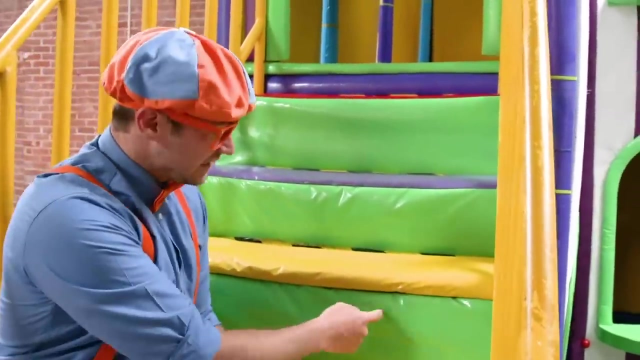 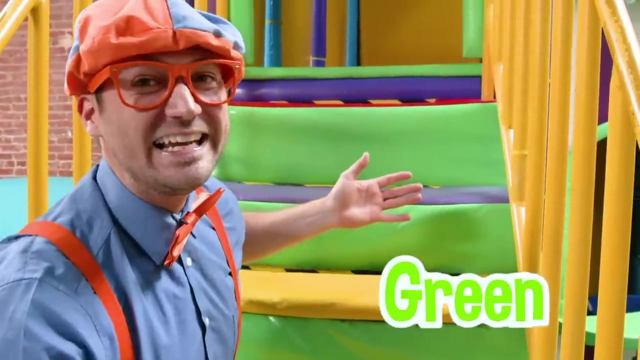 color pink, this color right here, yeah, the same color as the railings. what color is this? yeah, the color yellow. and right here, we learned this one already. this, this and this, yeah, these are all the color green. 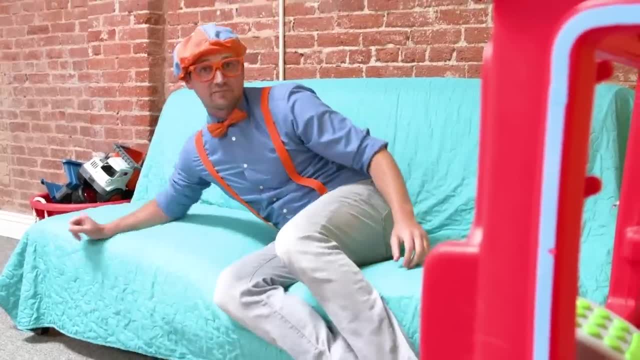 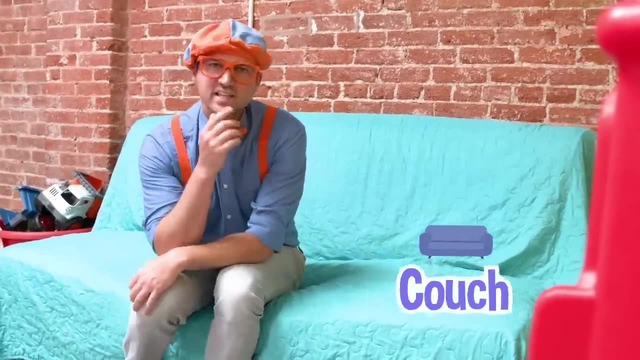 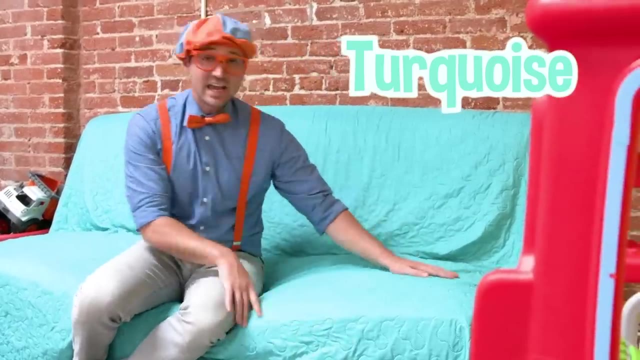 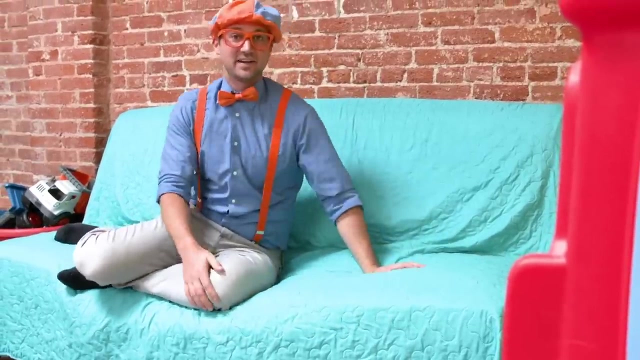 Oh wait, a second. no time for napping. but this is a nice comfy couch. you see what color it is? hmm, this is an interesting color. this color is the color turquoise. wow, it's kind of like a blue and a green mixed together. woohoo, but no time for napping, it's time. 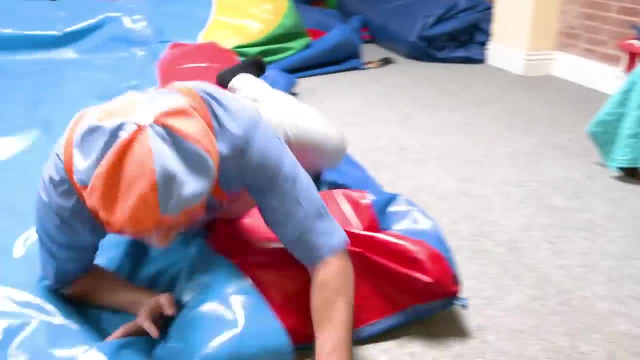 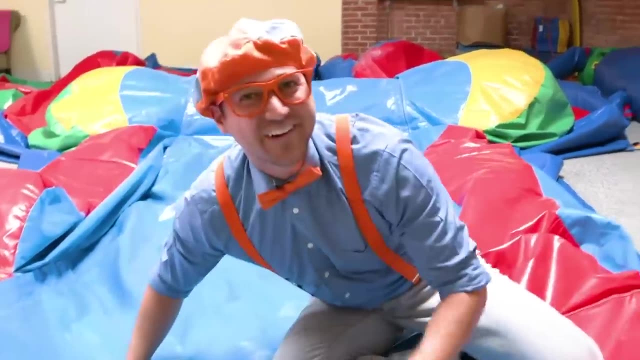 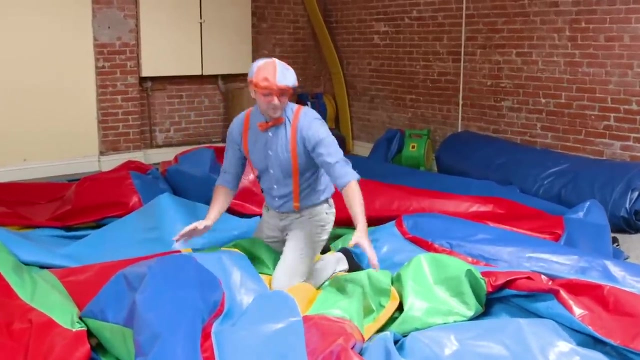 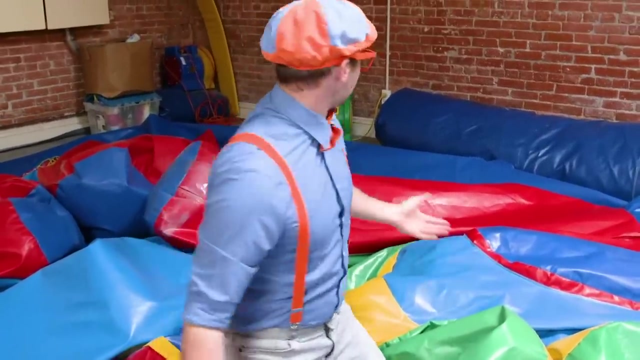 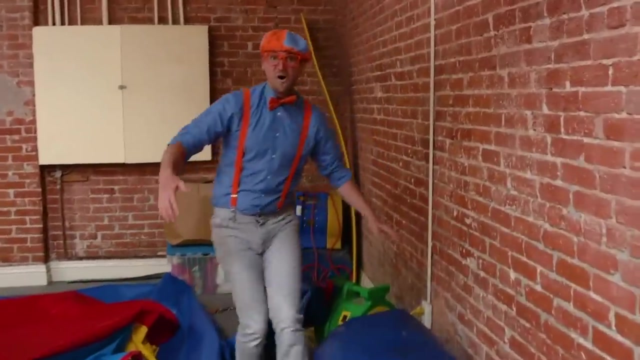 to do some rolling. woohoo, whoa, whoa, I love rolling around. this is so silly, it's so colorful and I think it's deflated. hmm, how do we inflate this? wait over here. whoa, this is the green. whoa, whoa, whoa, whoa. 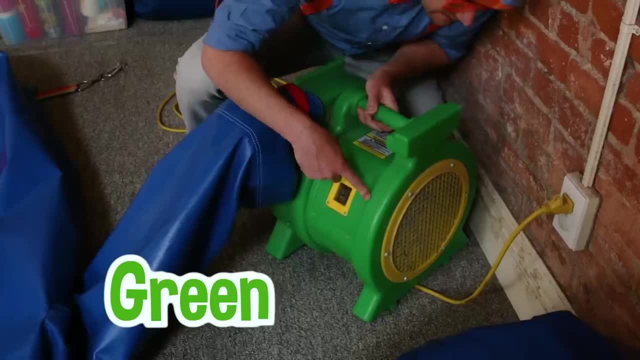 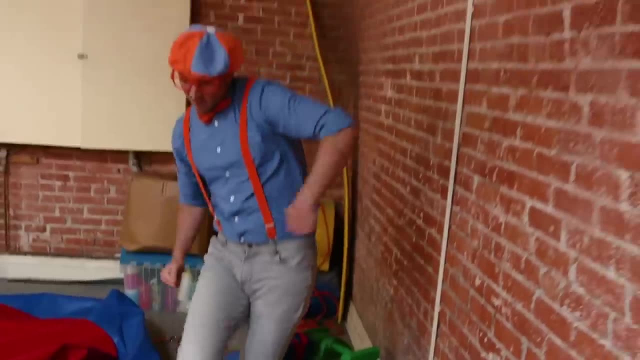 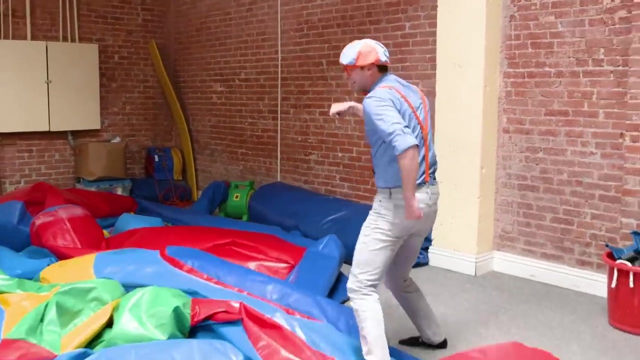 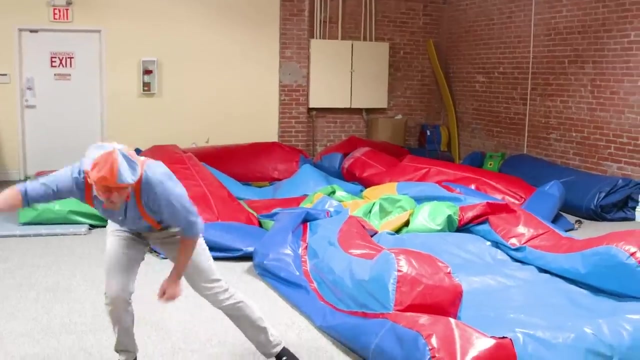 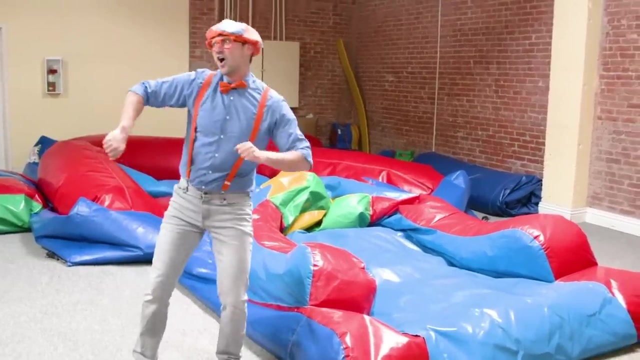 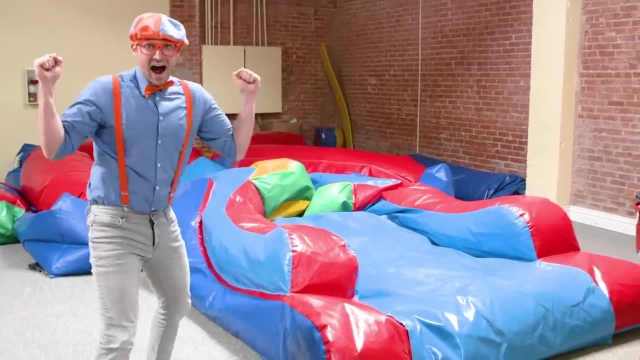 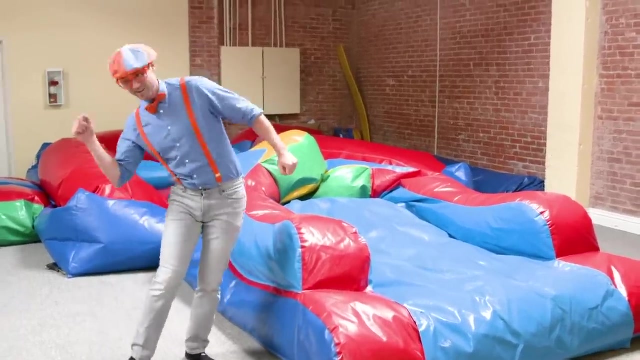 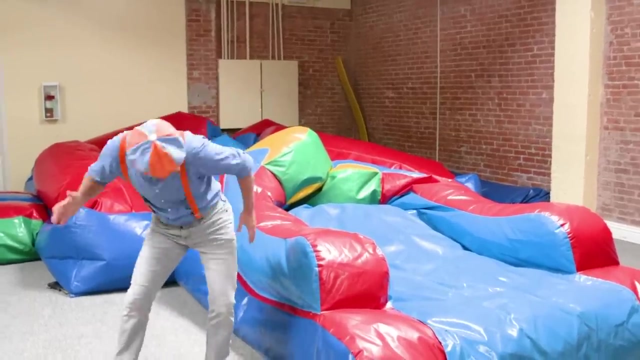 green motor. yeah, this is green and yellow. here we go, Hello, and welcome back to part two of S guilt. We're back at the video. G 🎵, 🎵, 🎵, 🎵, 🎵, 🎵. 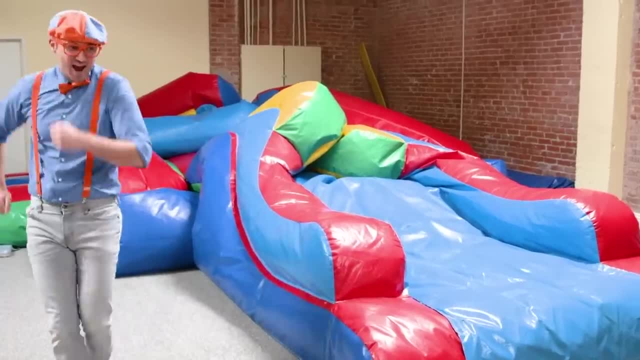 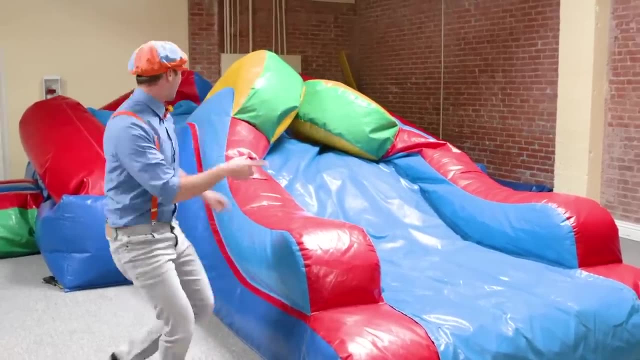 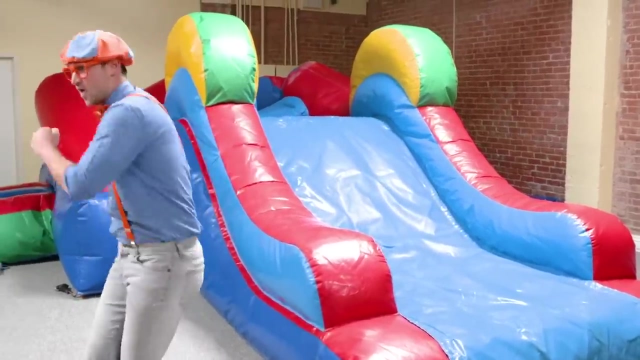 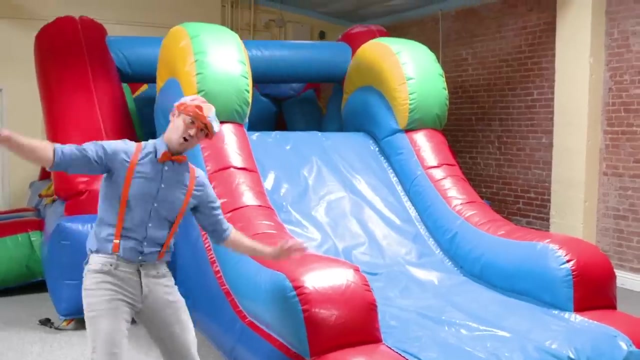 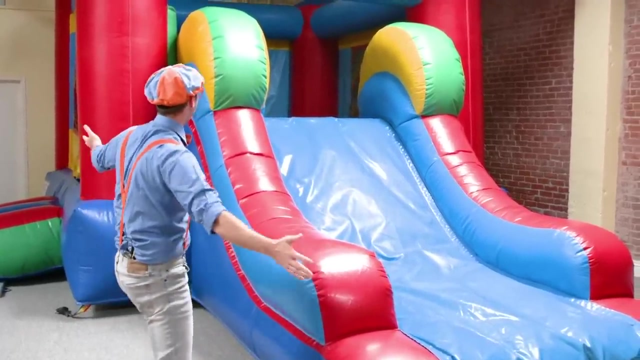 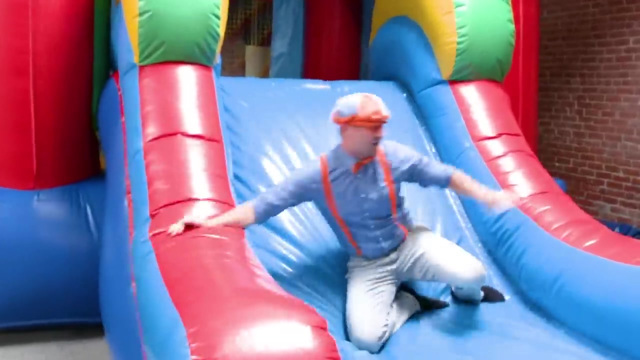 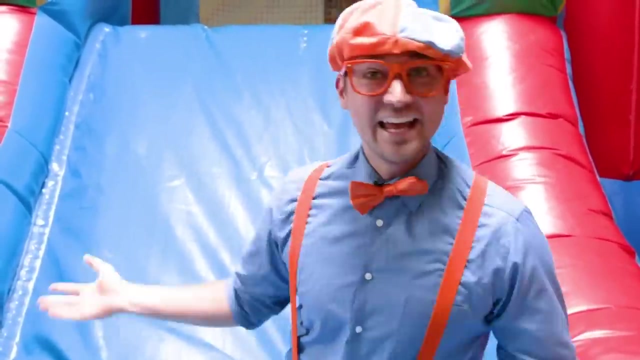 🎵. 🎵. Thanks for watching Whoa. Yeah, We did it. Good job, Woohoo, Woohoo, Whoa. What color is this? Yeah, It's one of my two favorite colors. Yeah, And it rhymes with two. 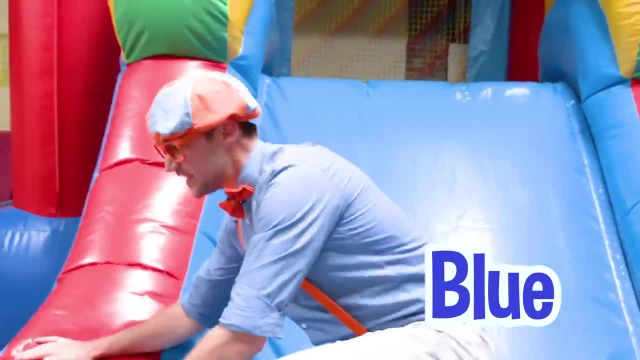 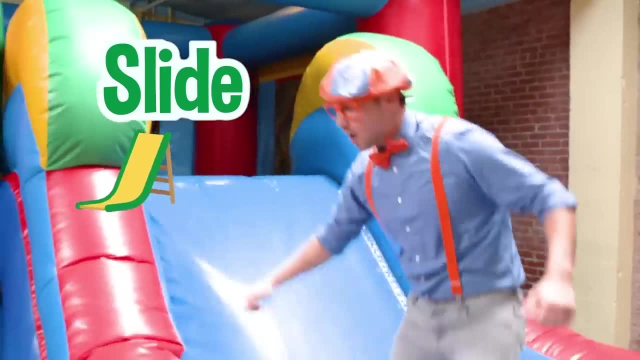 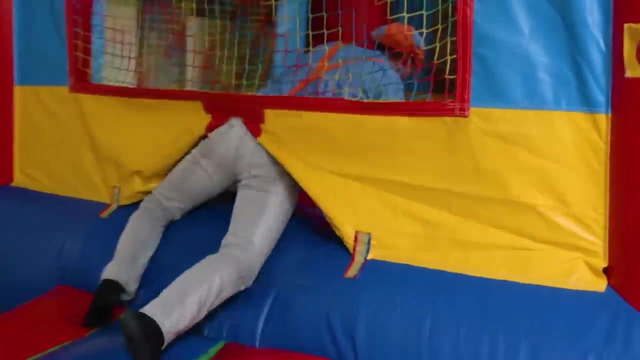 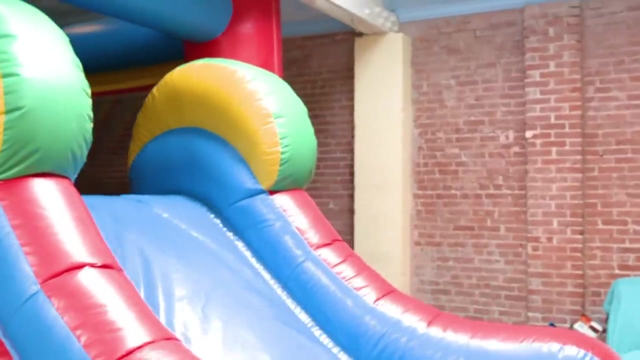 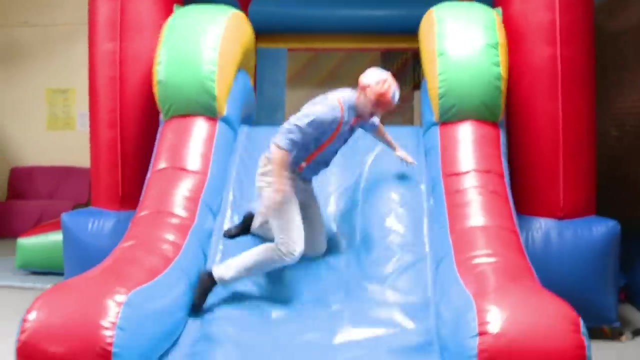 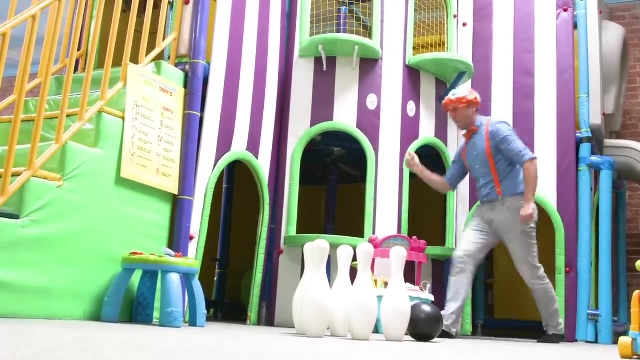 Blue And look at this: This is the color red. Alright, Time for me to go down the slide. Woohoo, Whoa, Here we go. Woohoo, Woohoo, Yeah, Hello, Hey, Woohoo. 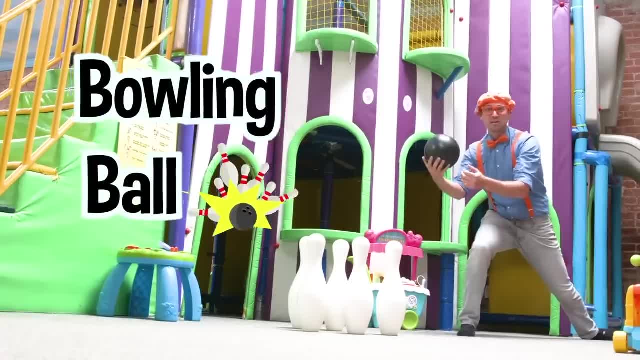 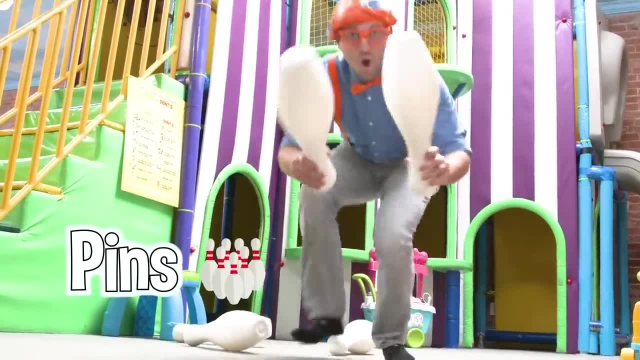 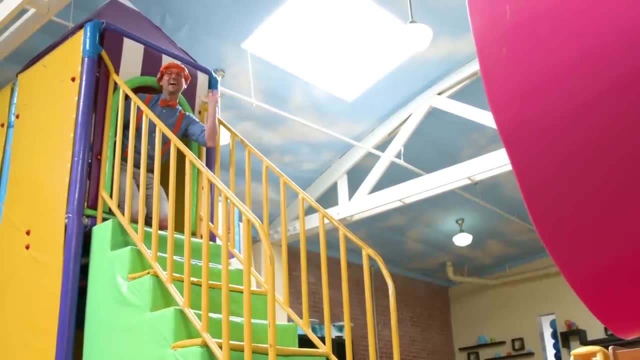 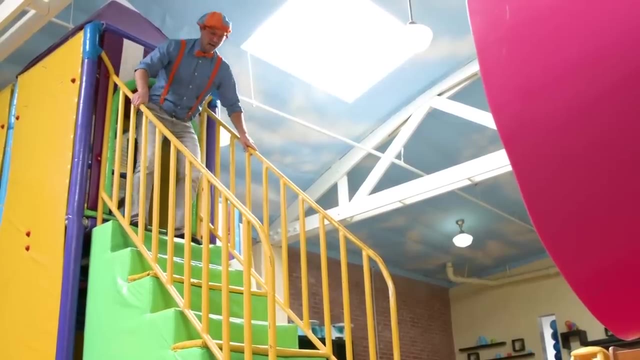 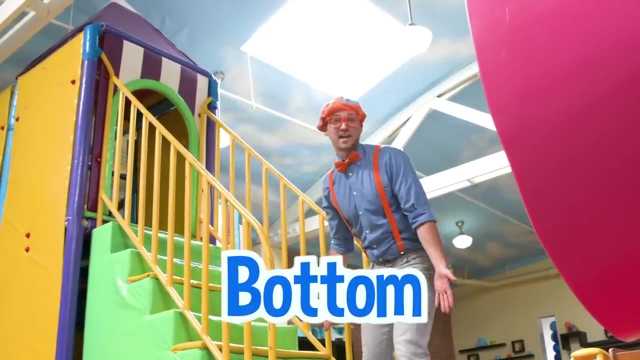 Hey, Hello down there. Look, I'm at the top of the stairs. Now I'm going to climb down. Whoa, Whoa, Now I'm going to climb down. I'm at the bottom of the stairs. I should probably climb up to the top of the stairs. 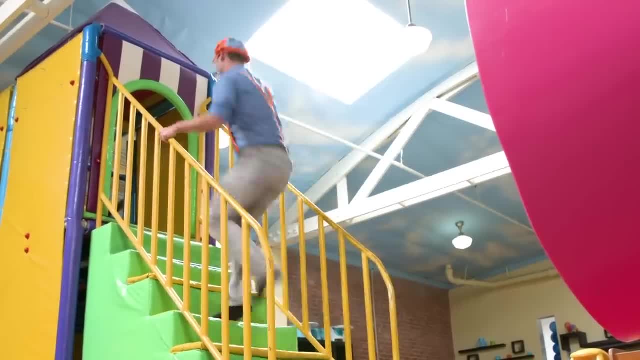 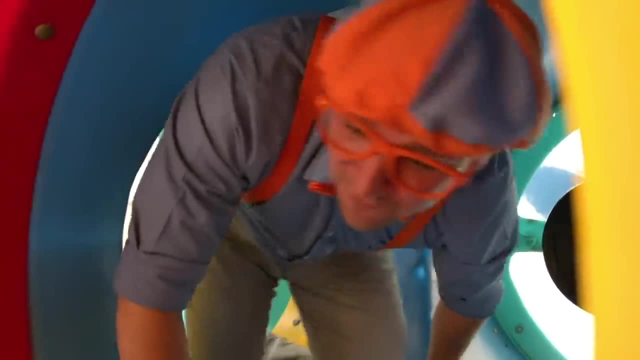 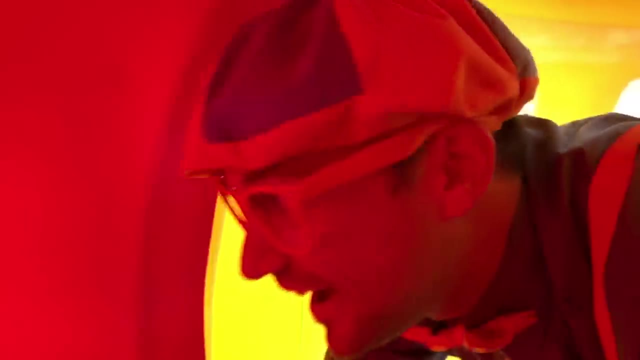 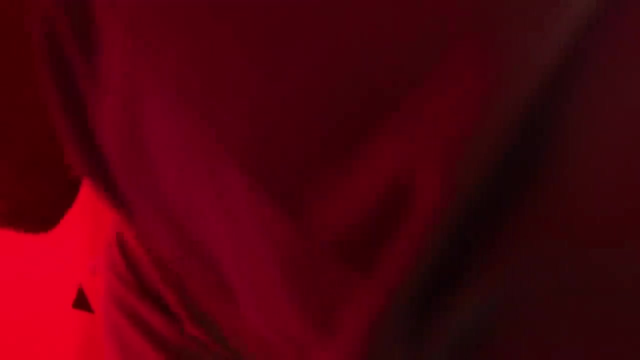 Woohoo, Bye-bye, Whoa, It's so colorful in here. Wow, I love crawling through these tunnels. Wow, Ooh, Okay, Oh, A slide. Haha, I'm excited. Woo, Okay, Are you ready? 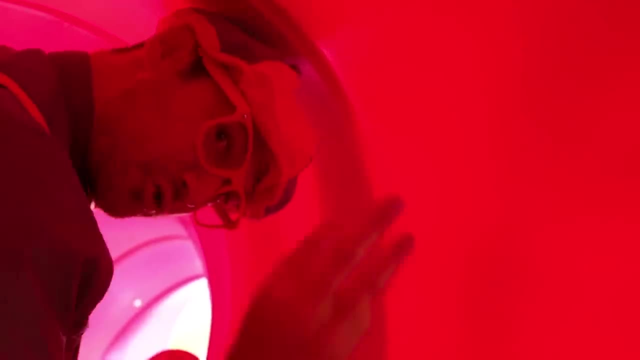 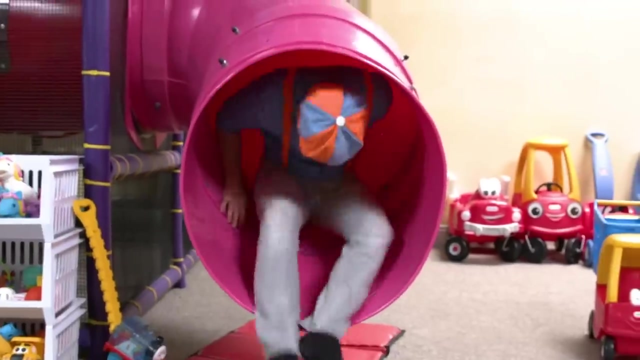 Three, two, one, Whoa, Whoa, Hello Woo. The slide was so much fun And it is a pink slide. Whoa, What is this? Whee, Whee, Whoa, Oh, Oh, Oh. 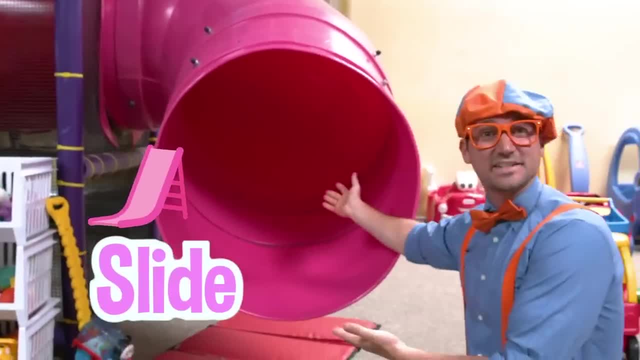 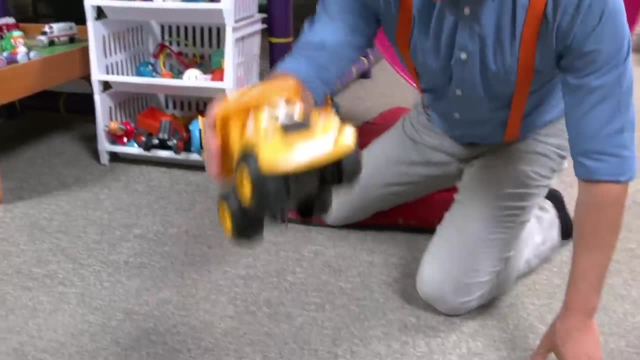 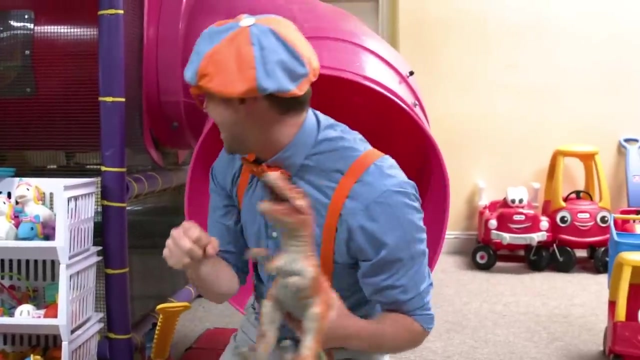 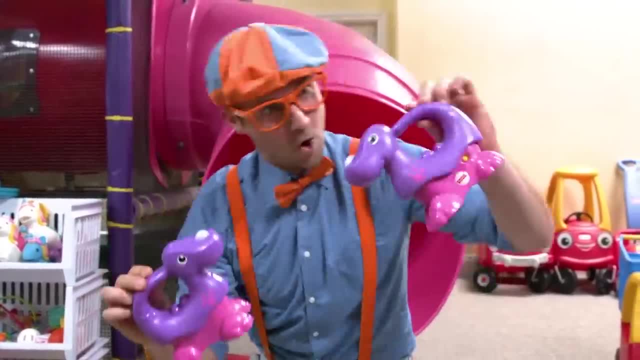 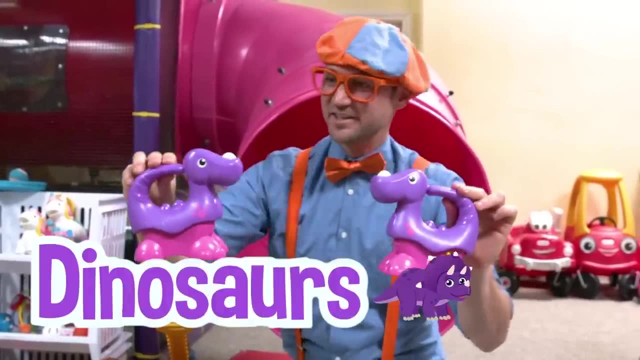 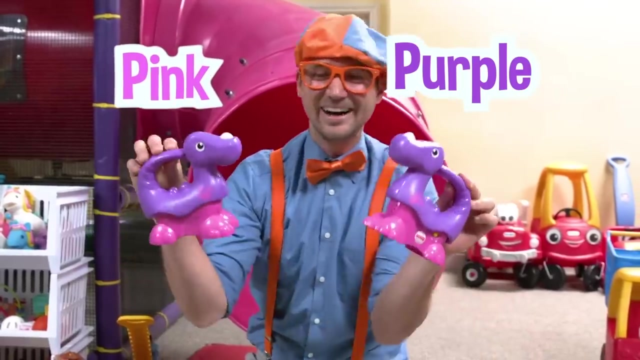 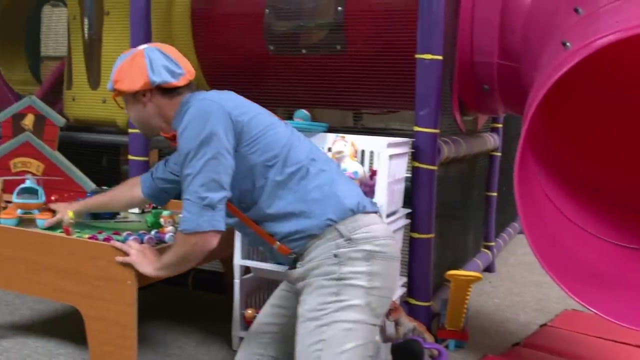 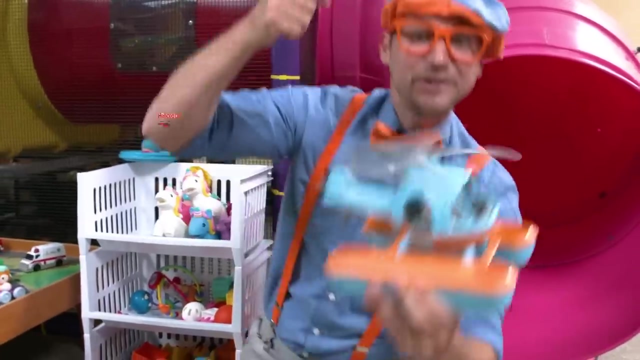 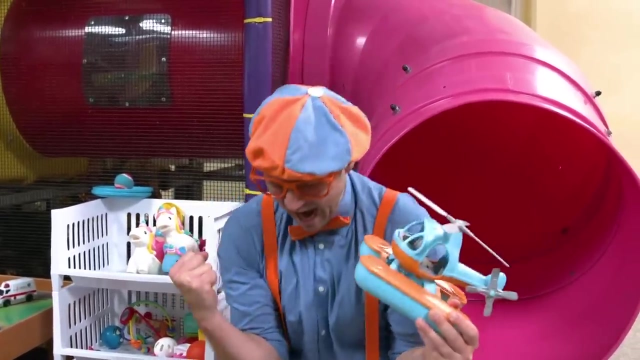 Oh, they're so cute. Hello, Hello Hi. How are you So silly? What color are these dinosaurs? Yeah, They are the color purple and pink. Look at this, it's a helicopter and it is my two favorite colors. yeah, what color is? 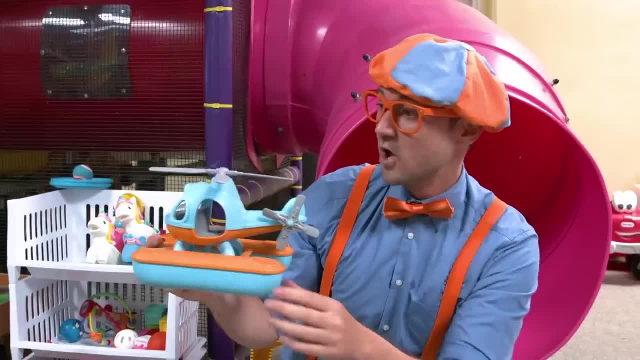 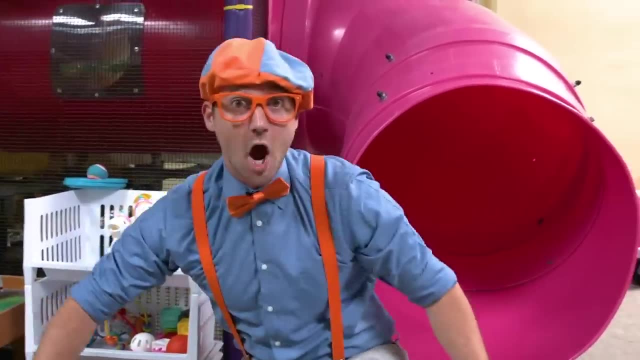 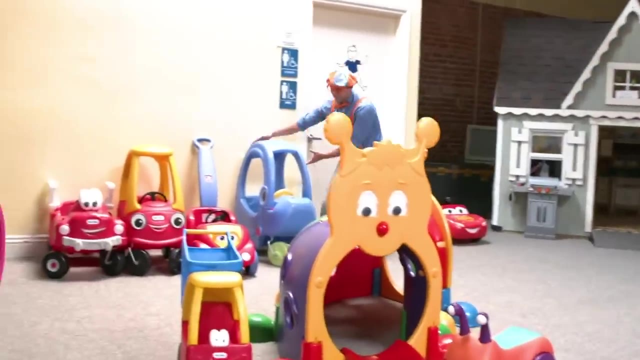 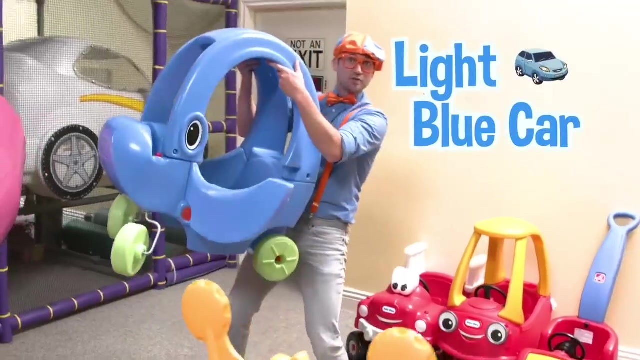 this helicopter. Yeah, there's two colors: blue and orange. woohoo, we'll set that back and go explore. whoop, whoop, whoop, woohoo, whoa free, free, whoa. look at this light blue car, real free. 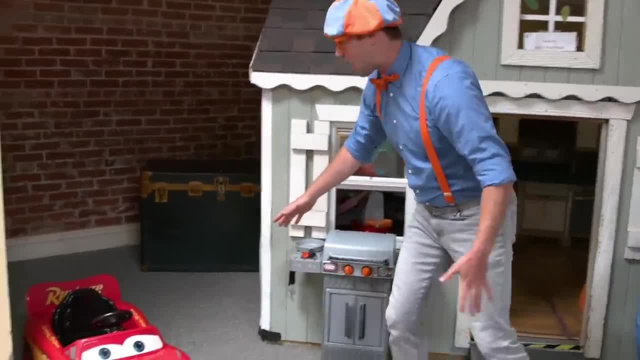 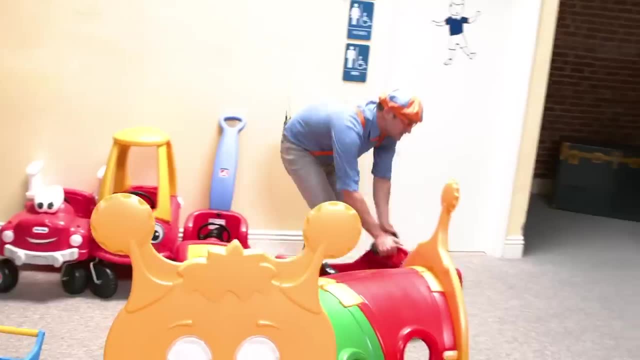 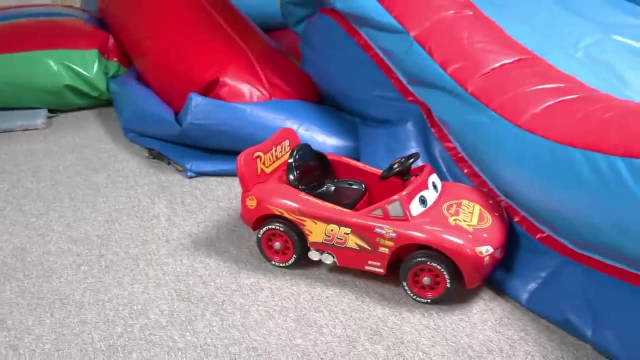 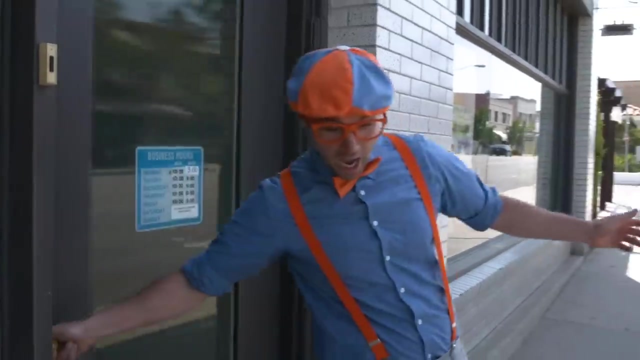 whoa, And look at this car. this car looks so fast, real, real, real, real, oh, real, haha, woohoo. I love learning my colors with you. haha, whoa, wow, that was so much fun playing at. 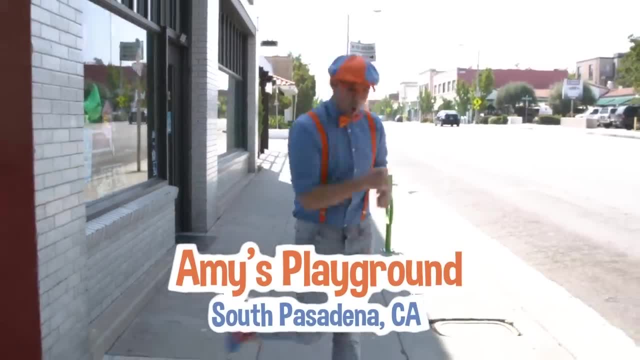 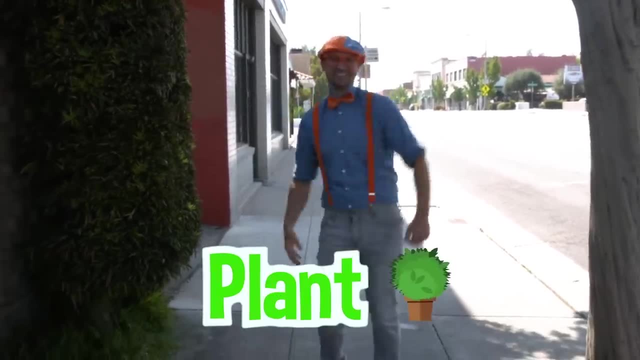 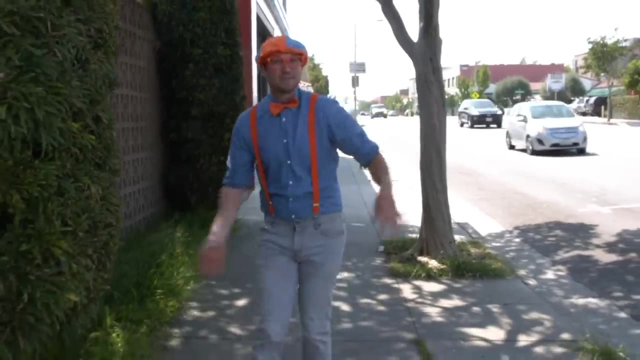 Amy's Playground From South Pasadena, California. woohoo, I really enjoyed learning about colors with you today. hey, like this green plant. haha, that was so much fun. well, this is the end of this video, but if you want to watch more of my videos, all you have to do is search. 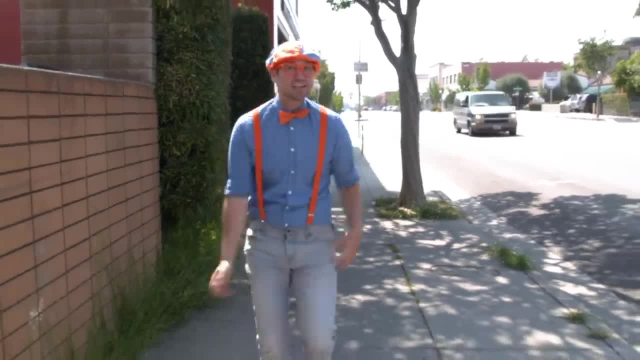 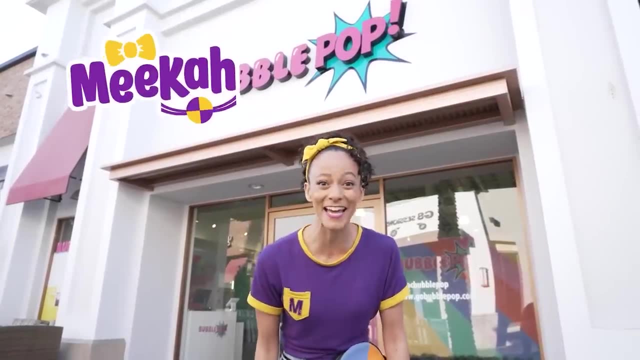 for my name. will you spell my name with me ready? B-L-I-P-P-I. hi, it's me Mika, and today I'm at Bubble Pop in Orange, California, and I'm going to show you how to spell my. name with me ready- B-L-I-P-P-I. Hi, it's me Mika, and today I'm at Bubble Pop in Orange, California, and I'm going to show you how to spell my name. with me ready: B-L-I-P-P-I. 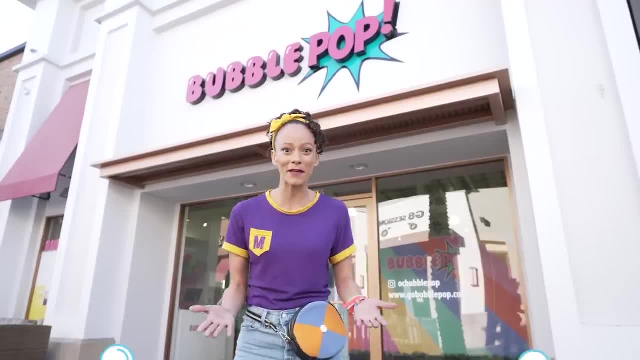 Hi, it's me Mika, and today I'm at Bubble Pop in Orange, California, and I'm going to show you how to spell my name with me ready: B-L-I-P-P-I. Have you ever played with bubbles before? 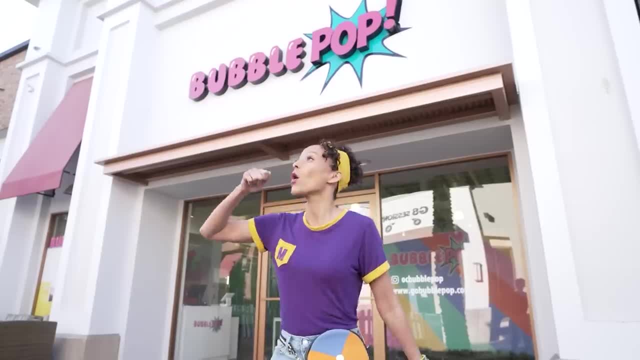 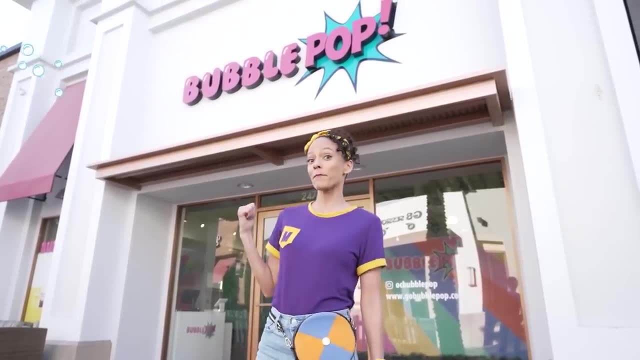 They're so much fun. maybe you've used a wand and blew bubbles into the air, or maybe you've taken a bubble bath. it's so fun. well, at Bubble Pop, we get to play with bubbles all day long. will you play with me? 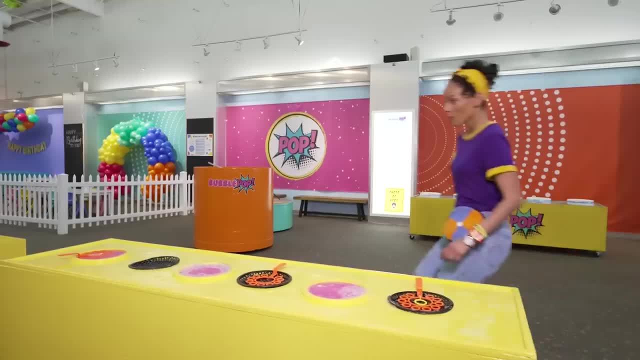 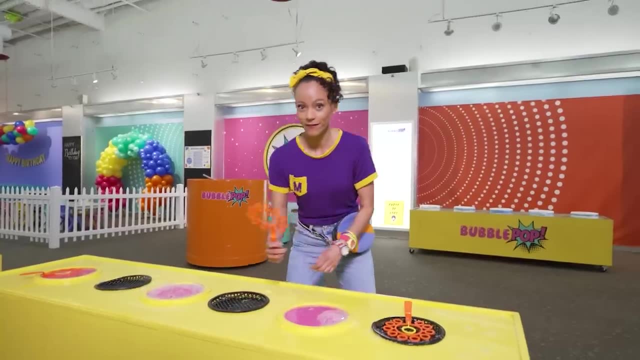 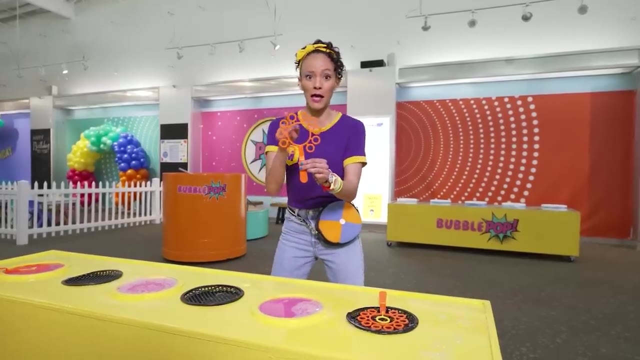 Let's go, Whoa, check it out. bubbles And Hmm, Hey, do you know what this is? A bubble wand. Whoa, and this one has a lot of circles on it. I wonder if that means it will make a ton of bubbles. 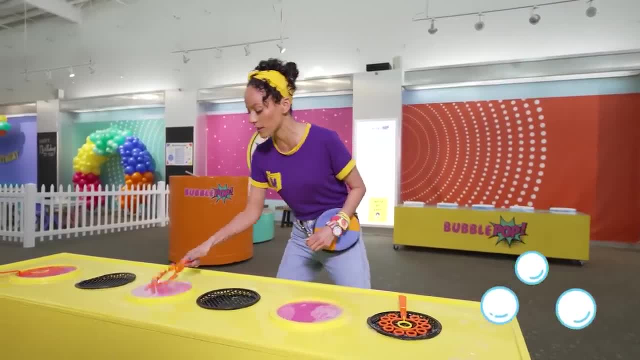 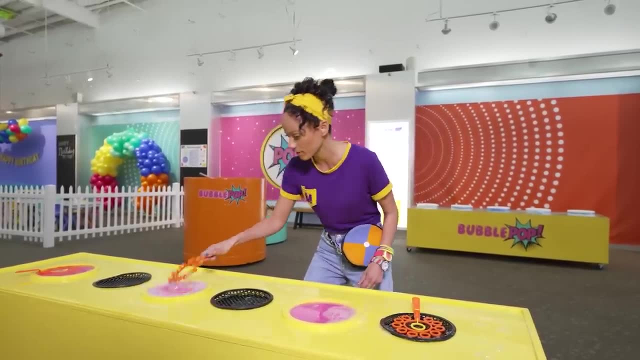 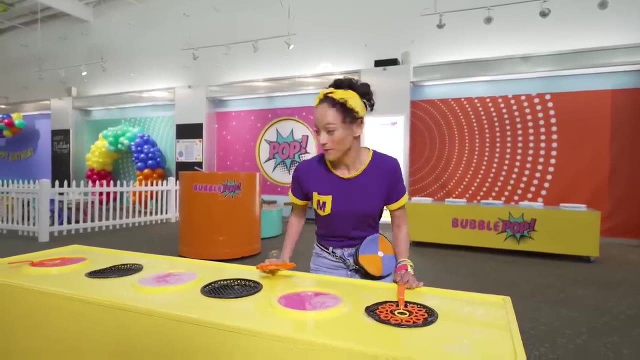 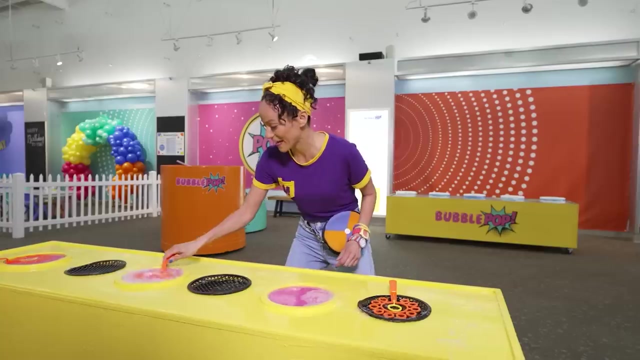 Let's find out. Okay, get some solution on there. I'll just try again. I only got two out. Do you hear that There's air blowing out from these two places here? That must mean, if I take the bubble solution. 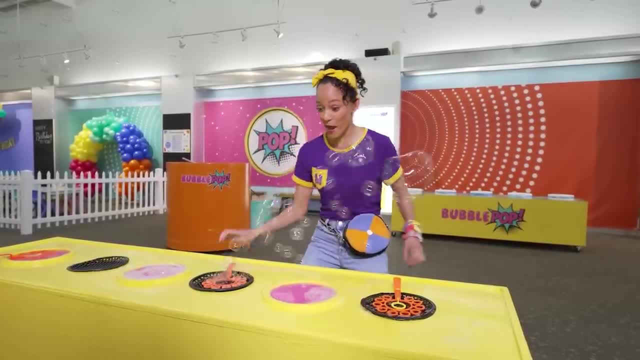 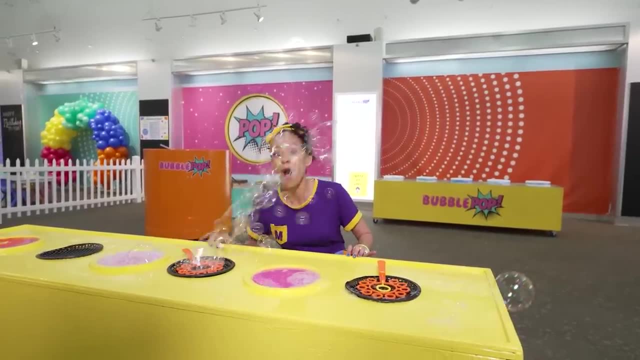 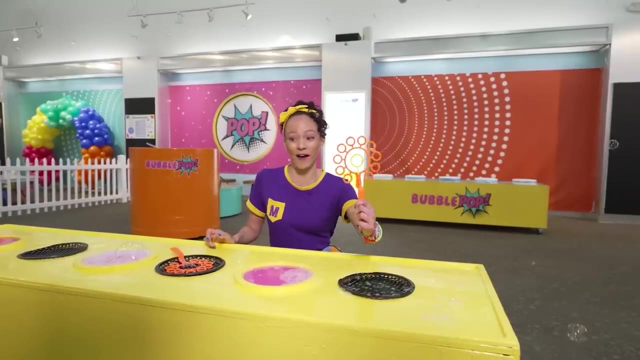 put it on the wand and then put it on the fan. That's so cool. Let's do it again. Whoa, look how many bubbles. Hey, here's another bubble wand. It looks just like this one, but there's something different. 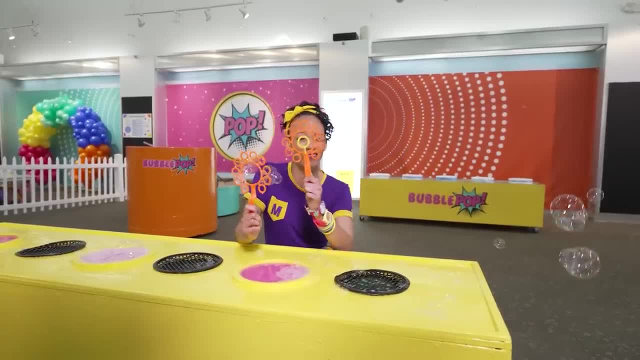 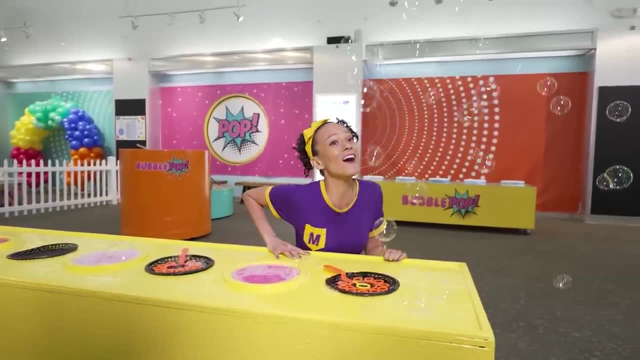 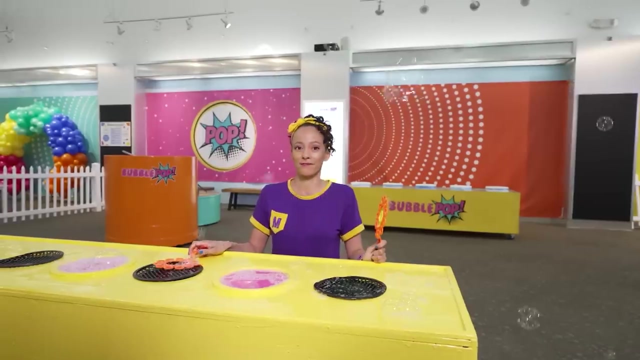 That's right. There's a yellow circle right here in the middle. Hello, All right, let's try this one. Whoa, even more bubbles. Wonder if I could do two at the same time? Okay, Three, two, one. 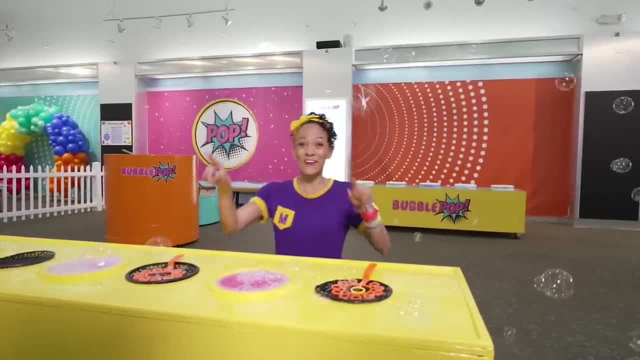 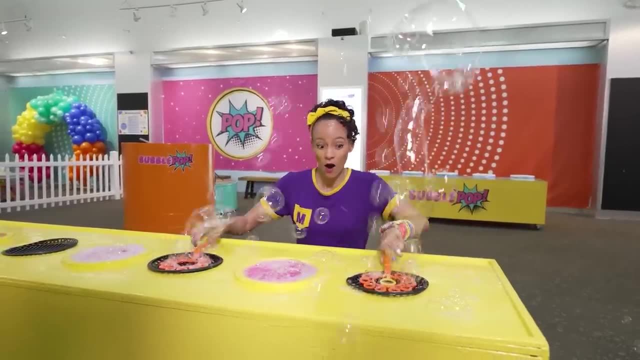 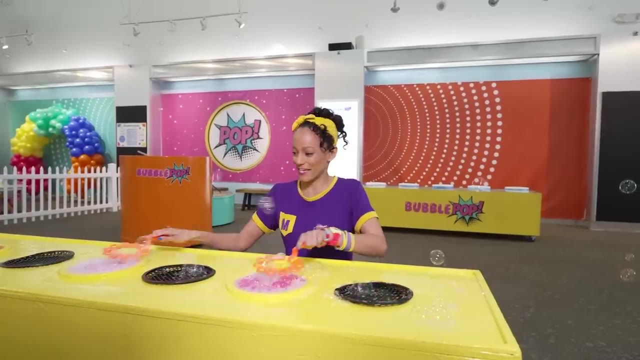 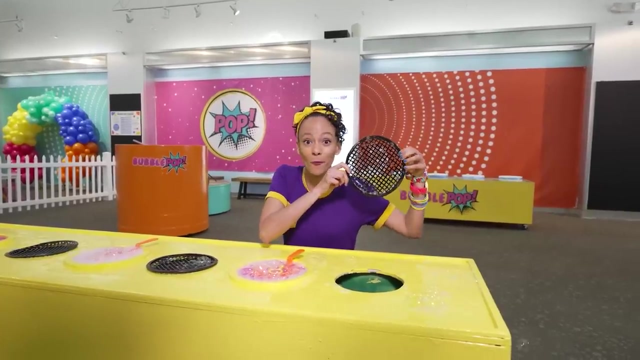 Whoa, So many bubbles. Whoa, I'm gonna do it again. Three, two, one. Whoa, Wait a second. I have an idea. Check this out. See, there's a bunch of squares in here. Kinda looks like a big waffle. 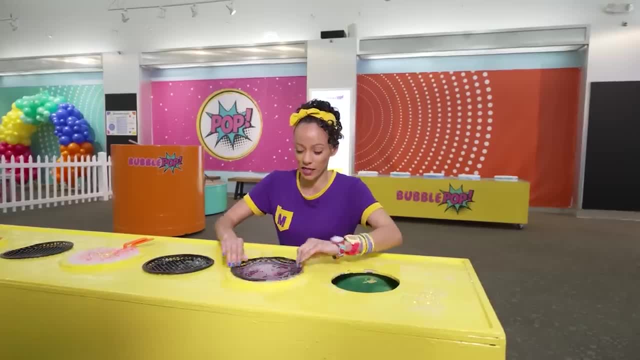 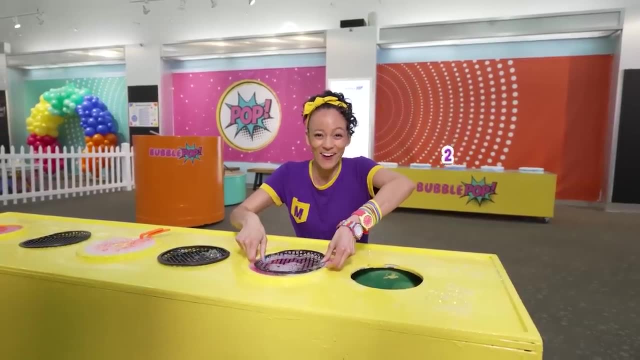 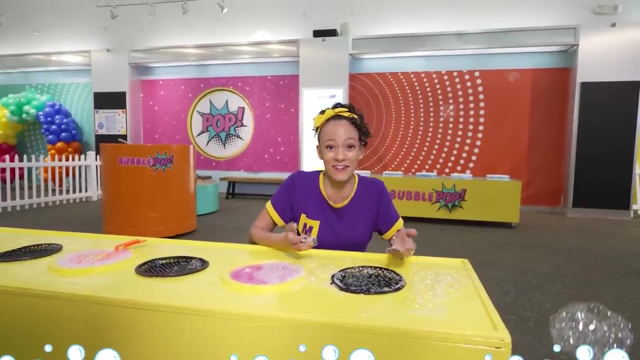 What would happen if I put some bubble solution on this? Okay, So I'm gonna go ahead and put it on the fan Ready: Three, two, one, Whoa. It kinda looks like the bubbles you would see when you're getting a bubble bath. 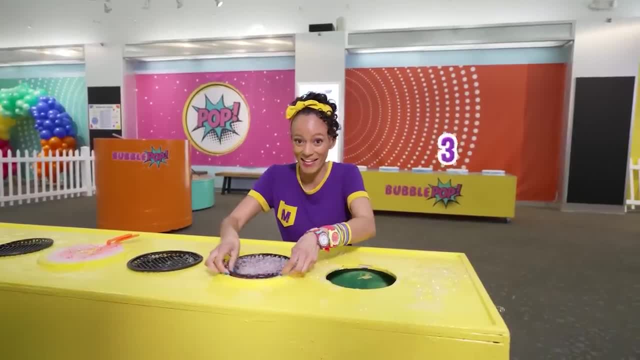 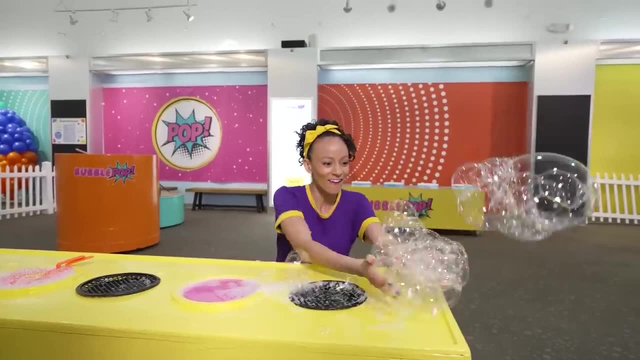 Gonna do it again. Ooh, ooh, ooh, ooh, Okay, ready. Three, two, one, Whoa, Whoa. Bubbles are so much fun. It's so fun. Yeah, I love bubbles. 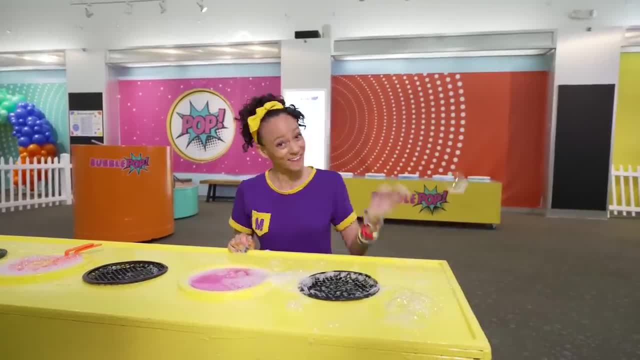 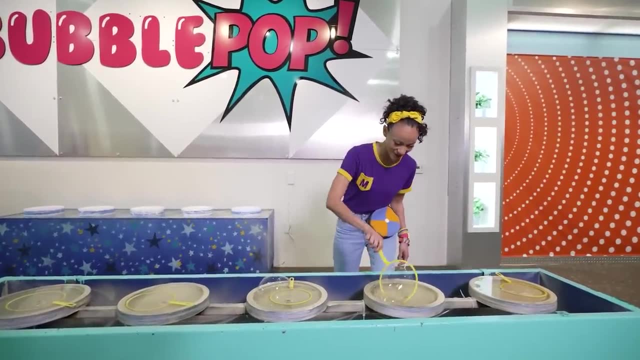 I love bubbles. I love bubbles. I wonder what else we can do here. Come on, Whoa, look even more bubbles. Whoa, let's check out this bubble wand. It's a big yellow circle, One of my favorite colors. 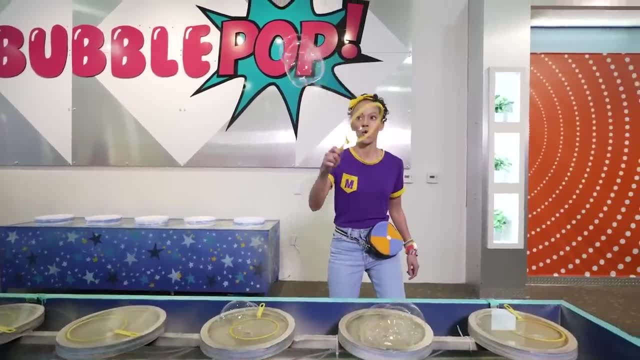 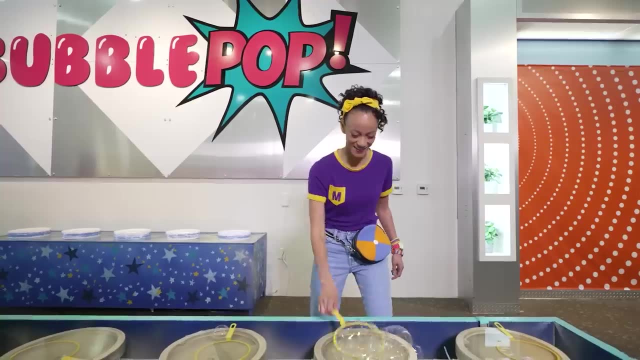 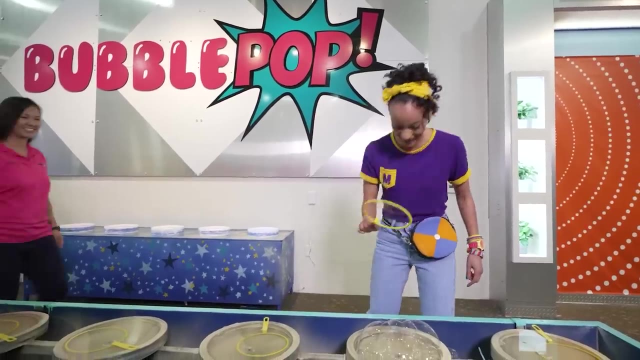 See if I can make a bubble. Whoa, Oh, I caught it. Do it again. Whoa, that was a big bubble. Oh hi Hi, I'm Theresa from Bubble Pop. Hi, Theresa, I'm Mika. nice to meet you. 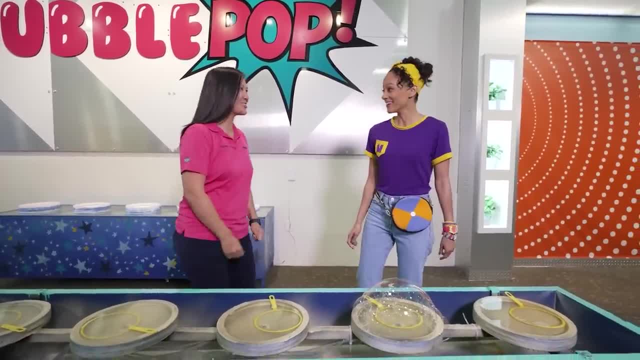 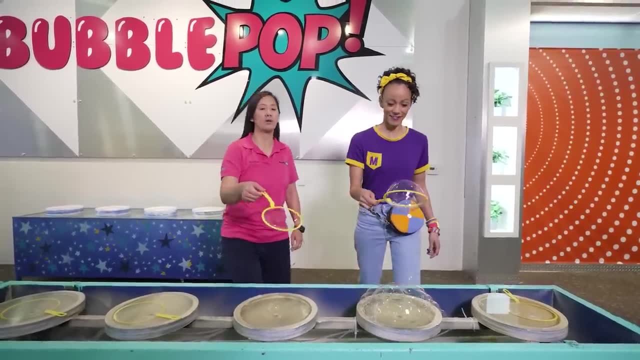 Hi, Mika, I'm so glad that you're playing with our bubbles. Yeah, Can I show you some bubble tricks? Oh, yes, please, let's see. So I saw you making a bubble, all right, So we're gonna make the bubble kind of like you just did. 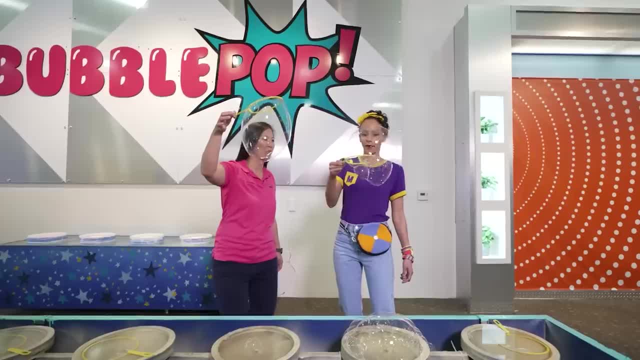 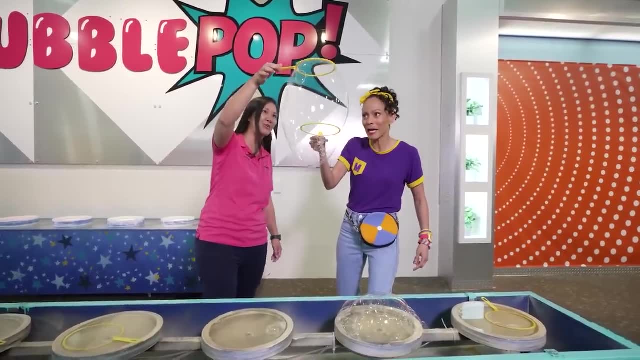 and then catch it, just like you did. Whoa, Whoa, you have three or more bubbles on your wand. Check it out. Our bubbles came out, Came together and made a huge one. Whoa, Wow, bubbles are awesome. 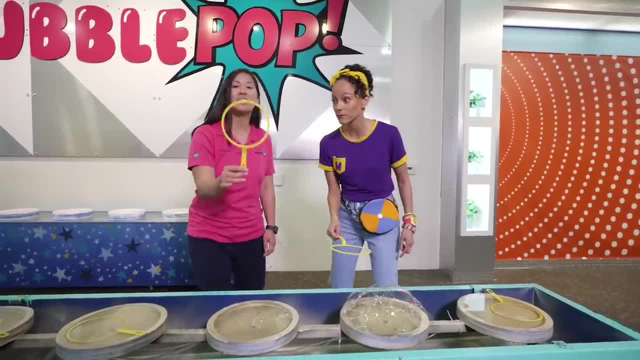 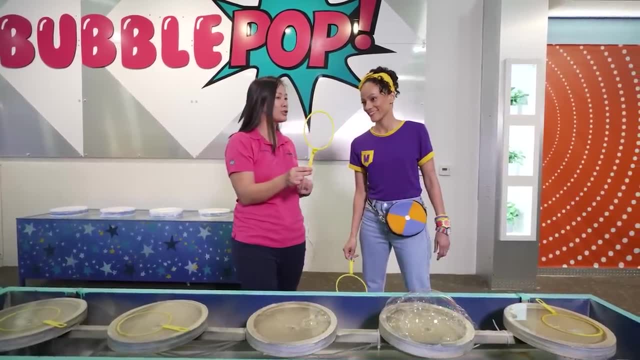 What is a bubble? Well, I'm glad you asked, Mika, because you can see right here, see this film on the wand. Yeah, it's like shiny. Yeah, it's our bubble solution. So usually bubble solutions are made of soap and water. 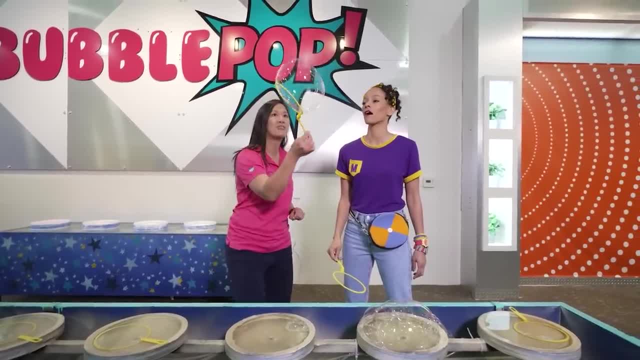 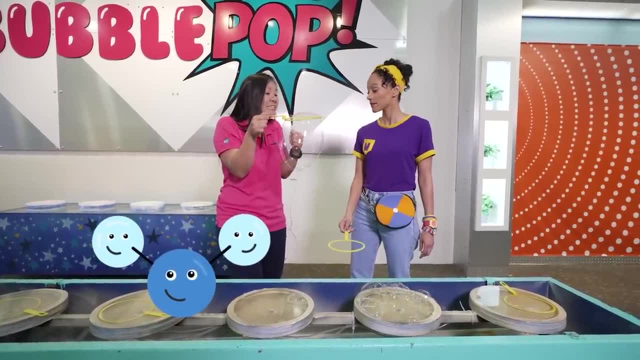 and usually something else. that's a polymer that will bind everything together. Water molecules love each other so much, They like to just hold hands and be really tight, and so they squeeze the soap molecule together, And that's why there's a thin film here. 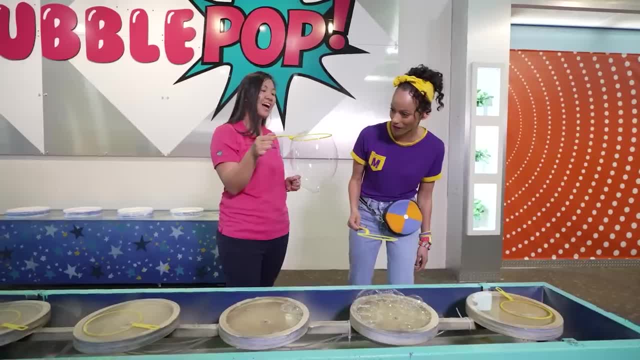 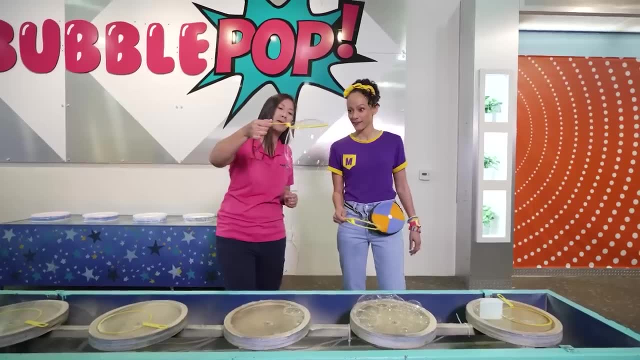 that makes your bubble. Oh, that's really cool. And when they do that, it's called cohesion, Cohesion, Yep, and that's what makes the bubble hold together, just like this. Wow, All right, you ready to do a bubble trick? 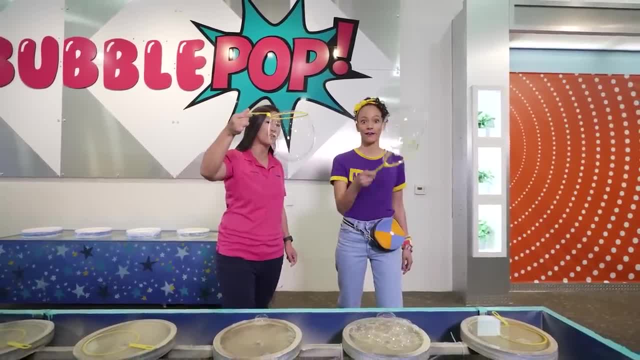 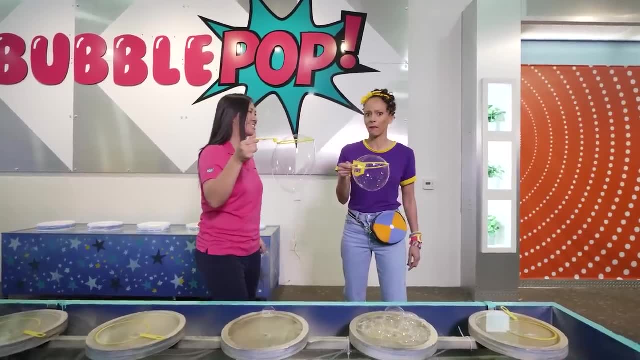 Yeah, Okay. so because bubbles love each other, they're gonna make a bubble. Okay, so because bubbles love each other so much- the water molecules inside a bubble- we can actually create a bubble inside this bubble. How, Wanna try it with me. 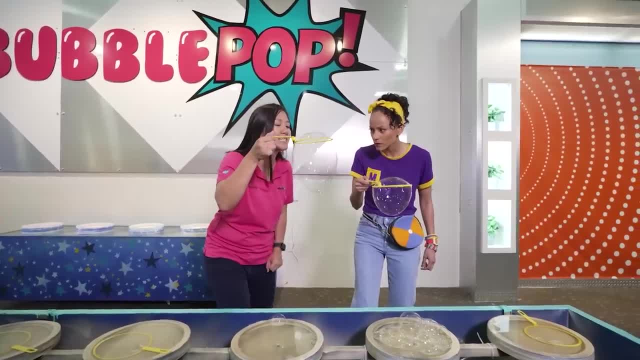 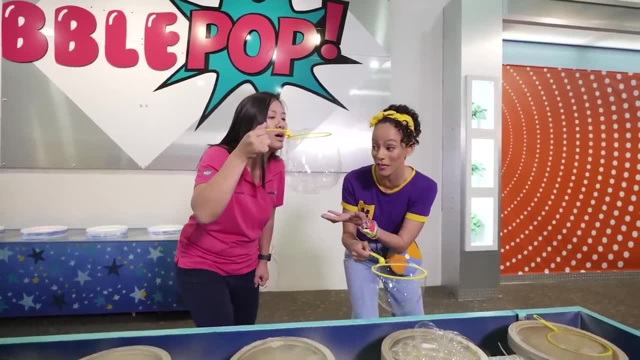 Yeah. So I want you to blow very short bursts inside the bubble. Whoa, do you see that There's little bubbles in the really big bubble? Whoa, Whoa. can I do that even in this little bubble? I think you can. 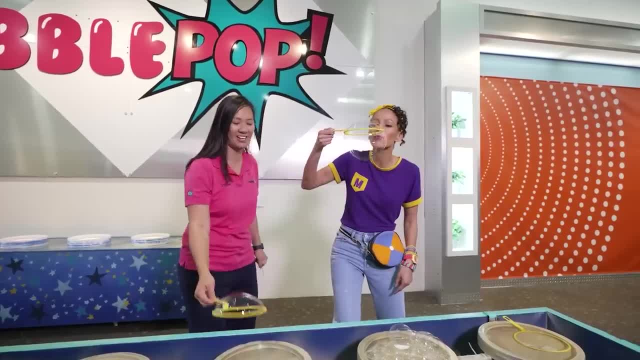 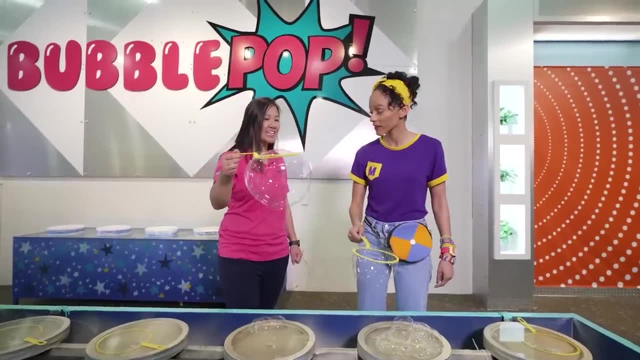 Oh, I see a baby one. Yeah, There's a tiny one right there. So, instead of blowing bubbles inside a bubble, something else that cohesion allows us to do is put a bubble on any surface that we want to. Oh, okay. 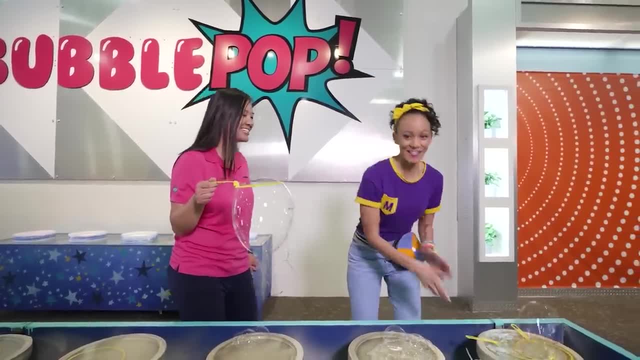 Like, how about your hand? You wanna try to catch one in your hand. Yes, yes, yes, yes, yes, Okay. so I will make a bubble for you and then you try to catch it with your hand. All righty. 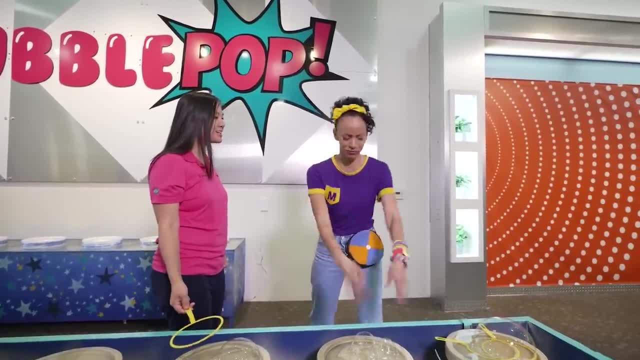 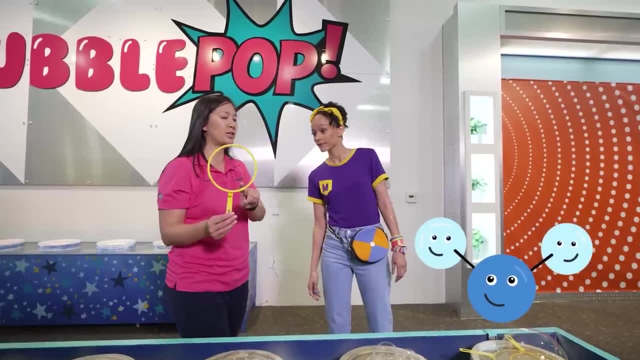 I'm gonna catch that bubble. Oh, it popped. That was so close. It did pop, So I'm gonna try to catch it. So the most important thing about cohesion is that you need water molecules together. right, Let me see your hand. 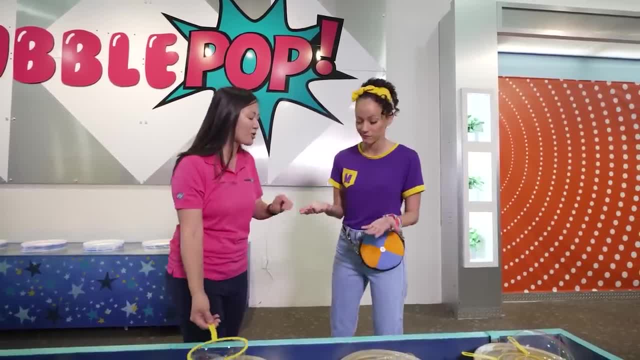 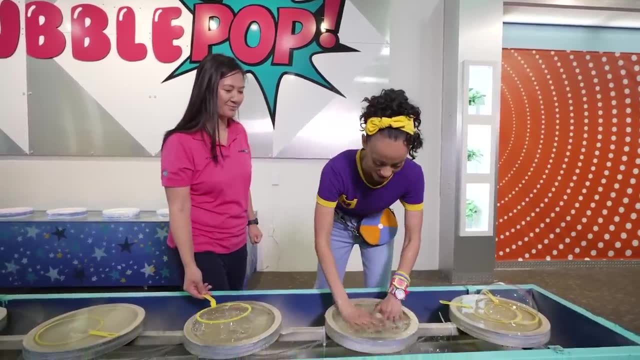 It's just a little wet. It was kind of dry. Yeah, Let's try it with a bunch of water molecules on it, and then they can link together. Ooh, okay, Get all the solution on my hands. Yes, I'm ready to catch this bubble. 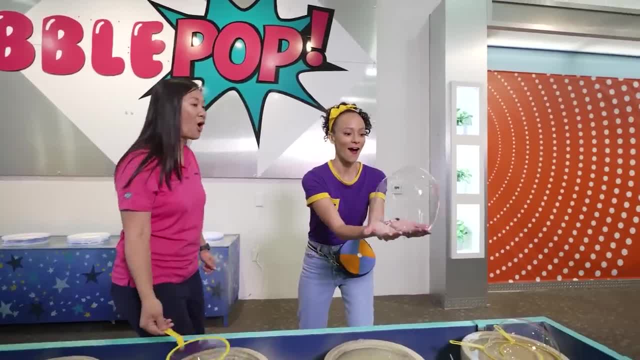 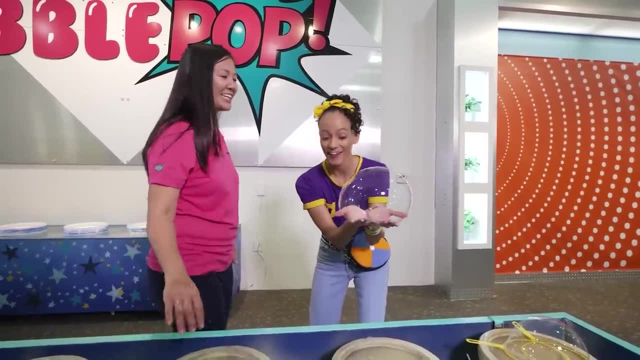 Okay, I am going to throw one at ya. You did it, you caught it. I caught a bubble. I caught a bubble. Wow, Hello, That's so cool. Let me see if I can even pop it. but I wet my hand. 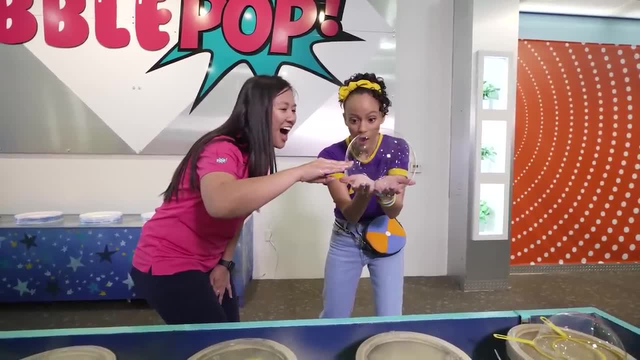 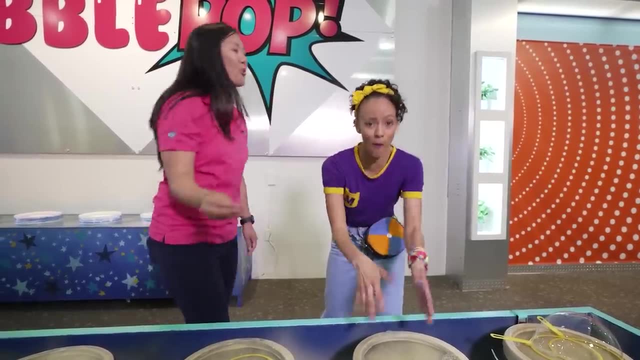 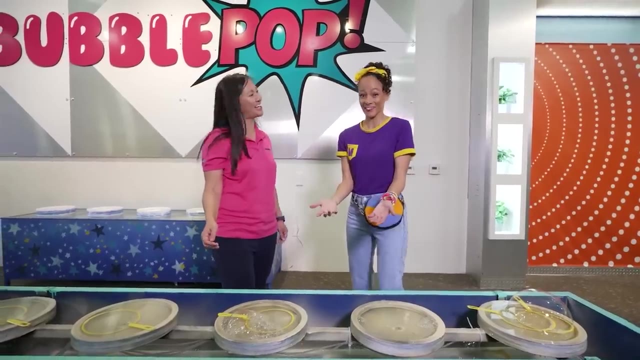 so I think the water is gonna like each other and I can put my hand inside your bubble. Theresa, you're a bubble magician. Ooh, Was that cool. That was amazing. Do you wanna see other cool bubble tricks? Yes, I do. 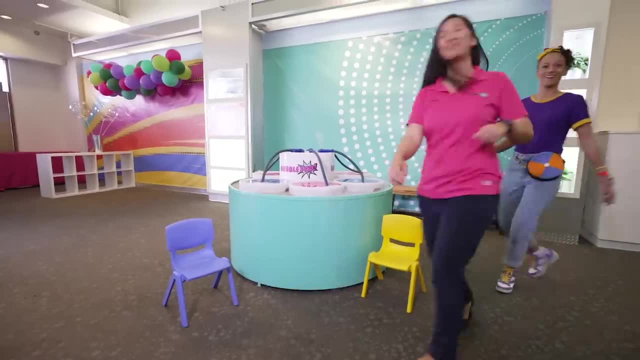 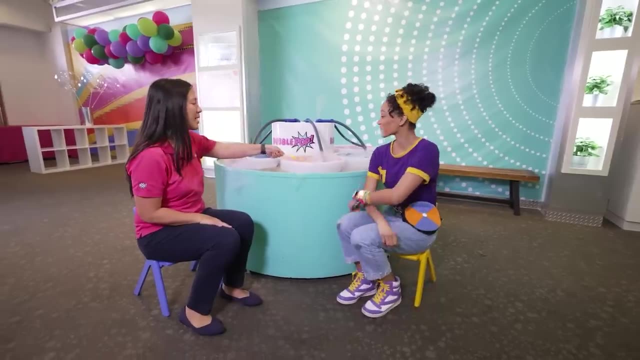 Okay, come on, let's go. Come with us, Mika. let me show you this phantom bubble station. Phantom bubble station. Yes, do you remember before how we made a bubble with just air in it? Mm-hmm. 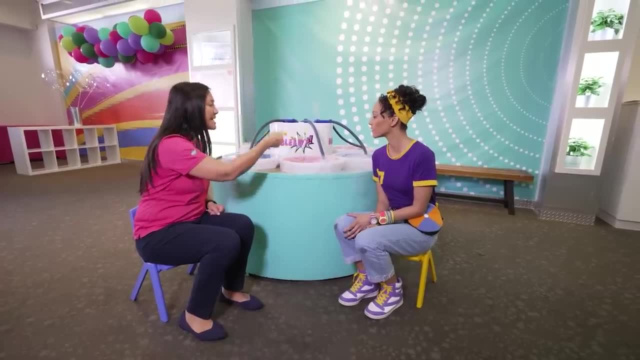 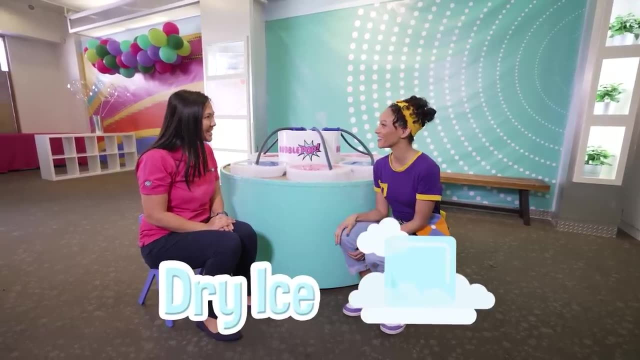 All right. well, this one, we're gonna make a bubble, but it's gonna be filled with something besides air. Oh, what is it gonna be filled with? Do you know what dry ice is, Mika? Yeah, So dry ice is made of carbon dioxide. 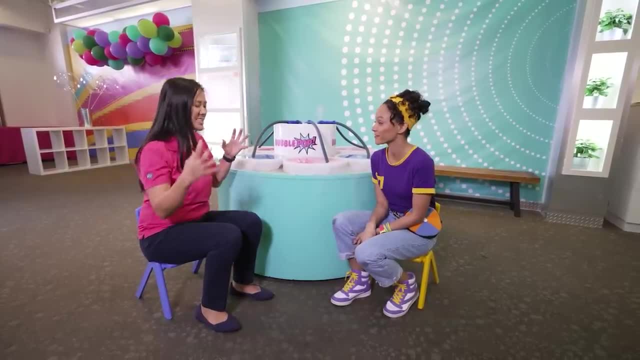 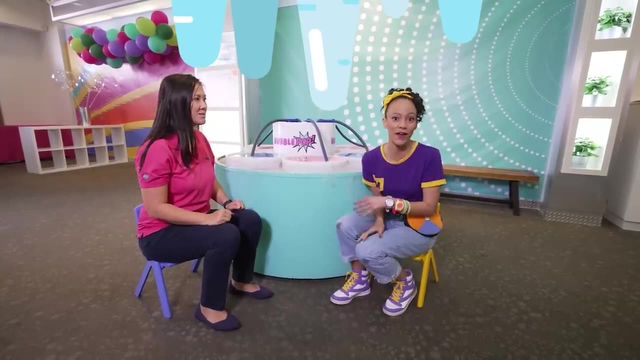 which is already in our air. We would just breathe it normally. but what they do is they make it really really tight so that it can get things really really cold. Whoa, and it's way colder than the ice you would find in your refrigerator. 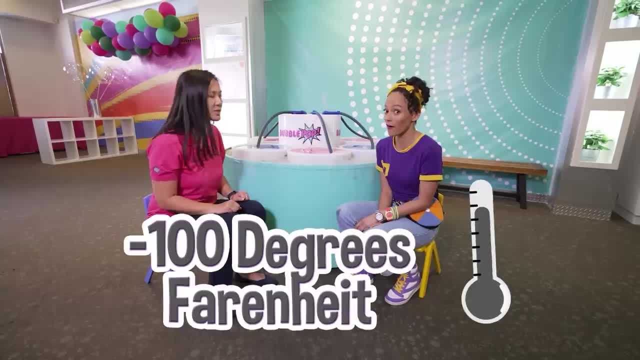 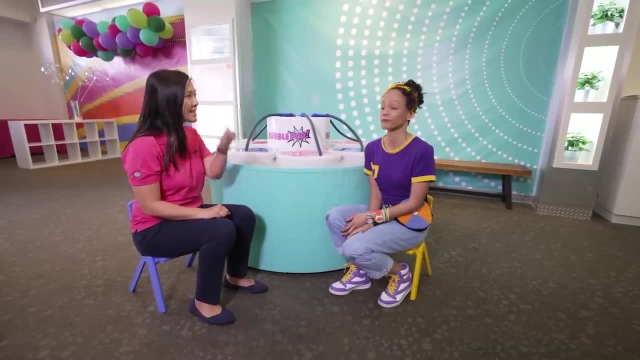 Yeah, that's right. It's negative 100 degrees Fahrenheit. That's super cold. In fact it's so cold it's not really safe to touch, So we never wanna touch it. So what we do is we keep it nice and safe inside here. 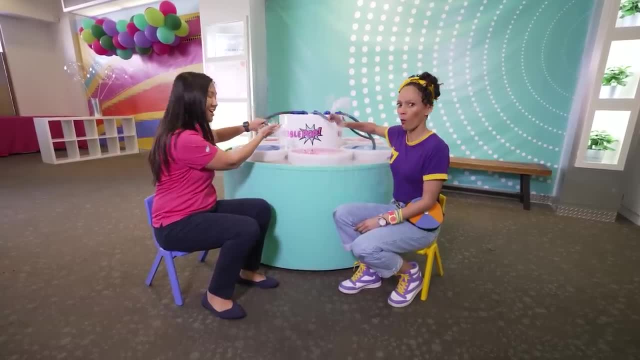 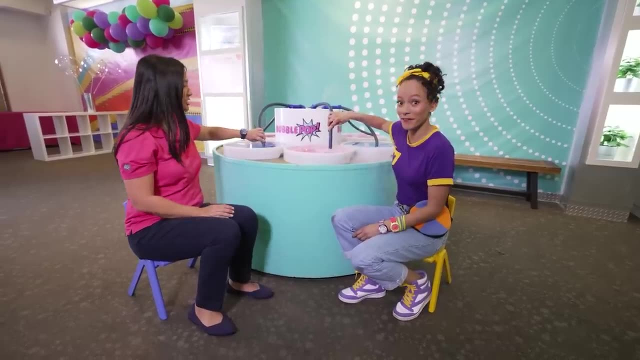 but what comes out is the sublimated form of carbon dioxide, which is this smoke that we see and it's neat, So we can put it here in our bubble solution. We turn it and it can trap the fog inside the bubble. 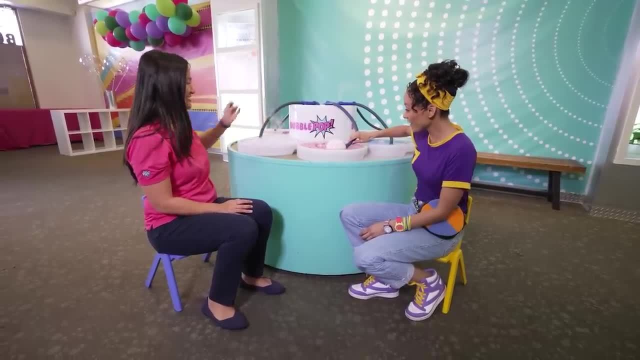 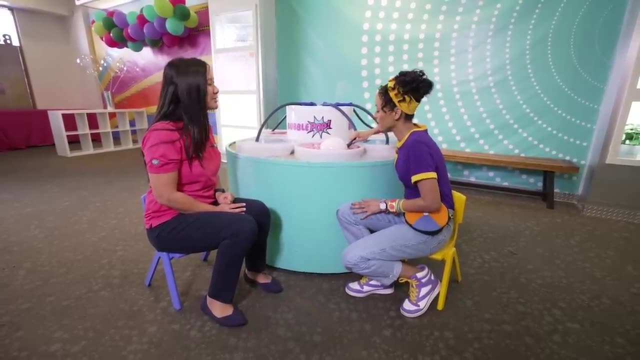 Wow, look, And now you have a smoke-filled bubble. That's really neat. It was kind of like a crystal ball, Yeah, and you know what's really cool? Remember last time how we put a bubble in your hand, Yep. 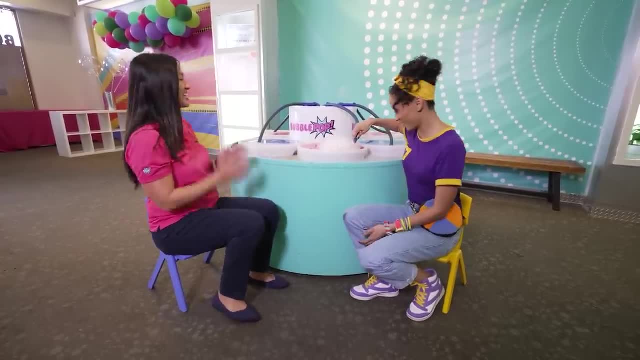 Would you like a smoke-filled bubble in your hand? Yes, I would thank you. All right, let's do it All right. so do you remember the trick to how we always hold a bubble? We hold a bubble without popping it. 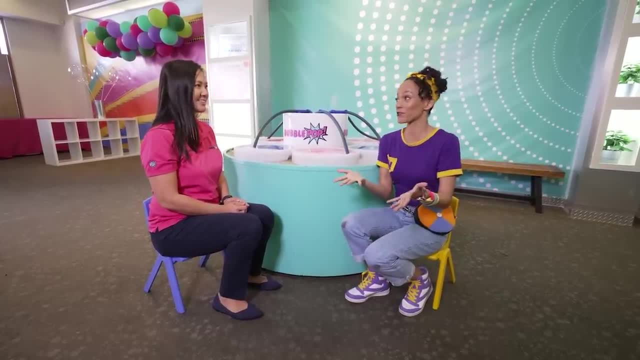 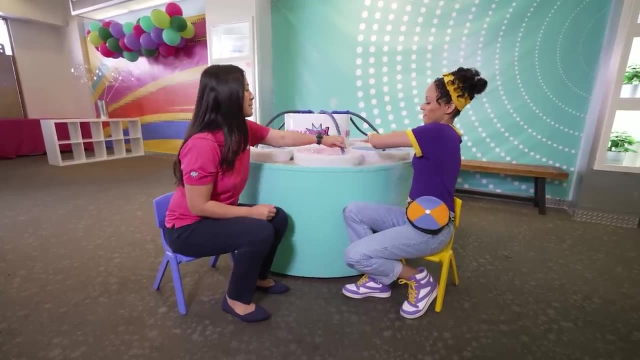 Right, you don't want your hands to be dry. My hands are really dry right now, so I'm gonna put some bubble solution on them so they get nice and wet. Perfect, All right, and I will help you. put the bubble inside your hand. 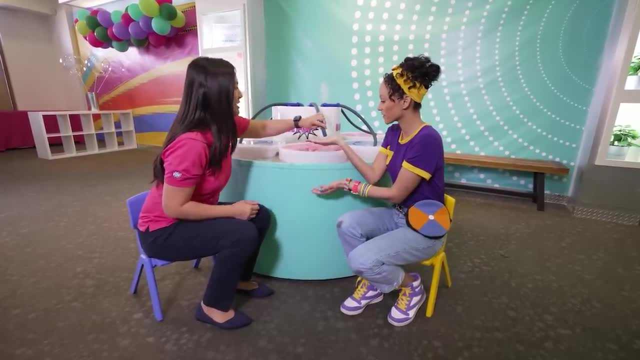 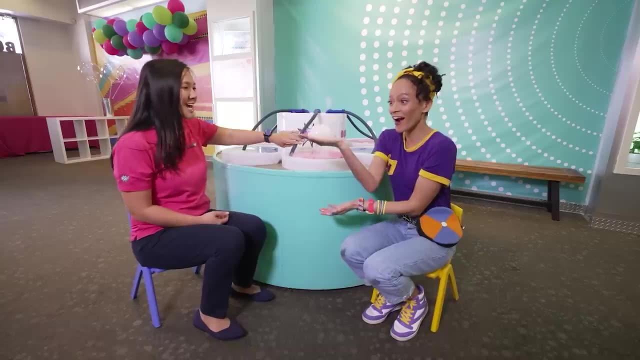 Okay, All right, here we go, Get it on here, hold up, Why don't we? there we go. Look at that. Whoa, Whoa. now you have a smoke-filled bubble in your hand. That's so cool. 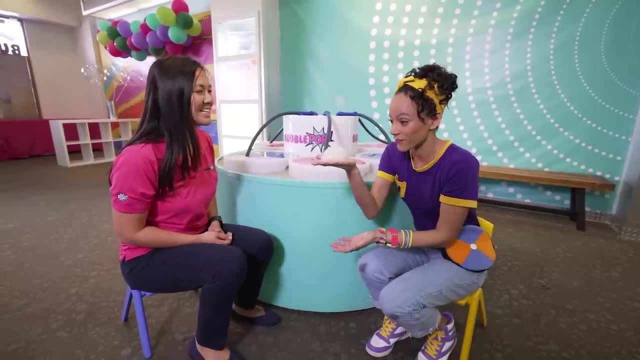 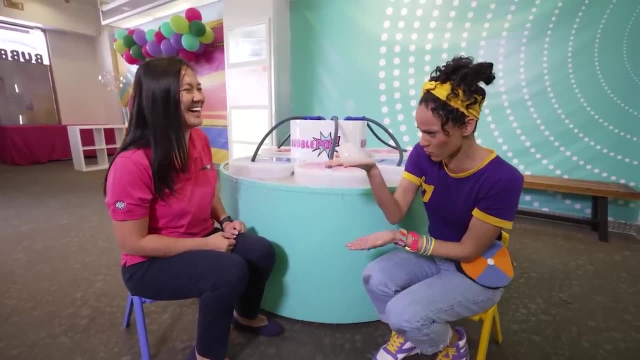 You can't even see through it. That's how much smoke is in there, Mm-hmm, can you make it dance? Do-do-do, ba-ba-da-ba-ba. Oh, come on bubble. Yes, oh, this bubble has moves. 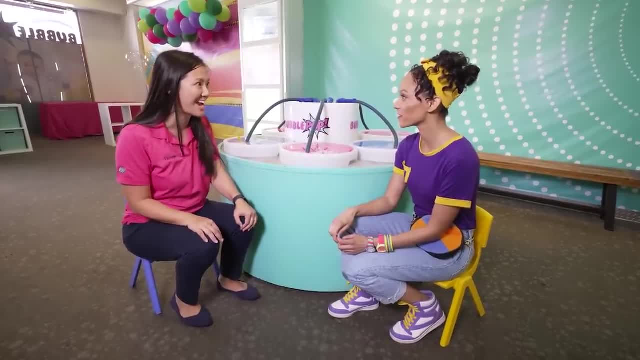 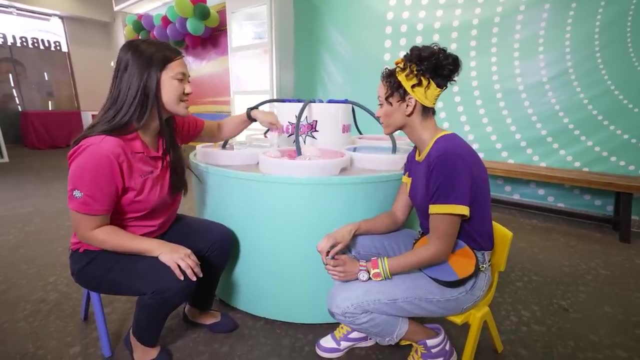 Did you know that carbon dioxide is actually heavier than regular air? Oh Yeah, so when we fill the bubble, we use only carbon dioxide, so all you see is the smoke that's inside. Yeah, you can't see through it, or anything. 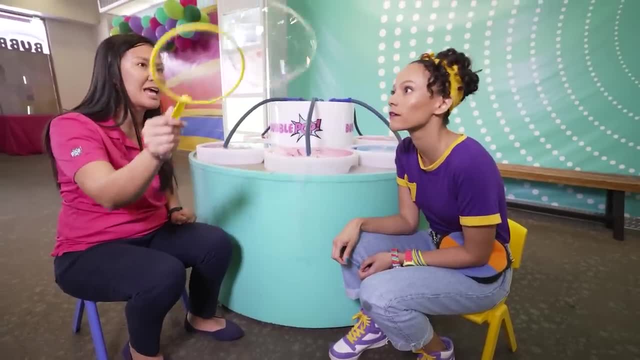 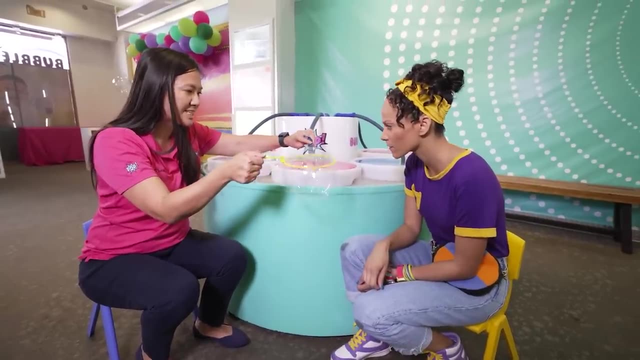 Nope, but if we make a bubble and we have both air and carbon dioxide, we'll be able to see which one's heavier. How does it get in there? So we're gonna use this and we're gonna stick it right inside here. 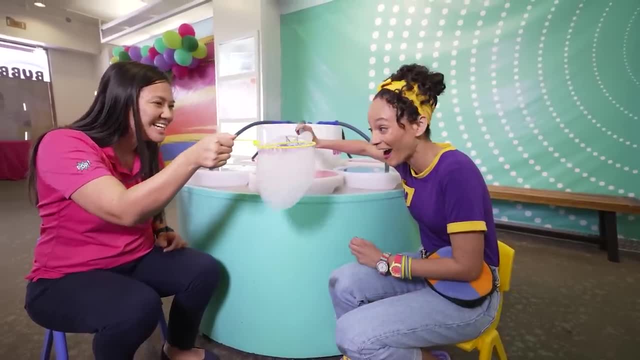 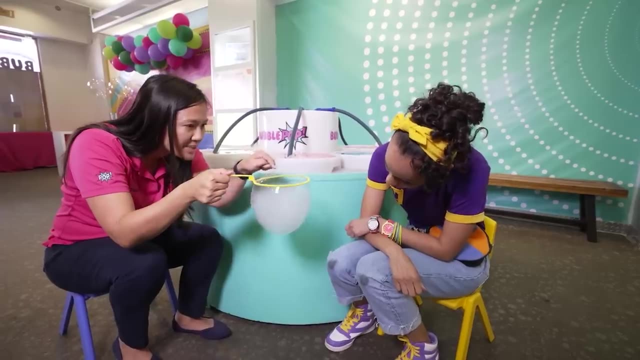 Thank you for your help, Mika. Yeah, All right. do you see that? Do you see how at the bottom there's the fog, carbon dioxide smoke and then Mm-hmm, And then at the top you can see that it's just regular air? 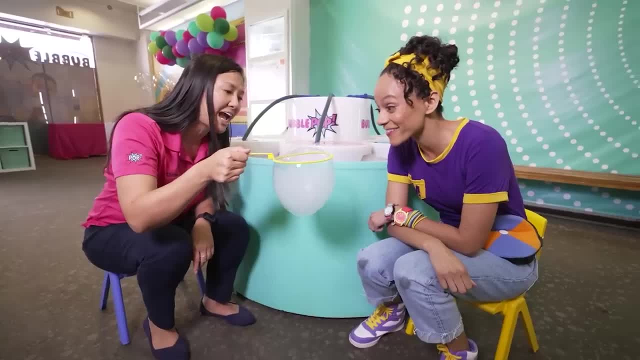 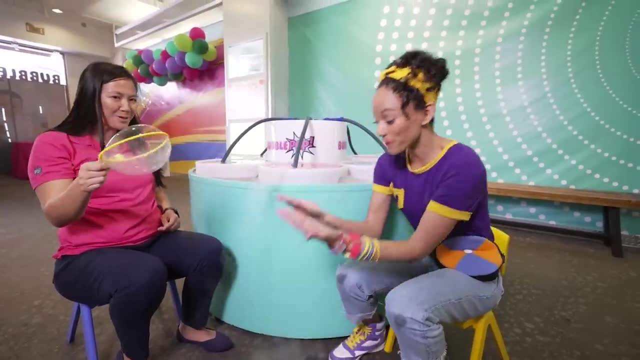 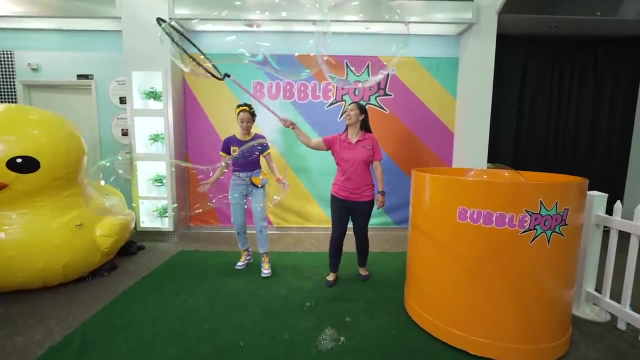 Right. So even though it's both air and gas, one is definitely heavier than the other. Yeah, and it's going to the bottom. Yeah, and then look, now you have a smoke-filled bubble. Oh Whoa, these are the biggest bubbles I've ever seen. 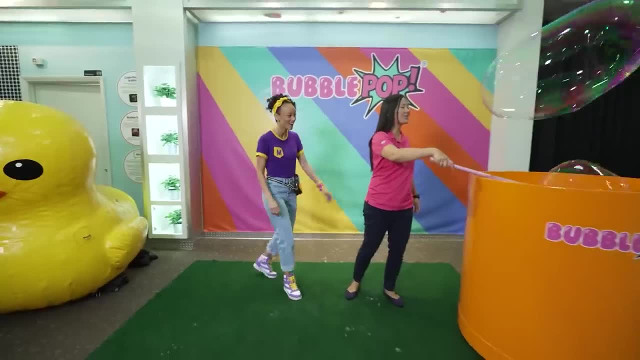 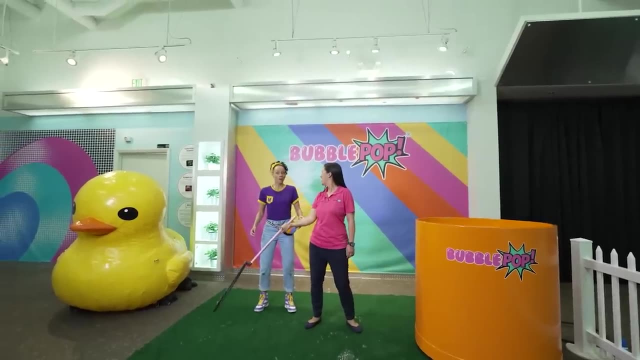 Ooh, Boob bubble hug. Yeah, that was cool. Do you wanna see something, Mika? Yeah, All right, I'm going to make a bubble arch. It's like a rainbow. All right, I'm gonna make one more, just for you, all right. 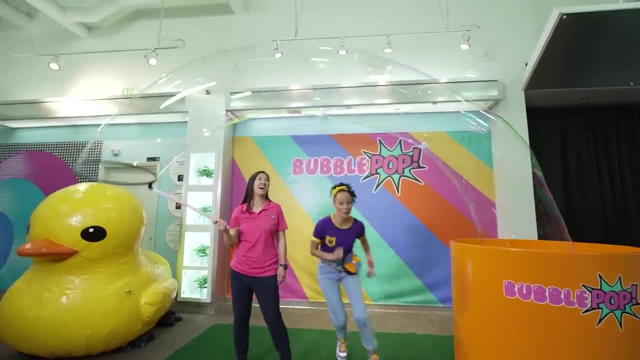 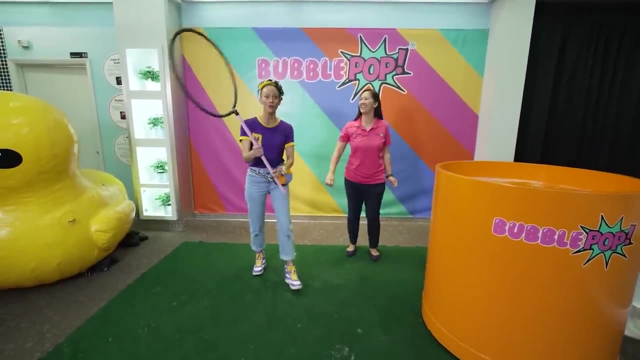 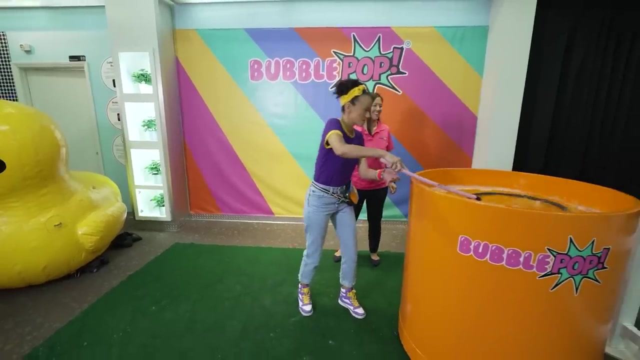 Thanks, Here we go. Oh Whoa, All right, do you wanna try? Yeah thanks, Oh look how big this bubble wand is. It's bigger than my head. All right, okay, get some solution on there. 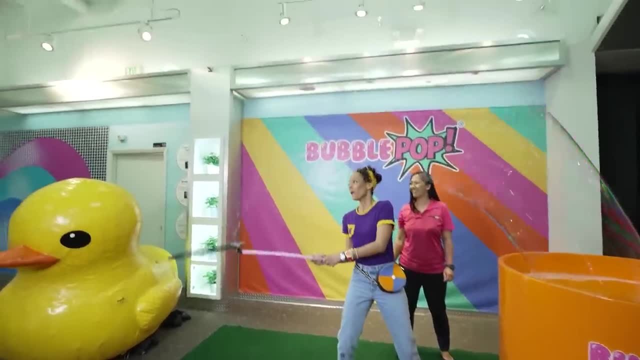 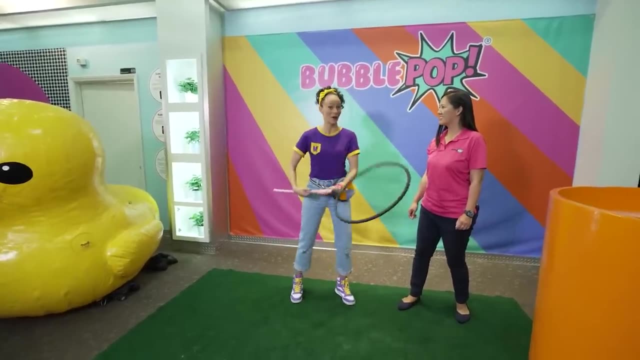 and whoa, Whoa, Whoa, it's so pretty. That was awesome, Great job, Thank you, and thanks for teaching me about bubbles and showing me all these cool bubble tricks. Yeah, no problem, I hope you're having a great time. 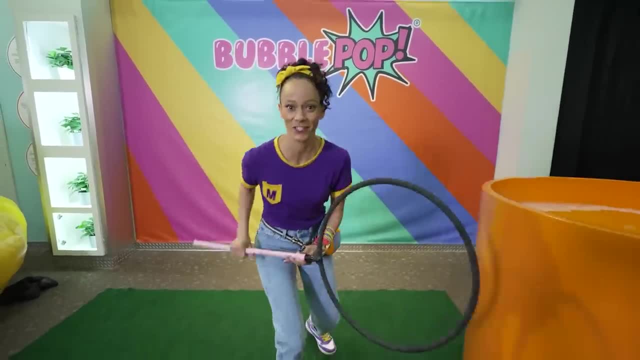 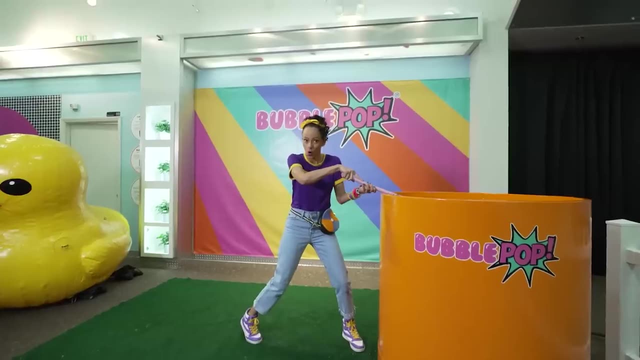 Oh yeah, Have fun. All right, I'll see you later, Okay, bye. Whoa, she knows a lot about bubbles. All right, I'm gonna do another arch Ready Three, two, one arch Arch. 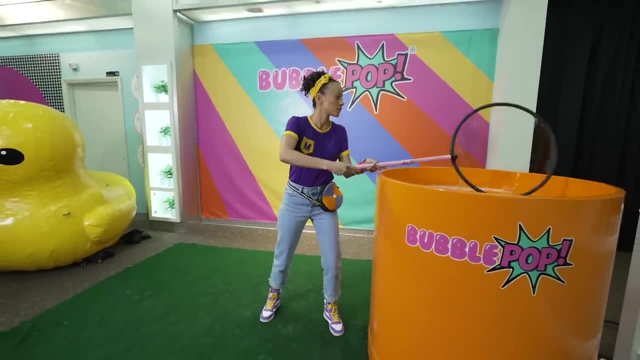 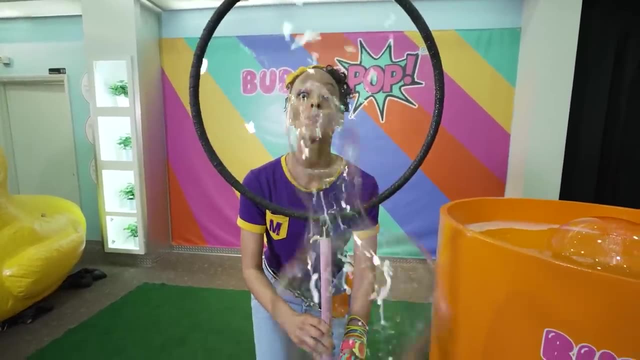 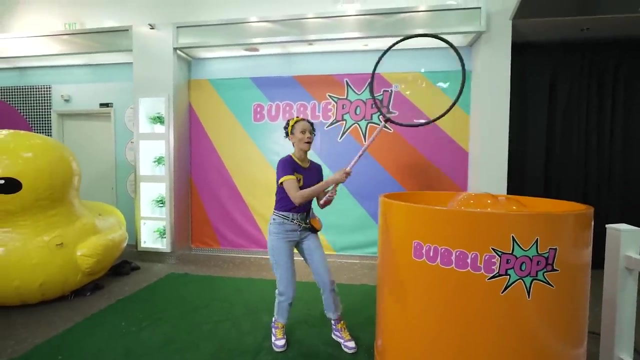 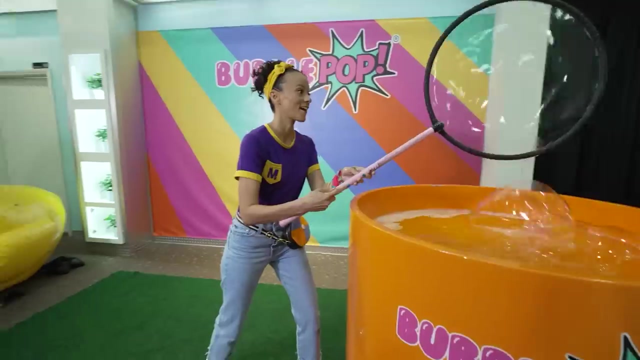 I wonder what else I can do with this big bubble wand. Whoa, look, It looks like a magnifying glass. Hello, Whoa, did you see that one? Oh, that one popped really fast. Whoa, that one popped fast too. 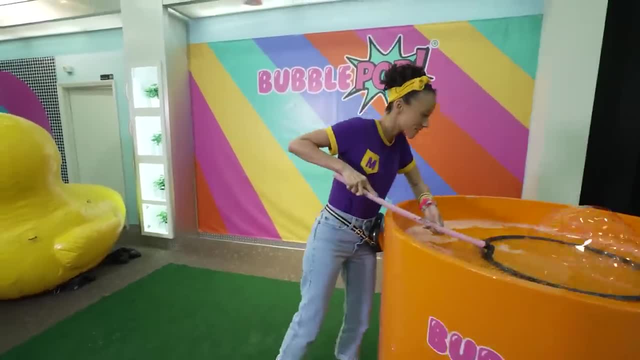 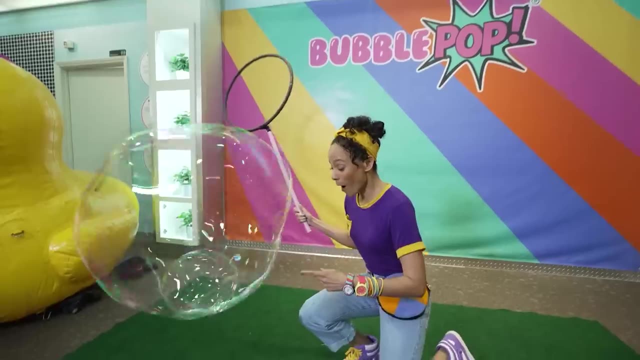 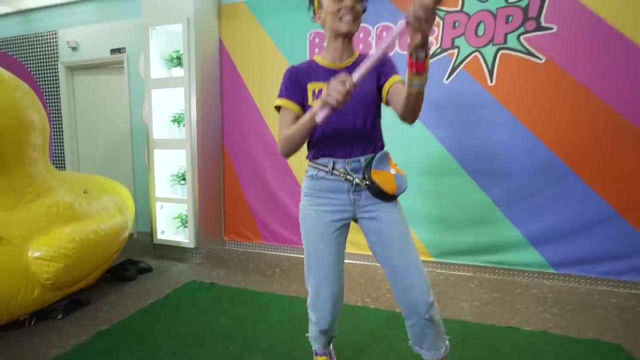 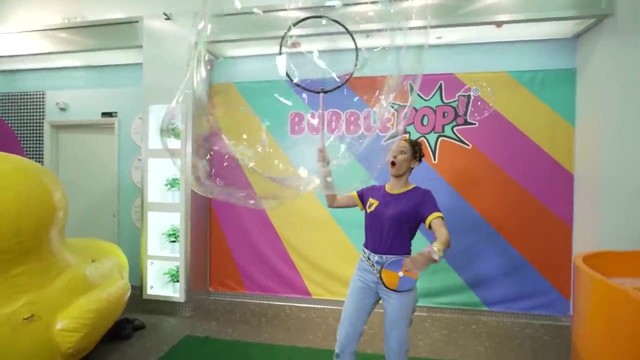 I wonder if I can make one that will stay and float a little bit Whoa Bubbles inside of a big bubble. Oh, that was amazing. Whoa, I could fit inside of that bubble, That's how big it was. 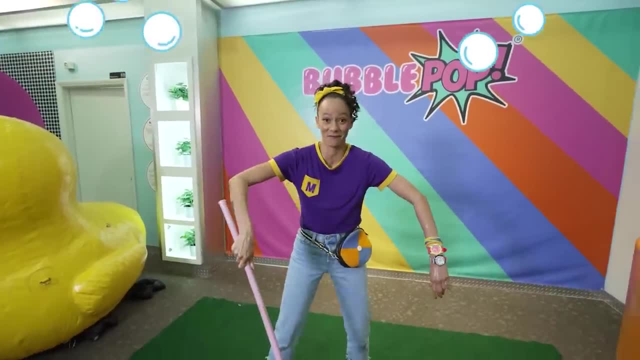 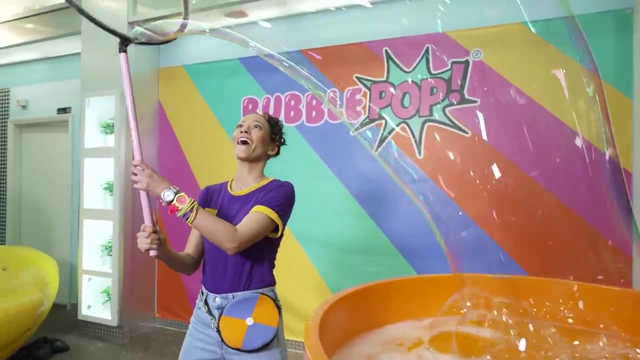 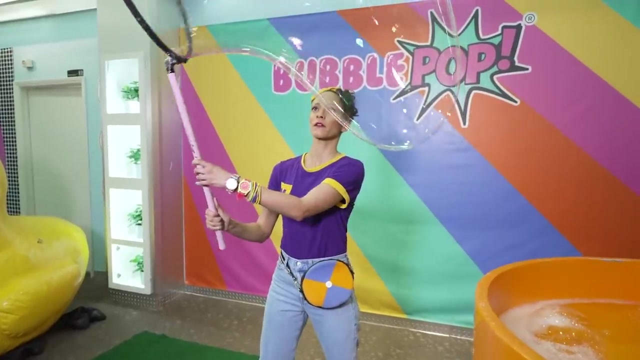 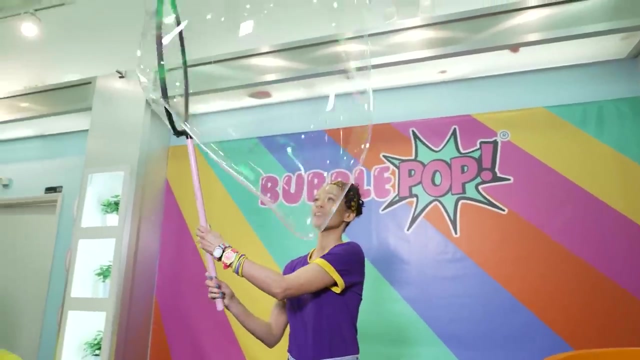 Whoa, it's raining bubbles on me. Whoa, I could fit inside of that bubble. That's how big it was. Whoa, it's raining bubbles on me. It's gonna make me a bubble like this. Who won? 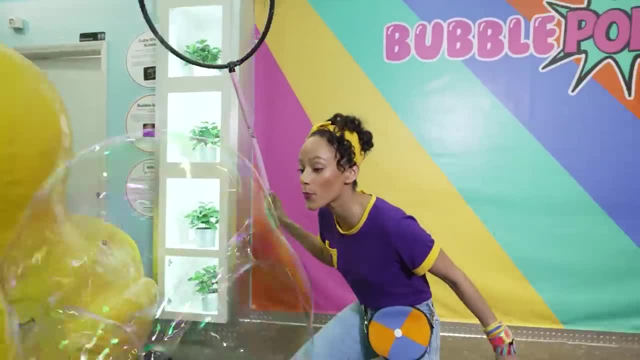 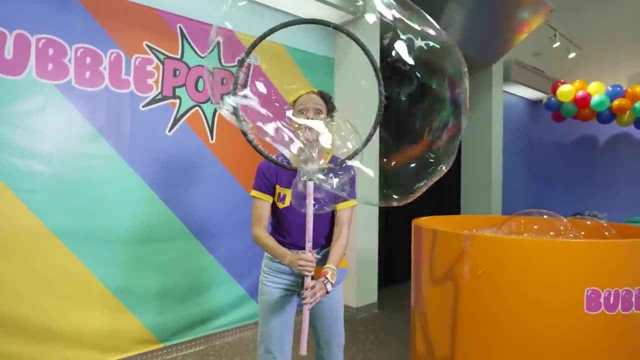 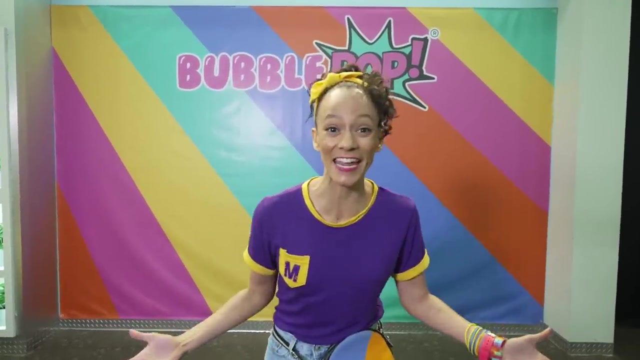 Who won? I'm gonna get my number. Okay, I'm gonna go get my number. Okay, It doesn't look too bad. Okay, almost finished. Okay, here we go. I can get my number. Whoa, You need a little chance to go away. 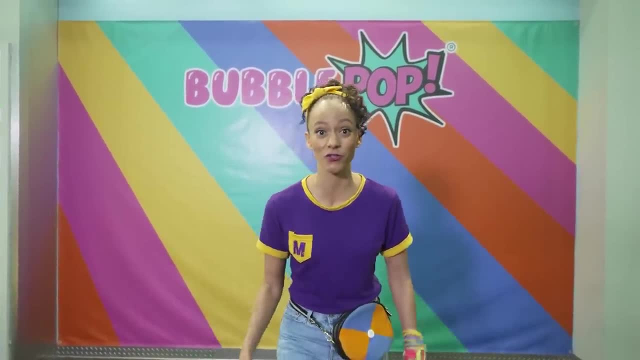 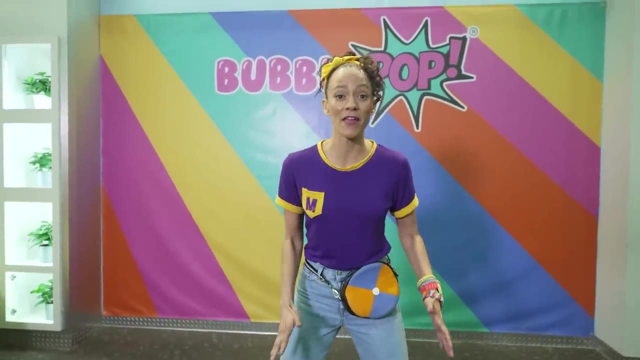 Something. Here it is. So it is Çaundererclawz, These Dwarfs, And I did like them. I'm so nervous. Alright, guys, What are you making to see that bubble tower that i made? oh, and my favorite was the big bubble arch. that was so much. 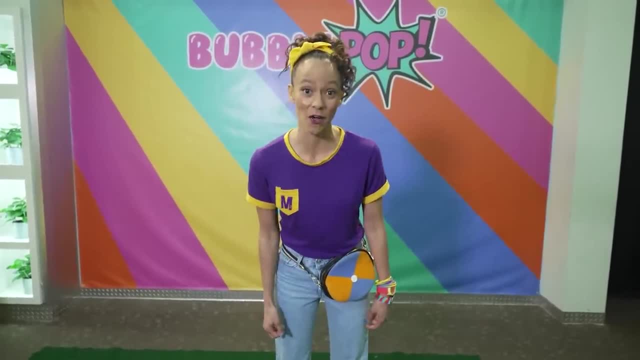 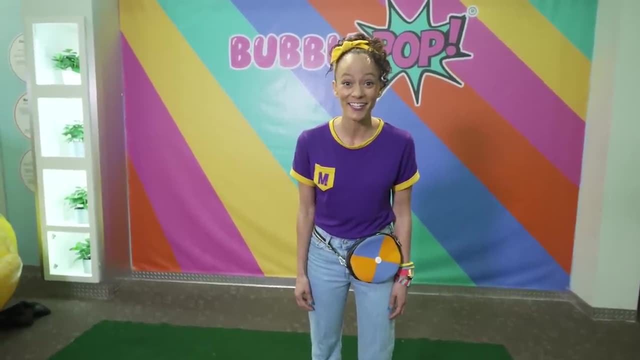 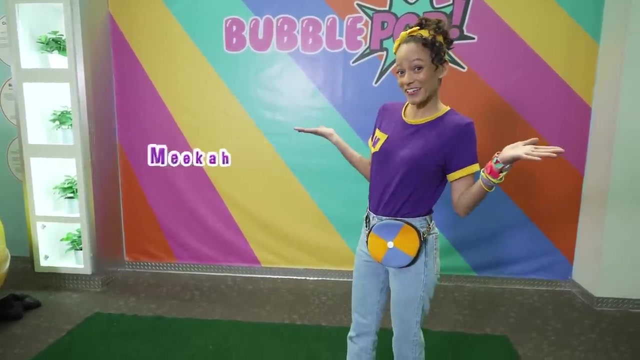 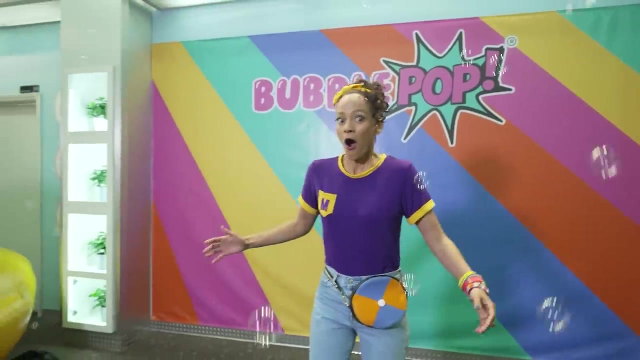 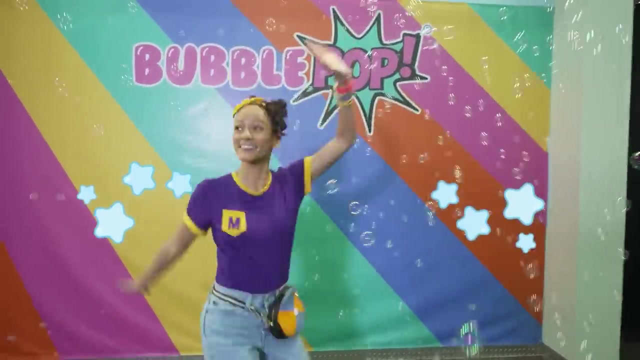 fun. well, this is the end of this video, but if you want to see more of my videos, all you have to do is search for my name. will you spell my name with me? cool, m-e-e-k-a-h. mika. well, thanks so much for learning with me today. a bubble dance party. let's dance. 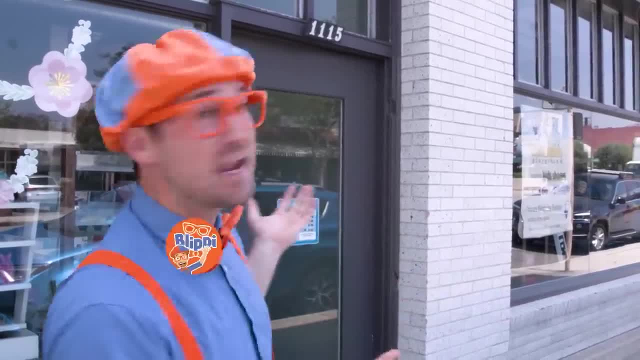 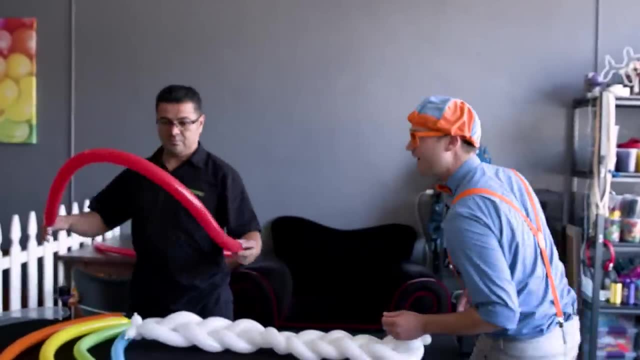 hello, it's me blippy, and today we're at amy's playground in South Pasadena, California. Come on, Whoa, Hey, who are you? I'm Brian the Volusionist. Ooh, that's cool. What are you doing? 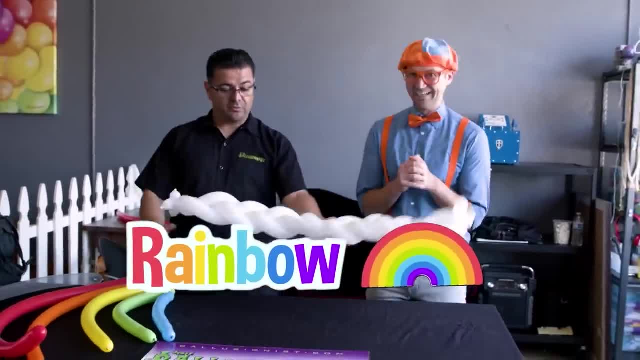 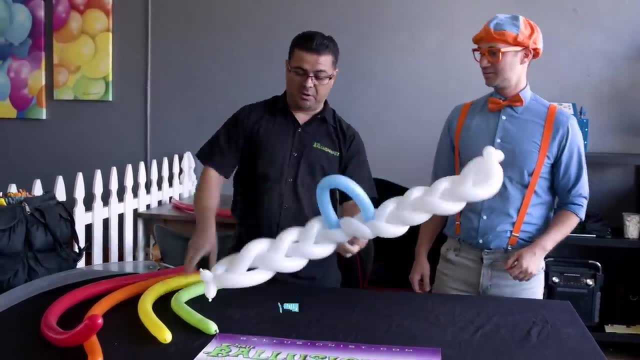 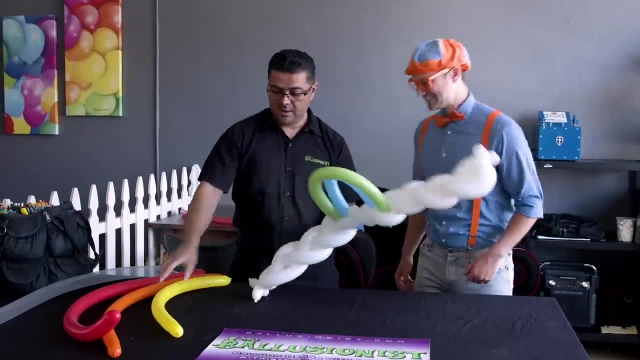 I'm building a rainbow, Ooh, a rainbow. First thing we need is a white cloud, Okay, A blue. I don't know what you'd call it, maybe an arch, A green one, Okay, Blue. Green Yellow, Okay, yellow, Just like. 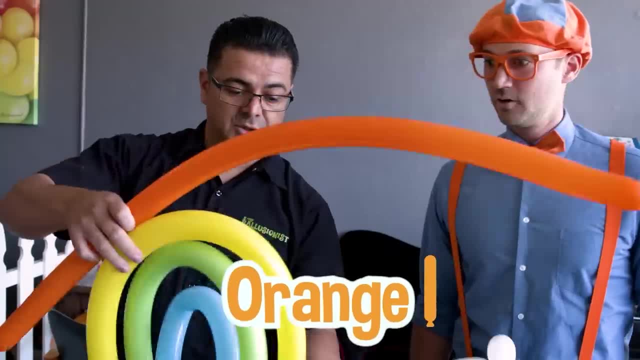 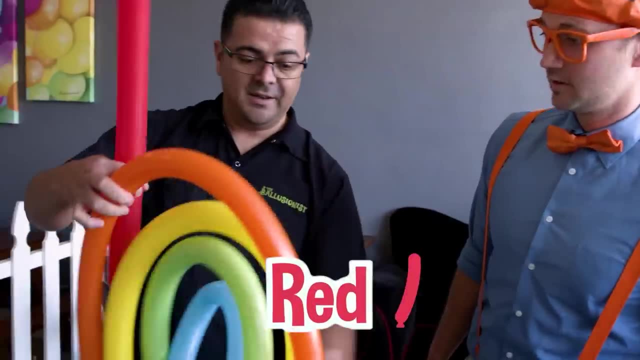 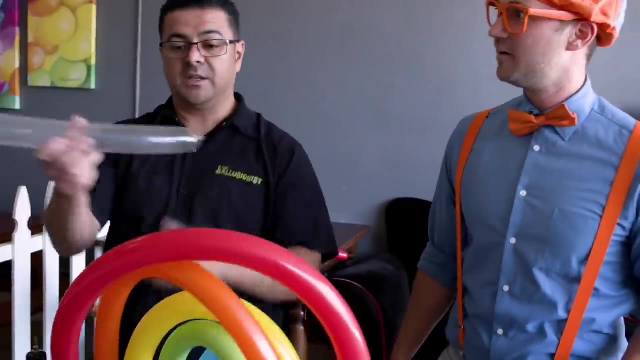 the color of the sun: Orange, Ooh orange. One of my two favorite colors, See Red, Ooh red. I love the color red too. And then we need clear for this extra special move right here. Ooh, what's he gonna do? 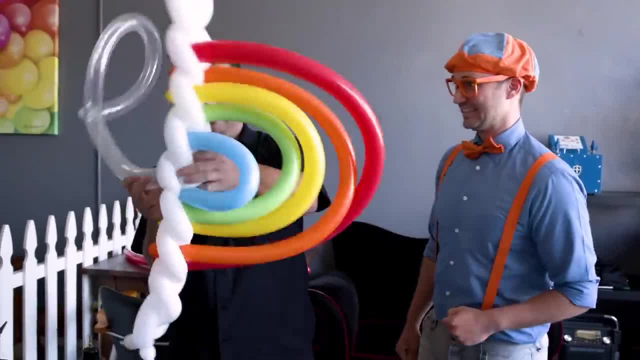 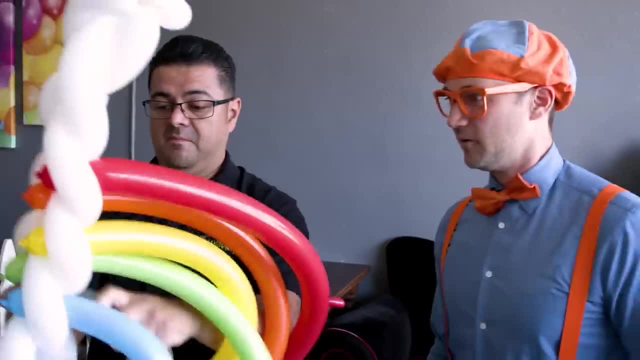 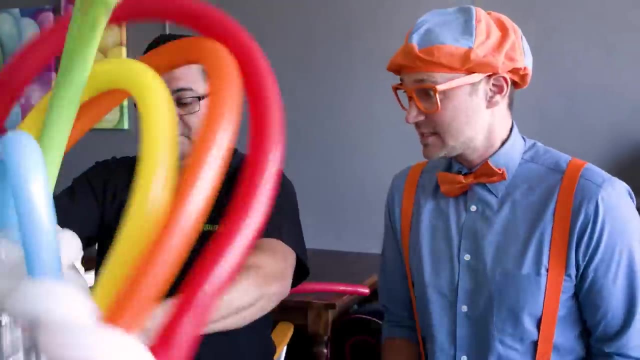 I don't know. I'm so excited. We'll find out, won't we? Yep, Whoa, Wow, I love learning my colors. This is the hard part. Okay, Here we go. Looks almost like it's complete, And there we have. 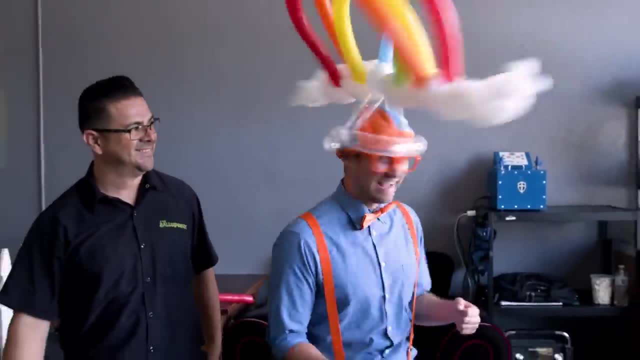 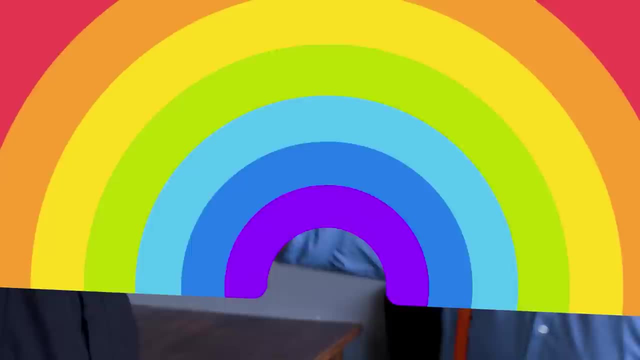 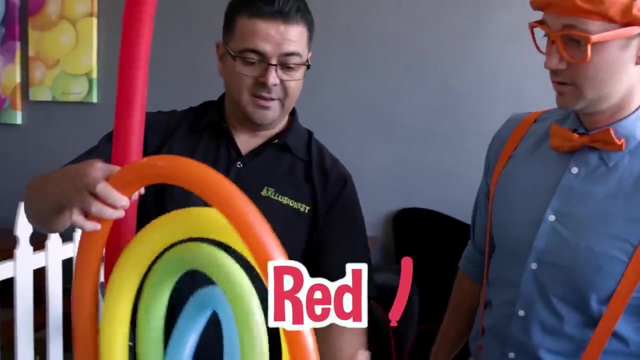 a rainbow. Oh, look at that, That looks so cool. Whoa, Hey, Woohoo. Well, thank you so much. Rainbows are fun. How many colors does this rainbow have? Let's see Red Orange. 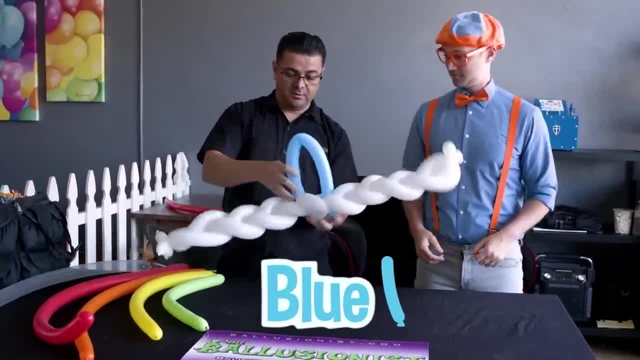 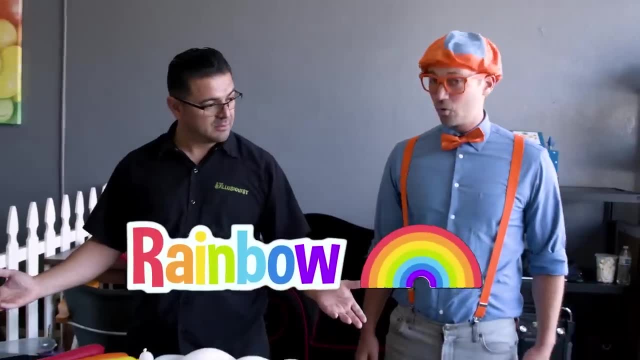 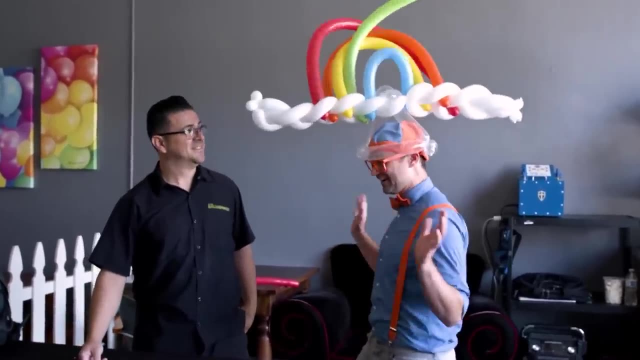 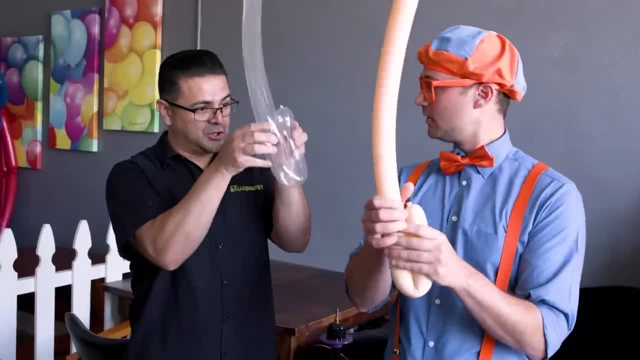 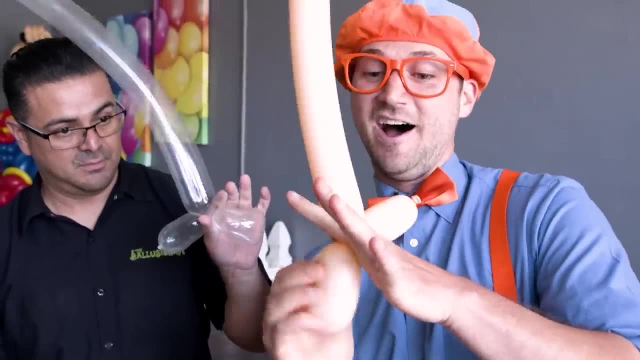 Alright, Start from here. Okay, Create sort of a U shape, Okay, And then tightly squeeze. The tighter you squeeze, the easier it is to twist. Okay, Whoa, Now we are gonna create another U shape, Alright. 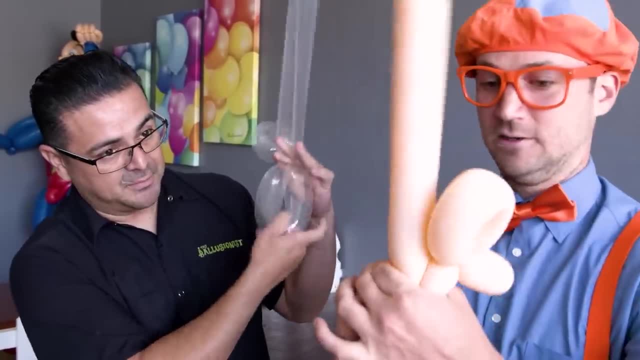 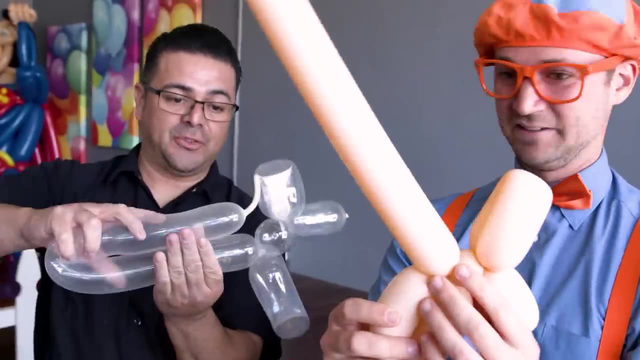 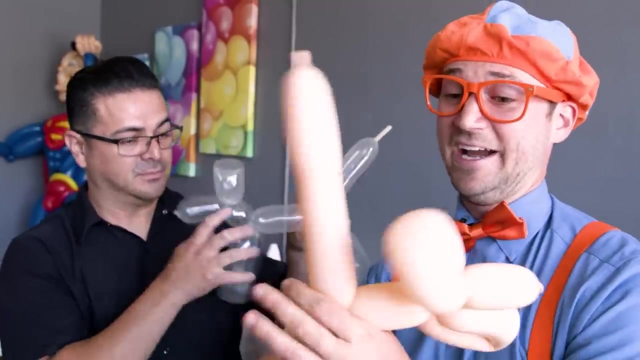 Tightly squeeze, leaving a bubble for a neck. Okay, This is fun. And then we are gonna fold the tail towards the neck, Create another U shape And tightly squeeze. Alright, I'm doing it Now. if you thought that was cool, why don't you place it on the table? 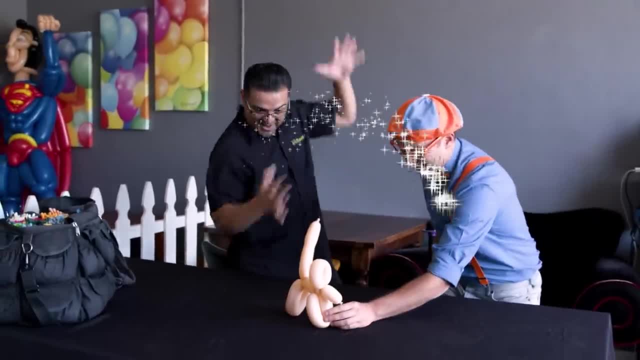 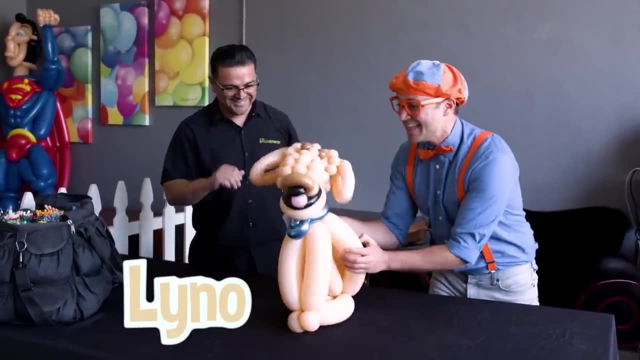 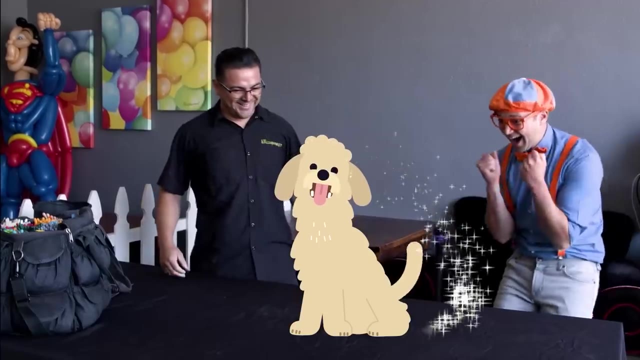 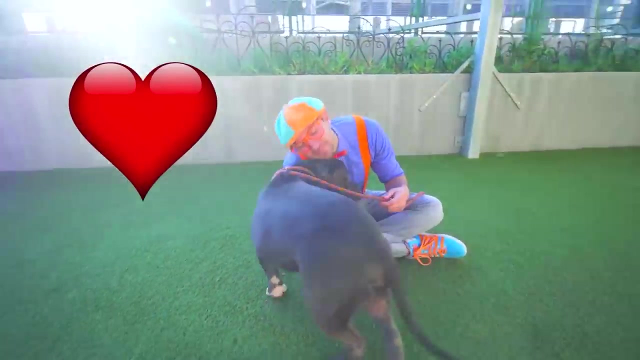 Okay, Awesome, Whoa, Look at it, That's my dog Lino. Hey Lino, That is so cool. If you think that was cool, what's this? Hey Lino? Whoa, I love dogs And puppies And kittens. 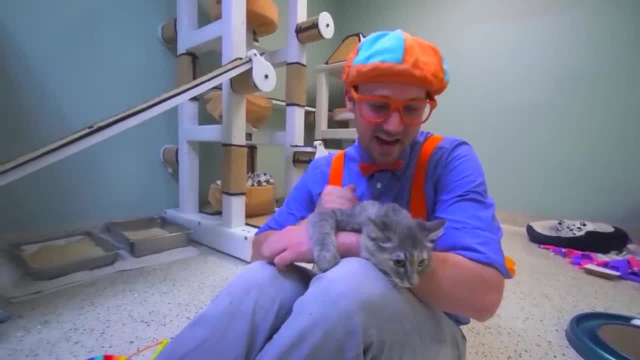 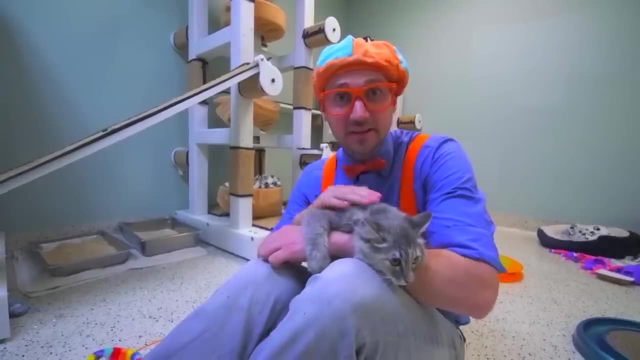 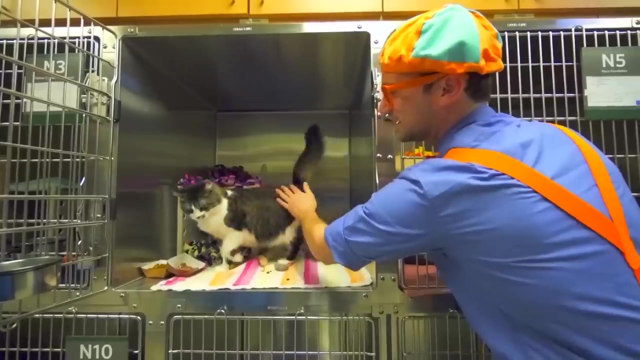 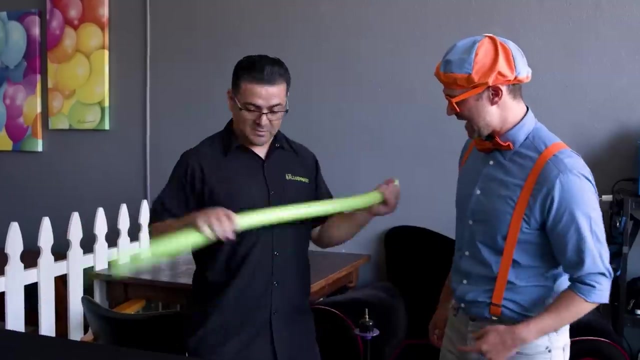 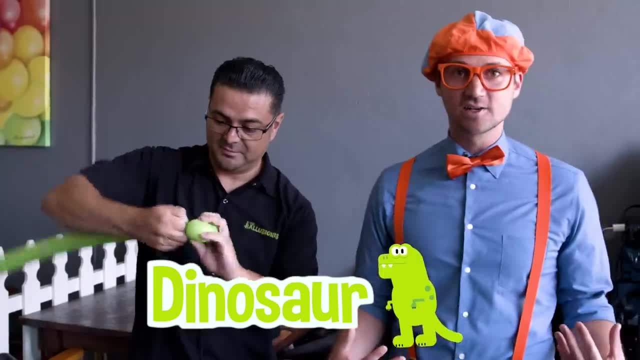 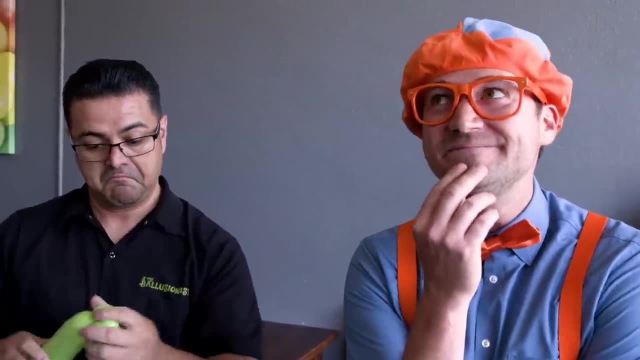 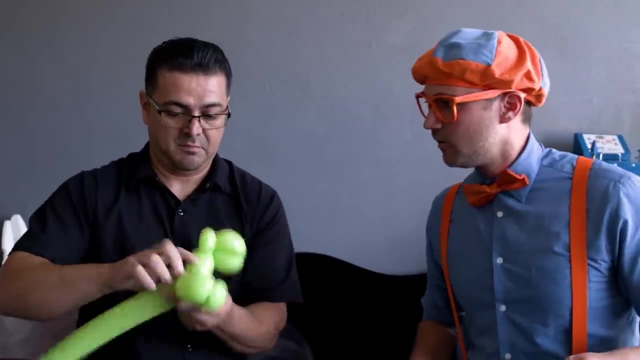 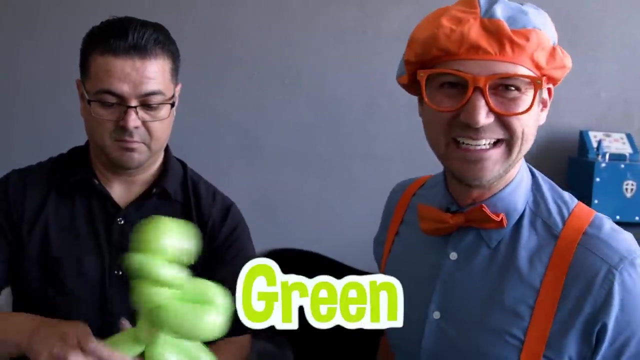 we can create a dinosaur, A dinosaur. I love dinosaurs. I wonder what one, my favorite dinosaur, is So silly? Whoa, Look at him Just twisting it. Whoa, Do you know what color that is? Yeah, A green dinosaur. 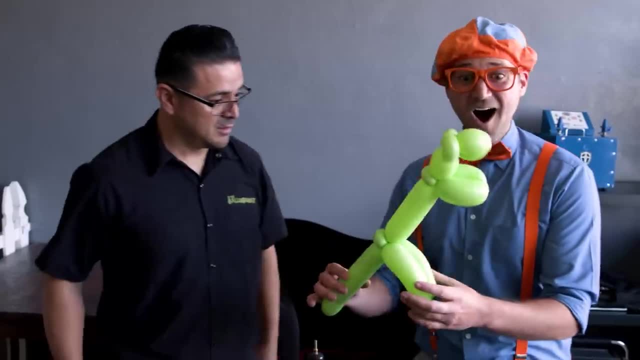 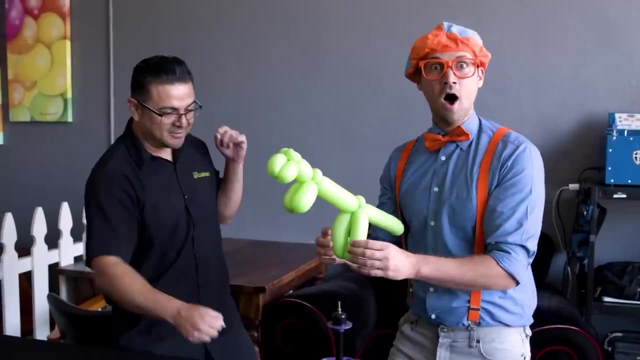 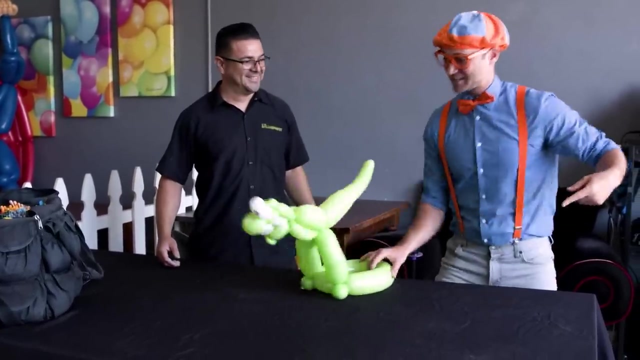 Whoa, There you are. Whoa, It's a T-Rex. Now, if you thought that was cool, place it on the table. Okay, Whoa. Oh, look A bigger T-Rex. That is so cool. Now, if you thought. 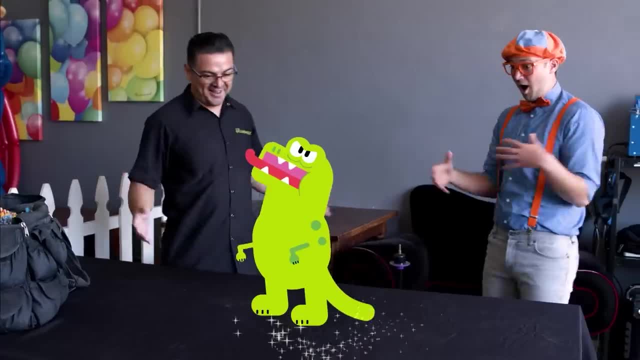 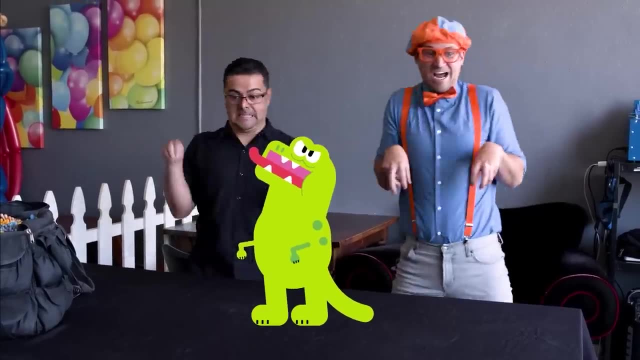 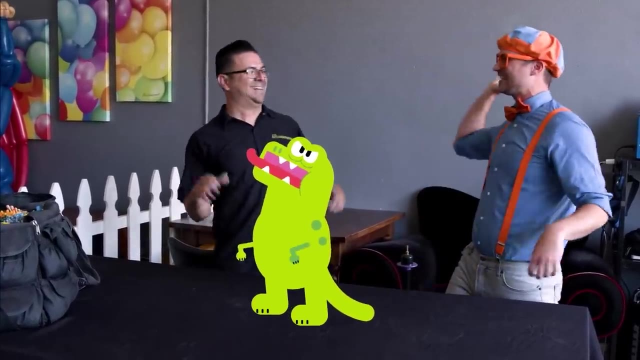 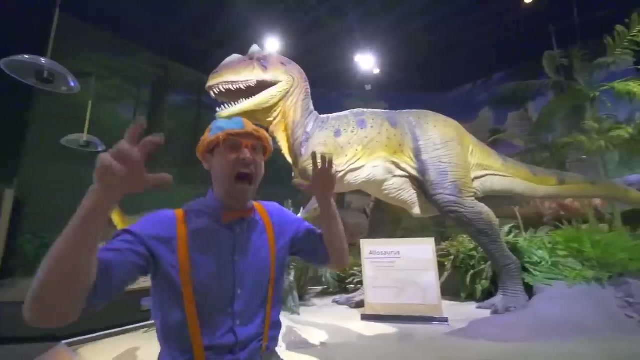 that was cool. check this out, Whoa. Let's act like T-Rexes together. Ready, That was so cool. Thank you so much. Whoa, What a scary T-Rex. Let's dance to this dino song. 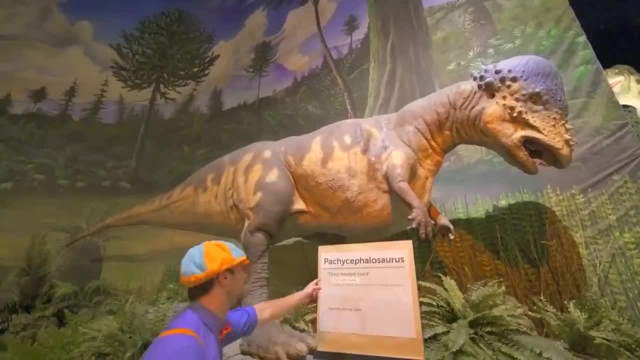 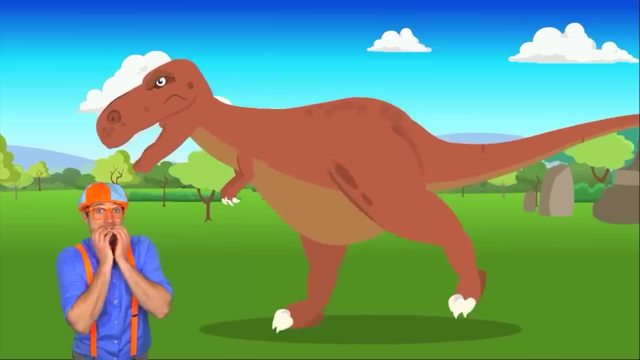 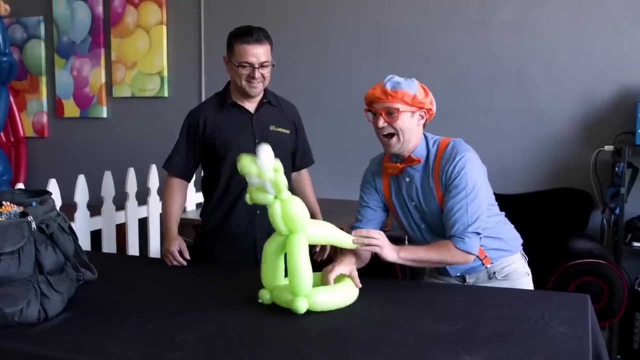 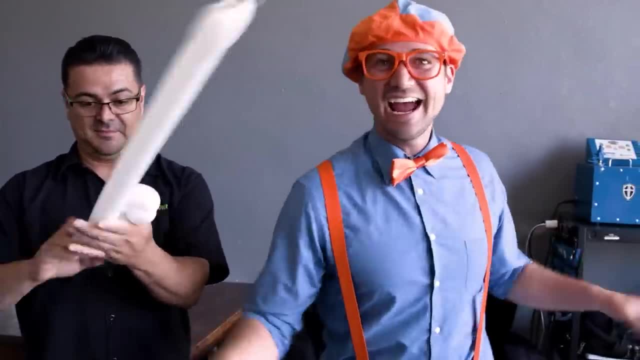 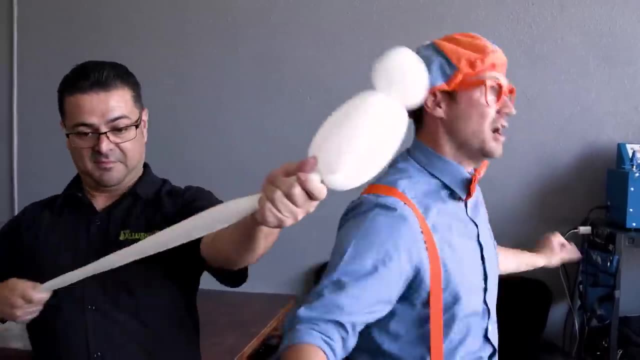 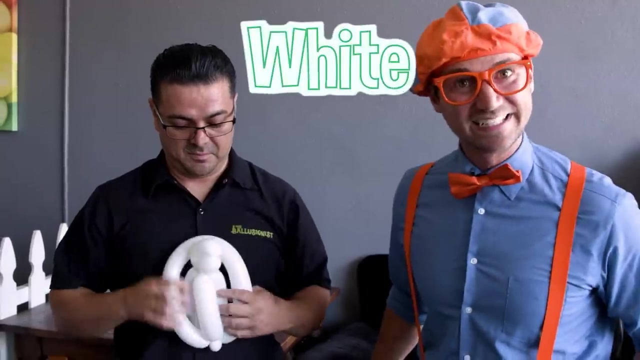 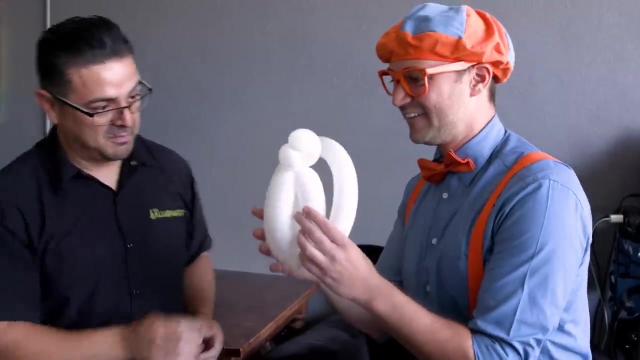 A parrot. Yeah, A parrot is a bird. I love birds. They just fly in the sky, And this parrot is the color white. That is so cool. Whoa, Look, It's a parrot in its cage. 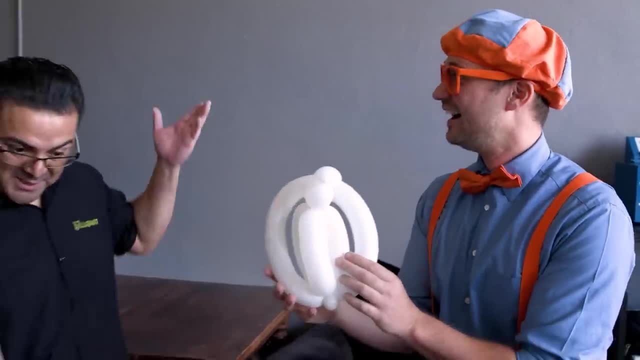 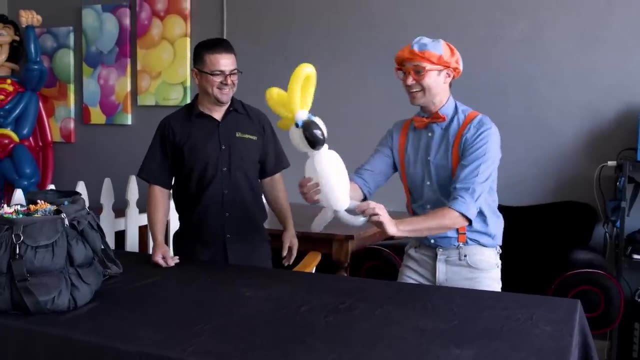 Caw-caw. That's so cool. Now, if you thought that was cool, place it on the table. Okay, Whoa, Look, It's even a bigger parrot now. Caw-caw, Caw-caw. 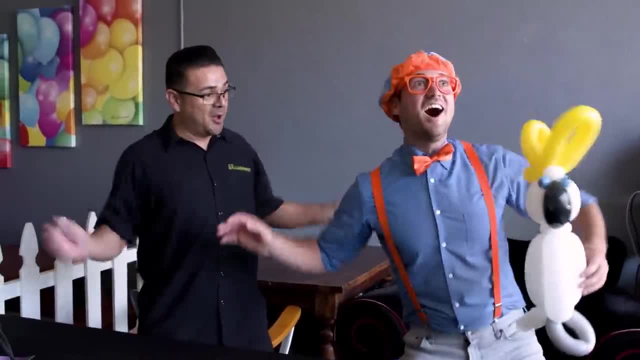 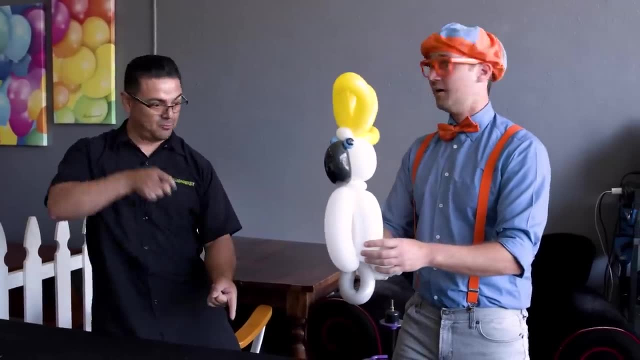 Will you act like a bird? Of course, Caw-caw, Caw-caw. We want a cracker. That's funny. Wow, This is so cool. Well, if you thought that was cool, round two Okay. 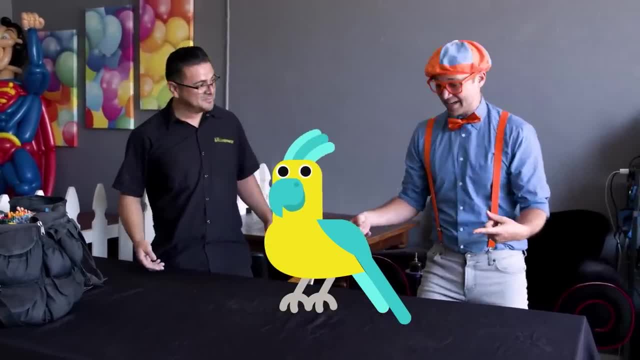 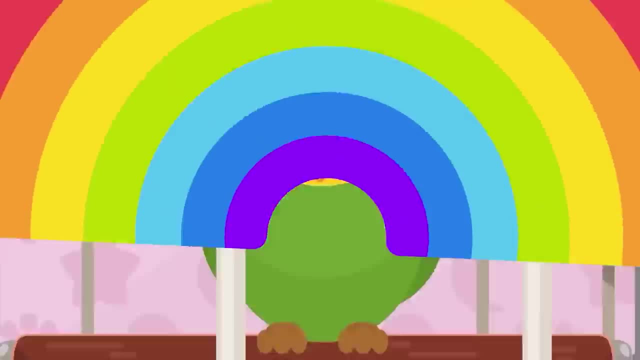 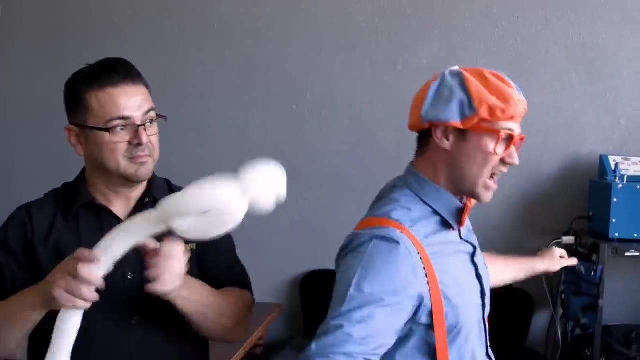 Whoa, Whoa. Look, It's a bird- Caw-caw, Caw-caw. See you later. Caw-caw. There are so many types of birds. They are so cool, They fly, And do you know what? 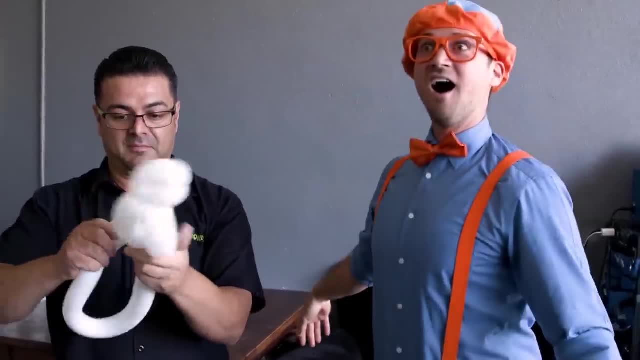 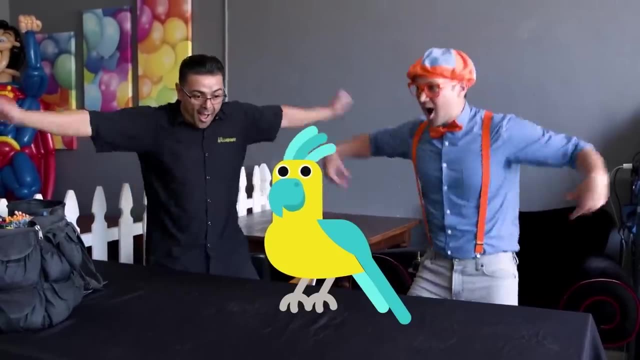 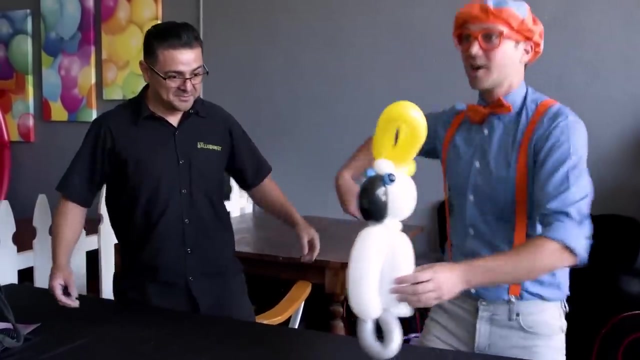 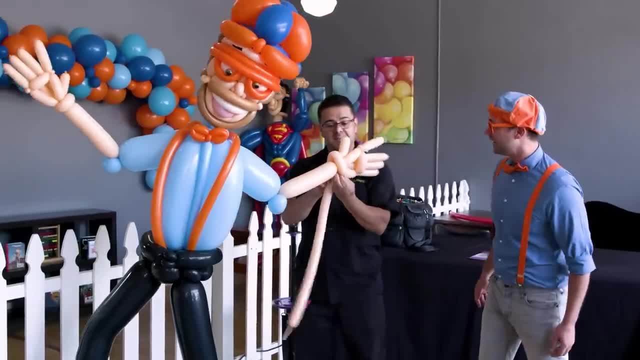 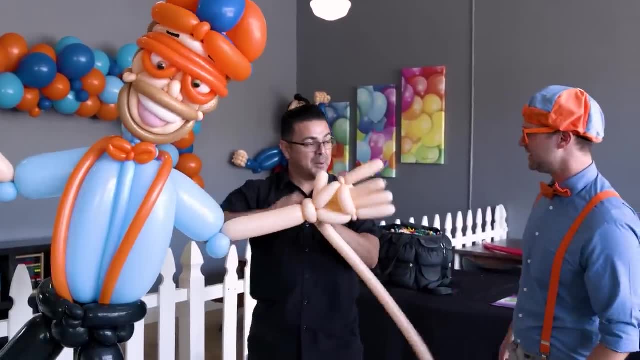 Caw-caw. What are you doing? Well, I was trying to make you out of balloons, but you couldn't stand still long enough for me to make it. That's silly. What was I doing? Jumping jacks, Jumping jacks, Really. 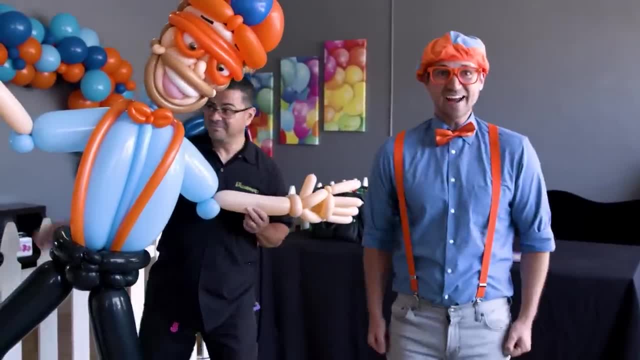 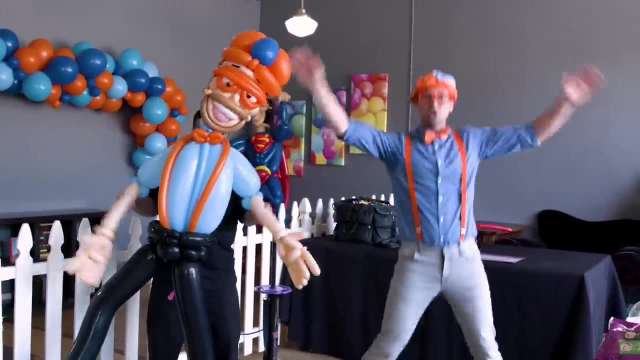 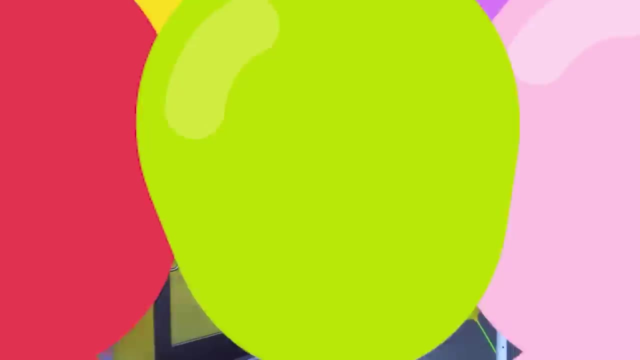 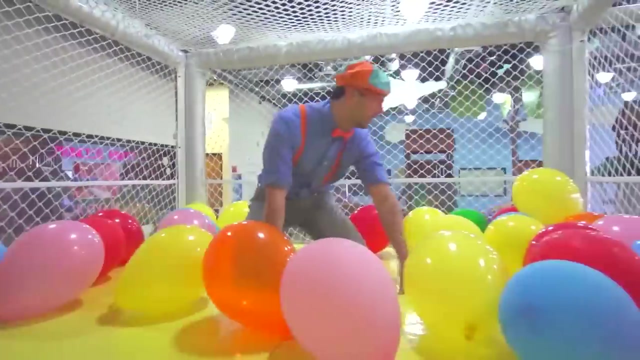 Will you do some jumping jacks with me? Ready, Here we go. Ha-ha, Yeah, Ha-ha, Whoa, Look at me go. Hey, Good job, Keep it up, I'm getting tired. Colorful balloons. 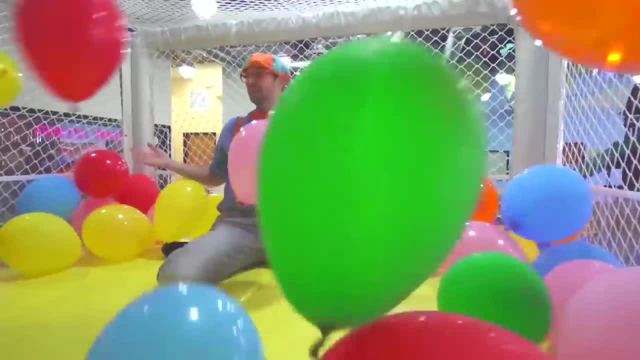 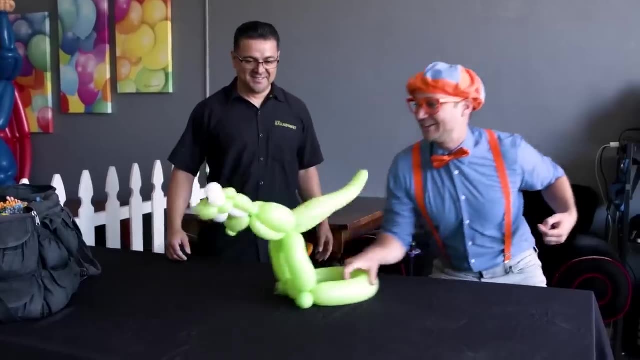 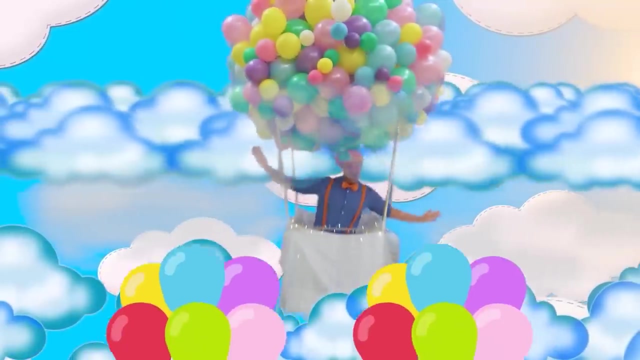 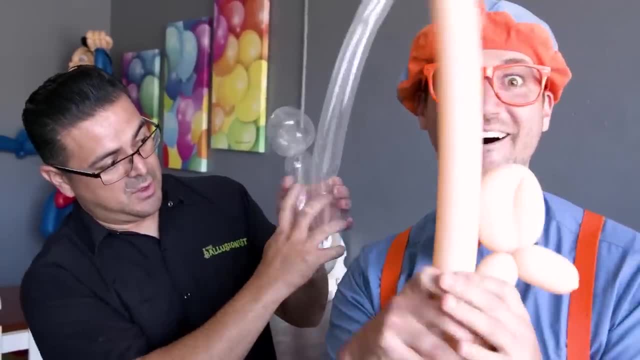 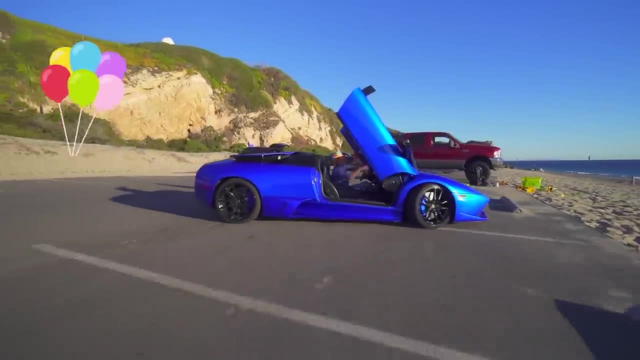 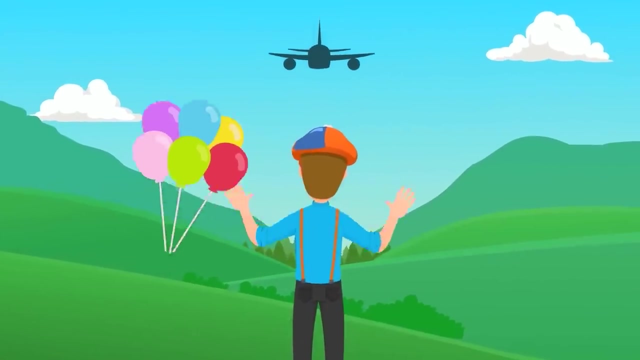 Don't bop them, They'll make a loud sound. Flying high and flying low. Let's see how far they're gonna go. Flying left, flying right, Flying far and out of sight. Colorful balloons flying high. Colorful balloons up in. 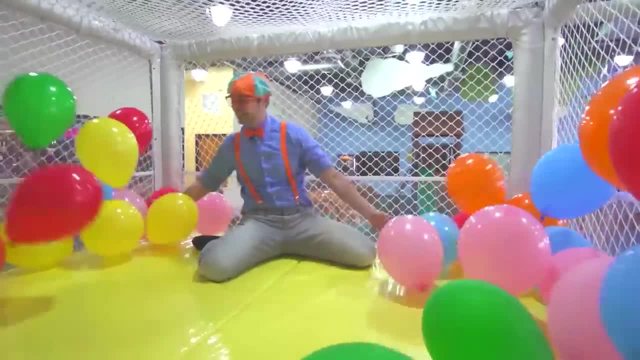 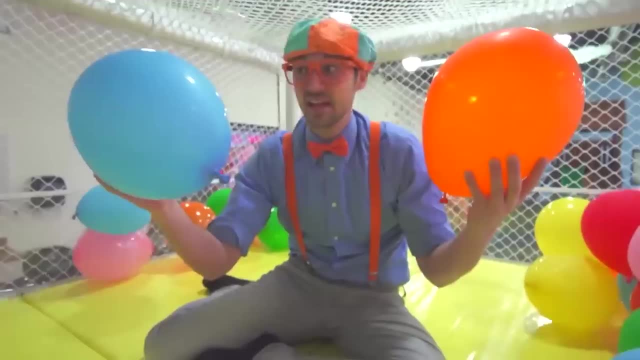 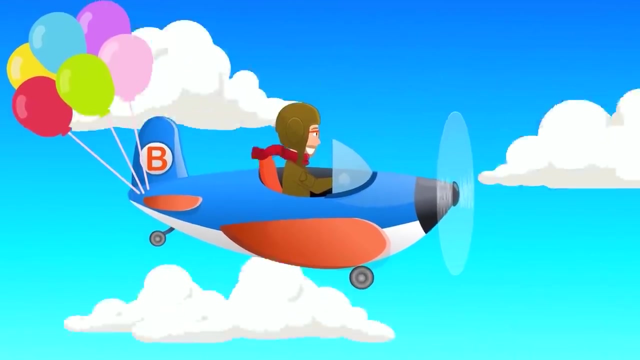 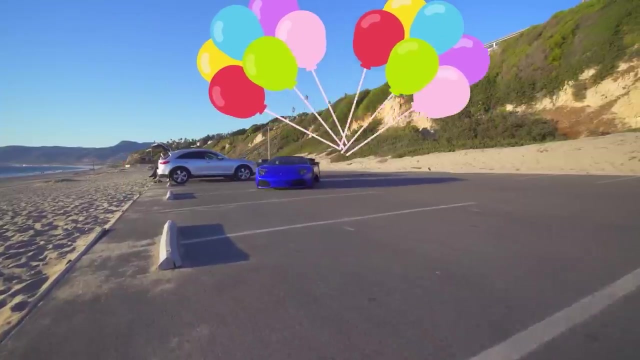 the sky. Colorful balloons, so many colors. What is your favorite one? Some are red and some are blue, Some are warm Orange- my favorite too, In the air Flying free Balloon fun for you and me. Flying high and flying. 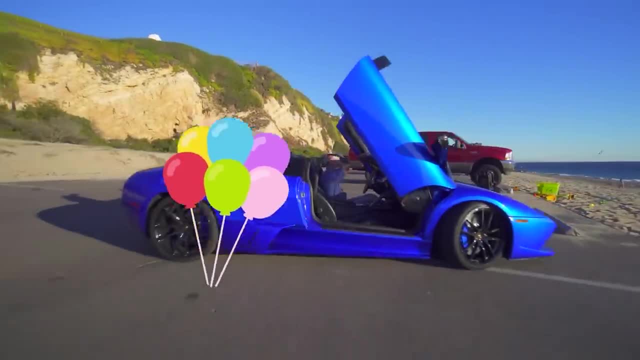 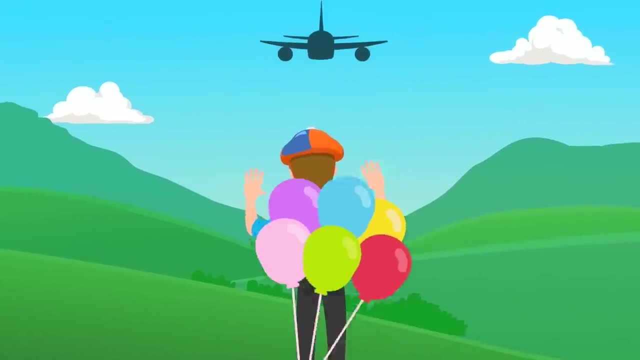 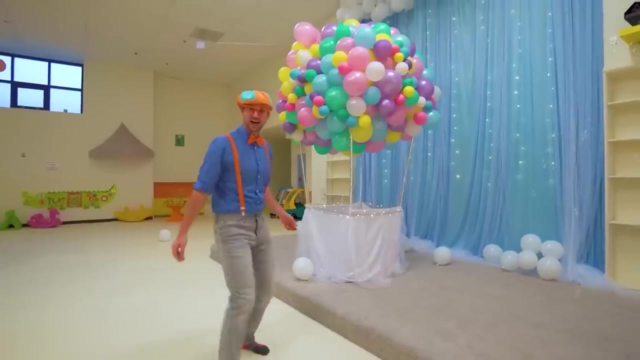 low. Let's see how far they're gonna go. Flying left and flying right, Flying far and out of sight. Now, how many colorful balloons can you see? Here we go: One, two, three, four, five, six, seven.